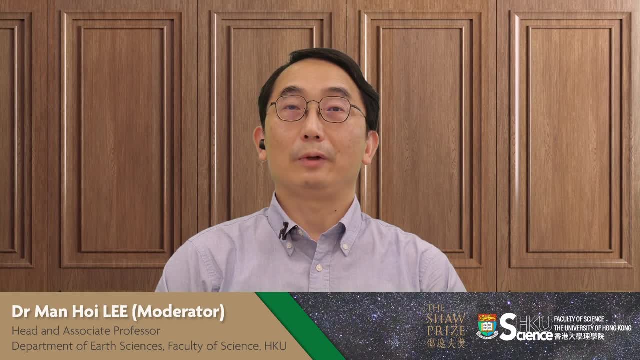 objects with far higher accuracy. The results from these missions offer an exquisitely detailed portrait of the distribution and properties of stars in our galaxy and of the celestial galaxies, as well as unique insights into its formation and history. These impact almost. 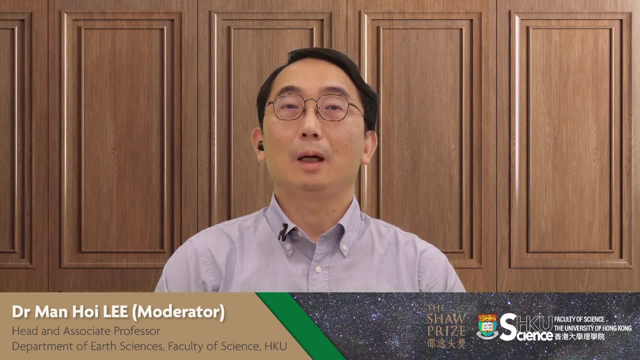 every branch of astronomy and astrophysics. Professor Leonard Lindegren originated many of the concepts of the Hipparcos mission design and was the leader of one of the two independent teams that carry out the data analysis for Hipparcos. He was a member of the Hipparcos science team for two decades. 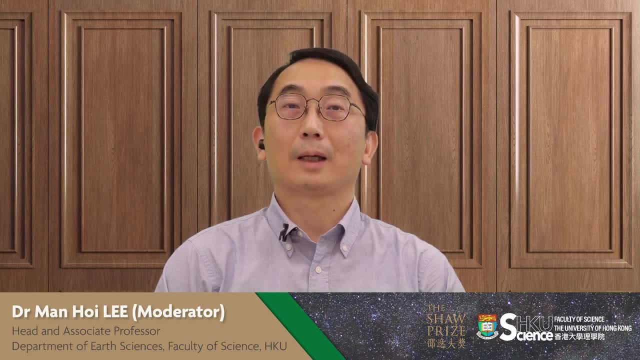 and the Gaia science team for two decades. after that, In addition to teaching science, he was also a member of the Hipparcos Space Aiming team, which includes the Hypparcos. after that, Professor Michael Perryman was Project Scientist for Hipparchos from 1981 to 1997,. 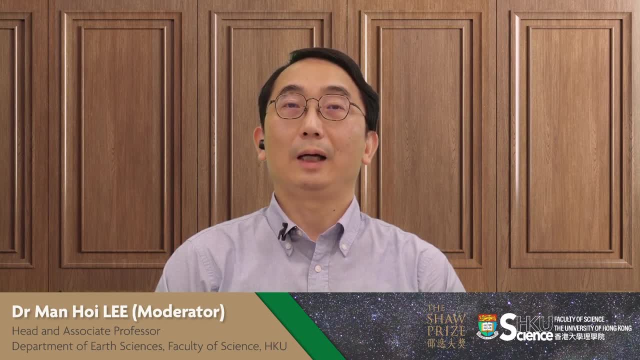 chair of the Hipparchos science team for the same period and lead author on the 1997 paper describing the Hipparchos catalog. He was also Project Scientist for the Gaia mission from 1995 to 2008,. chair of the Gaia science advisory group from 1995 to 2000, and chair of the Gaia science 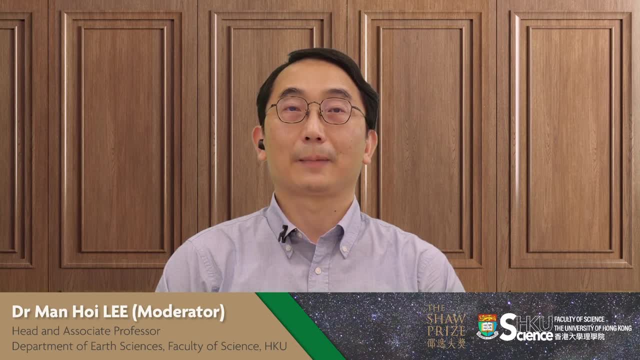 team from 2001 to 2008.. Professor Lindegren and Professor Perryman collaboratively proposed the concept for Gaia in the 1990s and were instrumental in its scientific and technical design. Before inviting our Shaw laureates to share their insights on space, 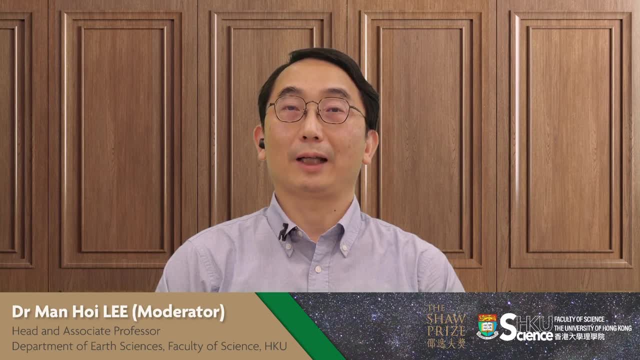 I would briefly introduce their academic background. Born in 1954 in Luton of UK, Professor Perryman is currently adjunct professor of the School of Physics at University College Dublin in Ireland. He received his bachelor's degree in mathematics and theoretical physics in 1976 and obtained a PhD in 1980 from the University of Cambridge, UK. He joined the 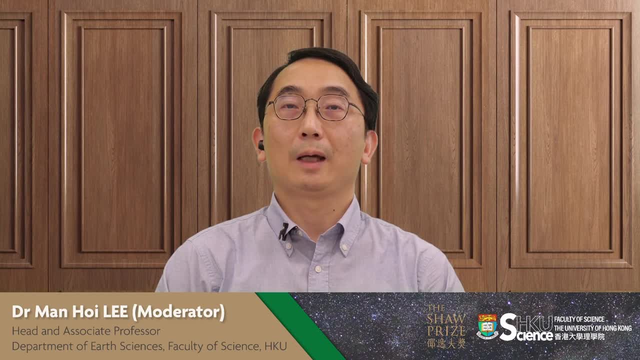 European Space Agency in 1980 and was nominated as Project Scientist for the Hipparchos mission and subsequently Study Scientist and Project Scientist for the Gaia mission. During his service in ESA, he has been professor of astronomy at Leiden University in the Netherlands. He held a 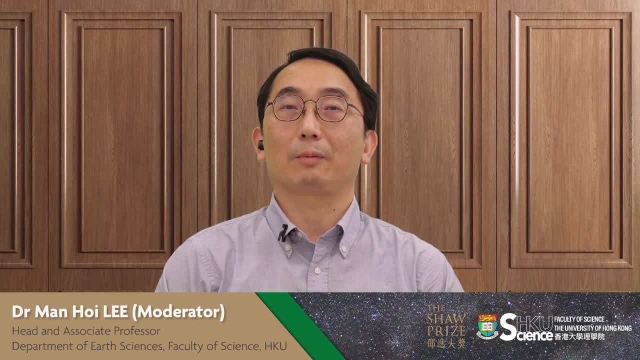 joint position at the University of Heidelberg and the Max Planck Institute for Astronomy, Germany, in 2010.. A year later, he became a university lecturer at the University of London in 2010.. He Later he joined the University of Bristol in UK as Visiting Professor of Physics. 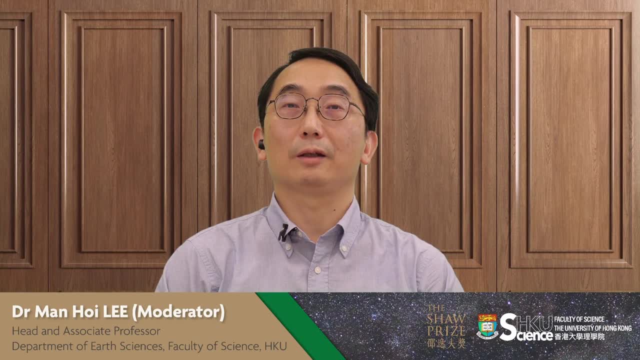 He has been Adjunct Professor at the University College Dublin since 2012.. In the upcoming lecture presented by Professor Perryman, he will look at the scientific aspects of this exciting journey. First, he will put their modern space measurements in the historical context and summarize what 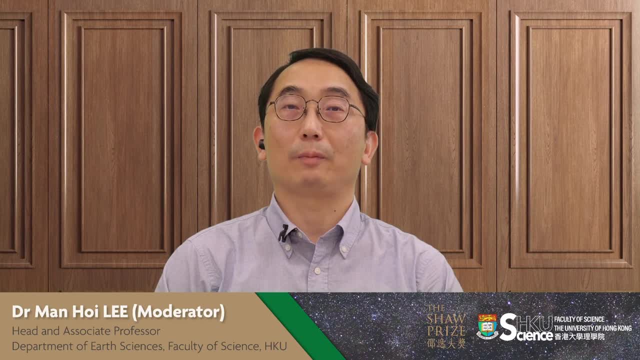 astronomers have learned from measuring the positions of celestial bodies over the past few hundred years. After that, a few of the remarkable scientific advances which are resulting from the extremely accurate measurements of positions from space, and also a little of what this is telling us about our place in the universe, will be covered. 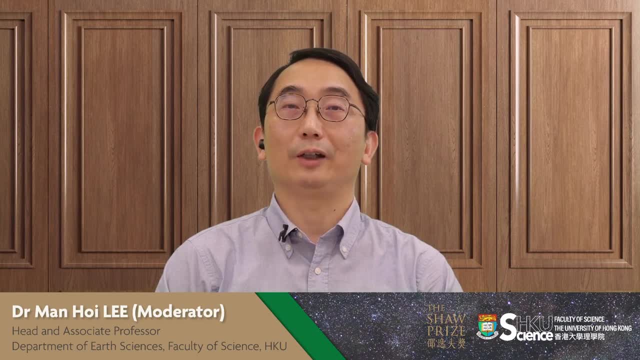 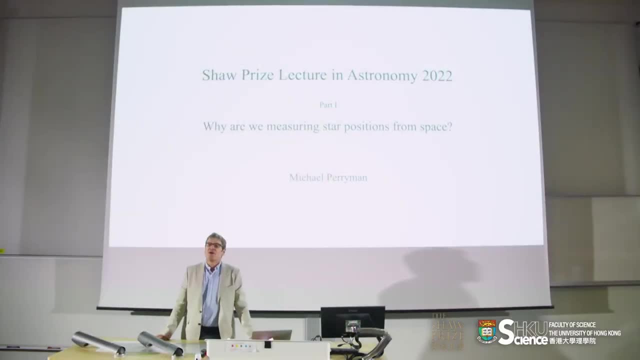 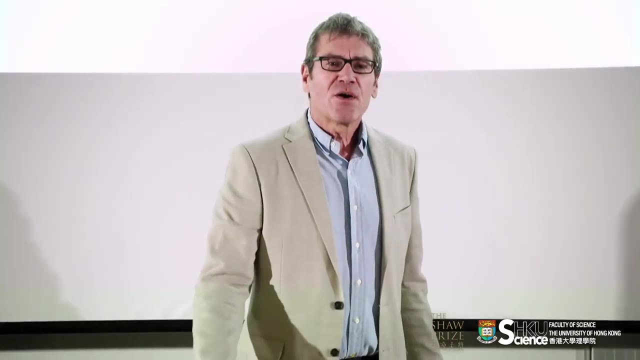 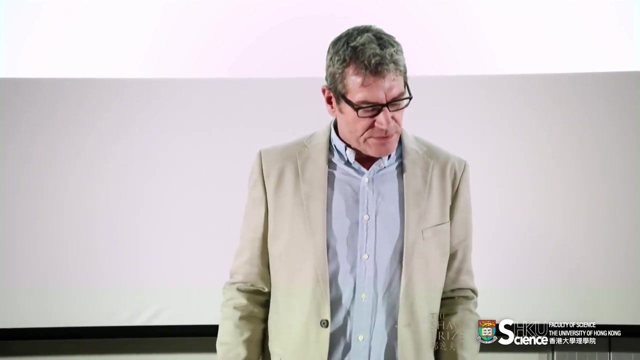 Now let us join Professor Perryman's lecture in this exciting field. Professor Perryman, Thank you for the opportunity to give this Shaw Prize Lecture in Astronomy 2022.. My colleague Leonard Lindgren and I are going to split this introduction to the projects that concern us into two parts. 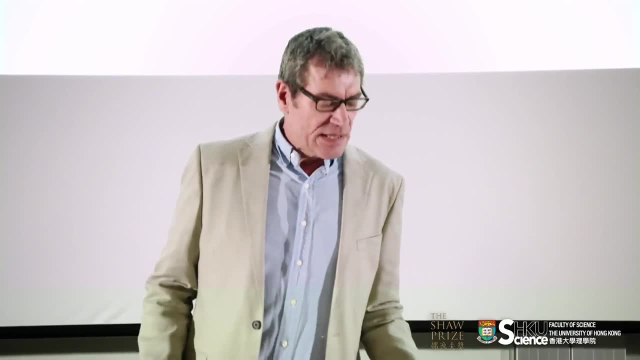 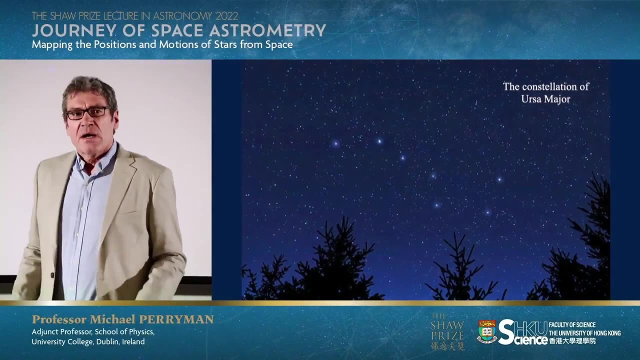 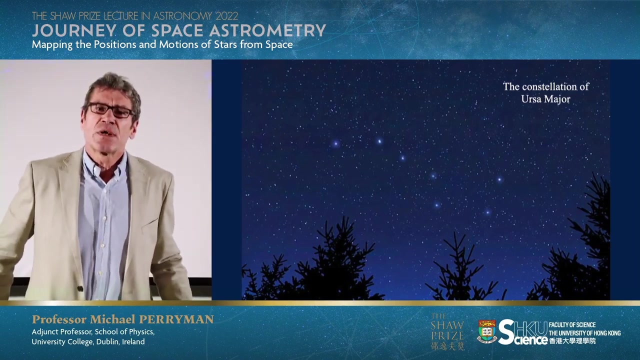 And my part, the introductory part, is to tell you why we are measuring star positions from space. Imagine you are looking up into the night sky and the well-known constellation of Ursa Major, and it will look the same to you now as it did to humanity 10,000 years or even. 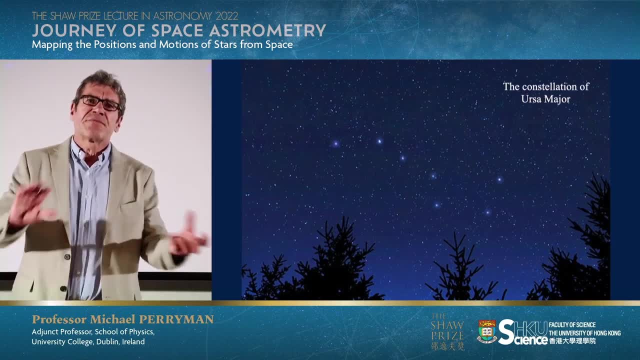 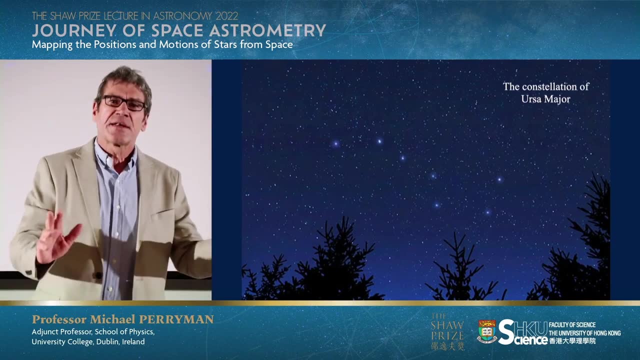 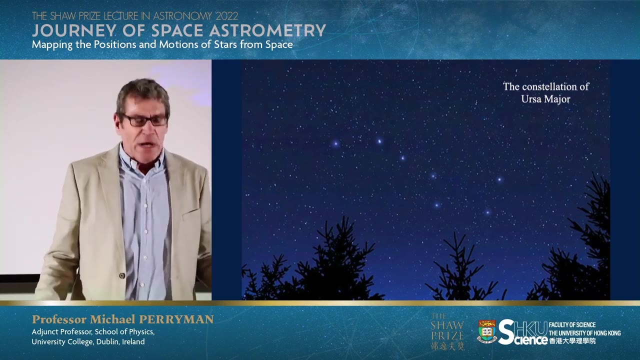 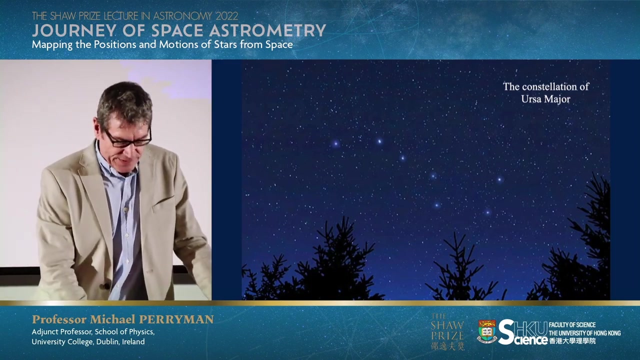 100,000 years ago. The heavens rotate, night after night, as the Earth spins on its own axis, but the stars stay stationary one with respect to the other. Amongst them moving stars, The moon, the sun, the moon and the small number of planets that were known to them. 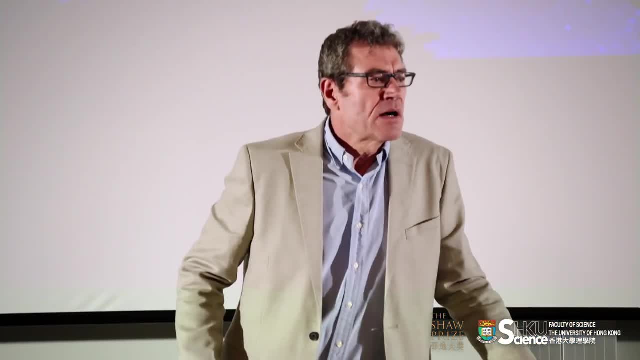 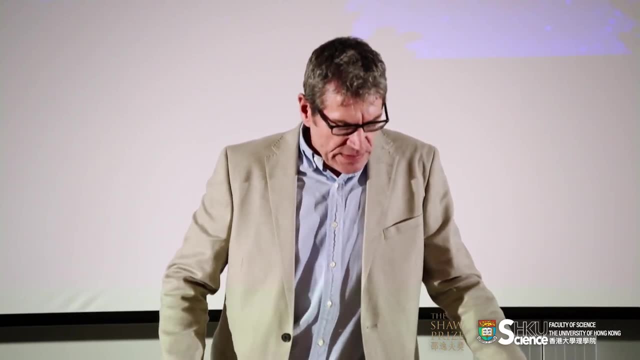 at the time. How far are these stars away from us? What do they tell us? What are these stars? What is the nature of the universe? This has been a subject of scientific inquiry for 2,000 years, since the time of the ancient. 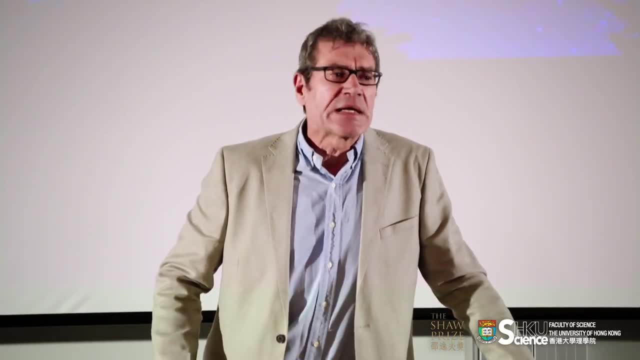 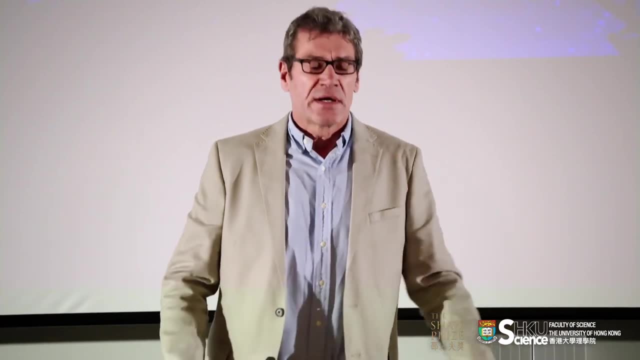 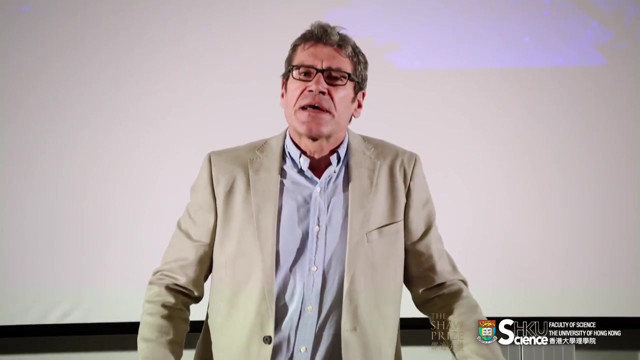 Greeks. Surprisingly, it was only less than 100 years ago that we knew what the stars were, what fuelled them, what powered them, But over the course of the past 400 or 500 years, there has been a great advance in understanding. 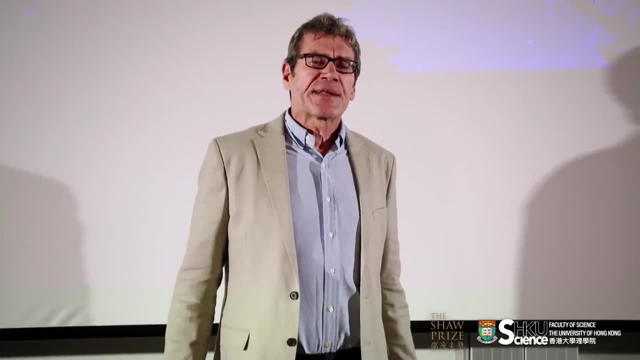 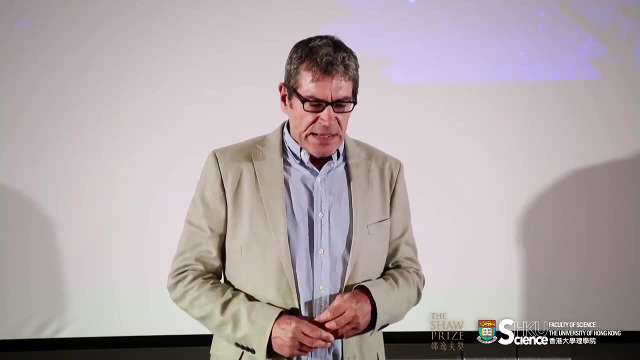 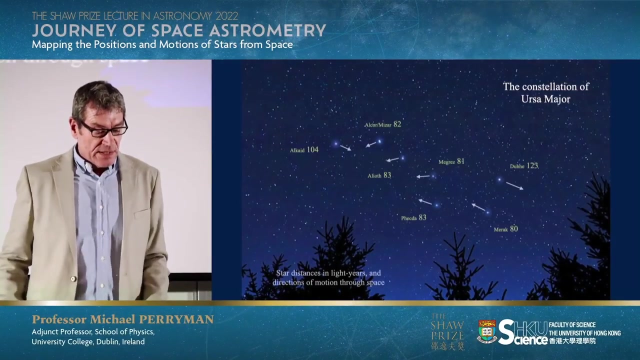 their distance, how they move through space, and this has told us, in turn, an enormous amount about the nature of the universe around us, And what we know today, for example, is that the stars in the Earth's atmosphere have a major constellation and not all at the same distance. 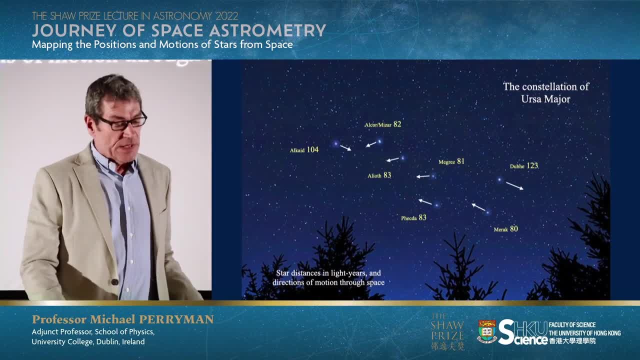 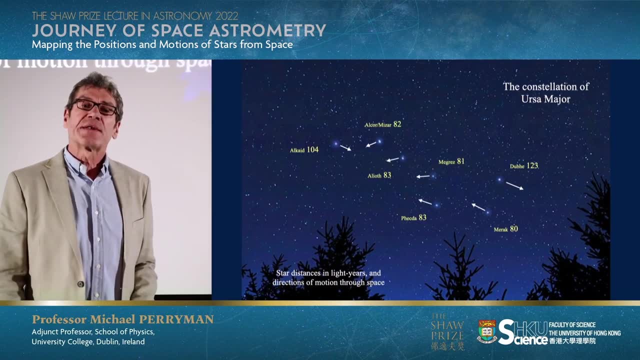 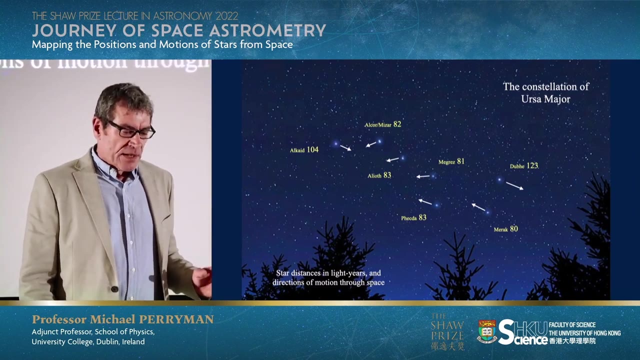 They are in light years. I've put the numbers here about 80 light years, but notice Al-Qa'id on the left and Dubey on the right are about 120 light years, much more distant, And they're moving in different ways as well. 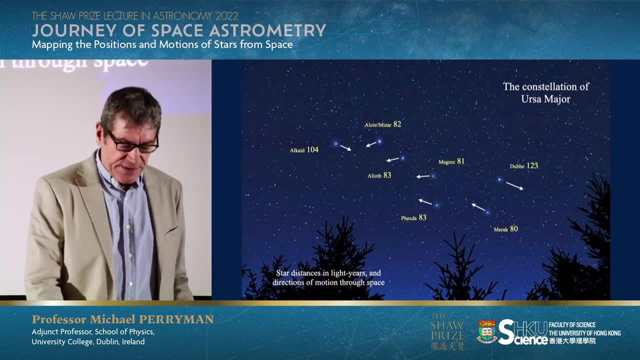 So, although they're moving, space is so vast that even at the end of their life, our lifetime, the constellation of Earth's atmosphere is still moving. So, although they're moving, space is so vast that even at the end of our lifetime, the 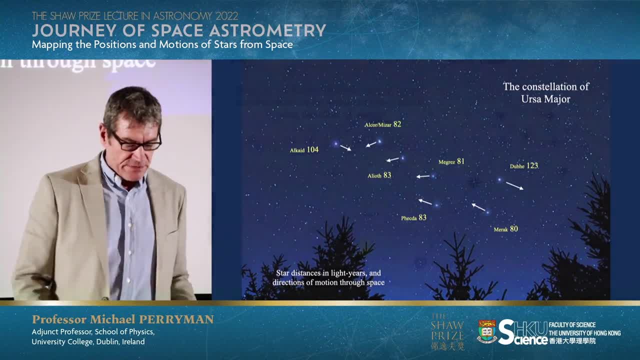 constellation of Earth's atmosphere is still moving. So, although they're moving, space is so vast that even at the end of our lifetime- our lifetime- the constellation of Earth's atmosphere is still moving. So, although they're moving, space is so vast that even at the end of our lifetime, our lifetime- 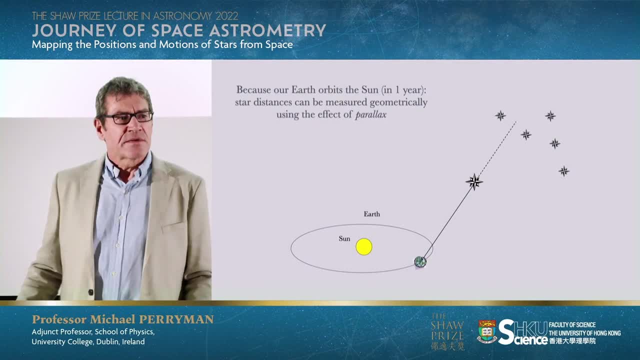 the constellation of Earth's atmosphere is still moving. So, although they're moving, space is so vast that even at the end of our lifetime- our lifetime- the constellation of Earth's atmosphere is still moving. So, although they're moving, space is so vast that even at the end of our lifetime, our lifetime- 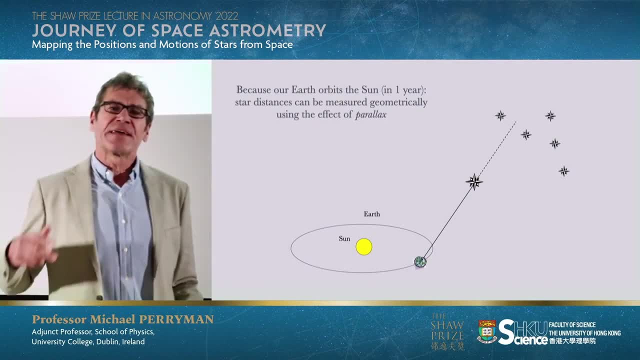 the constellation of Earth's atmosphere is still moving. So, although they're moving, space is so vast that even at the end of our lifetime- our lifetime- the constellation of Earth's atmosphere is still moving. So, although they're moving, space is so vast that even at the end of our lifetime, our lifetime- 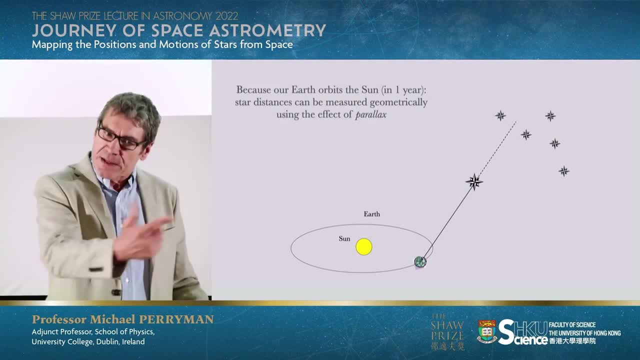 the constellation of Earth's atmosphere is still moving. So, although they're moving, space is so vast that even at the end of our lifetime- our lifetime- the constellation of Earth's atmosphere is still moving. So, although they're moving, space is so vast that even at the end of our lifetime, our lifetime- 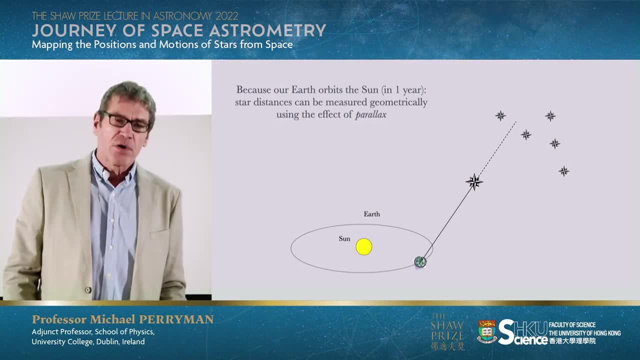 the constellation of Earth's atmosphere is still moving. So, although they're moving, space is so vast that even at the end of our lifetime- our lifetime- the constellation of Earth's atmosphere is still moving. So, although they're moving, space is so vast that even at the end of our lifetime, our lifetime- 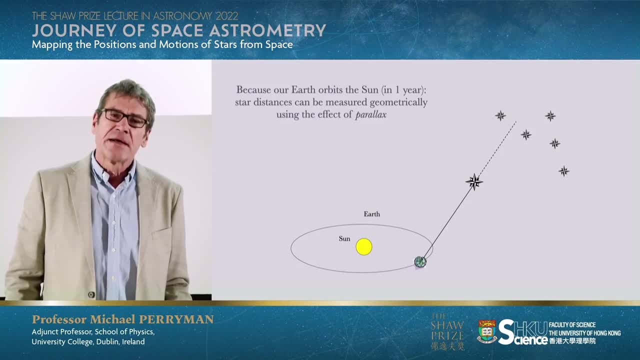 the constellation of Earth's atmosphere is still moving. So, although they're moving, space is so vast that even at the end of our lifetime- our lifetime- the constellation of Earth's atmosphere is still moving. So, although they're moving, space is so vast that even at the end of our lifetime, our lifetime- 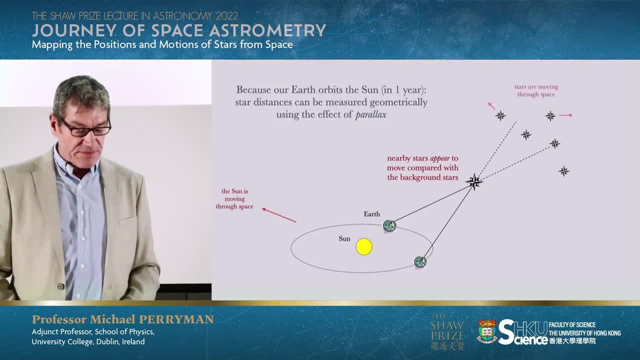 the constellation of Earth's atmosphere is still moving. So, although they're moving, space is so vast that even at the end of our lifetime- our lifetime- the constellation of Earth's atmosphere is still moving. So, although they're moving, space is so vast that even at the end of our lifetime, our lifetime- 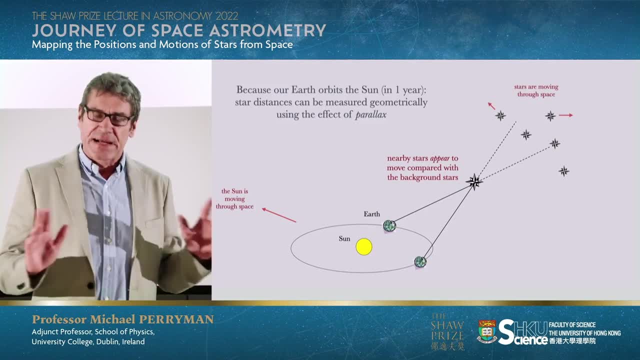 the constellation of Earth's atmosphere is still moving. So, although they're moving, space is so vast that even at the end of our lifetime- our lifetime- the constellation of Earth's atmosphere is still moving. So, although they're moving, space is so vast that even at the end of our lifetime, our lifetime- the constellation of Earth's atmosphere is still moving. So, although they're moving, space is so vast that even at the end of our lifetime- our lifetime- the constellation of Earth's atmosphere is still moving. So, although they're moving, space is so vast that even at the end of our lifetime, our lifetime- 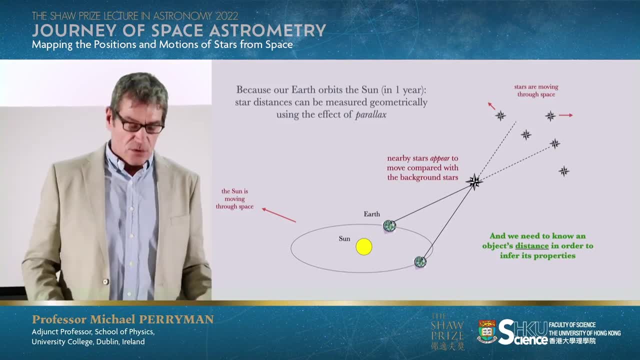 the constellation of Earth's atmosphere is still moving. So, although they're moving, space is so vast that even at the end of our lifetime- our lifetime- the constellation of Earth's atmosphere is still moving. So, although they're moving, space is so vast that even at the end of our lifetime, our lifetime- 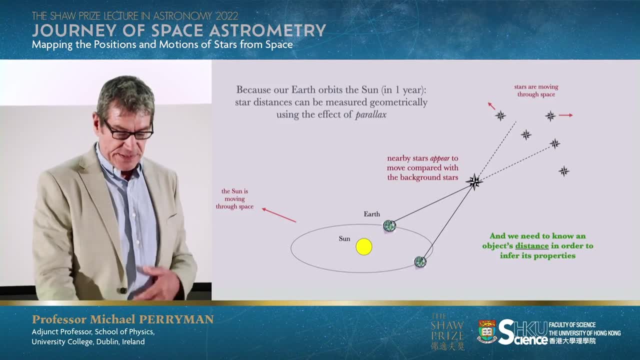 the constellation of Earth's atmosphere is still moving. So, although they're moving, space is so vast that even at the end of our lifetime- our lifetime- the constellation of Earth's atmosphere is still moving. So, although they're moving, space is so vast that even at the end of our lifetime, our lifetime- 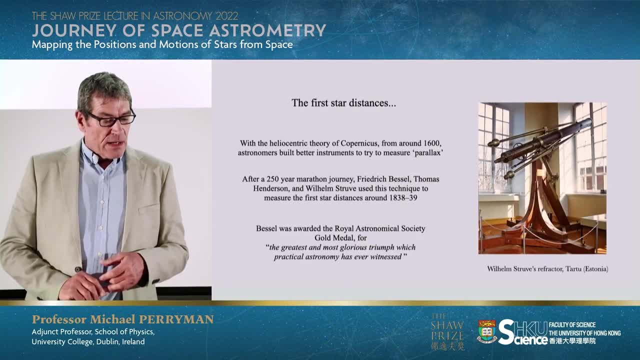 the constellation of Earth's atmosphere is still moving. So, although they're moving, space is so vast that even at the end of our lifetime- our lifetime- the constellation of Earth's atmosphere is still moving. So, although they're moving, space is so vast that even at the end of our lifetime, our lifetime- 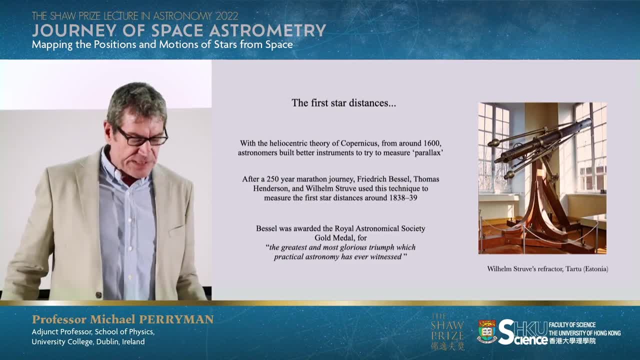 the constellation of Earth's atmosphere is still moving. So, although they're moving, space is so vast that even at the end of our lifetime- our lifetime- the constellation of Earth's atmosphere is still moving. So, although they're moving, space is so vast that even at the end of our lifetime, our timelines 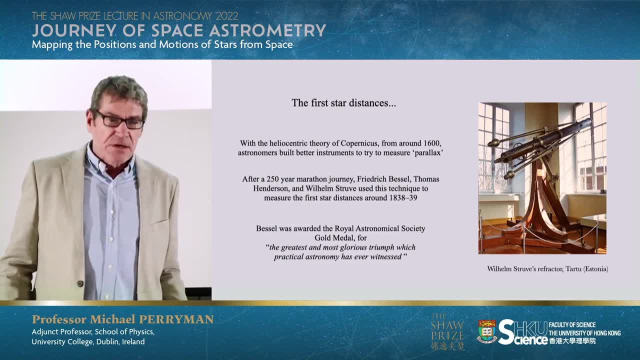 are still moving, But to donner light we should scope at some Ukrainian 37-year old child to an Earth star at an apple tree, And they lived there, no matter what the distance to the stars. And this started a journey of about 250 years, a real marathon journey in. 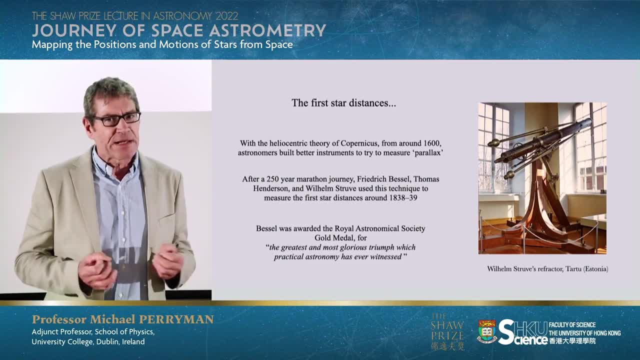 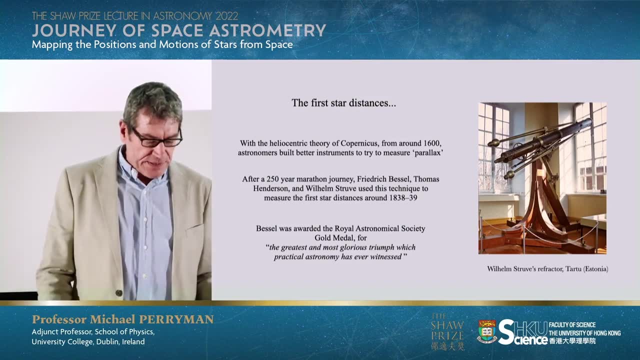 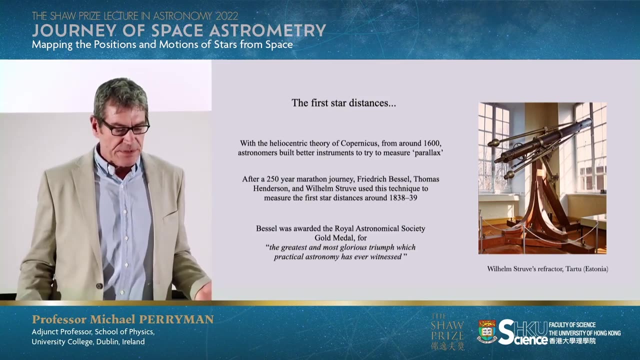 which astronomers built better and better scientific instruments, pushing the angular accuracy of their instruments to better and better levels. And after something like 250 years, around 1830, 1840,, the first distances to the stars were measured using this technique And this is the refractor used by HP Hurricane Neil Humphreys. 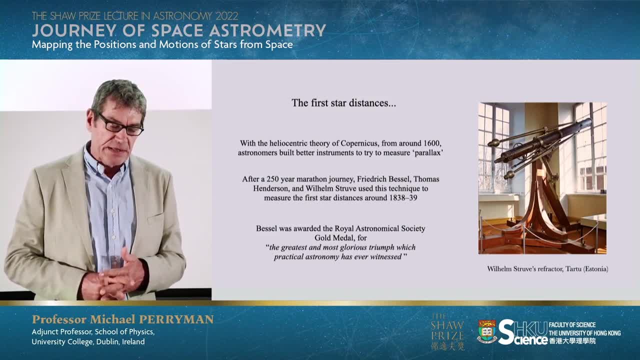 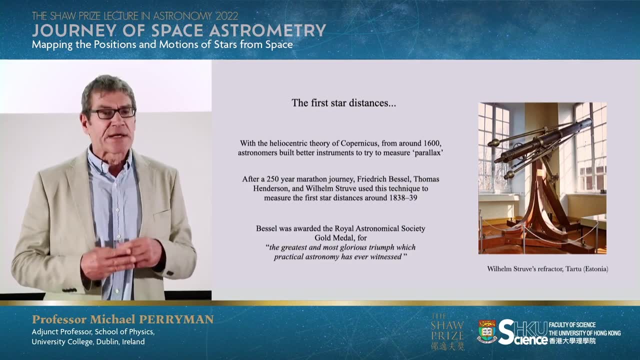 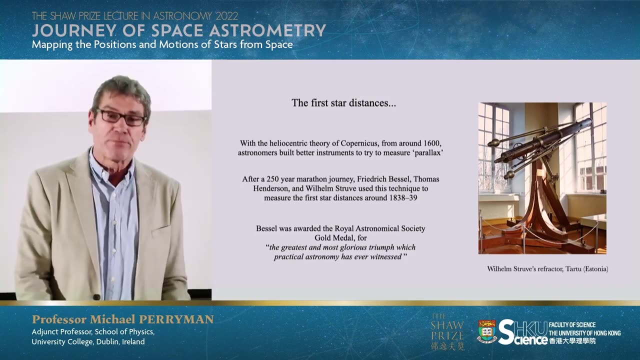 by Wilhelm Struve at his observatory in Estonia. the determination of the first star distances was recognized as a major achievement in astronomy, and Bessel was awarded the Royal Astronomical Society's gold medal for this most glorious triumph, as the president of the society reported. 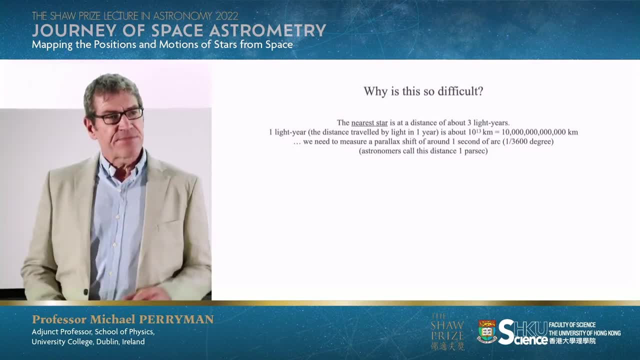 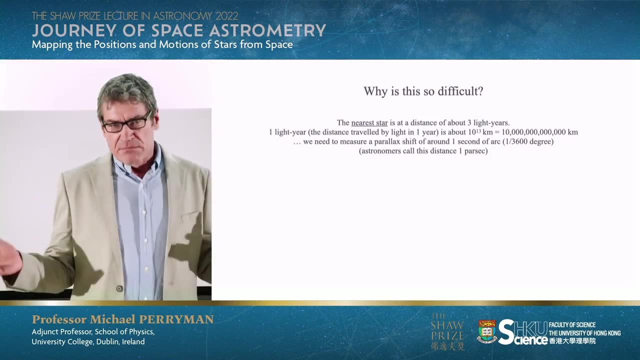 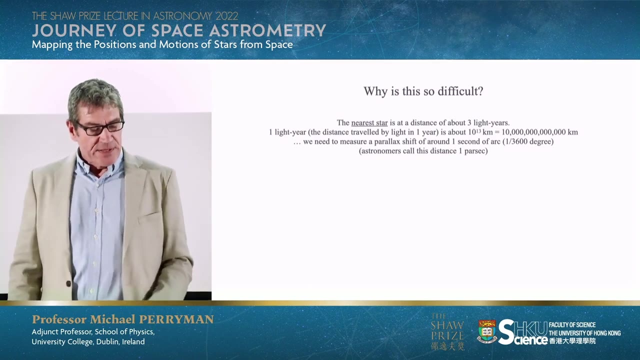 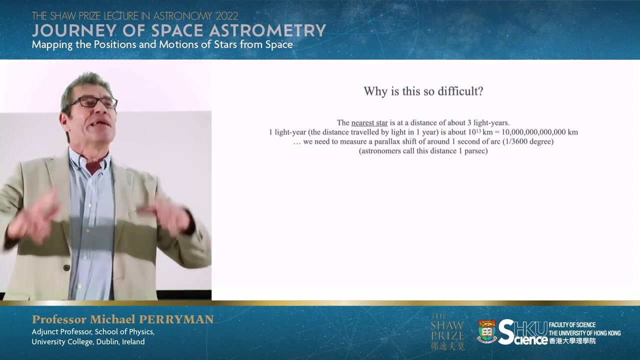 at the time. Now, why is this so difficult? It's difficult because even the nearest star lies at colossal distances. Most of you will have heard of a light year. A light year is the distance that light travels. in one year It's about 10 to the power of 13 kilometers, 10 million kilometers. 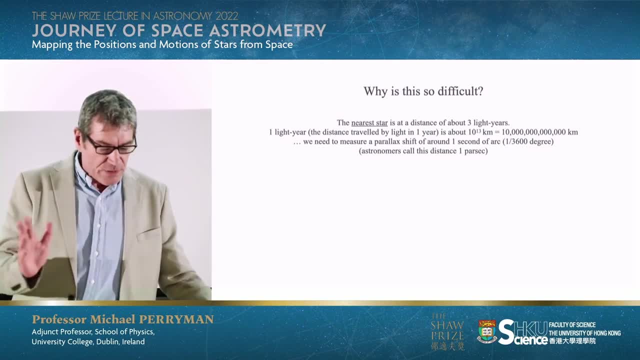 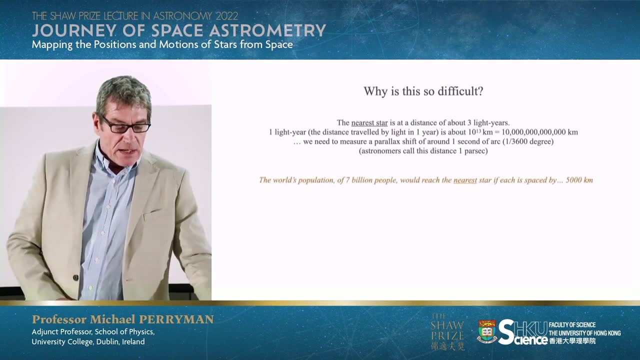 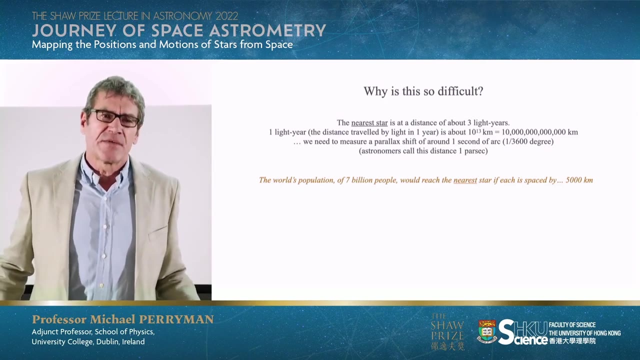 And we need to measure that angle, one arc second or thereabouts, in order to be able to measure The distance to the nearest stars. I've tried to come up with my own analogy of how can we comprehend the distance, say, to the nearest stars. 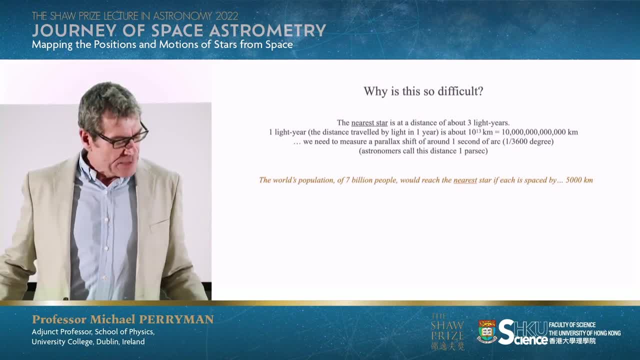 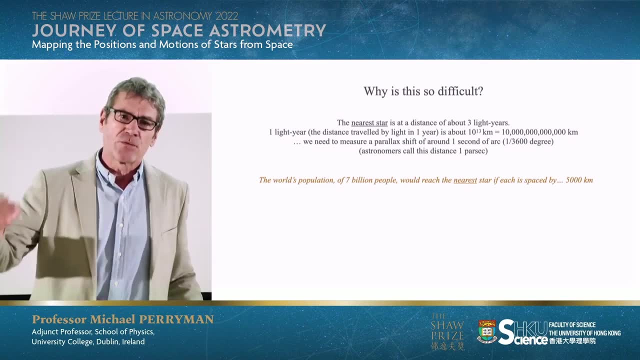 And I don't think it's easy for humans to appreciate that. but here is an analogy: If we took the world's population of 7 billion people and we spaced them out at regular intervals, how far would we need to space them to get to the nearest star? 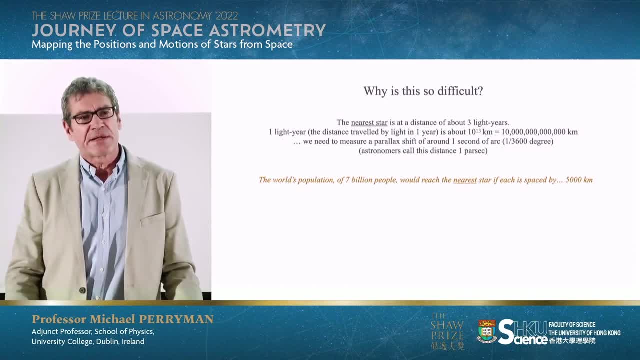 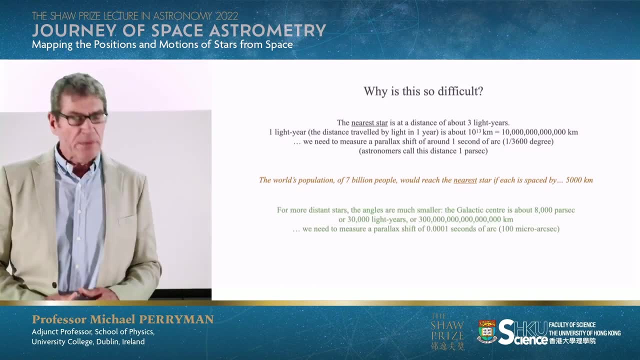 And the answer is about 5,000 kilometers. So 7 billion people each spaced at 5,000 kilometers would get us to the nearest star. And the problem becomes much more serious if we want to measure distances to the more distant stars. 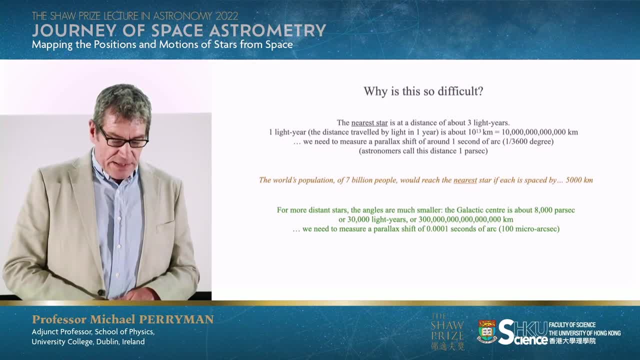 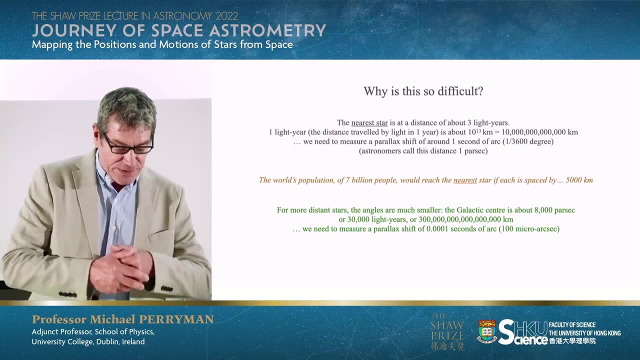 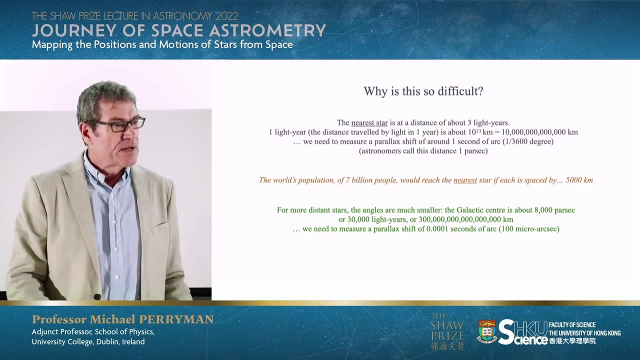 For example, the center of our own galaxy is a distance of about 30,000 light years, So 300,000 billion kilometers, And we'd need to measure angles Getting down to levels of a millionth or a few millionths of a second of arc in order. 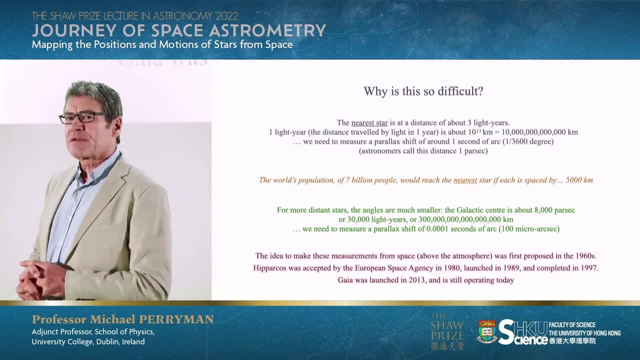 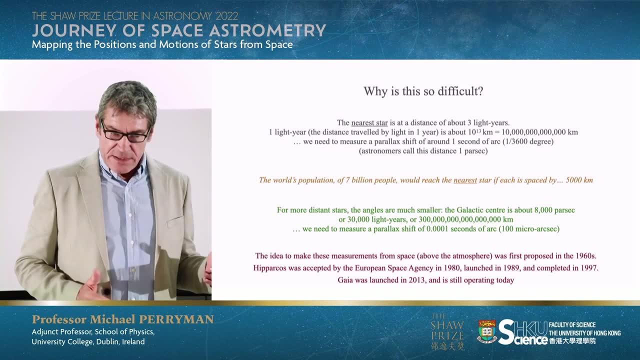 to be able to do that Now. the idea to make these measurements from space came about in the mid-1960s. The idea was to get above the atmosphere so that we can reduce the perturbations that the atmosphere brings to these measurements. 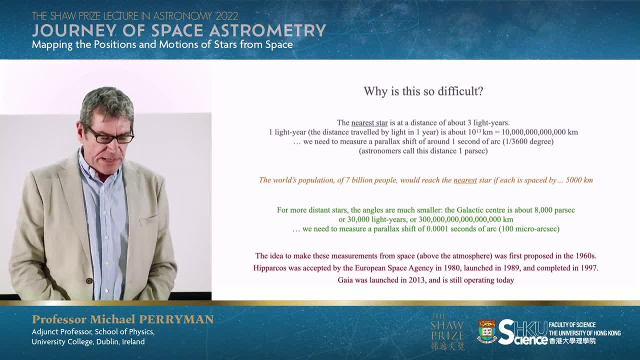 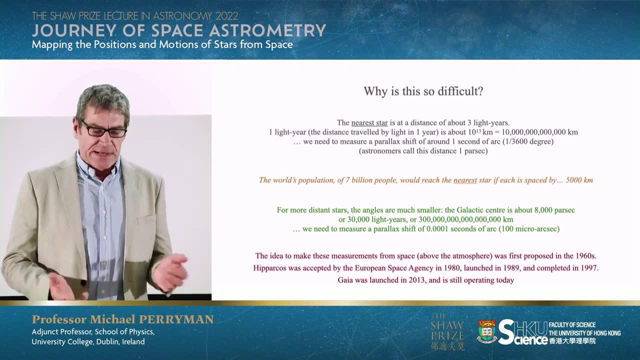 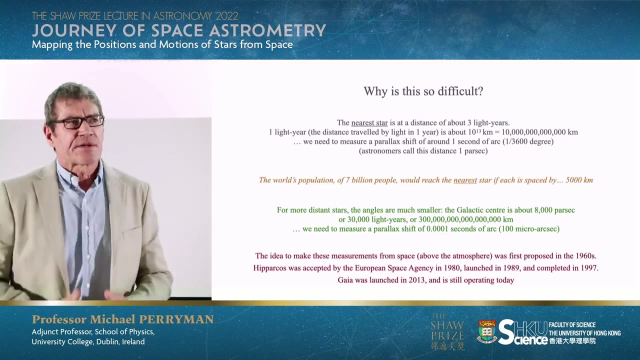 And Hipparcos was really a trailblazing experiment adopted by the European Space Agency in 1980. It was launched in 1989.. The mission completed its activities in 1997.. And it enabled the measurement of the distances to something like 100,000 stars. 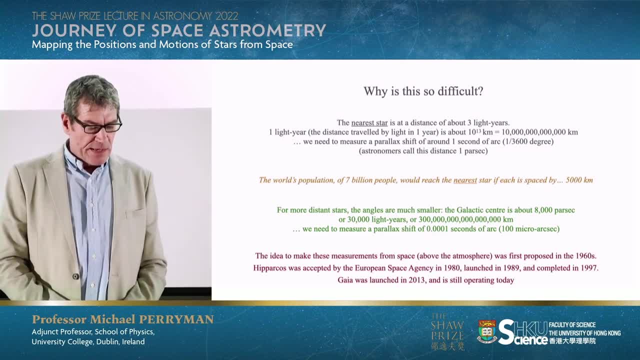 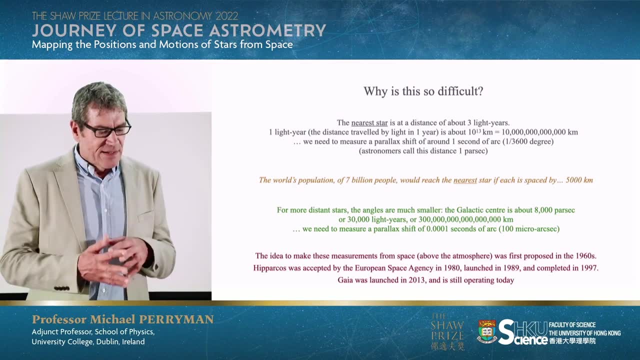 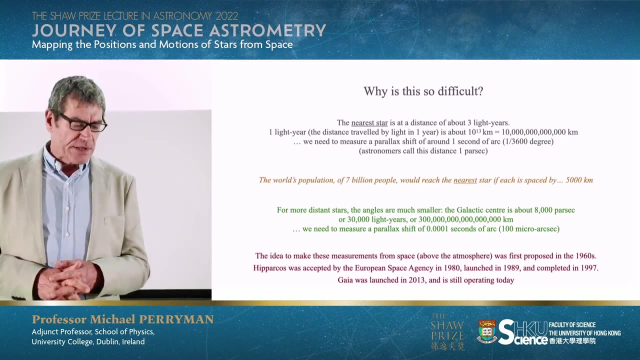 So that's just over 20 years ago. Hipparcos was so successful, so illuminating, that a second mission was accepted by the European Space Agency very quickly afterwards- Gaia. Gaia was launched in 2013.. And it's still operating today. 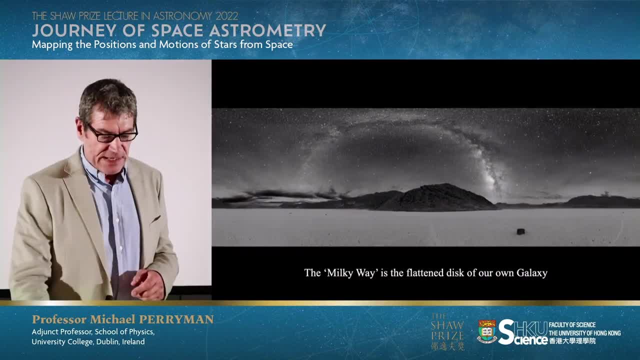 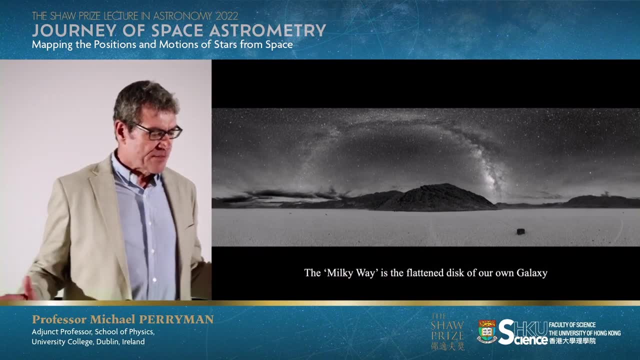 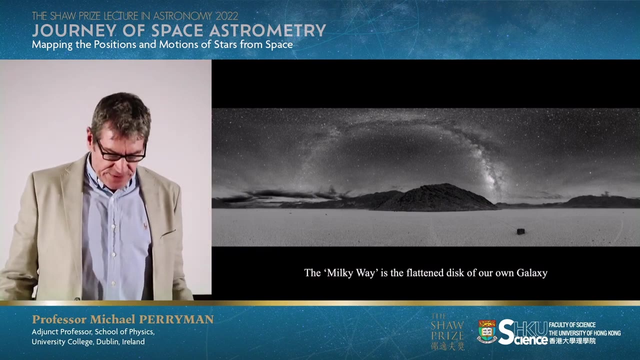 And it's taking these measurements to much, much greater levels and much, much greater distances. So from a dark sky location, you can look up into the sky and you see this band, the Milky Way. And the Milky Way we now know is the flattened disk of our own galaxy. So if we could step outside of our galaxy, it would look something like this: This is the Andromeda Galaxy, Galaxy M31. It's part of our local group of galaxies And we think our own galaxy looks something like this. We would be sitting, the sun and the planets around it would be sitting somewhere out. 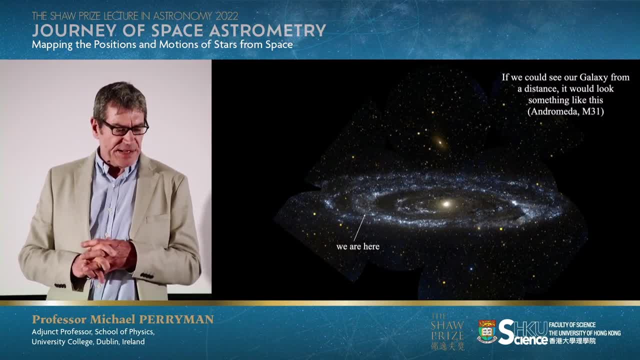 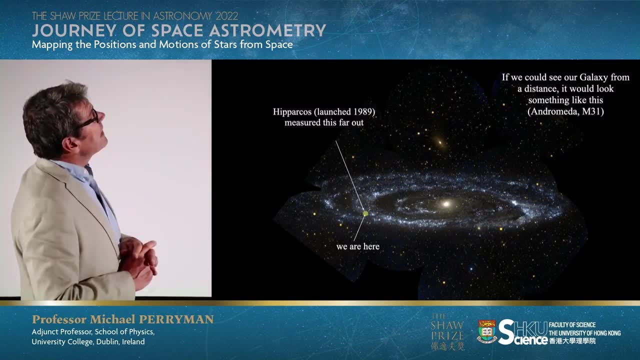 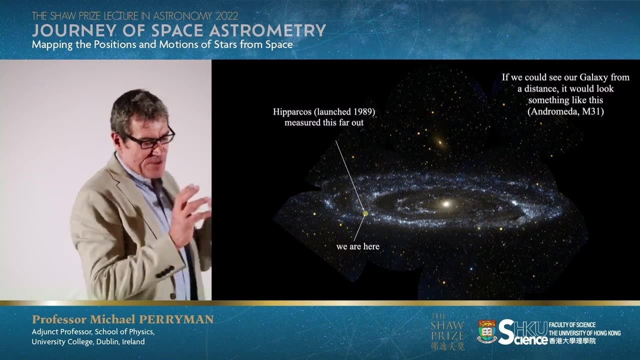 here, 30,000 light years from the center, And this circle shows very roughly the sphere that we're able to access with Hipparcos. This small red circle, This small red circle, This region around our sun, is the region out to which we could measure accurate distances. 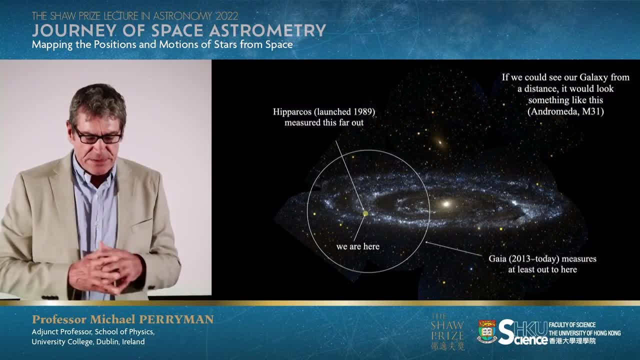 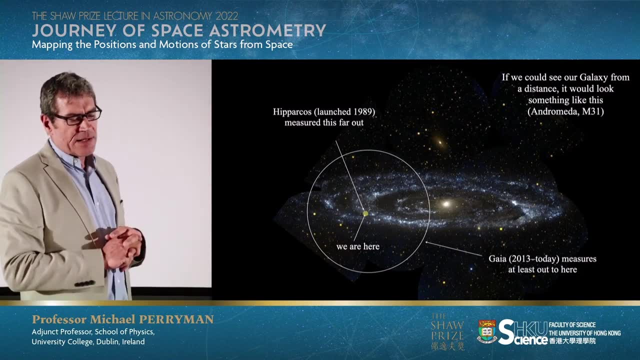 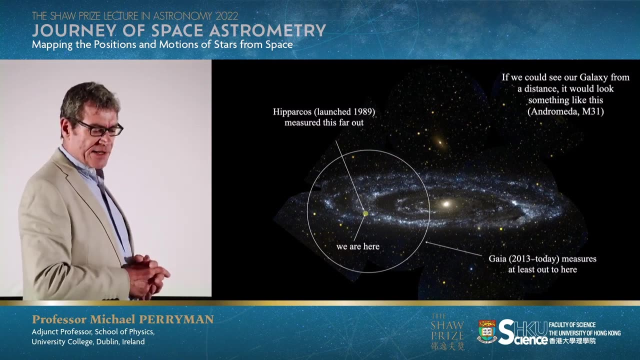 and star motions. What Gaia has been able to do- by improving enormously the accuracy that we can measure from space- is to expand our distance horizons out to much greater distances, Out to distances something like the center of our own galaxy, And this means that we can measure the distances. 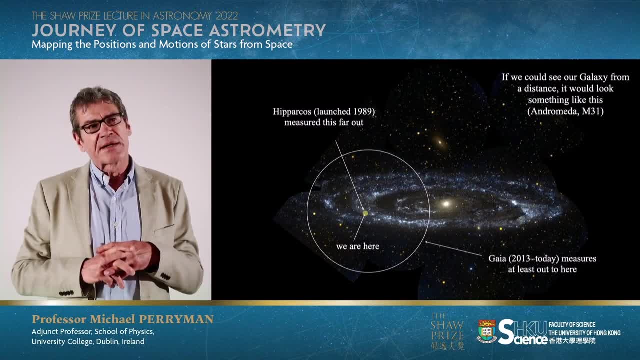 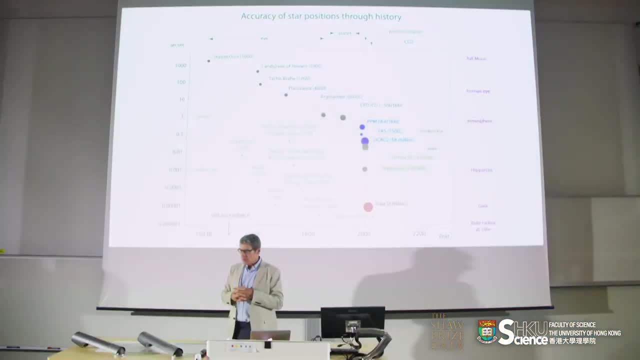 The full stereoscopic distribution- OK- stars in our galaxy and also how they're moving through space. Now, just to put this in a little bit of a historical context: there's a lot of information on here, but I show here the accuracy of measurements over time and this is going. 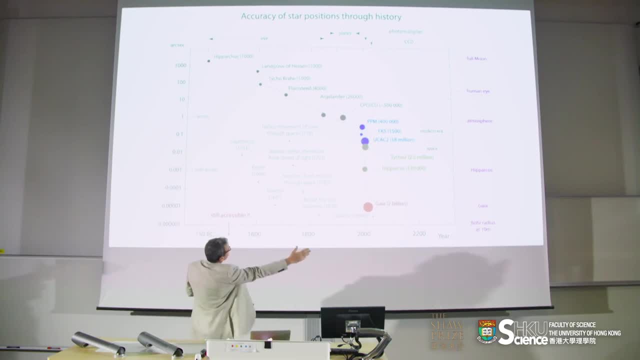 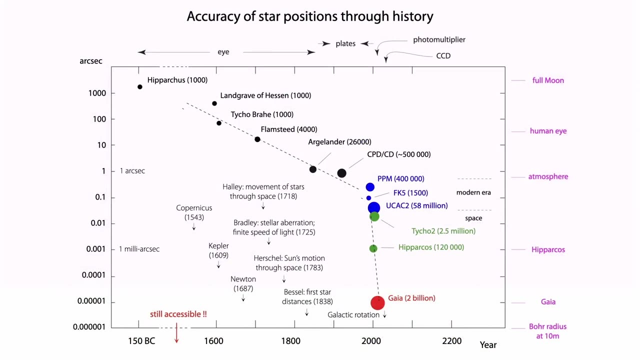 back to say 1500,, 1600, 1800 and the year 2000, and there's a logarithmic scale on the left and it shows how the accuracies have improved over time. You see this dashed line going down and about 20 years ago, with the advent of space, 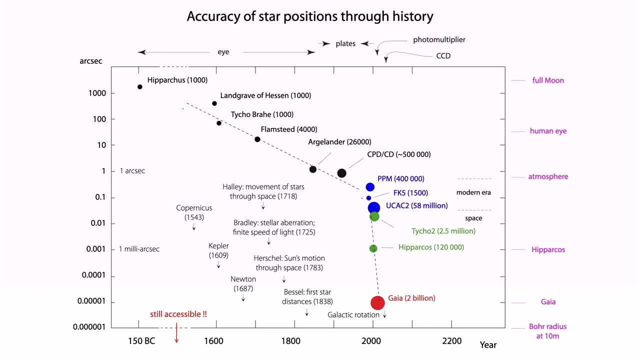 techniques. you can see Hipparcos suddenly moves the accuracies well down, and Gaia even much further still. And if we go back through history, we can see that each of these improvements in accuracies has led to considerable insights into the nature of our galaxy and the universe surrounding us. 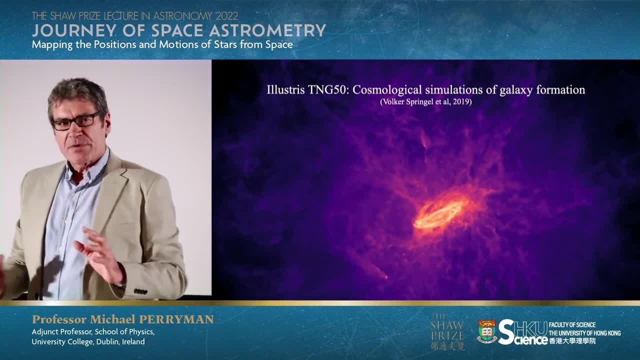 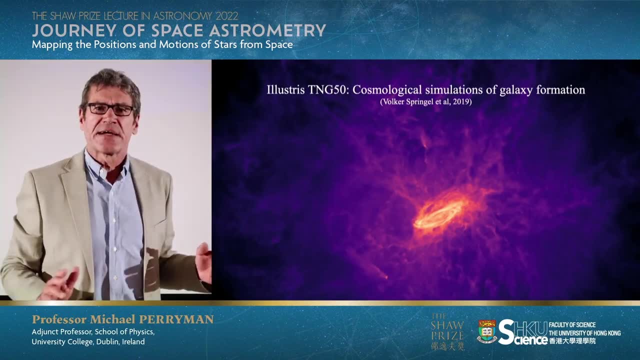 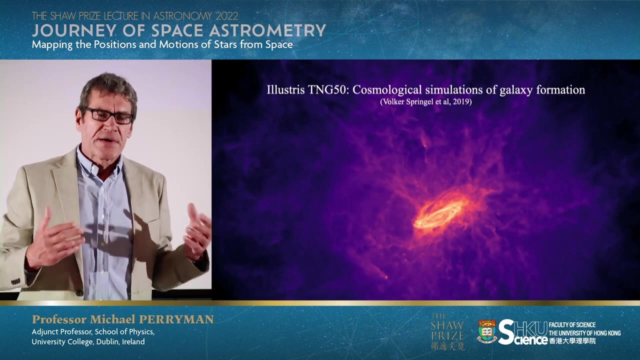 I'm just going to come at the problem from a slightly different direction momentarily. This is nothing to do with Gaia, but it shows the state-of-the-art understanding of how our universe formed and how the galaxies within our universe formed, and it's from very extensive cosmological simulations that use all 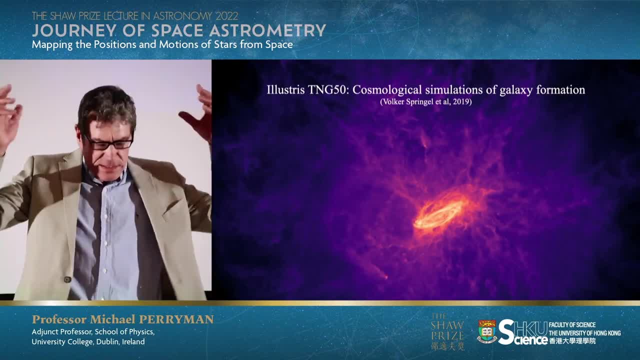 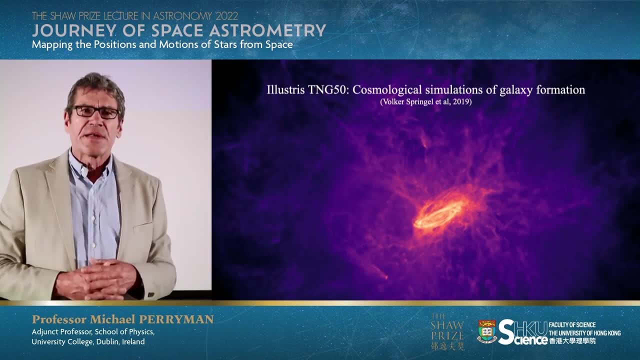 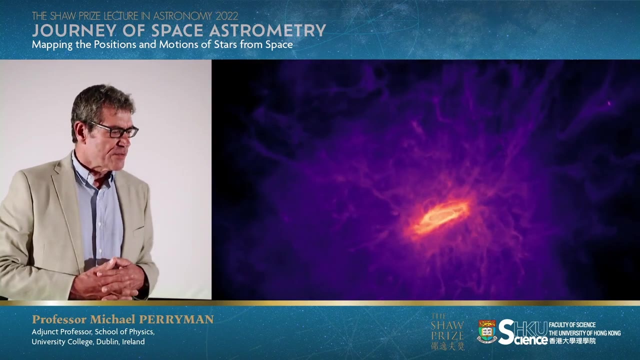 the ingredients that we understand today apply to our galaxy, our universe, The Big Bang, visible matter, dark matter, dark energy and so on, And these models are so detailed and so comprehensive that, setting this in motion, you can see over billions of years. you can see. 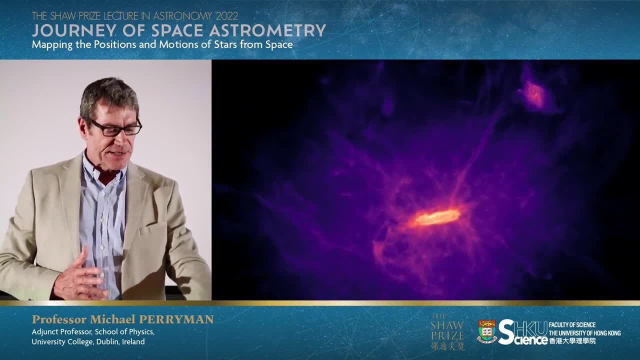 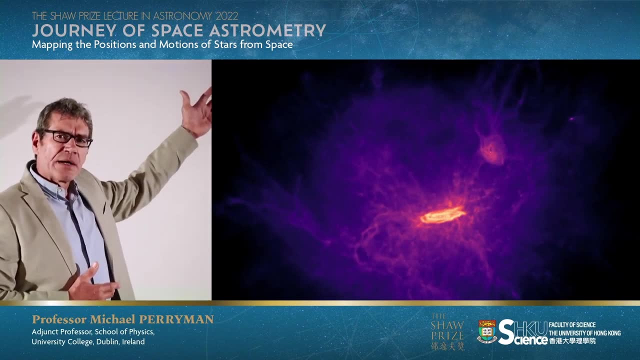 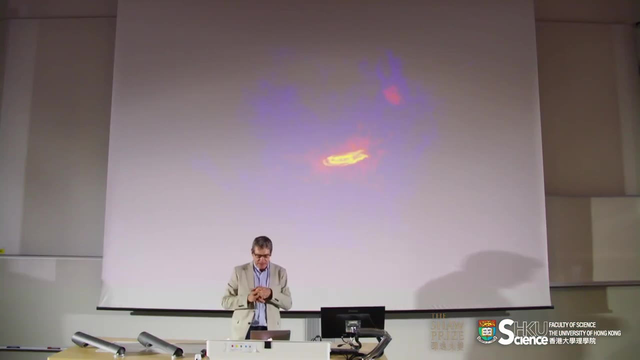 structure forming in there which looks a little bit like our own galaxy, and satellite galaxies which are moving into the frame of the picture, which look very much like the Large Magellanic Cloud, one of our neighbouring galaxies. The importance of this little animation is that it shows you that, in any understanding of how our own galaxy 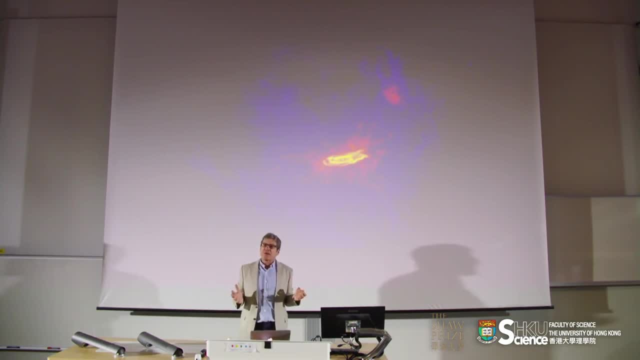 formed. there's going to be an enormous amount of structure in there, concentrations of stars and complex motions of stars, and what Gaia is all about is really measuring huge numbers of stars and trying to put together a more complete picture of how our own galaxy formed. now I'm going to just drop. 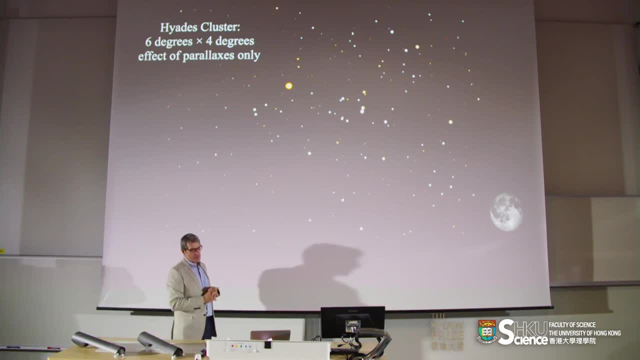 back and show a little, three little animations coming from the work on Hipparcos, so 20 years ago, and these, I think, still show quite effectively what it is we're trying to measure. this is a region of the sky about six degrees by four degrees. so in this the, the moon would occupy a region of sky, something. 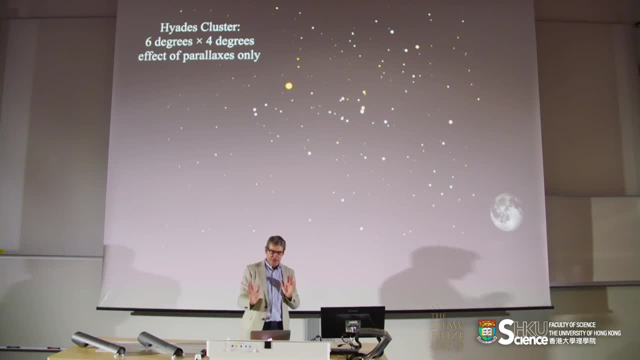 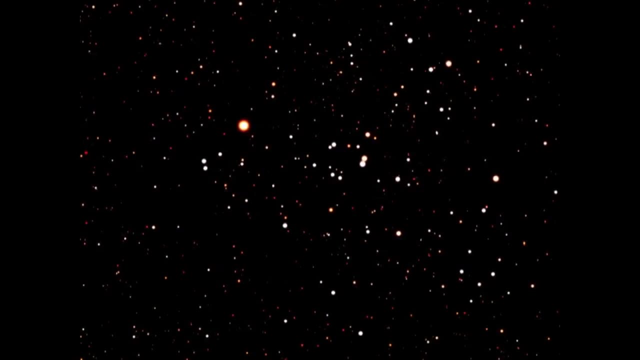 like that, and what I've done in this animation is just to swing backwards and forwards around those stars to show you the effect of the distances. it's very difficult to communicate the idea of distances in a two dimensional presentation, but by making this animation that swings backwards and 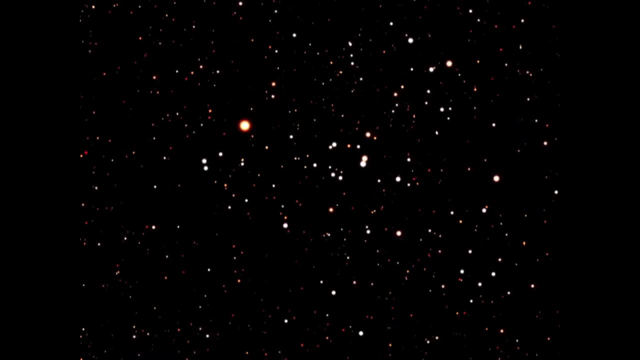 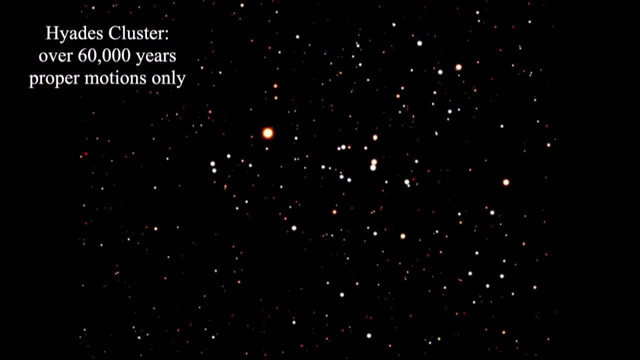 forwards the stars that are moving most of the stars nearest to us and the stars that are moving least to the background stars, and that is illustrating the effect of parallax that I talked about earlier on. now, at the same time, it turns out that we can measure how the stars are moving through space, and this shows: 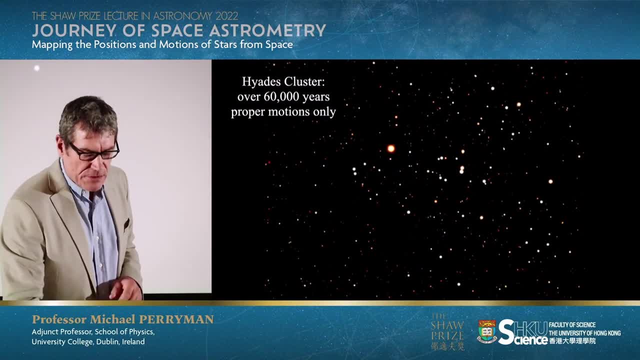 the same region-itime 구 Genesis Layer on the top. I just can't understand what the sky is here from. dash juxtaposition between reality程 is in 그렇죠 of sky. it's the Hyades cluster and it shows how the stars would be moving over 60,000 years. 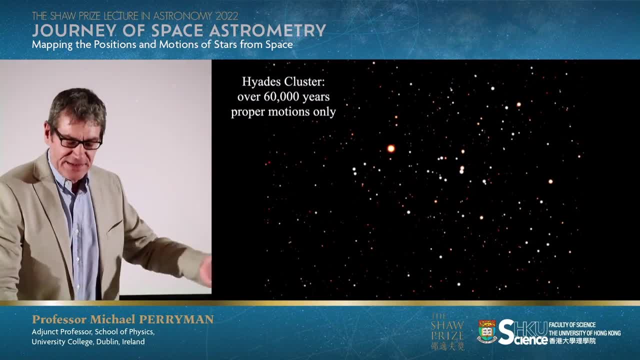 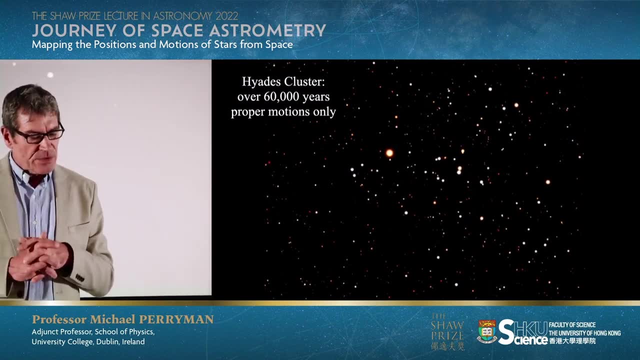 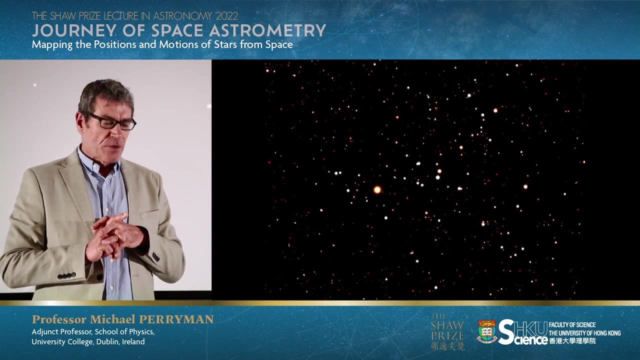 on the basis of the measurements that we've made from this satellite over just three or four years, We can measure them so accurately that we can propagate their motions forward, And you can see there that over the 60,000 years, stars are not moving the same way at all through space. Some of 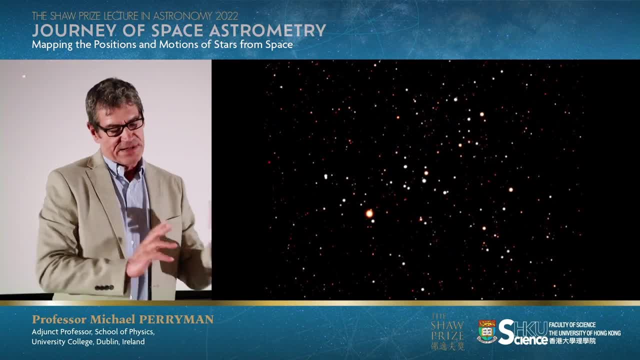 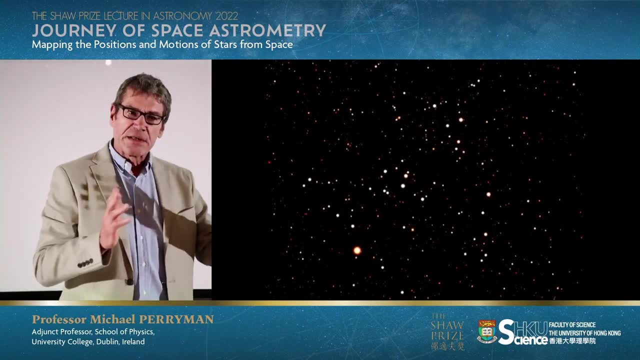 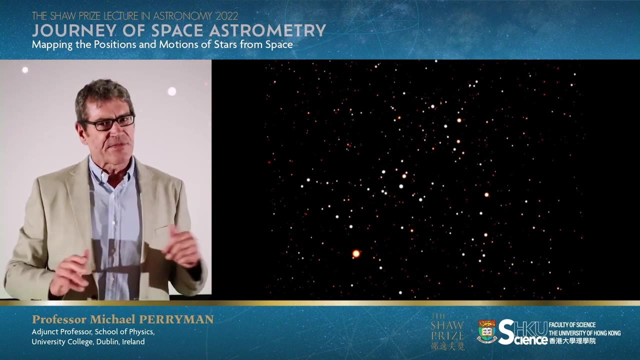 them are. most of them are moving right to left. As we look at this, this is the bright star, Aldebaran, and it's moving from top to bottom, but other stars are in the background and moving in very different ways. So, again, this is trying to explain that, if we can measure simultaneously the distance, 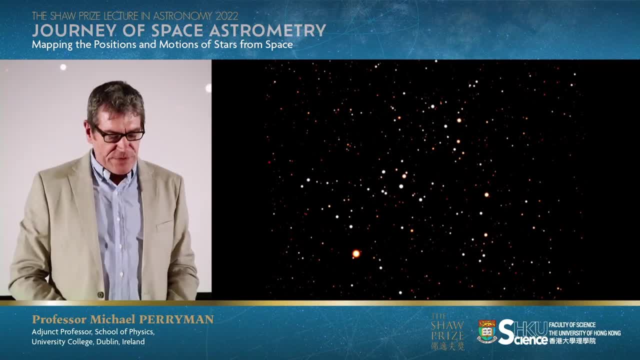 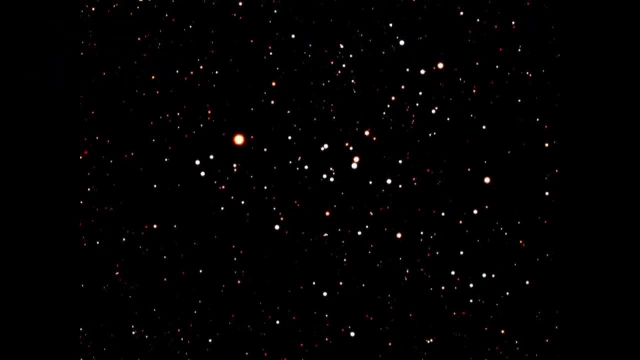 to the stars and also the way the stars are moving through space. we can infer a lot about the structure of our galaxy And we can put those two effects together, combine the parallax motion and the parallax motion, and we can infer a lot about the structure of our galaxy And we can put those. 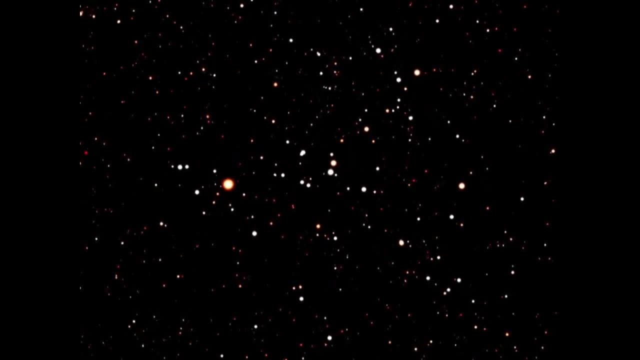 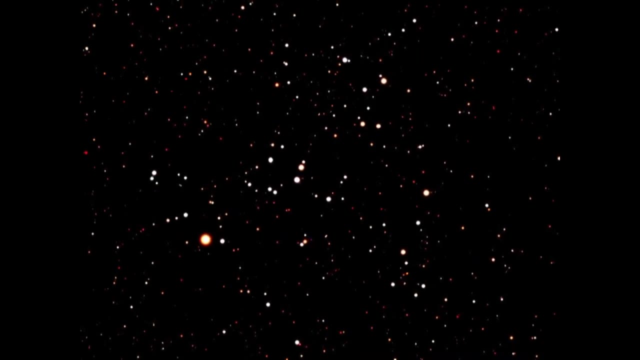 two effects together. combine the parallax motion and the parallax motion and we can infer a lot about the proper motion. And you can see that these stars are moving in apparently very complex ways and they're encoding the information about their distance and their motion through space. I will just 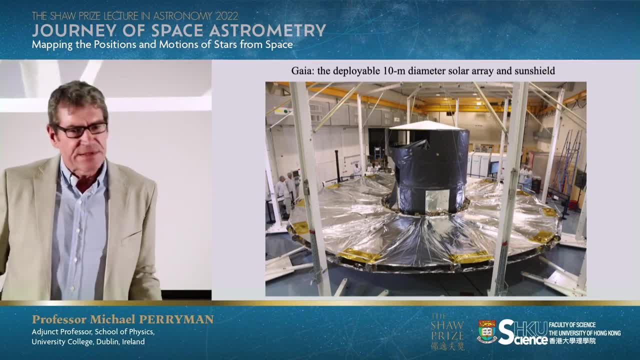 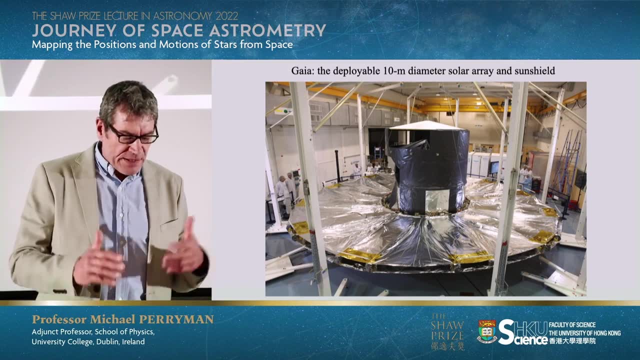 show. it's not my goal today to tell you in detail how this is done or to tell you in detail about the Gaia satellite, but I think it's a nice opportunity to just show you a couple of pictures. Here is Gaia in the test facilities assembly for the Gaia satellite, And I'm going to show you a couple of. 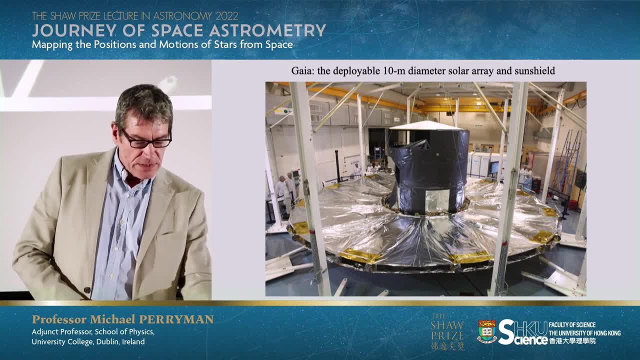 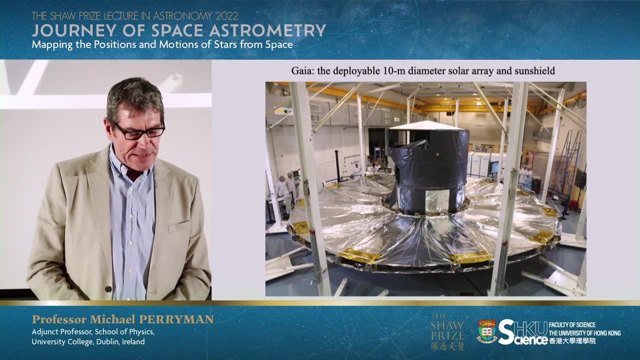 itten the test facilities assembly for the Gaia satellite And I'm going to show you a couple of facility. There are people around the side of it. It's a sun shield which is very much like the sun shield that you've seen with the James Webb Space Telescope. It was deployable And it shields. 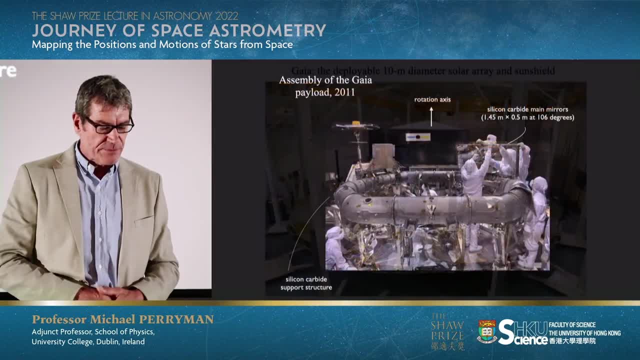 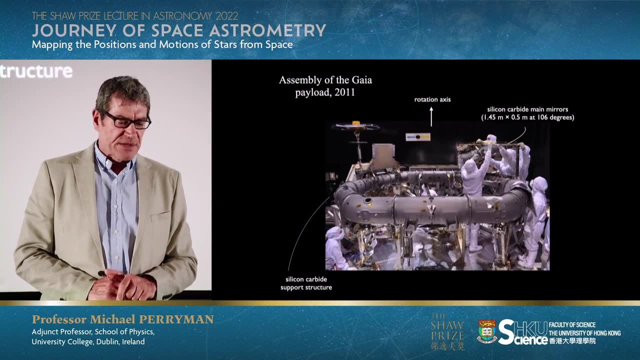 this very delicate payload assembly from the intense radiation from the Sun. The telescope is a huge and very, very accurate system. It's built around a very stable. The telescope is a huge and very, very accurate system. It's built around a very stable. The telescope is a huge and very, very accurate system. It's built around a very stable. 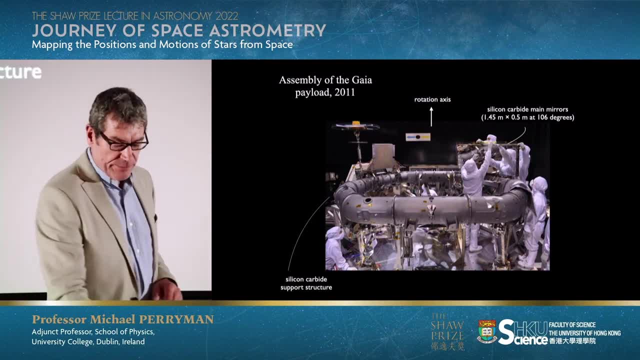 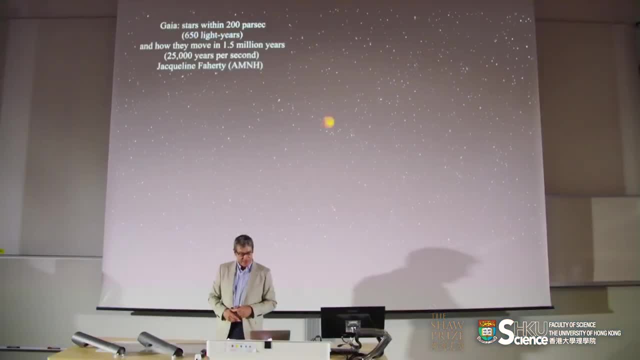 Taurus structure and you can see one of the two main mirrors there being assembled back in 2011,- shortly before launch. That's all I'm going to say on the Gaia satellite itself. Where are we with the results from Gaia? Well, what we can start to do now is to put together 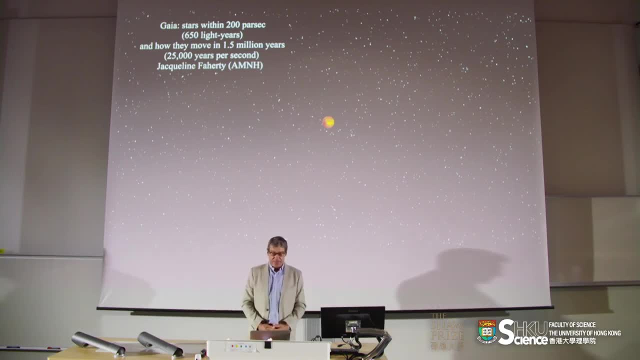 a little animation, and this is one created by Jacqueline Flaherty at the American Museum of Natural History, And what she's done is to take the stars within 200 parsecs. it's about 500, 600 light years, so it's still very close to us in absolute terms, and she's just made this. 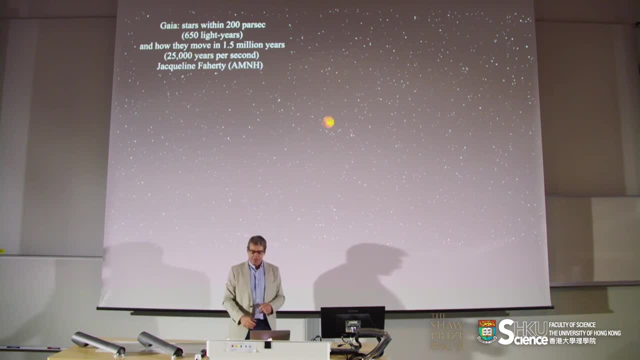 little animation which shows how the stars move over a period of one and a half million years. Again, we can't possibly measure them over one and a half million years, but we can measure them sufficiently accurately that we can predict how they will move through space over one and a half. 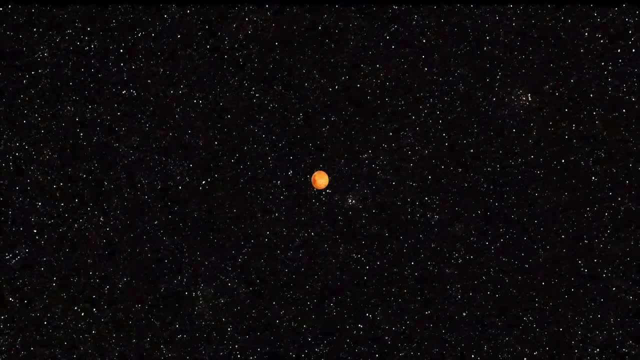 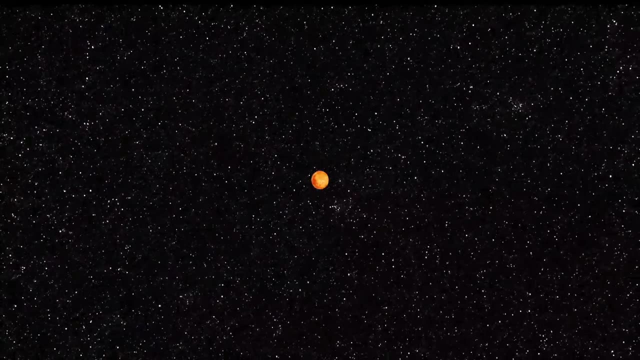 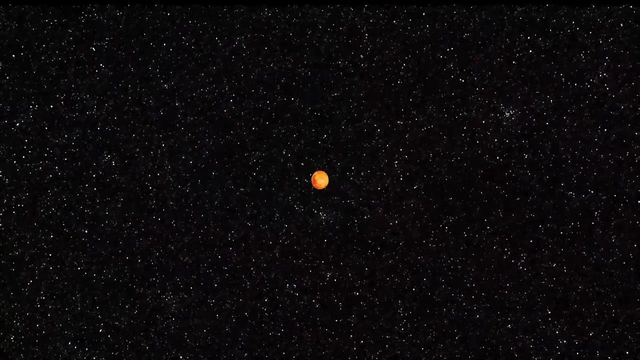 million years And if we watch that little animation unfolding, you'll see all sorts of complex structures. We've got clusters of stars, open clusters moving in different ways, stars moving in very complex ways, and you can see from time to time stars shooting through the animation at very 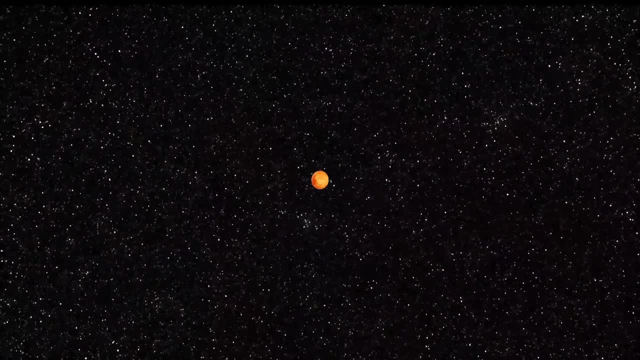 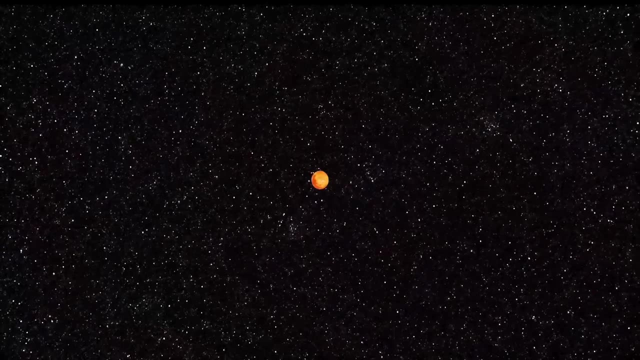 high speed. These are stars which are in the halo of our galaxy and just passing through, very close to us and very rapidly. So this is just a little, one little snapshot of the Gaia results, but it gives you a clue as to how we are. 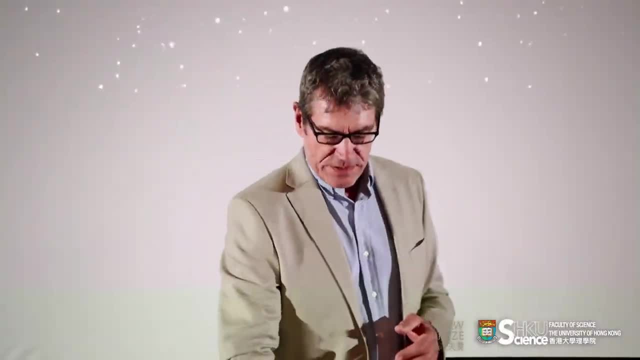 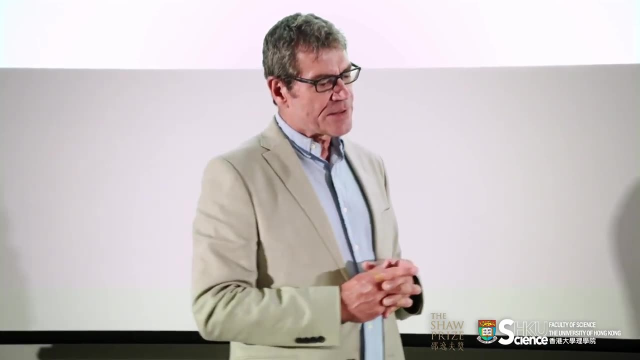 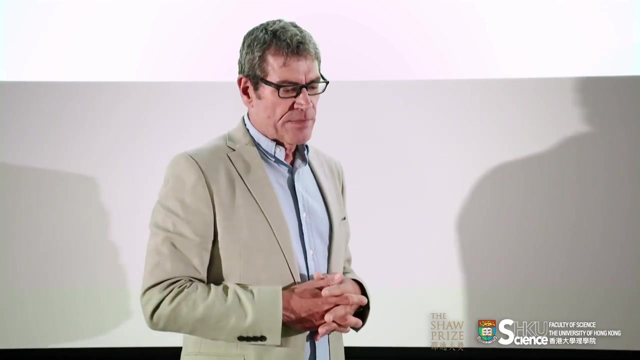 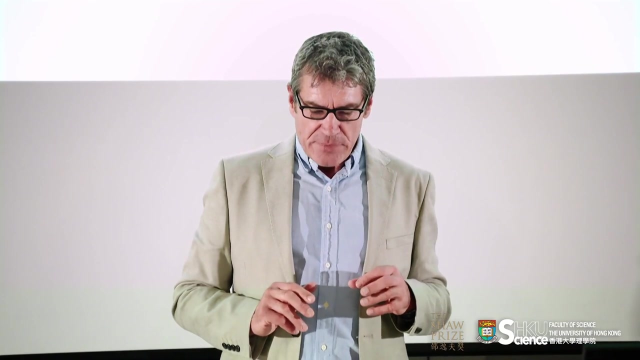 piecing together these stellar motions in our region of the galaxy. Now, what I'm going to do in the remainder of my talk is just to pick out five or six of some of the things that are emerging from from these investigations. Now you may imagine that, with two billion stars being measured by Gaia, Gaia is really 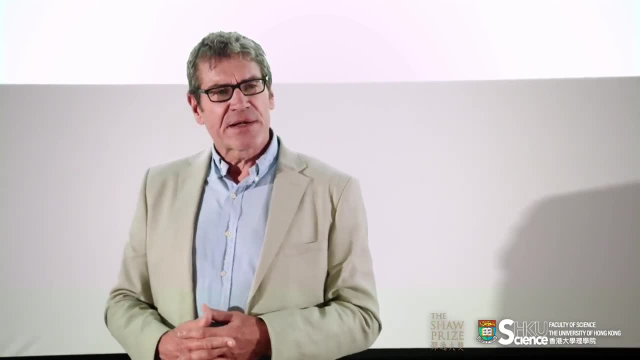 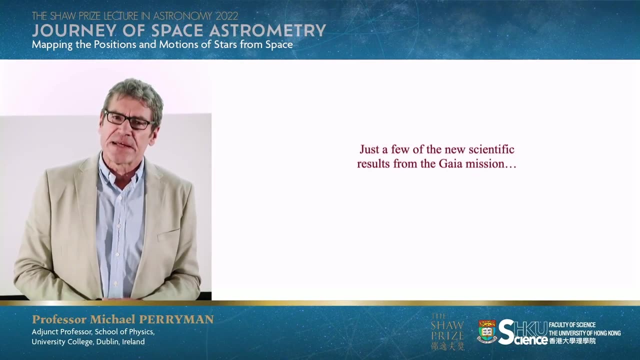 impacting almost all areas of Astronomy. So let's look at some of the things that are emerging from these investigations. So it's pretty much impossible to give you a detailed insight into what's coming on, But I hope I can give you a little bit of a flavor of what we are discovering. 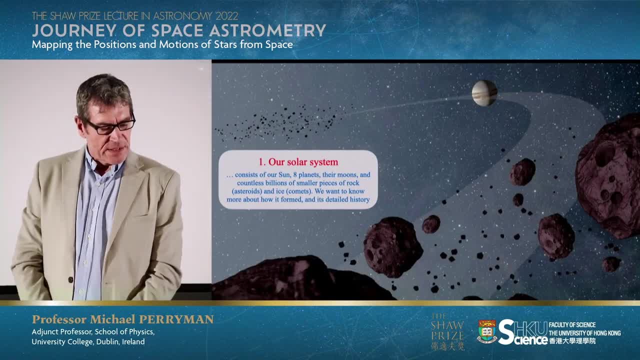 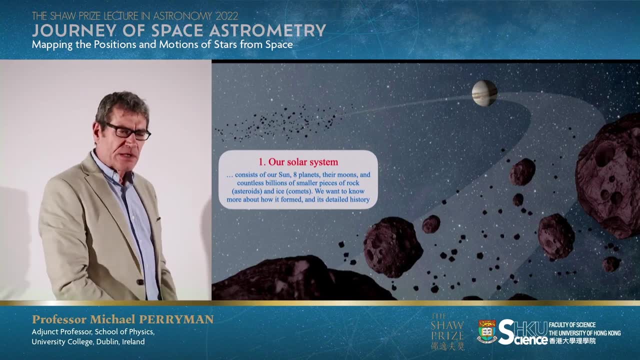 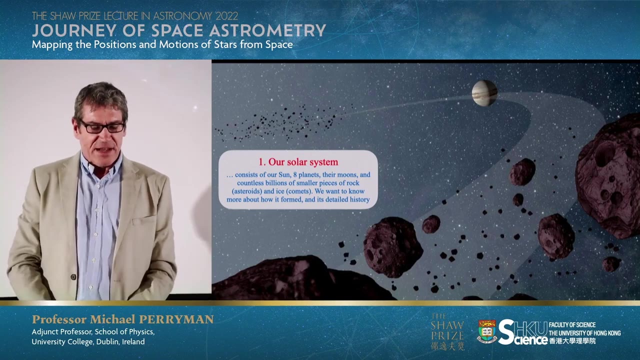 So I'm going to start from the nearby and move outwards, go through each of these quite quickly. The first is the solar system. It turns out that Gaia is not only measuring stars in our galaxy, but we're also measuring asteroids and other bodies in the solar system. 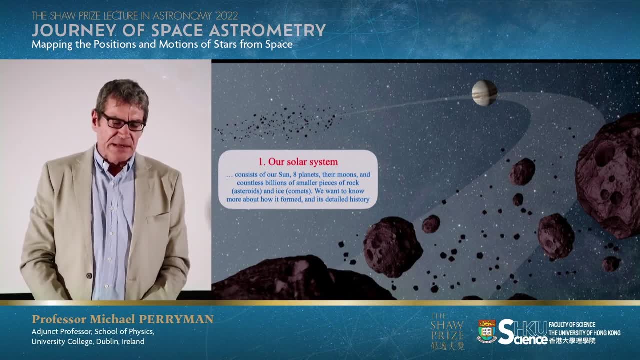 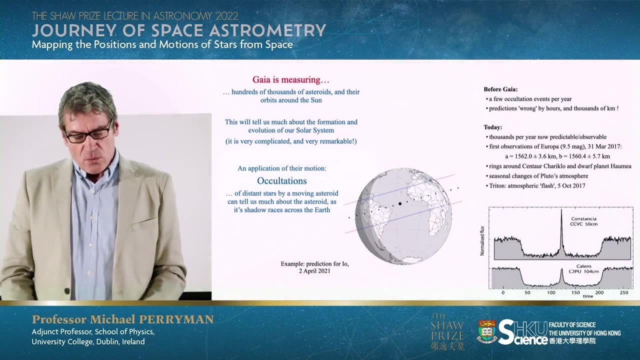 And Gaia will eventually, in the final catalog, contain several hundred thousand of these rocky bodies in our solar system. What are we using this for? We're using this to try and understand the history of the formation and the evolution of our own solar system. 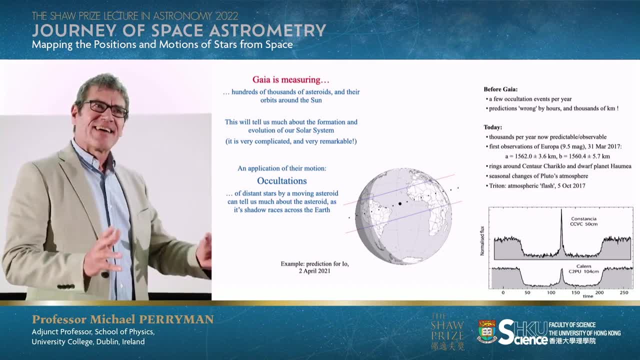 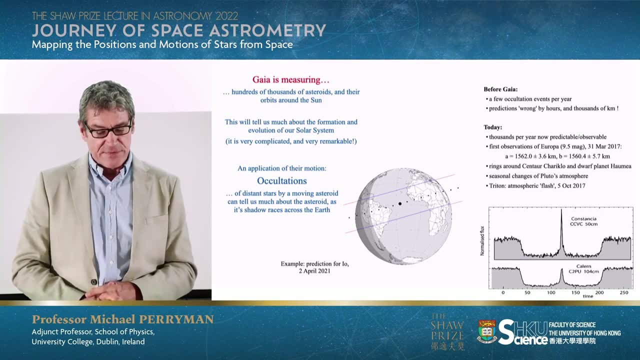 And one of the very beautiful, clever techniques that's actually being used as well by amateurs who are assisting the Gaia scientists with this is the occultations of stars, And it's very interesting to see how these stars, as the asteroid bodies, move across them. 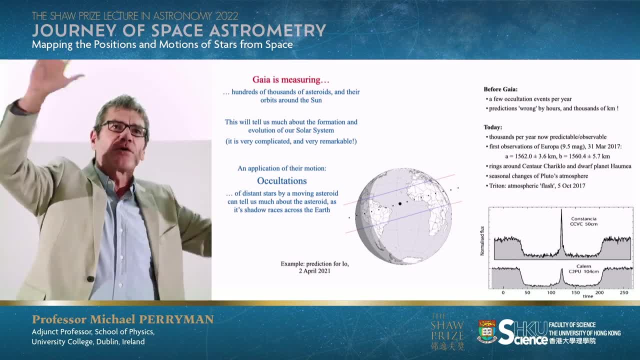 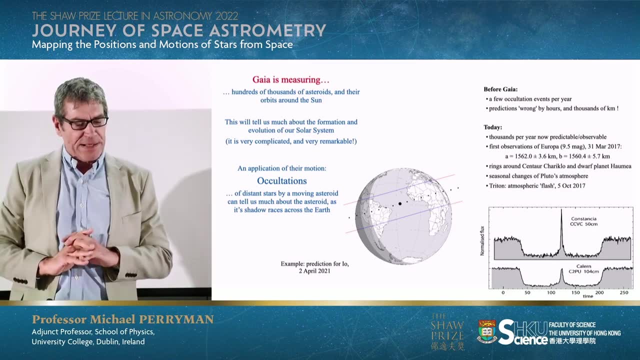 Now I ask you to imagine hundreds of thousands of rocky bodies moving in front of billions, millions or billions of stars that are also moving slowly through space, And you may imagine that from time to time, one of these rocky bodies passes in front of the star. 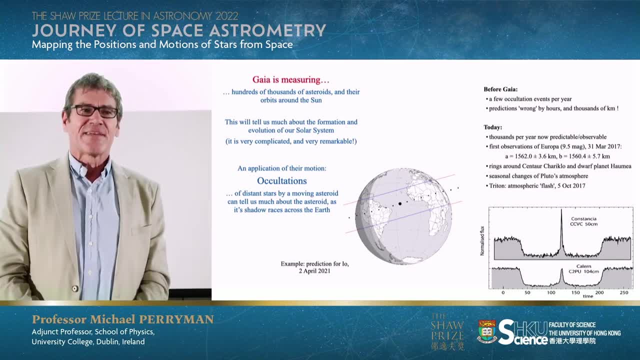 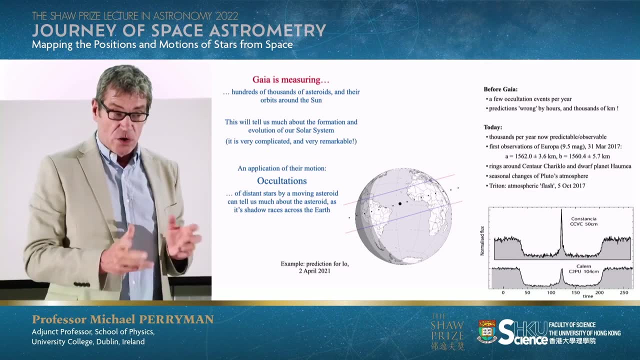 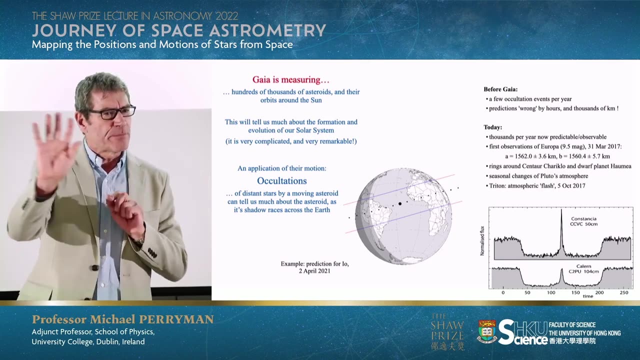 A star And when it does that, the light is diminished coming from the star, And if we predict where these occultations are going to happen on Earth. astronomers can watch this, look out for them and measure the attenuation in light as the rocky body passes across the face of this star. 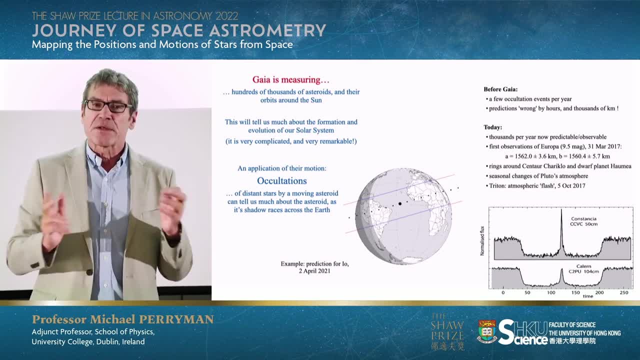 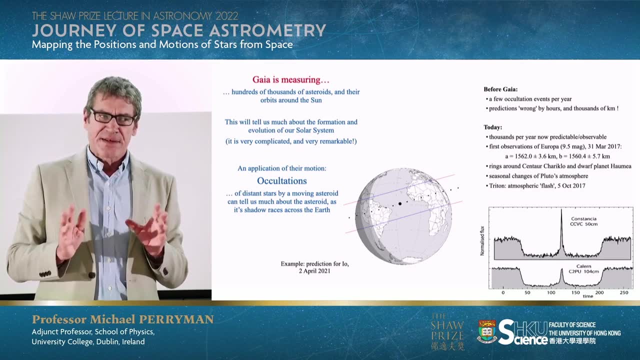 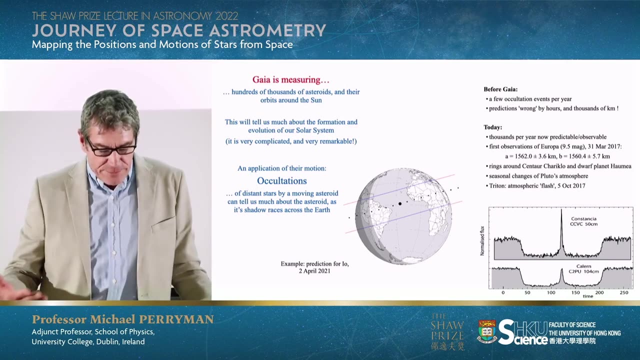 And now we're in a position to predict thousands of these each year, to get the occultation time accurate to a few seconds and to start saying an awful lot about the sizes of these rocky asteroidal bodies, or even if the body has an atmosphere. 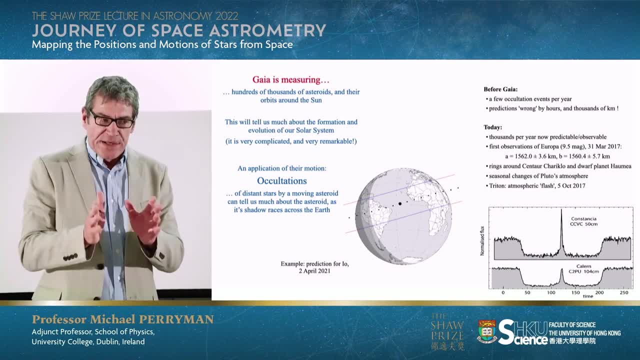 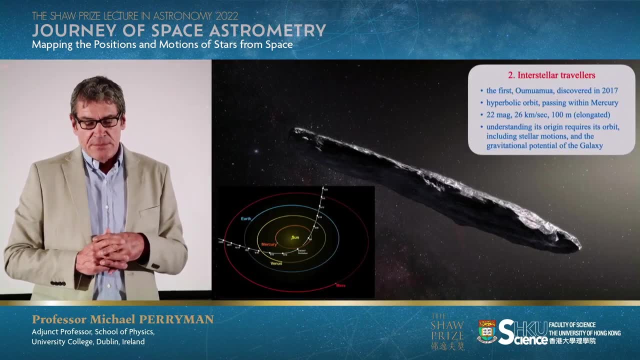 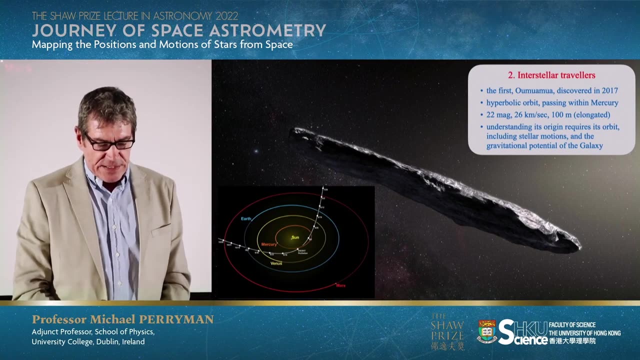 for example, Pluto. we can see the effects of the atmosphere as the asteroid passes across the star. My next example is something which emerged into great excitement five years ago: the discovery of the first interstellar traveller, or interstellar vagabond. 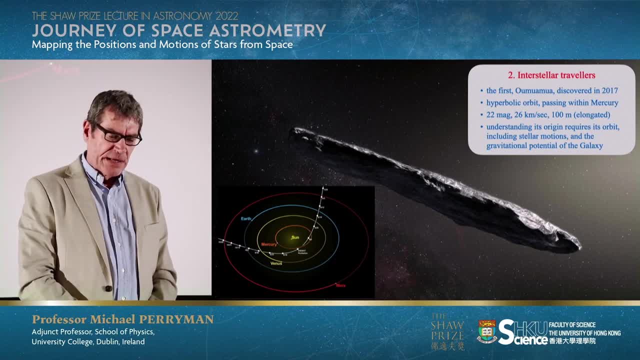 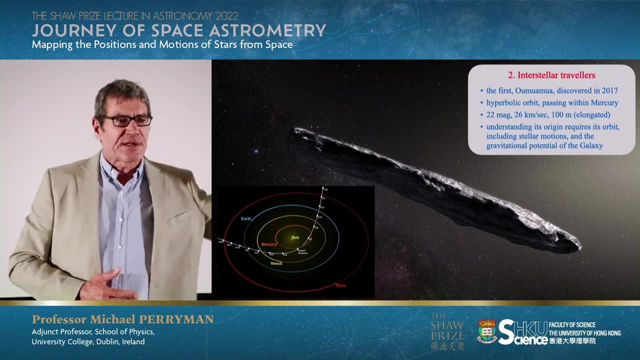 This is a piece of rock that is passing through the solar system, which has an orbit such that we can say definitively it's not bound to the solar system. it must have come in from somewhere and it's going to fly past the sun. 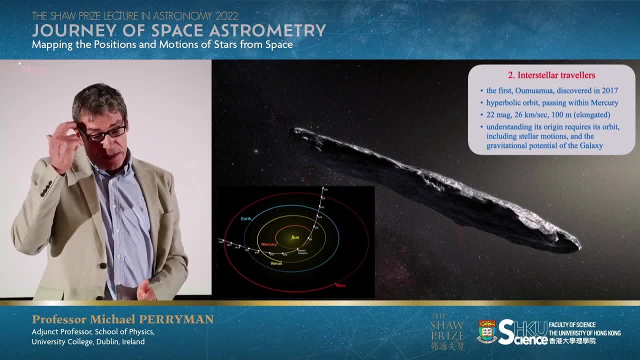 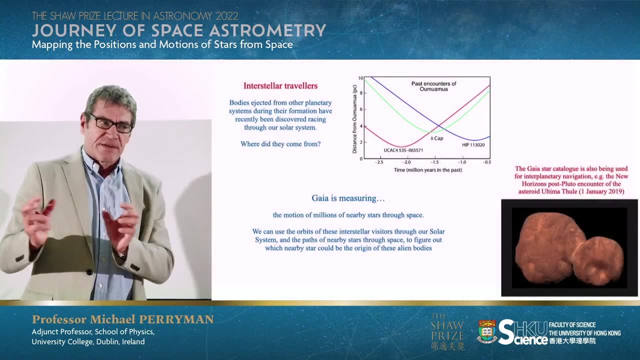 and it's going to head off into space And there was a great excitement with this and one of the things that Gaia is now doing is to taking the orbit of these interstellar travellers and piecing it together with the orbits of the stars. 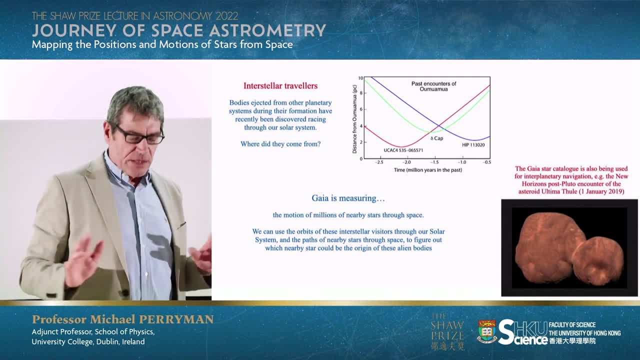 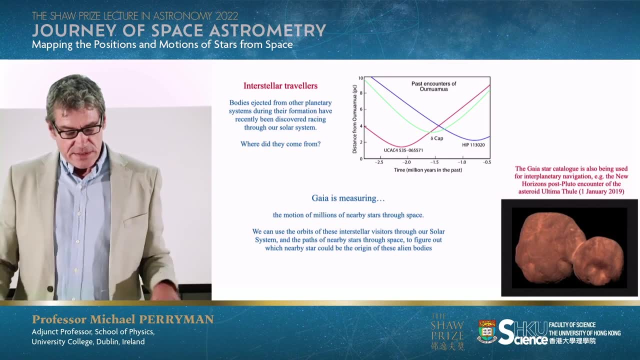 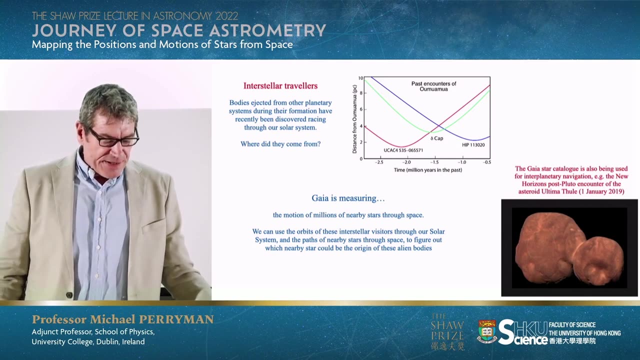 is to figure out which star system close to us this particular piece of rock is. And this particular rock was ejected from. So there's a greater excitement. there's more of these interstellar travellers been discovered since The Gaia system. the stars in the catalogue. 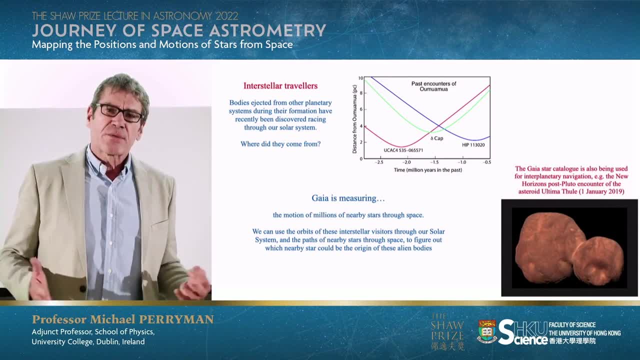 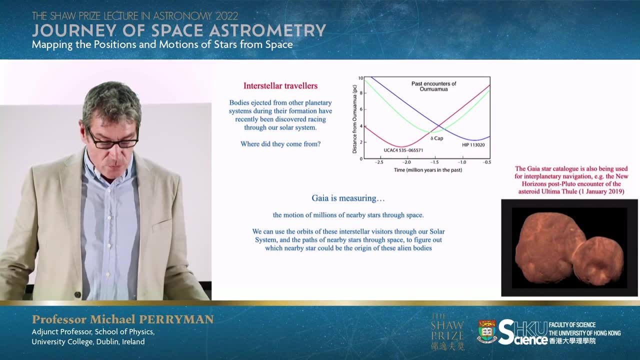 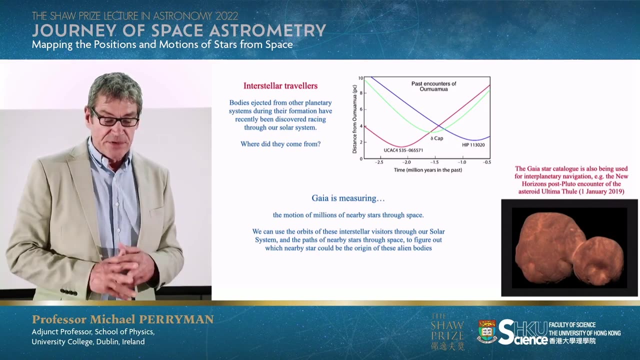 are so accurately placed that they're being used as well for interstellar navigation- sorry, interplanetary navigation. and a highlight three years ago was the reorientation of the New Horizons spacecraft by NASA in its close encounter with an asteroid called Ultima Thule. 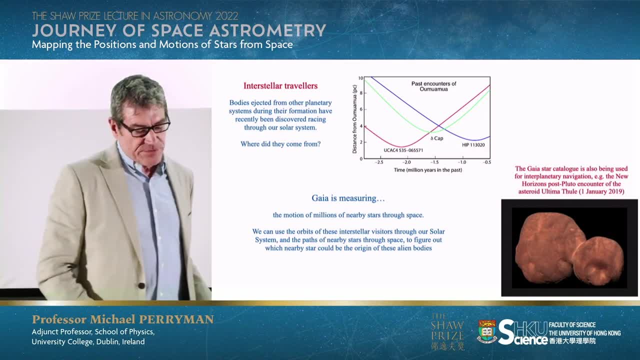 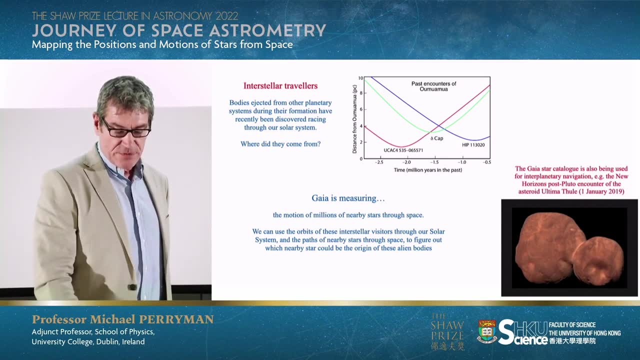 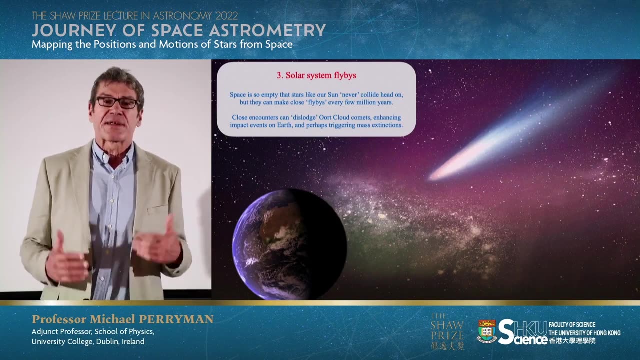 and, using the reference system from Gaia, enabled the imaging camera to be pointed directly and get this great snapshot of Ultima Thule. I move on to the third topic which I want to mention, which is solar system flybys. Our own sun is moving through the galaxy. 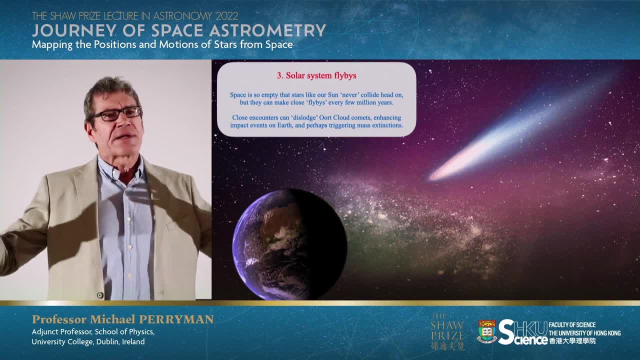 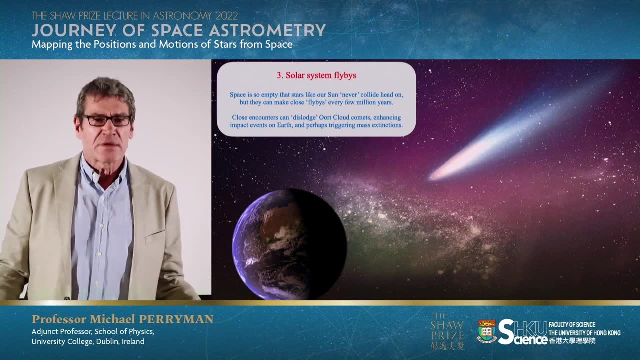 all the other stars are moving through the galaxy. you may ask the question: how long will it take our sun to collide with a nearby star? Well, the answer is fortunately never, or effectively never. It will take thousands of times the age of the universe. 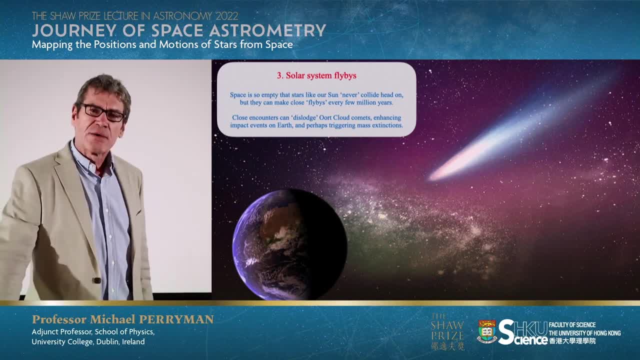 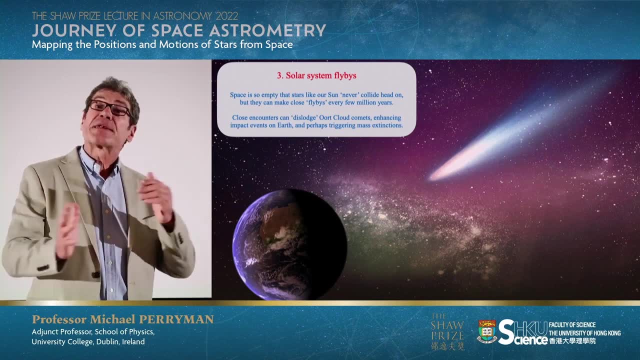 for our sun to stand any chance of hitting one of the other moving stars. But what can happen is that nearby stars which are moving through space can come close to our own star, relatively close to our own star, our own sun. 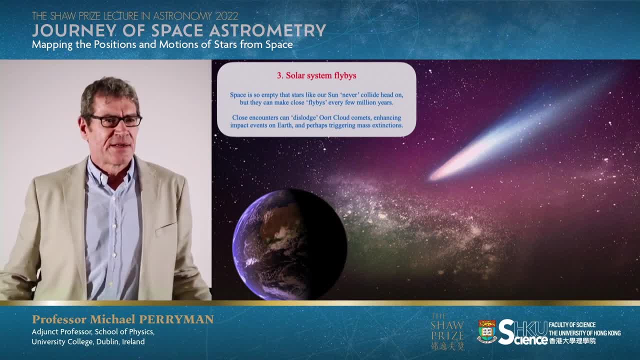 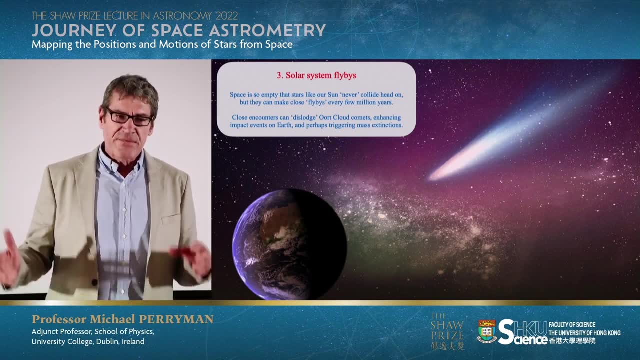 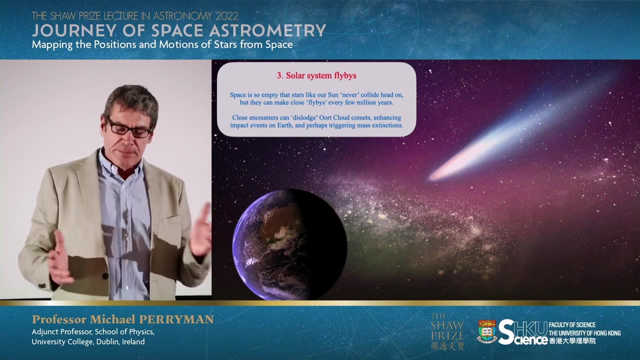 and this turns out, dislodges some of the icy comets that are sitting far out in the solar system, remnants of its early formation, and they can be deflected inwards and create cometary clouds that are timed with these close passages of these stars. 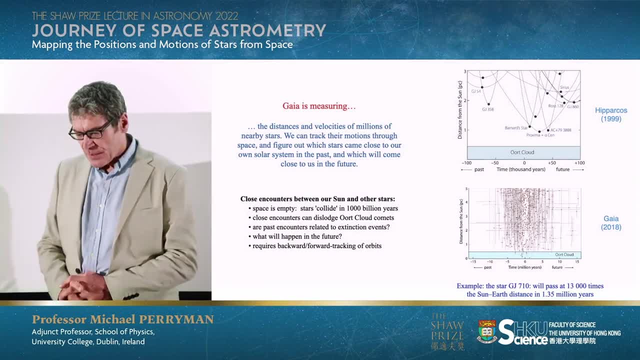 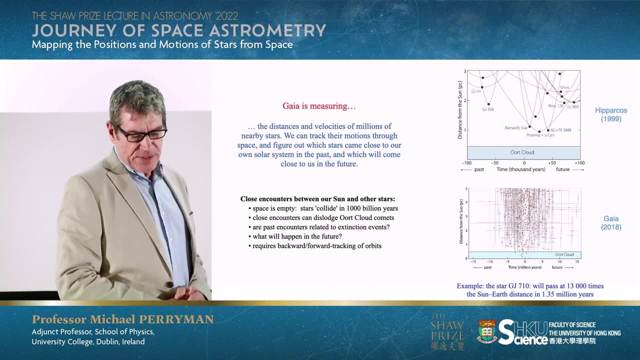 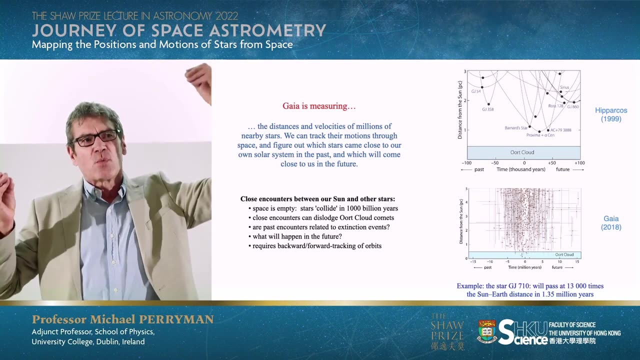 So one of the scientific topics that was started with Hipparchos results and has now become a lot more more precise and rigorous with the accuracy of Gaia, is to look at the stars in our neighboring region of the galaxy and see which ones could have come close to us in the past. 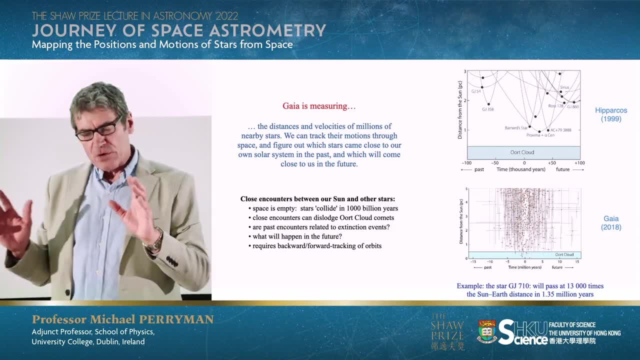 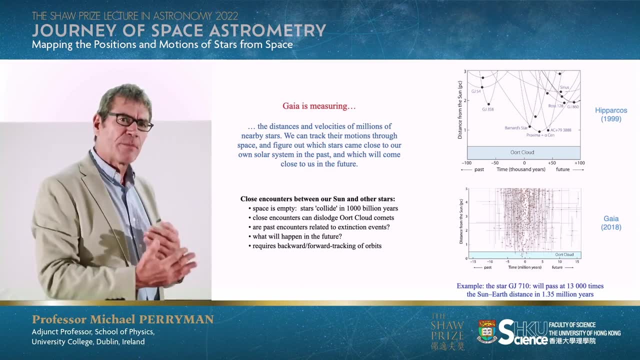 and which ones will come close to us in the future, And some groups. what they're trying to do is to figure out whether these close, stellar passages might have created the kind of cometary impacts that, for example, could have created- could have led to the extinction of the dinosaurs. 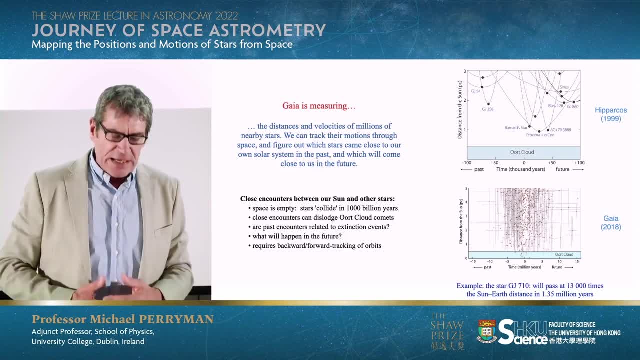 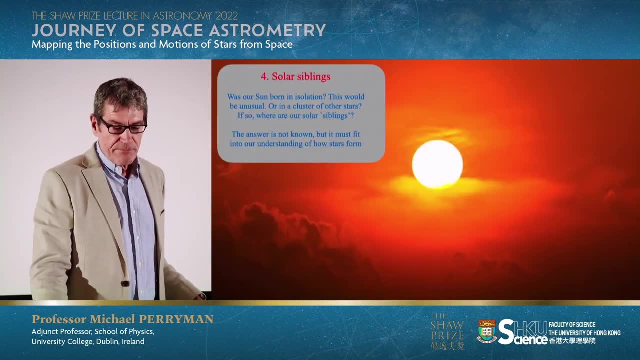 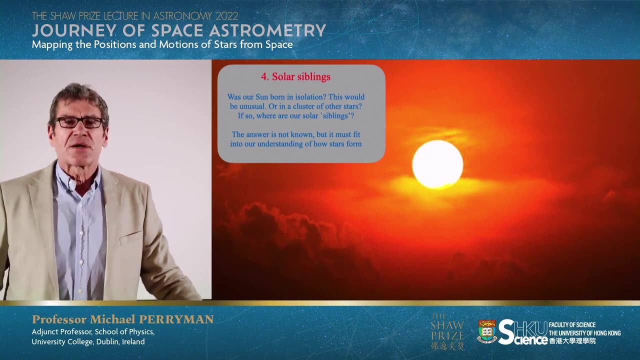 63 million years ago. So stars don't collide, but they can come close enough to disrupt the other bodies in the solar system. The fourth topic that I've selected is to ask a very, very interesting question in astronomy: Was our sun born alone? 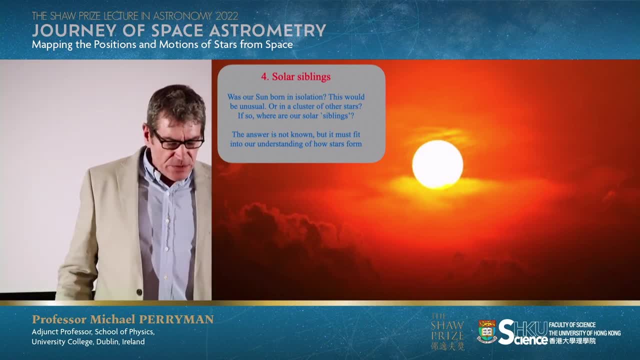 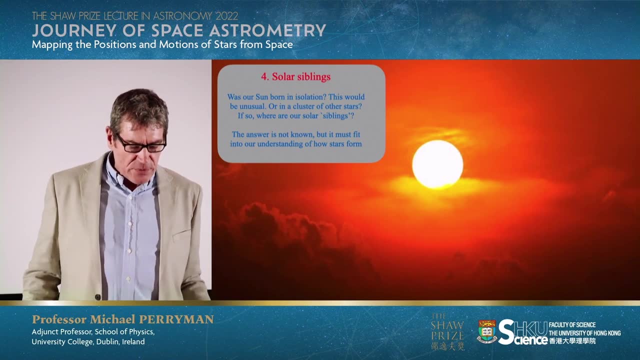 Was it formed on its own? This would be very unusual in astronomy. This is not the way stars are believed to form. Stars are believed to form in groups, clusters and so on. Our sun almost certainly formed in a cluster of other stars. 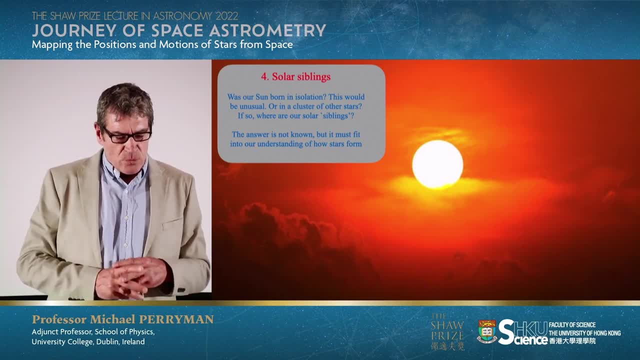 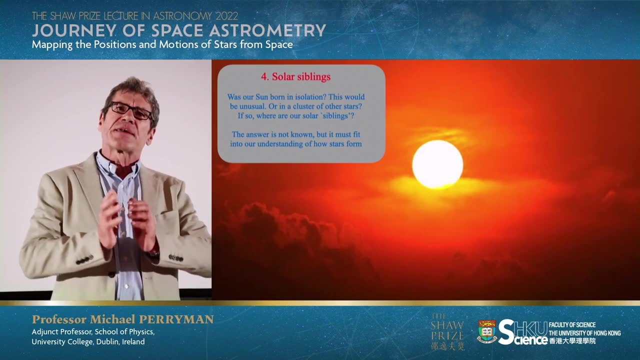 but they're not there now. So where are they? We have sufficiently good models of how clusters disrupt under the influence of the rest of the galaxy and so on to know that these stars, after they've been formed, will move away from us slowly. 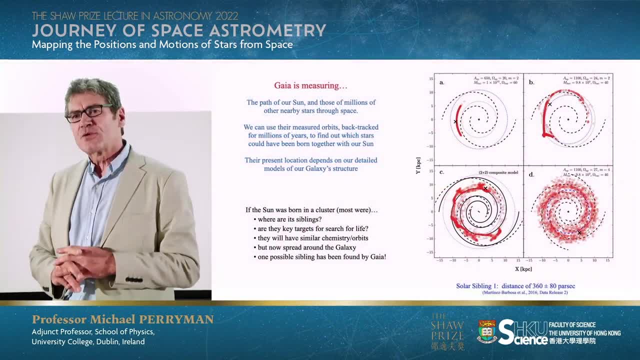 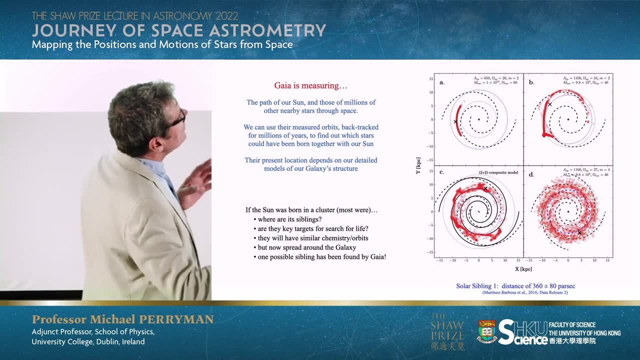 But the interesting thing is that they will continue to move on orbits very, very similar to the orbit of our own sun around the galaxy, And what some groups are now doing is trying to develop different models. These are four different models looking down on the face of our galaxy. and trying to figure out where these stars that could have been formed in the same nursery as our sun. where are they now, And with some success? the first of these candidates- Solar Sibling 1, was announced five years ago already. 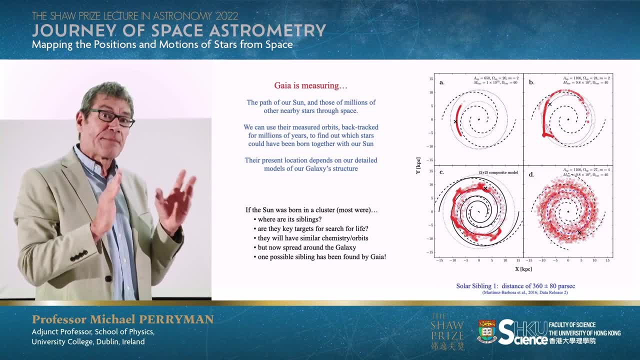 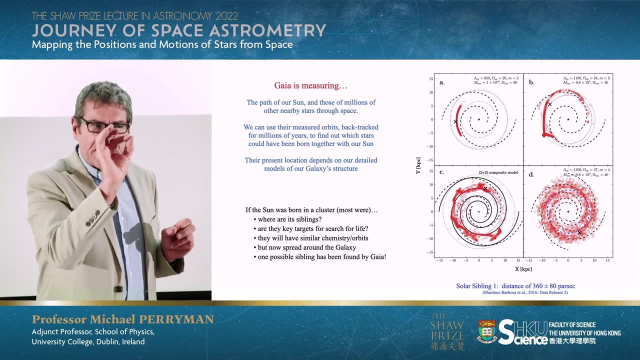 And the interesting thing is that not only these objects share the same dynamical motion as our sun around the galaxy, but they have a very similar chemical composition. So people are starting to look at these stars. This one is about a thousand light years away from us. 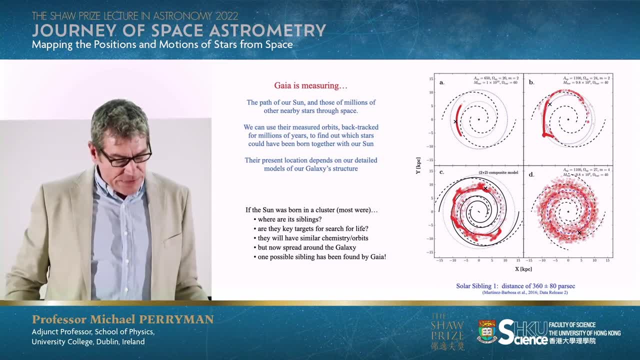 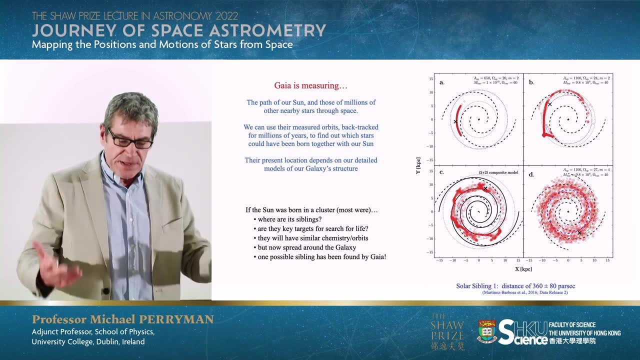 but probably formed in the same stellar cloud. And the idea is, perhaps there are signs of life in these stellar systems, that life formed at a similar time, in a similar way to life in our own solar system. So this is the search for solar siblings. 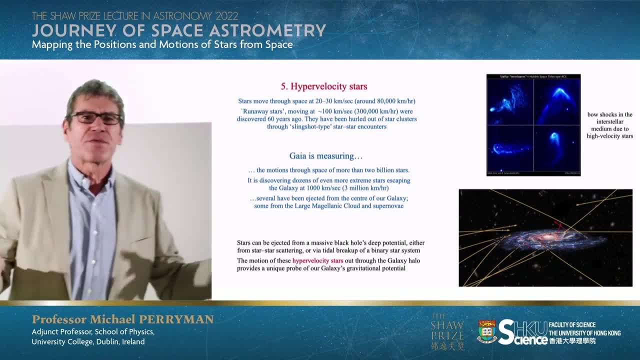 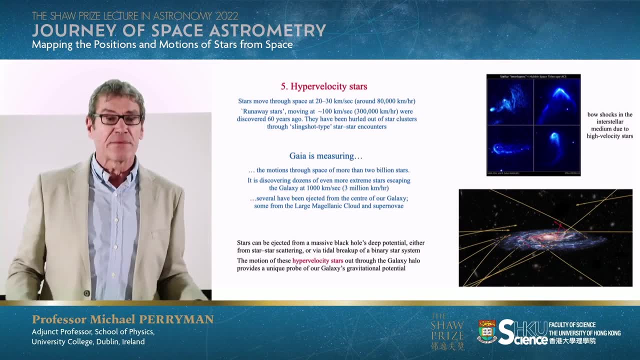 A next example: hypervelocity stars. Stars move through space at about 20 kilometers per second. 20 kilometers per second doesn't sound too much, but that's 80,000 kilometers an hour. There are stars that have been known for 50 or 60 years. 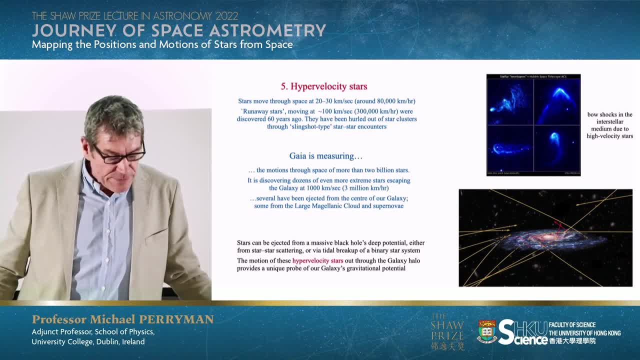 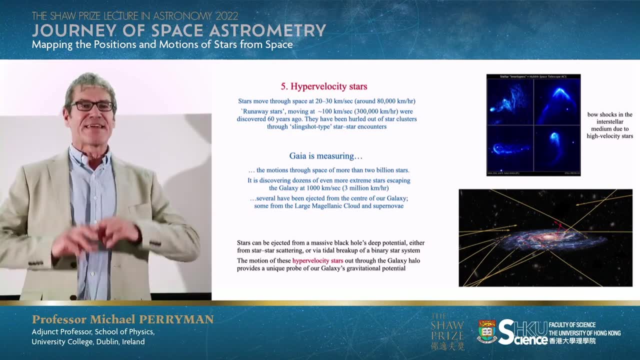 that move at even greater speeds: 100 kilometers per second, Runaway stars, 300,000 kilometers per hour. In the last few years, even faster stars have been discovered, hypervelocity stars. The first was discovered before Gaia. 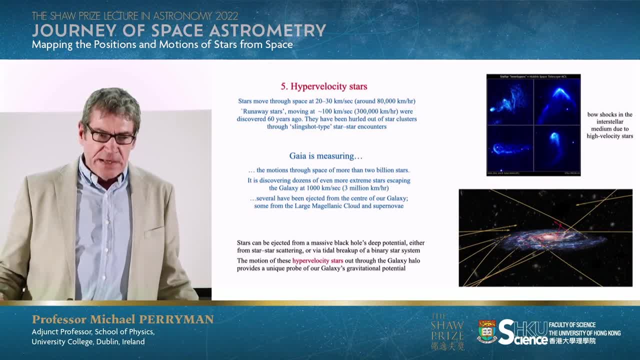 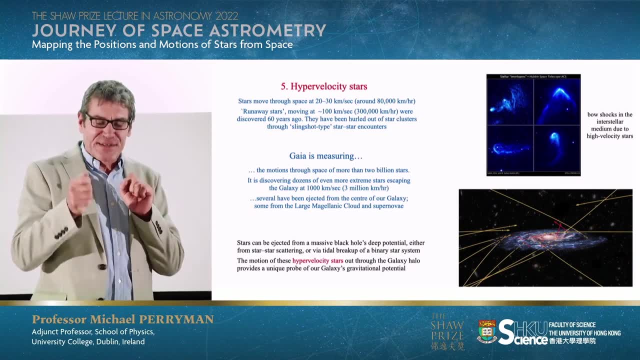 but Gaia is discovering many more of them, And the interesting thing is that it's being able to show where these stars are coming from. We can measure their distances and we can measure their velocities through space and we can trace back where they're coming from. 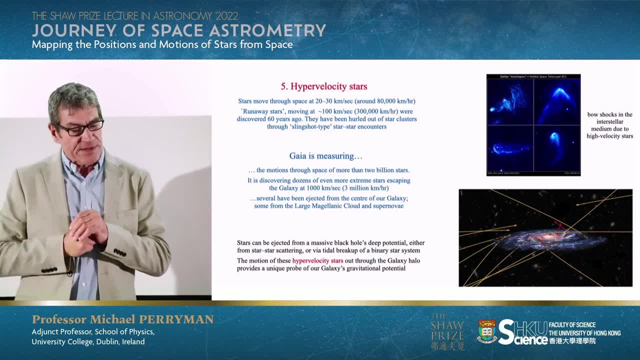 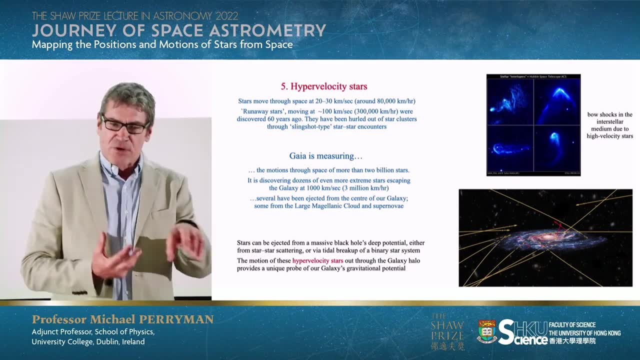 And it does seem that most of these hypervelocity stars are coming from the center of our galaxy, and theoreticians have been busy working on this, figuring out that disruption of stellar systems in the vicinity of the black hole at the center of our galaxy. 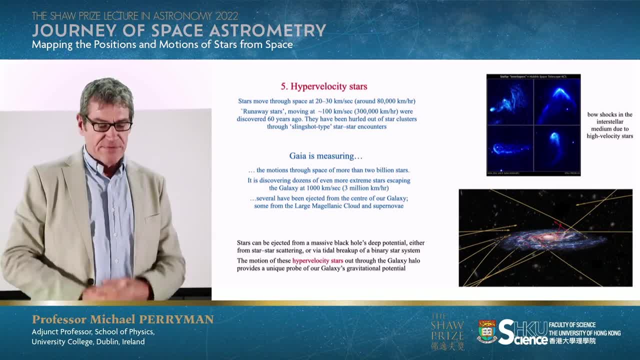 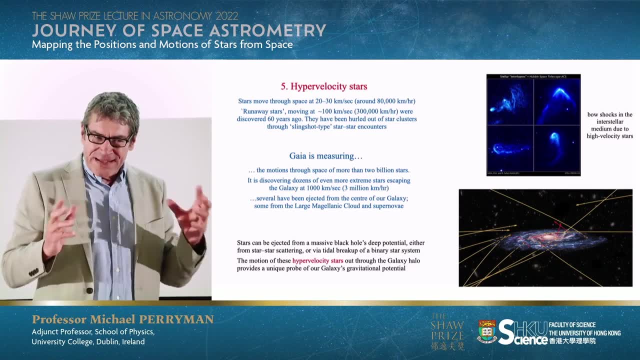 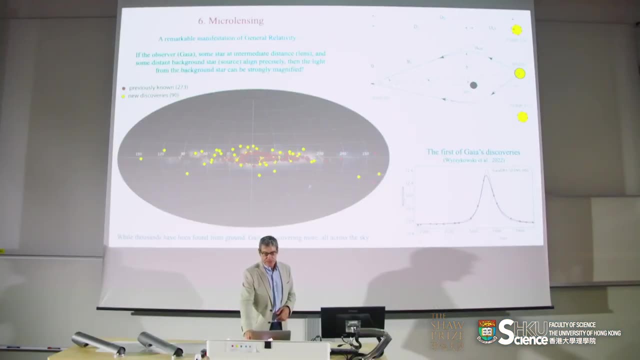 can tear binary systems apart and eject them at very high velocities through space. Again, there are very interesting applications of these: figuring out the mass of our own galaxy and figuring out the halo properties of our galaxy. My penultimate example: microlensing. 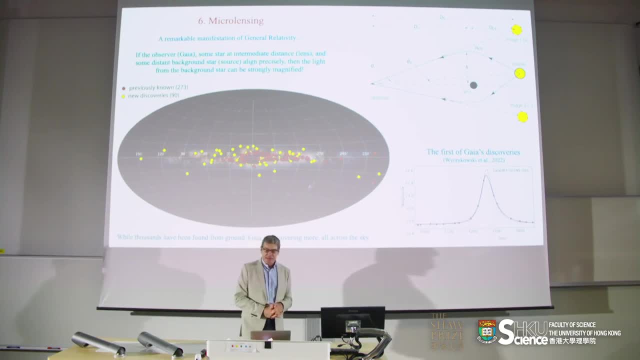 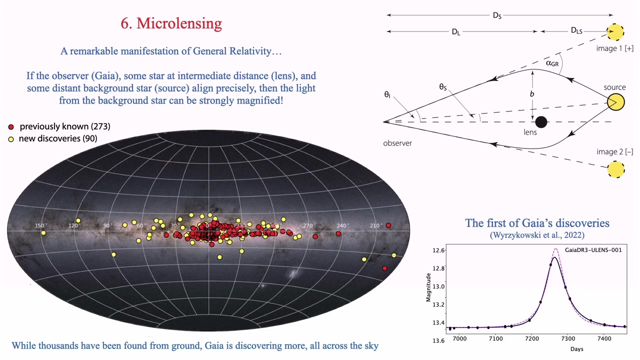 a very bizarre manifestation of general relativity. If you have a star lined up with another star on the path to us as an observer, if it happens that those stars- the observer and the distant star and the foreground star- if it happens that they're lined up almost exactly, 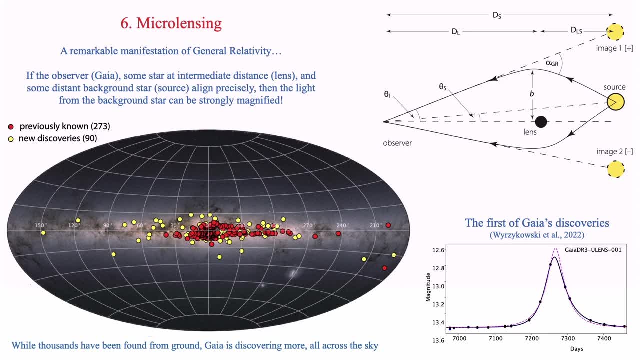 then the foreground star acts as a kind of gravitational lens and the background star suddenly increases. The background star suddenly increases in brightness as it's lensed by the foreground star. Now again, this is not something that was pioneered by Gaia. not at all. 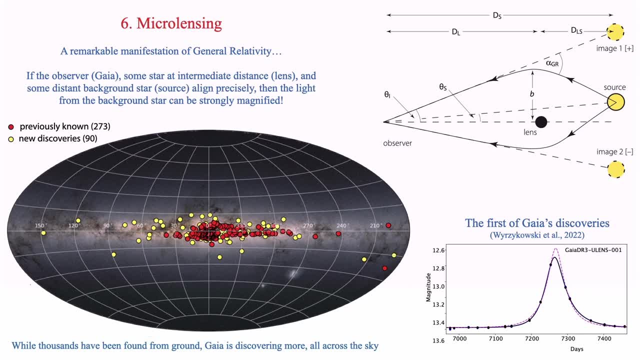 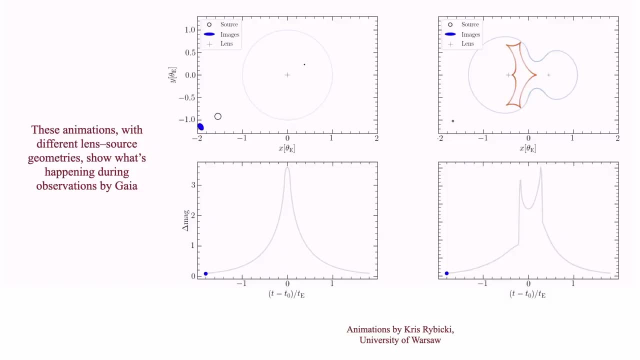 And there are several thousand of these microlensing events that are known already. But what Gaia is doing is searching over the entire sky, and it should be able to measure also the motions of the stars as they're deflected by these lenses. 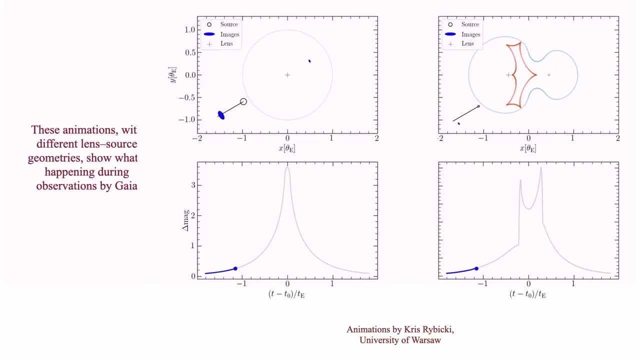 And in these little animations here, which I should go just very quickly, but at the bottom, you can see the light curves that result from the passage of the background star or the foreground star compared to the background star. So again, I've covered that topic very, very quickly. 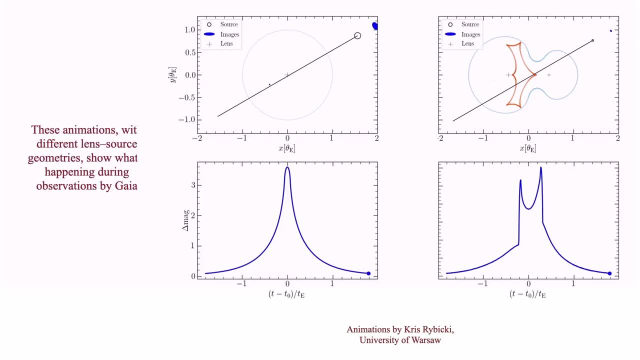 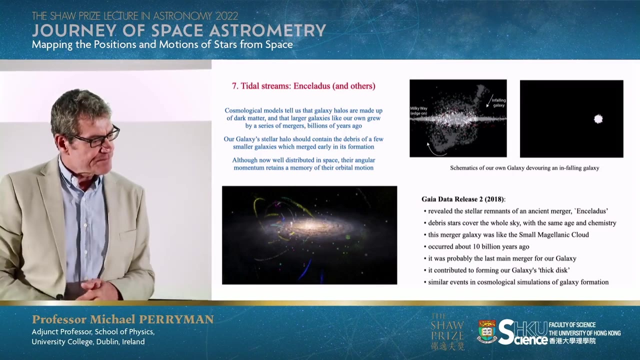 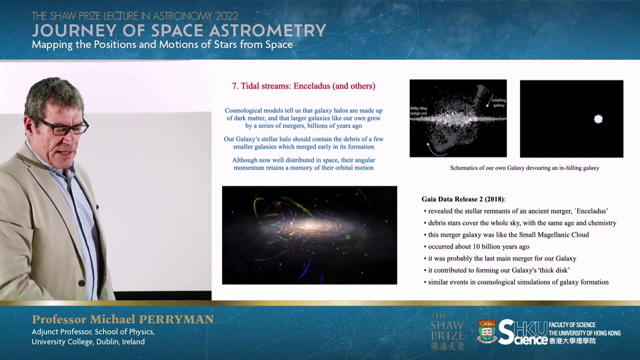 but it's one of the bizarre manifestations of nature, this curious alignment that can occur and give rise to observable phenomena that we can measure and disentangle a lot about the nature of these stars. My final example is on a much bigger scale. It started to become apparent perhaps 20, 30 years ago. 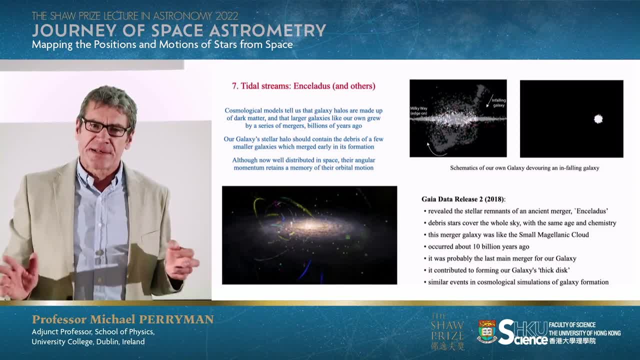 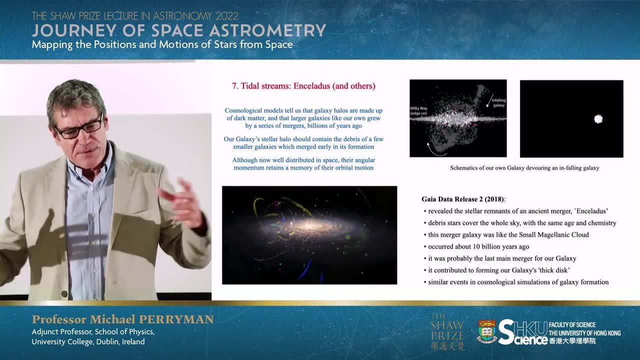 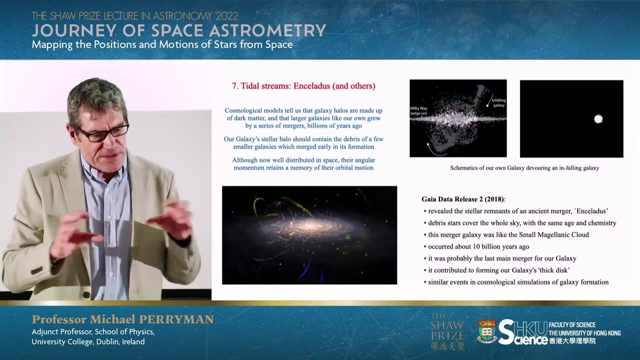 that our own galaxy formed by cannibalizing other galaxies. Our own galaxy is quite large. When the universe was created, there were smaller galaxies there, many smaller galaxies in our local group, And the idea that cosmologists have put together in their models. 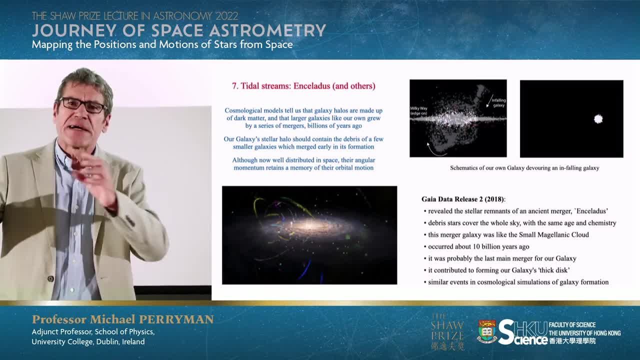 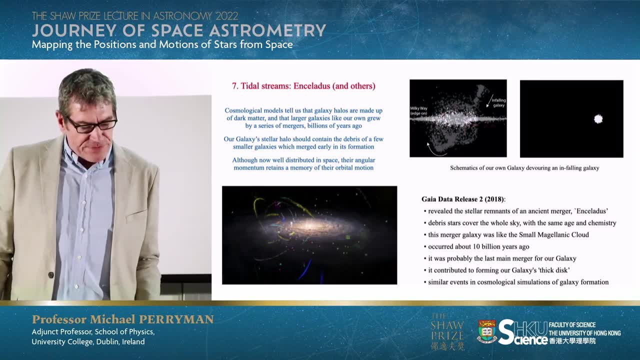 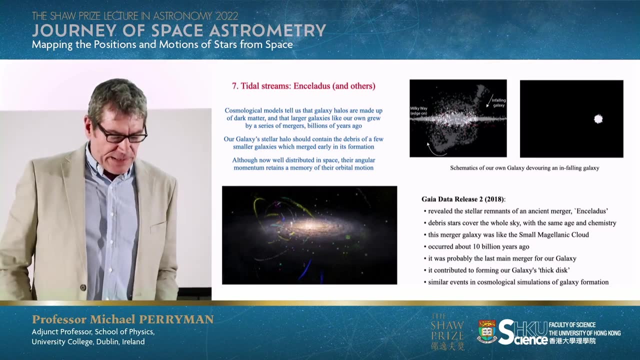 is that our own galaxy will have grown by devouring some of these smaller galaxies in the distant past. The first signs of this came already from Hipparchos, And with Gaia there are many more of these streams being discovered. The first of them is called Enceladus. 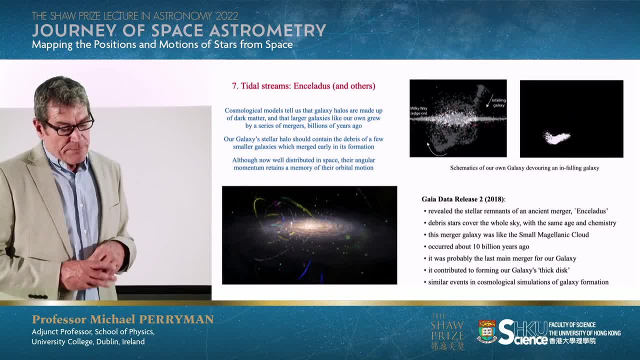 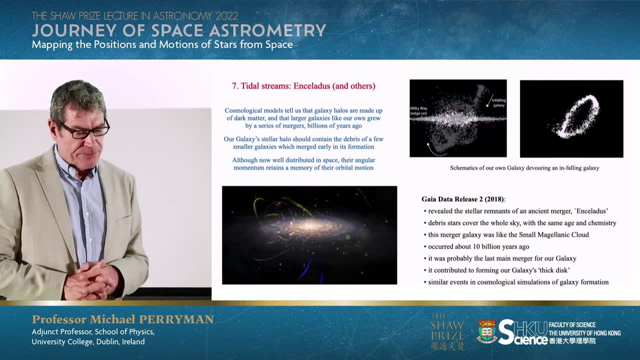 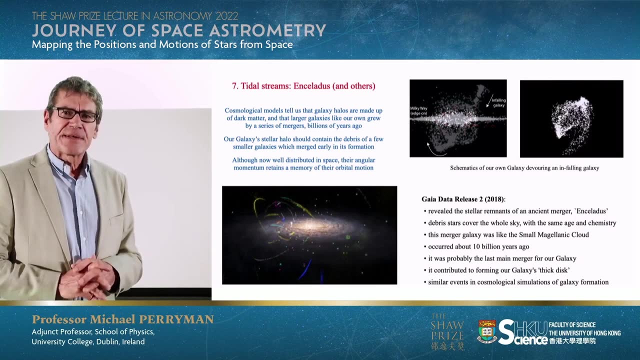 It's believed to be the last major merging event that took place between our galaxy and a precursor galaxy something like 10 billion years ago, And the more of these systems that we can measure, the more secure we can be about piecing together the history of the formation of our own galaxy. 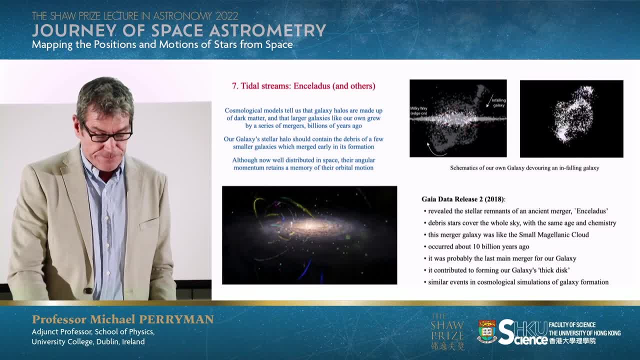 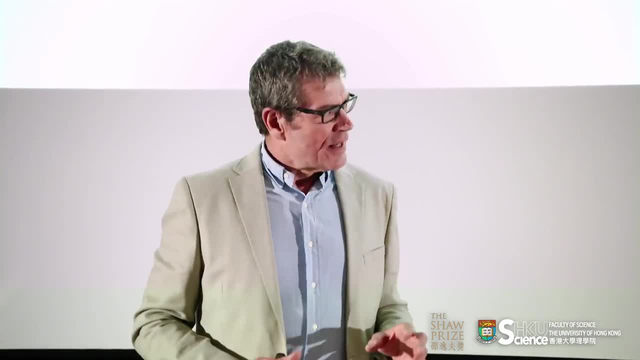 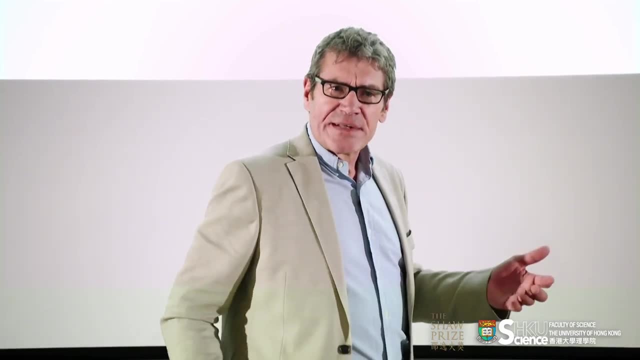 and the history of the evolution of our universe as a whole. So these are really just a few quick, short examples. I've gone over them far too quickly for you to be able to understand many of the details, but I hope this is just this little snapshot. 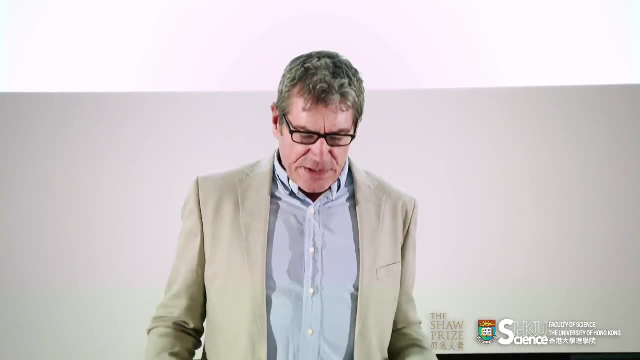 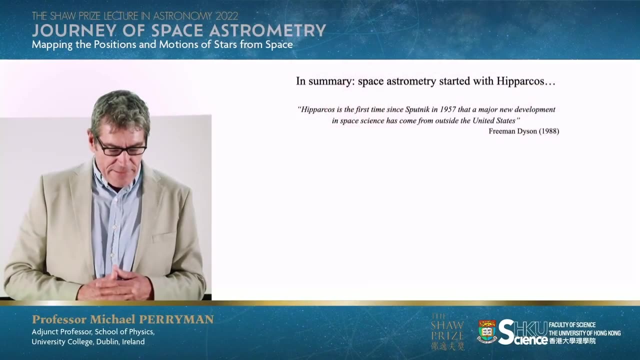 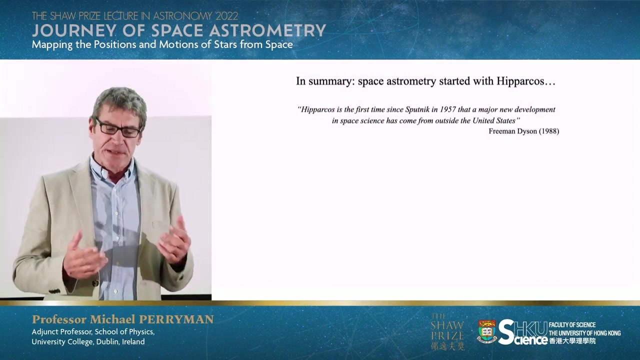 is giving you a clearer picture of some of the science that is going to come out of an advanced technological mission like this. In my summary, then, I'll say space astrometry- Astrometry measuring the positions of the stars. Space astrometry started with Hipparchos. 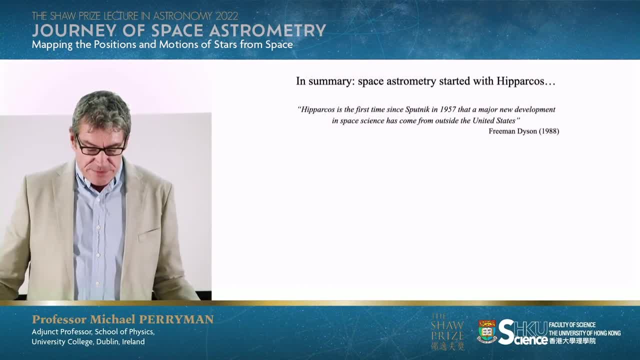 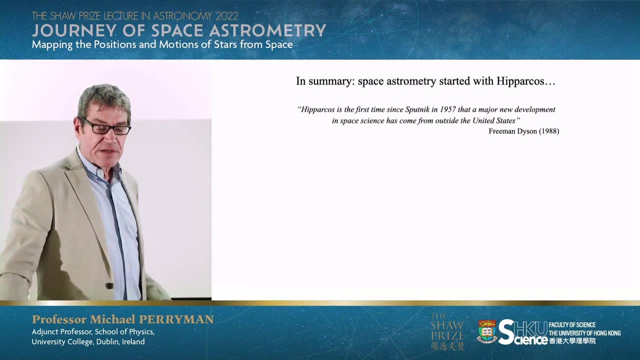 with the European Space Agency And in fact a very eminent physicist, Freeman Dyson, wrote in 1988 that Hipparchos was the first time since Sputnik in 1957 that a major new development in space science has come from outside the United States. 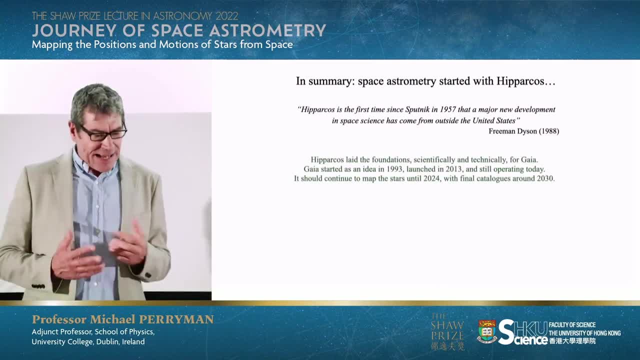 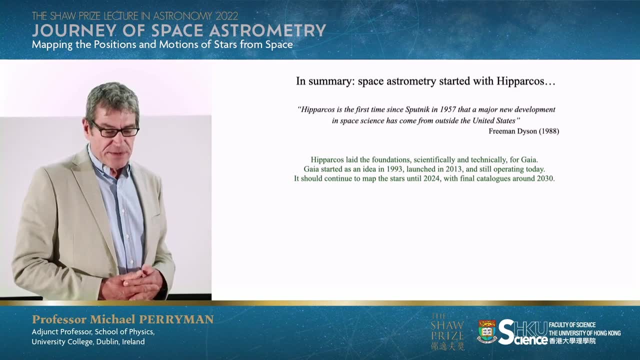 Hipparchos really laid the foundations, scientifically and technically, for Gaia. Gaia started as an idea back in 1993, it was launched in 2013,. it's still operating today and it should continue to map the stars until 2024 or thereabouts. 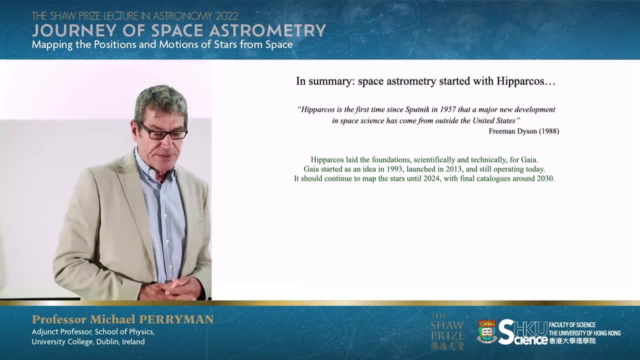 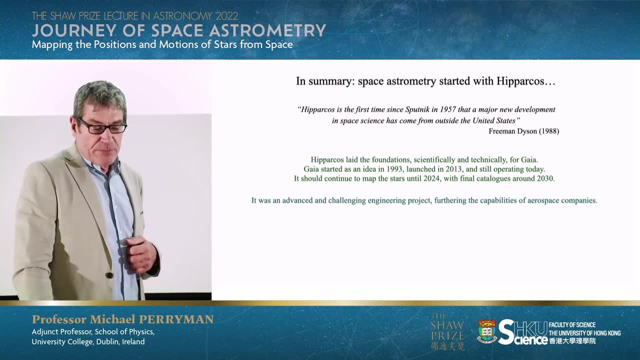 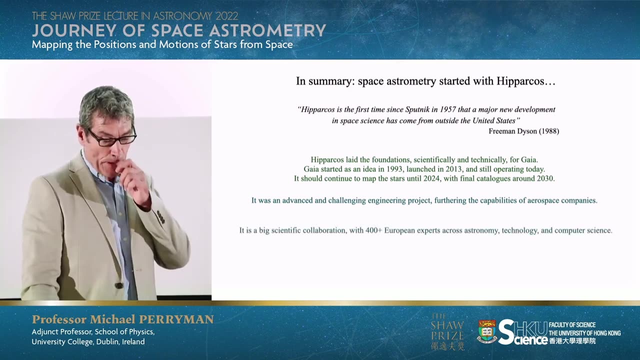 with final catalogues coming out in about 2030.. It was an advanced and very challenging engineering project, furthering the capabilities of aerospace companies as well as pushing forward the boundaries of science. I should stress that it's a huge scientific collaboration. there are 400 or more European experts. 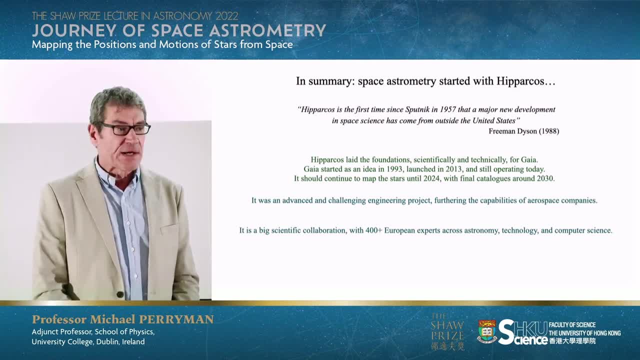 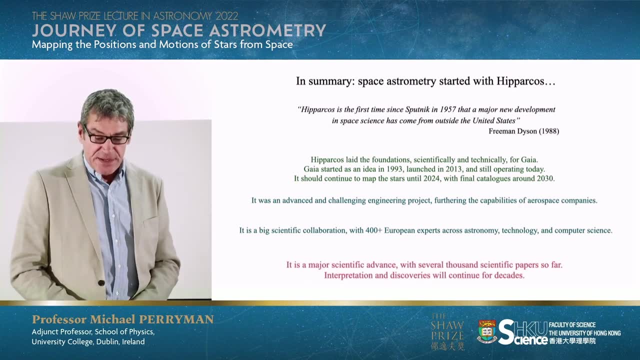 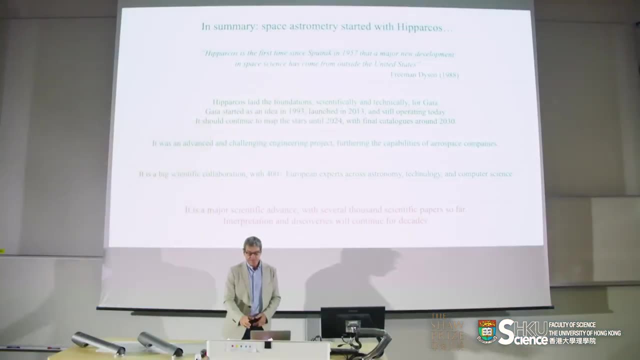 across the fields of astronomy, technology and computer science working on it today. It's a major scientific advance. several thousand scientific papers have been published so far and the interpretation and discoveries will continue for decades. I'm going to play out with a video. 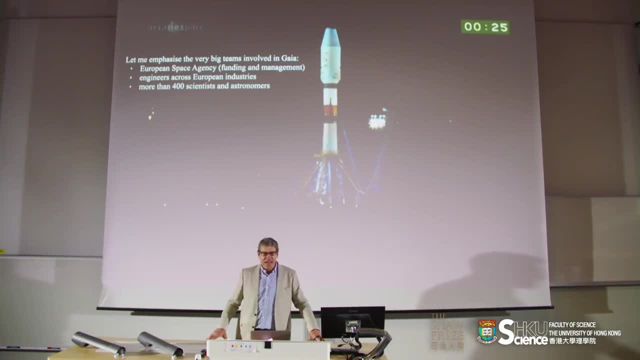 I haven't told you how Gaia works. I haven't told you the great challenges in building it. I haven't told you how the data is analysed on the ground. I've just given you this snapshot of what it is we're trying to achieve scientifically. 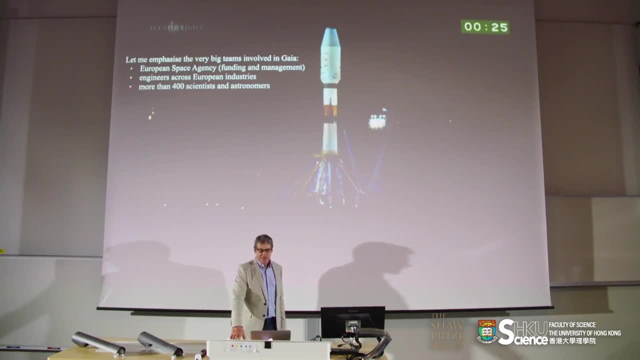 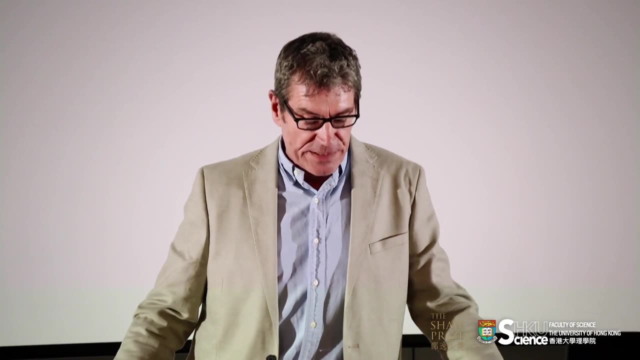 But let me just show you the launch of this, a very spectacular event in December 2013,. and as I play it out, let me emphasise again that very big teams are involved in these space missions, like Gaia. Among those, credit the European Space Agency. 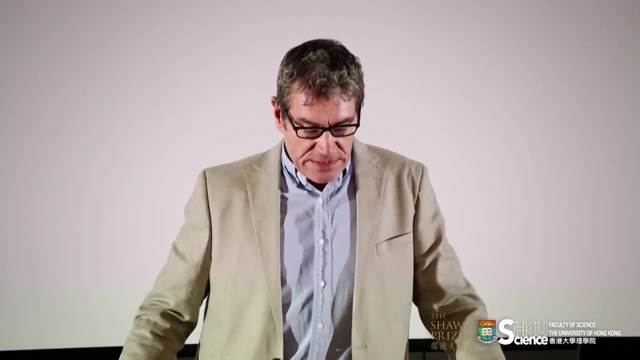 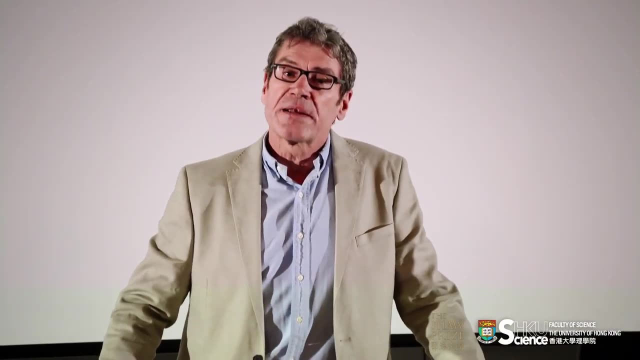 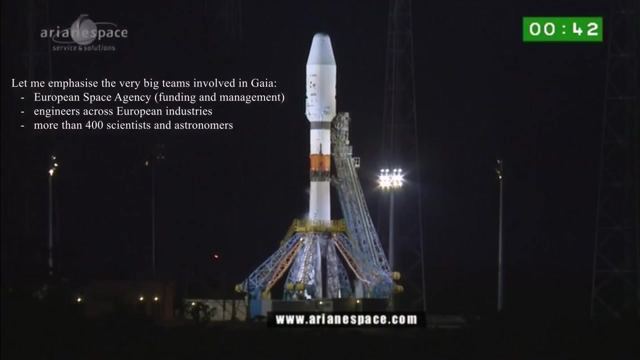 for the funding, the management, the innovation and the initial acceptance of these ideas. tremendously skilled engineers across European space industries that are able to put these kind of missions together and, as I said, more than 400 scientists and astronomers throughout Europe working on the data. 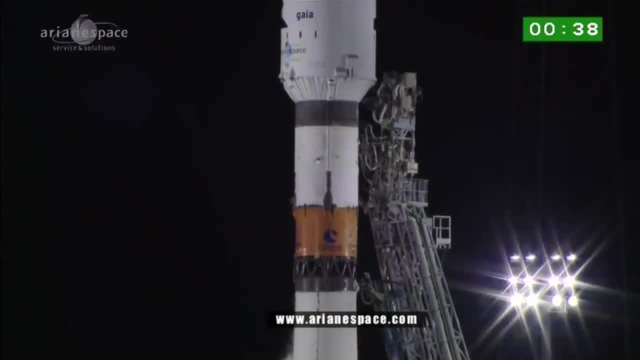 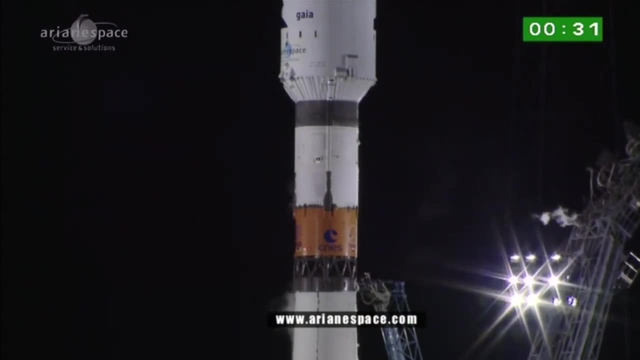 The ignition sequence is in three stages. part of it is a sequence from minus 17 seconds down to minus 6 seconds, during which the engines are tested. There are the arms rolling away. that's one of the final moments. At minus 15 seconds is the first controlled ignition. 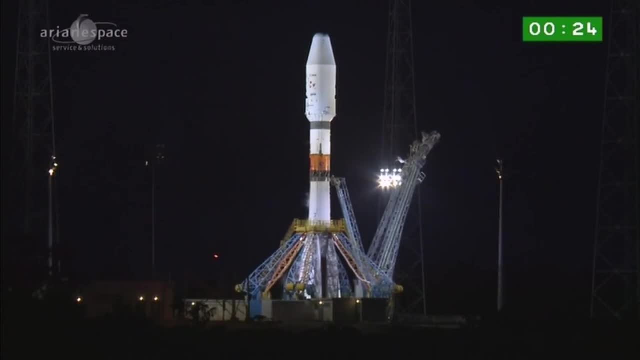 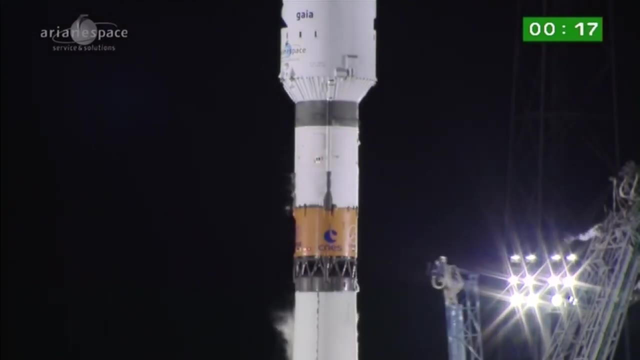 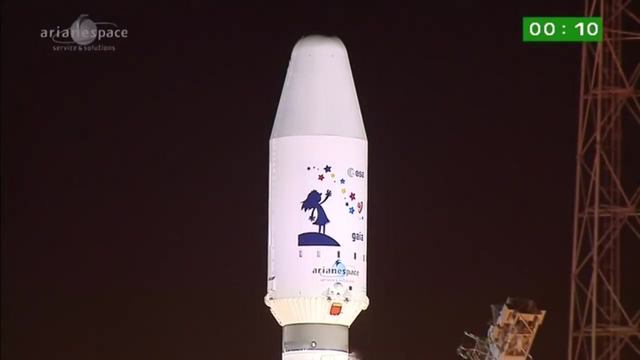 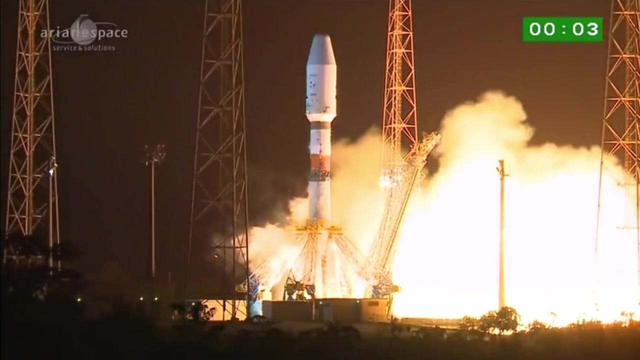 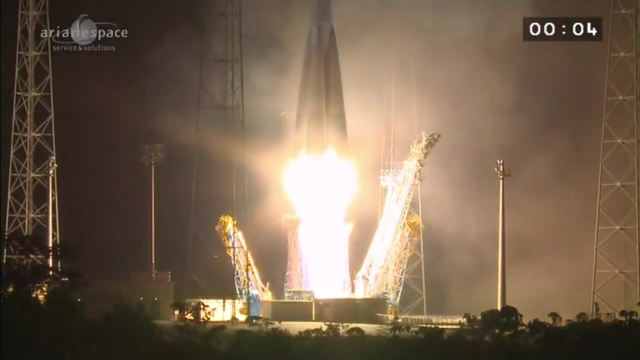 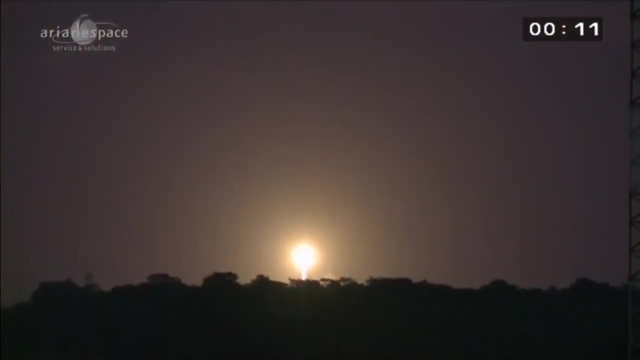 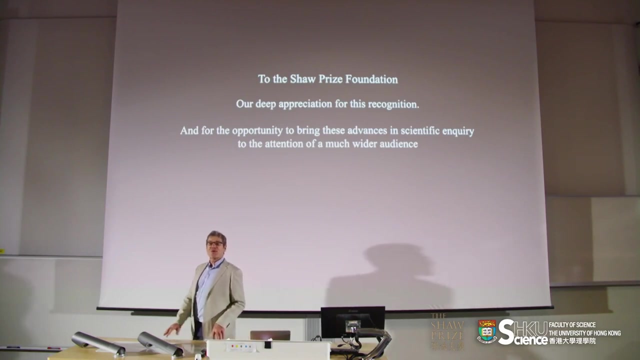 at minus 7 seconds is another control. There's another one at about half pressure and then at minus 3 seconds the order is given for the third and final phase. There's the gantry arms going. It's still very emotional watching that launch. 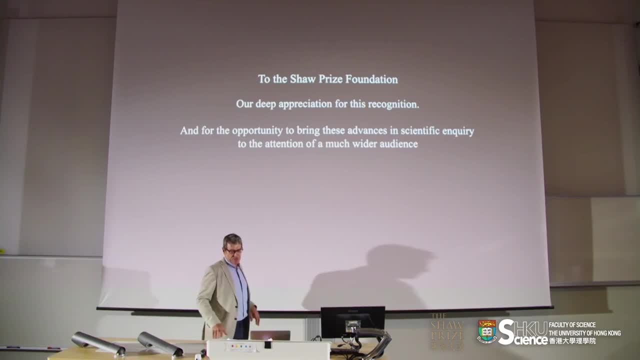 knowing that you've consigned this delicate piece of engineering to the top of these massive rockets. That brings me to the end of my presentation. May I say finally, of course, to the Shaw-Price Foundation, our deep gratitude and appreciation for this recognition. 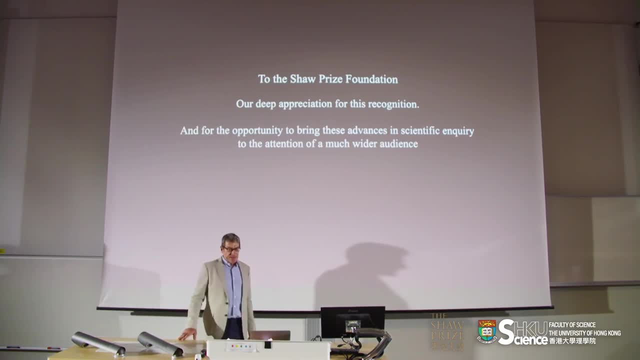 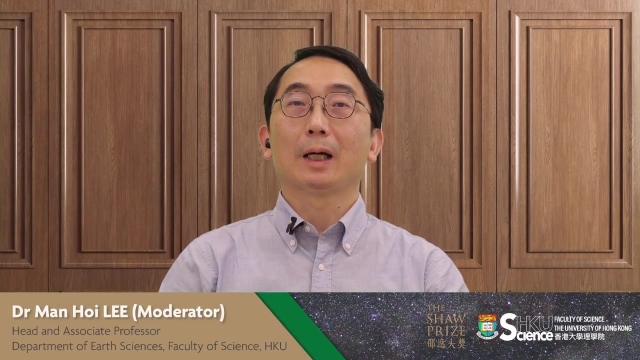 and really for the opportunity to bring these advances in scientific inquiry to the attention of a much, much wider audience. Thank you, It is a truly inspiring lecture. Thank you, Professor Perryman. Next, we are very glad to have Professor Lindegren. 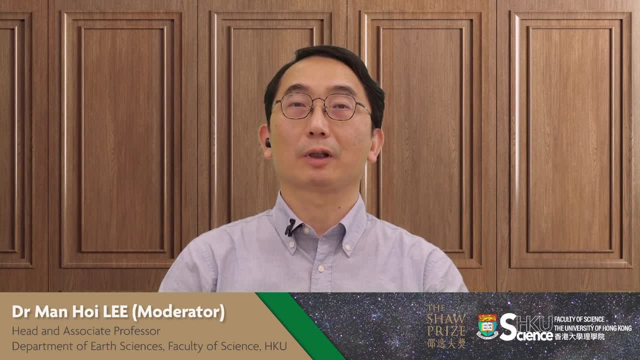 to share his insight on fundamental concepts of global astrometry. Professor Lennart Lindegren was born in 1950 in Sweden and is currently Professor Emeritus of Lund Observatory Department of Astronomy and Theoretical Physics at Lund University in Sweden. 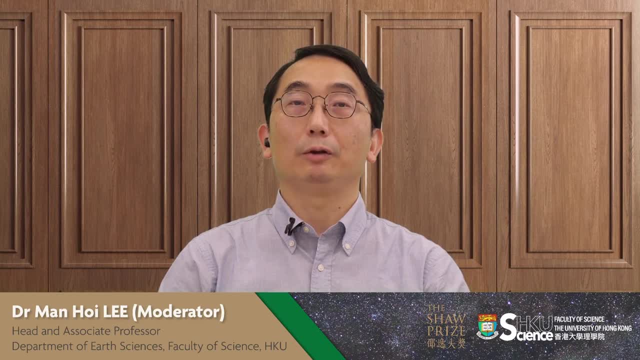 He received his PhD in 1980 from Lund University. He then joined as a member of the teaching staff at Lund University and became Fru Professor of Astronomy in 2000,, serving until his retirement in 2017.. During this time at Lund Observatory, 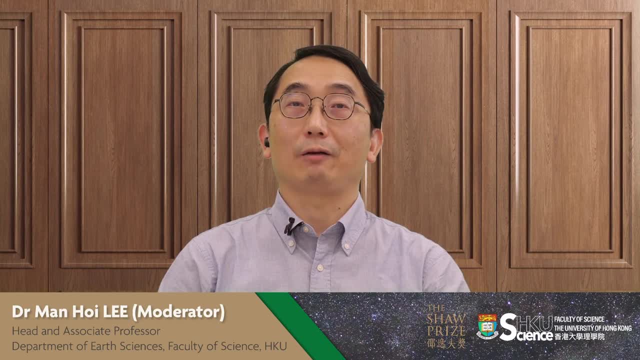 Professor Lindegren had served as the director for six years. He was a member of the European Space Agency's Hipparco Science Team and Gaia Science Advisory Group. He leads the scientific implementation of the astrometric global iterative solution in the Gaia Data Processing and Analysis Consortium. 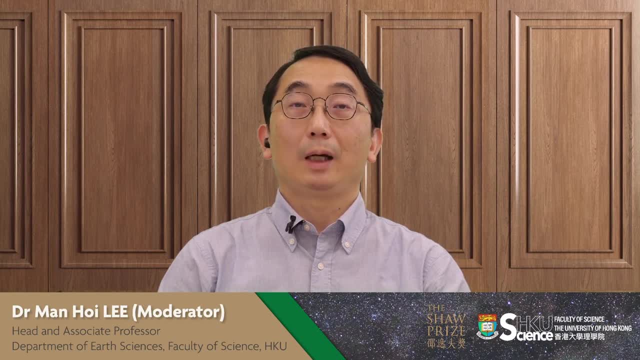 and is also a member of the Gaia Science Team. He also served as project coordinator for the Marie Curie Research Training Network. He is a member of the Royal Swedish Academy of Sciences. In the following lecture, Professor Lindegren will describe how optical observations 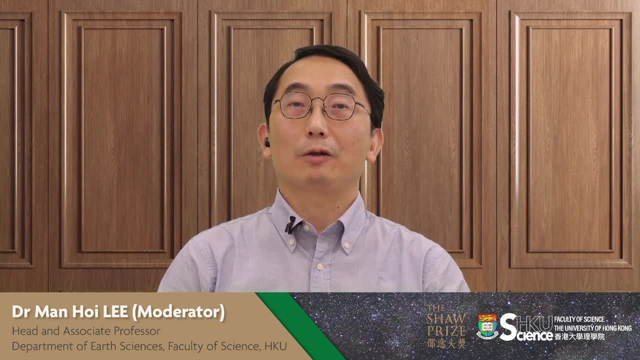 using a scanning satellite, allow us to measure accurate, absolute parallaxes and proper motions, and to build a rigid reference frame over the whole celestial sphere. The principle was first applied to Hipparcos data in the 1990s and the same principle is now used for Gaia. 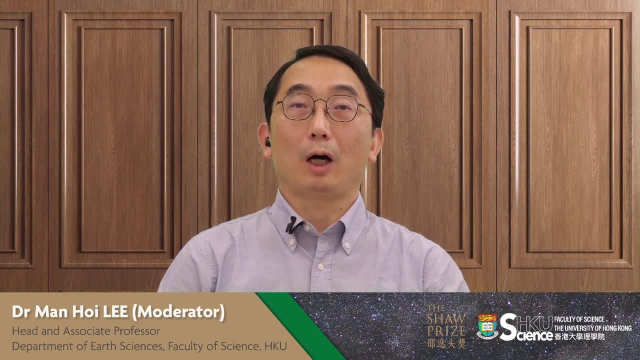 The intertwined measurements of all objects bring formidable data processing challenges that could not be mastered for Hipparcos without certain approximations. The exponential growth in computing power since then makes it possible to treat the Gaia data much more rigorously, in spite of the immensely larger data volume. 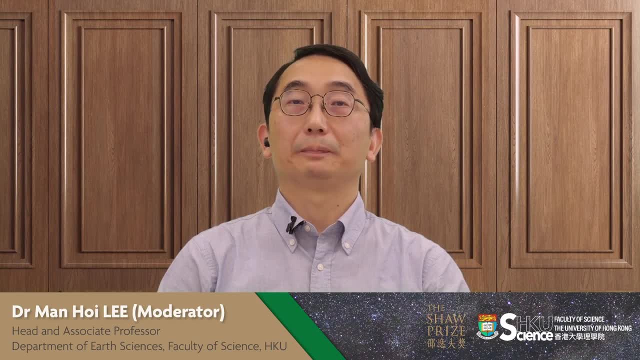 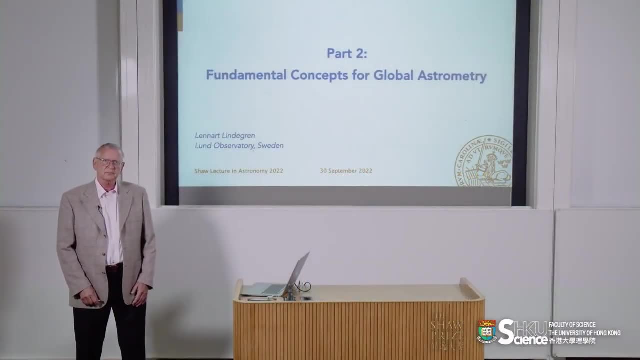 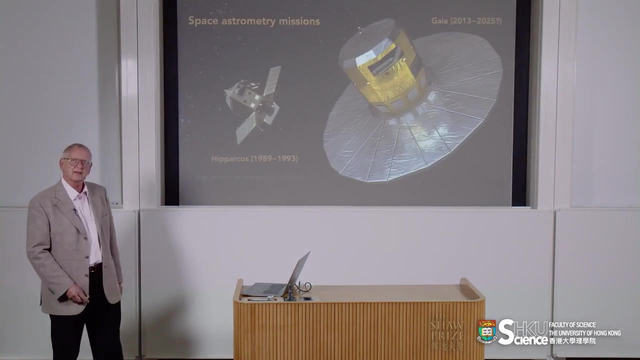 Now please join Professor Lindegren's lecture. In this second part of the lecture, I want to explain some fundamental concepts underlying the two very successful space astrometry missions, Hipparcos and Gaia. Hipparcos was launched in 1989,. 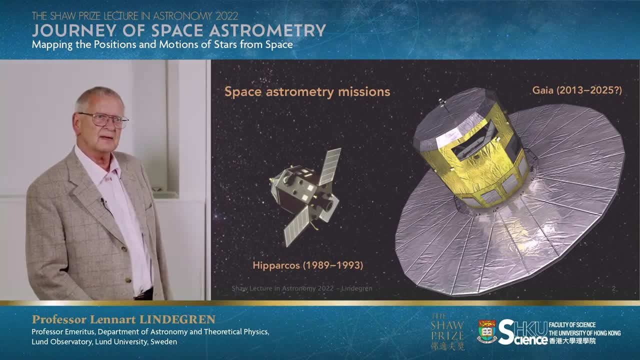 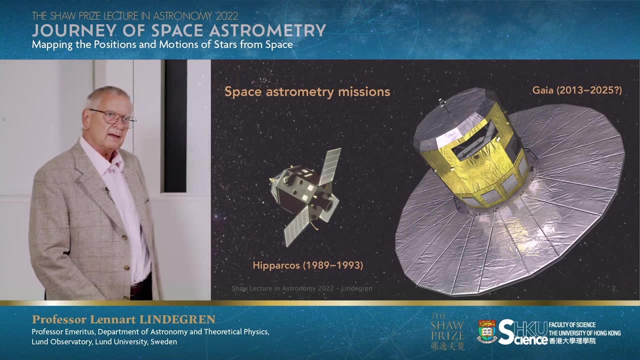 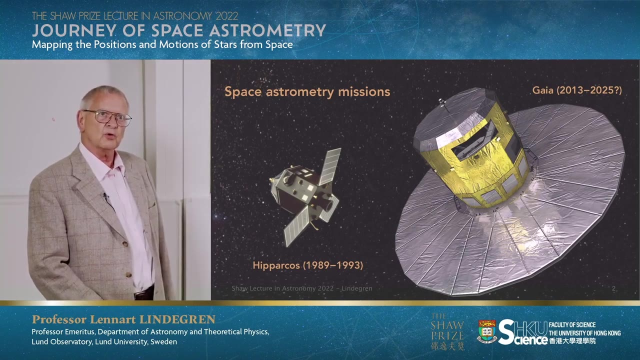 and the data came out eight years later. Gaia was launched in 2013,, and it is still operating. Gaia is, of course, much bigger, both in size, as shown in this drawing, and in scope and in accuracy. 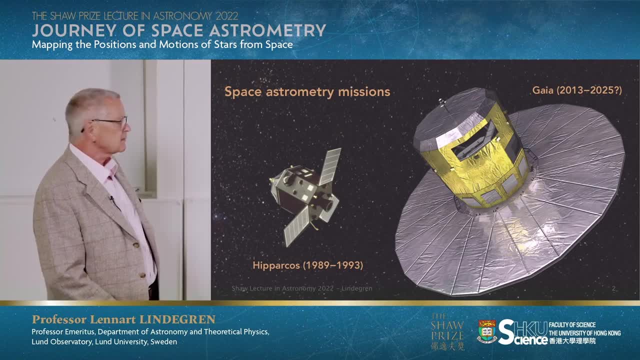 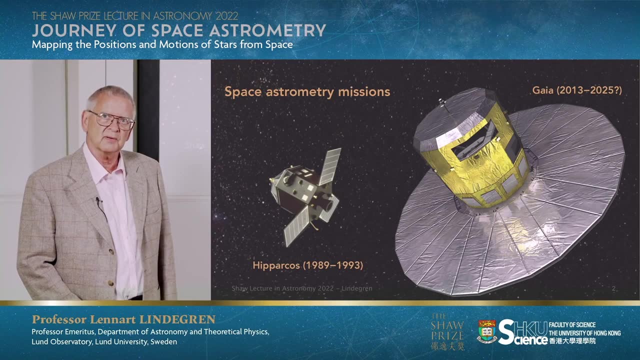 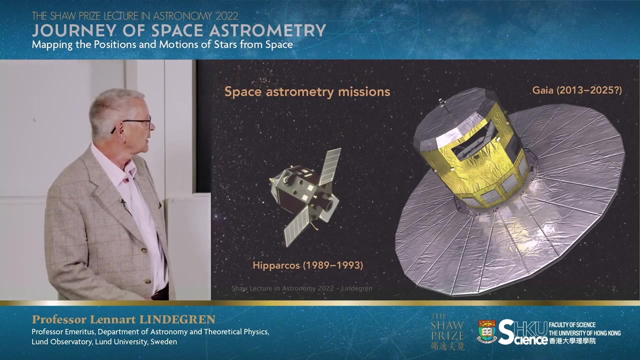 and in almost every respect. But the two missions are actually fundamentally very similar because they are using the same principles for doing astrometry from space, And that is what I want to explain in this talk. I will focus on the global nature of these missions. 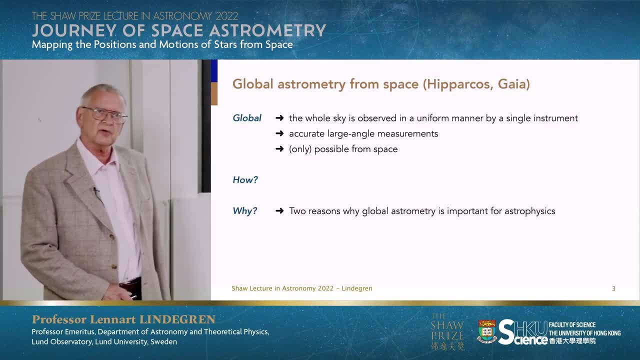 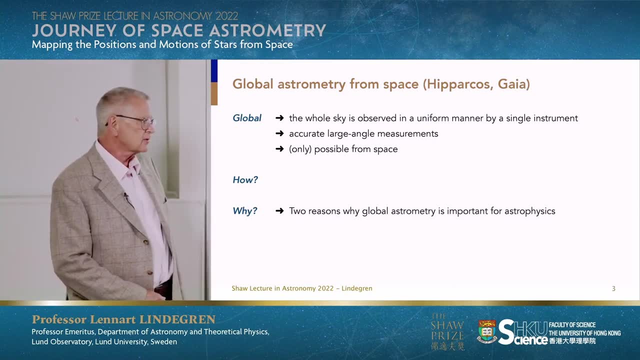 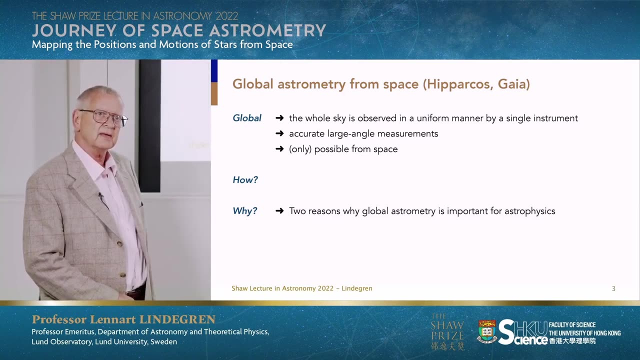 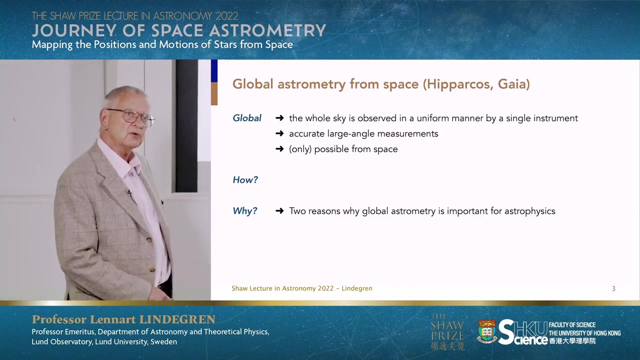 Global means that the whole sky is observed in a uniform manner from a single instrument. This requires accurate, large-scale measurements over the whole sky, which, as we will see, is only possible from space. I will explain how this is possible, but first I will give two good reasons. 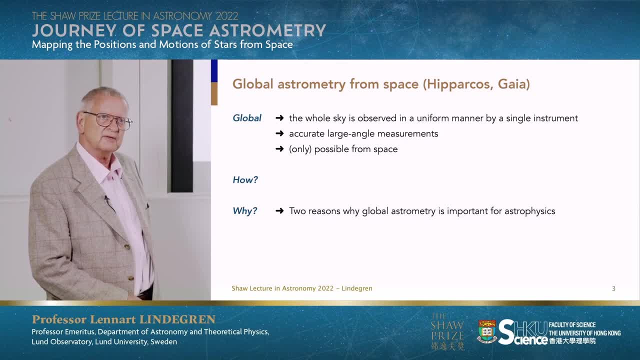 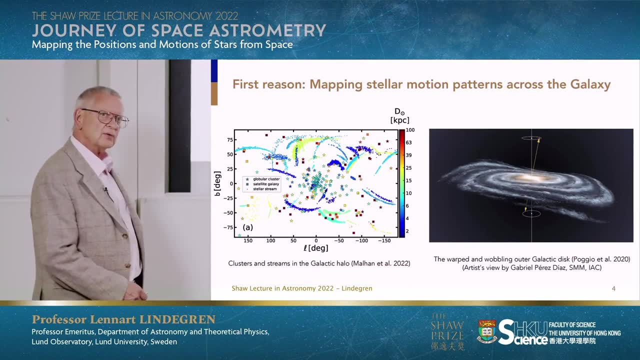 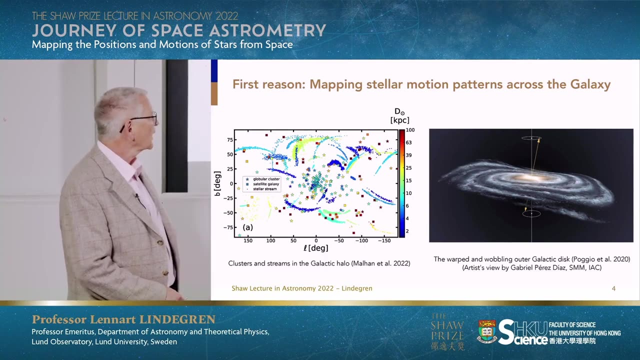 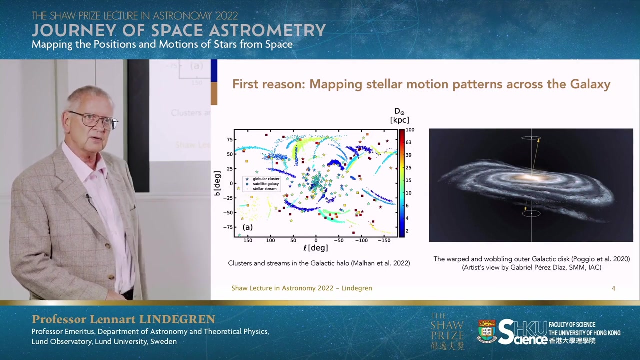 why such global astrometry is important in astrophysics. The first reason is that, in order to understand how our galaxy is built, how it is formed and how it works, we need to map stellar motions across the whole galaxy. And because we are sitting inside the galaxy, 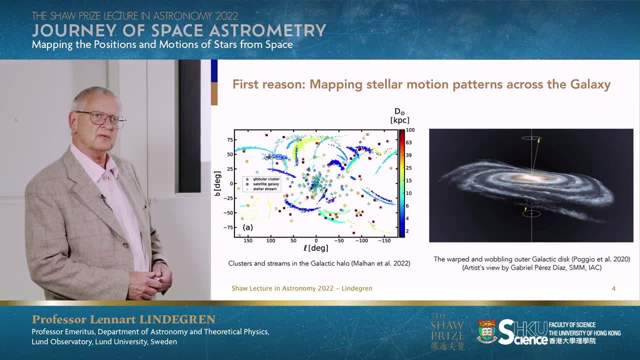 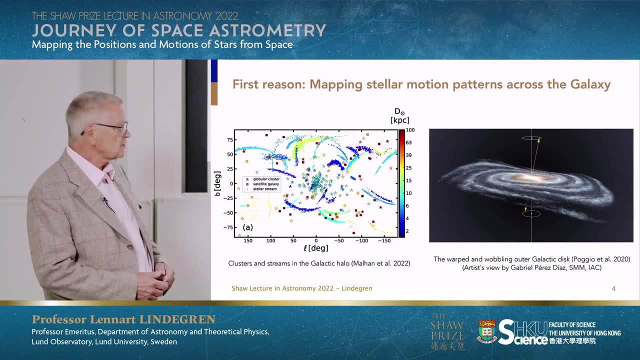 it means we have to measure these motions across the whole sky. That means global astrometry. These diagrams show two examples of why we want to map these global patterns. In the left diagram we have the clusters and streams in the outer part of the galaxy. 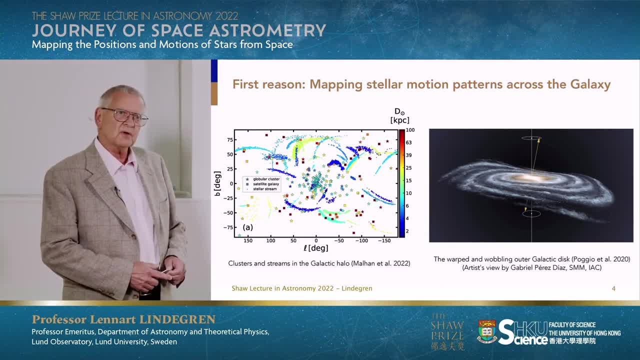 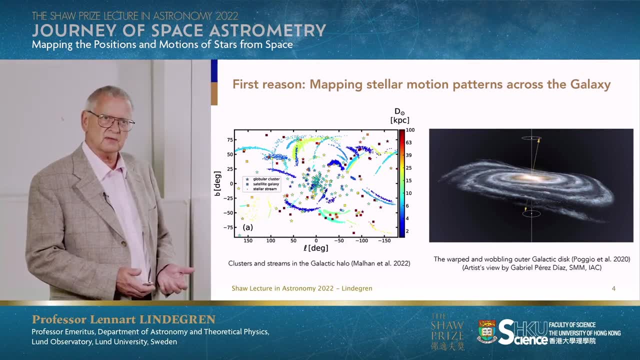 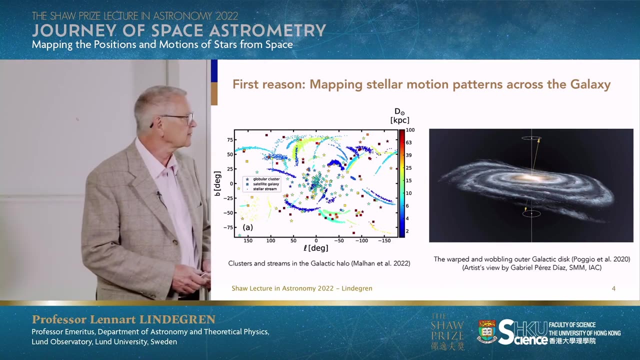 the halo, which tell us a lot about our galaxy. They make it possible to weigh the galaxy and tell us how much dark matter there is, for example, But they also tell us how the galaxy was assembled from the merging of many smaller galaxies. 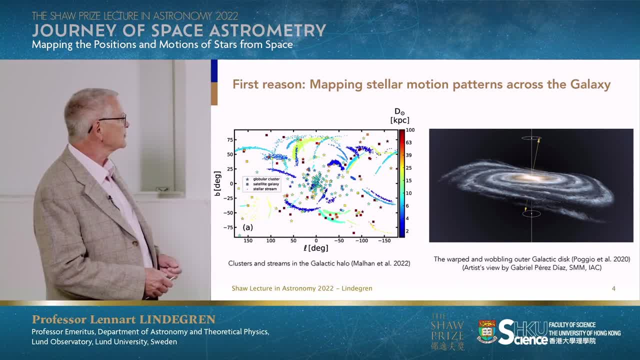 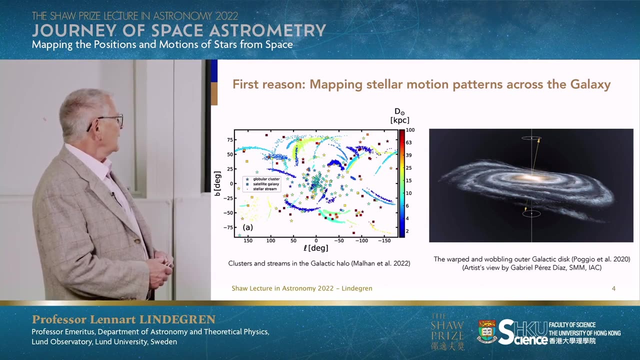 In the drawing to the right it is illustrated that our galaxy is not just a flat rotating disk. This disk is warped and it is processing in a complicated way, much like a spinning top, And this again tells us something about the dynamical history of the galaxy. 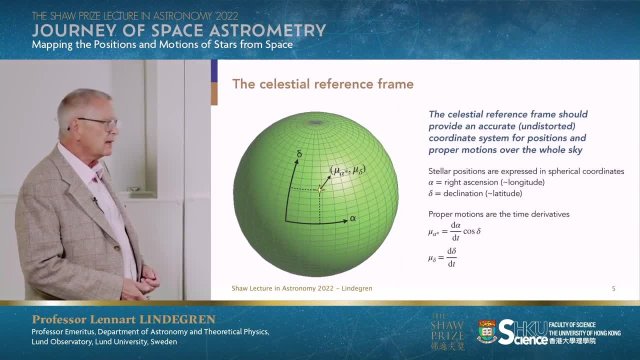 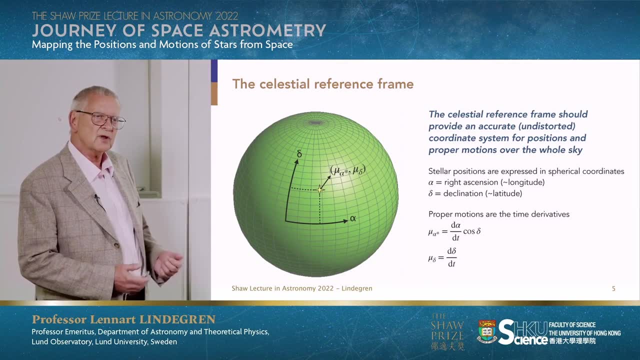 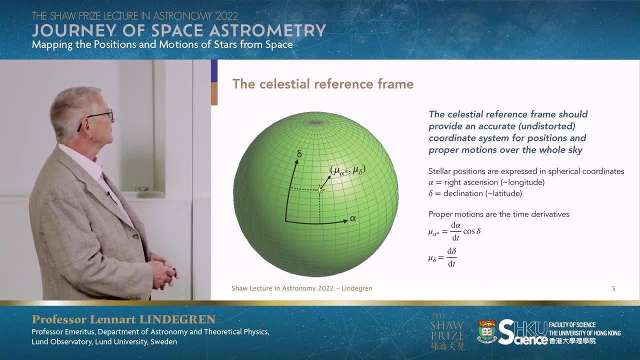 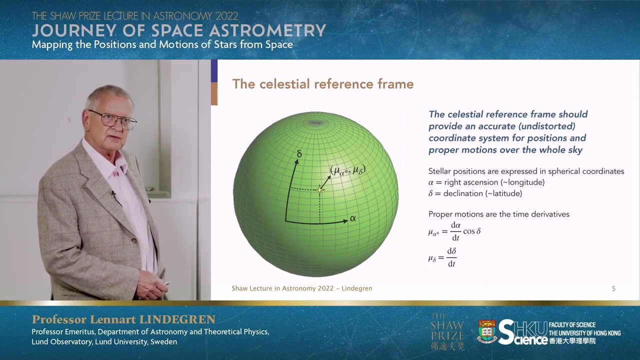 In more technical terms, what we need is a celestial reference frame that is very accurate, which means it has no distortions, So it provides a coordinate system for positions and proper motions over the whole sky. Stellar positions are normally expressed in spherical coordinates called right ascension and declination. 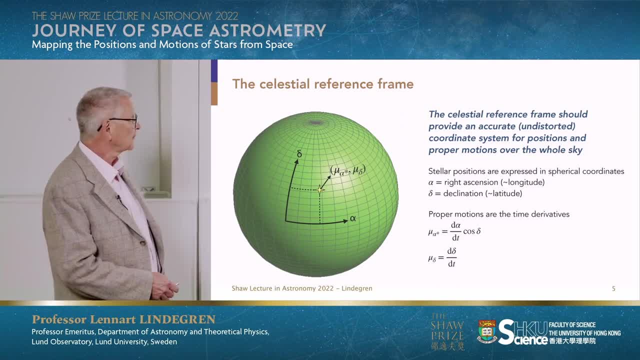 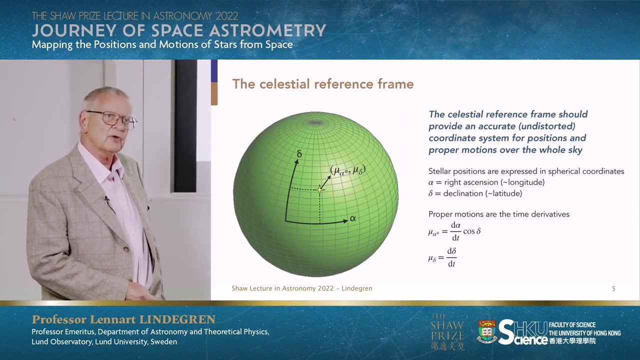 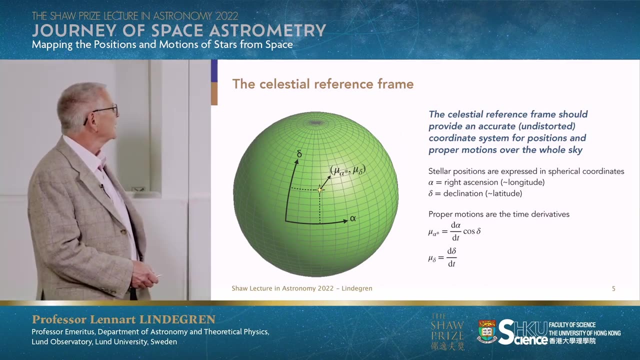 and denoted with the Greek letters alpha and delta. Proper motions are the time derivatives of these angles, And stars move so slowly that there is seldom any reason to use higher derivatives than the first derivative. The proper motions can be visualized as vectors on the celestial sphere. 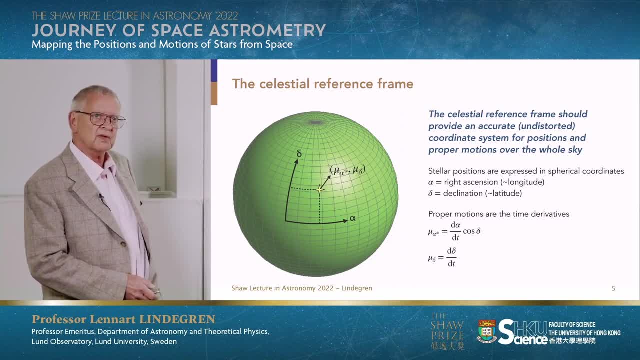 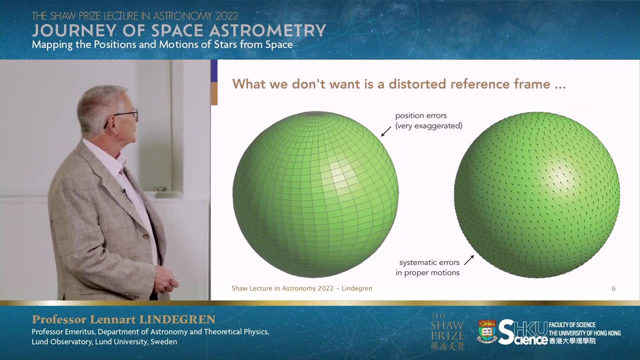 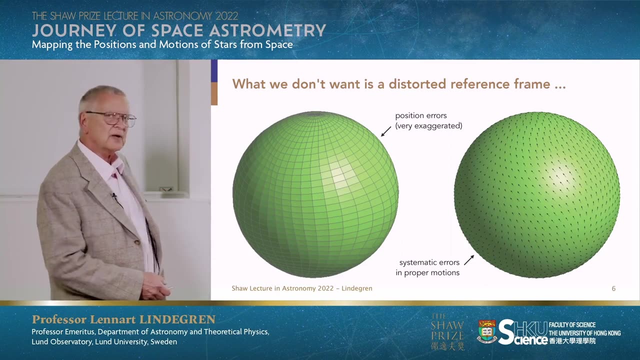 showing the motion of stars perpendicular to the line of sight. What we don't want is a distorted reference frame, That is, that the positions of the stars don't map a regular grid on the sky, but a distorted pattern, like illustrated in the left figure. 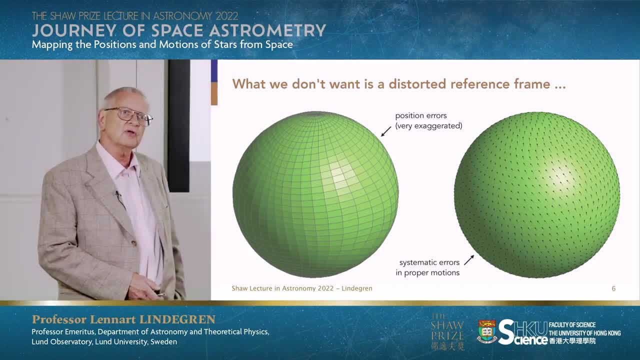 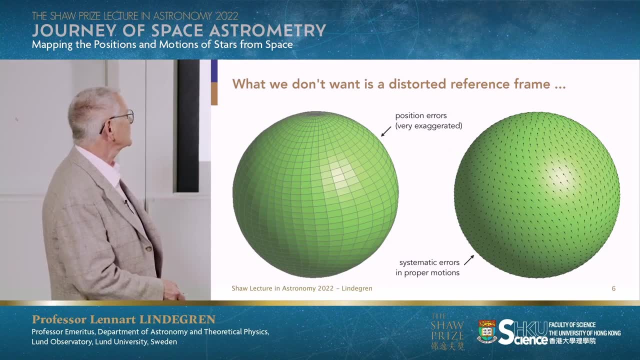 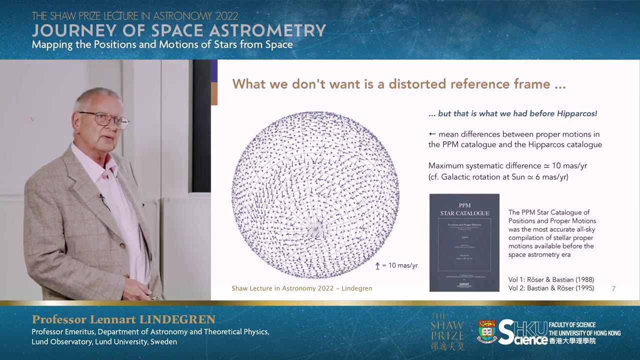 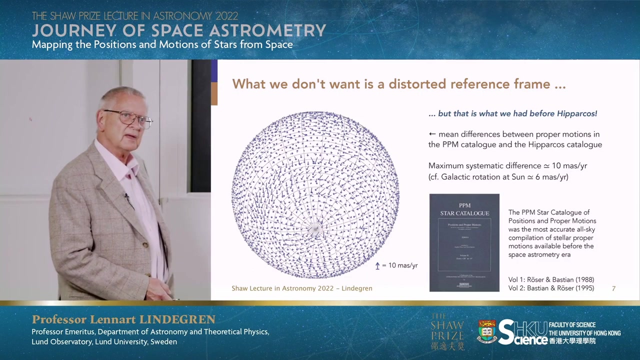 And similarly the proper motions should be undistorted, which means that they they don't make large-scale patterns in their errors. But that is not what we have in the data before Hipparchus. This diagram here shows the systematic errors in proper motions. 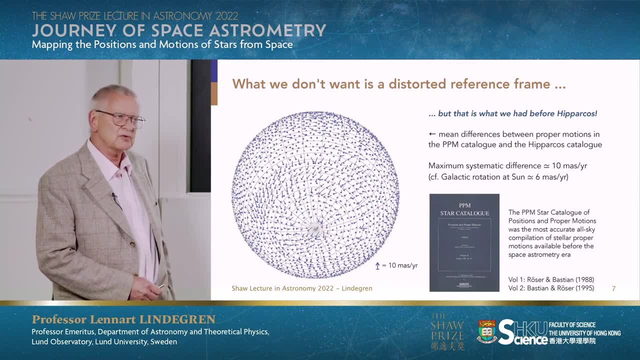 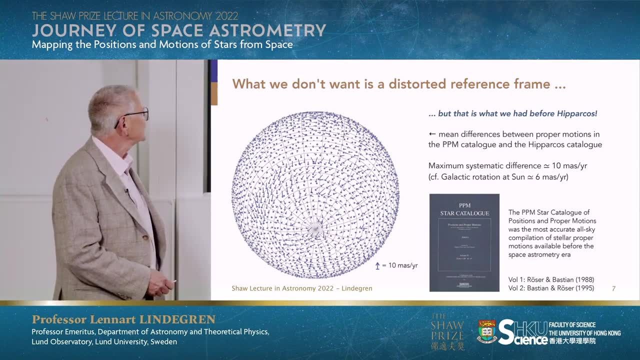 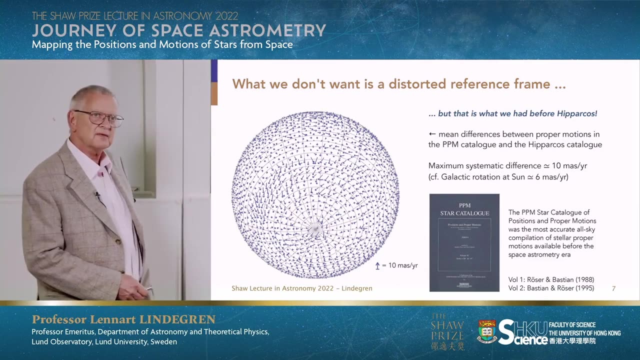 in the best compilation of stellar proper motions before Hipparchus: the PPM catalog. What you can see from this vector plot is that in some areas, in some parts of the sky, the errors are rather small, but in others they are as much as 10 ms per year. 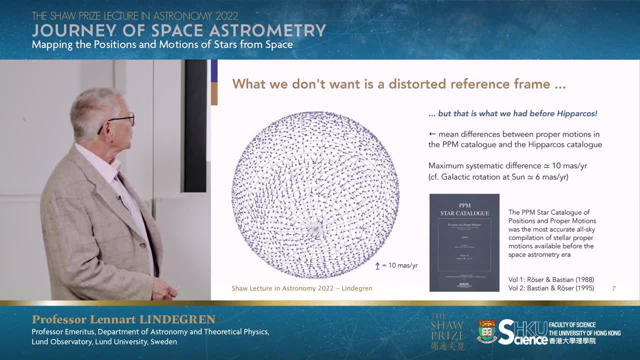 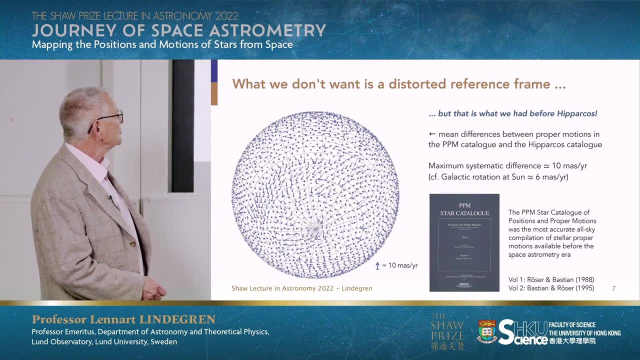 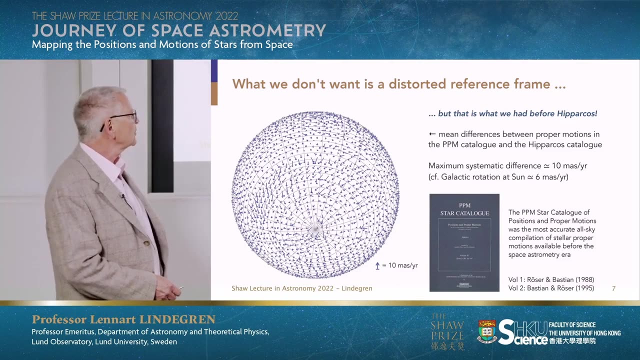 This is not a big, proper motion, but it is large compared to the patterns that we want to measure. For example, the galactic rotation itself around the galactic center, as seen from the Sun, is only about 6 ms per year. 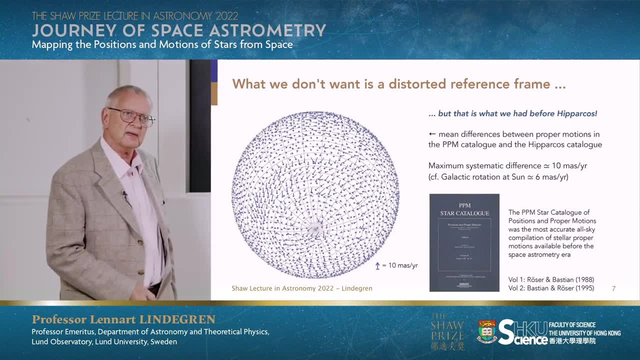 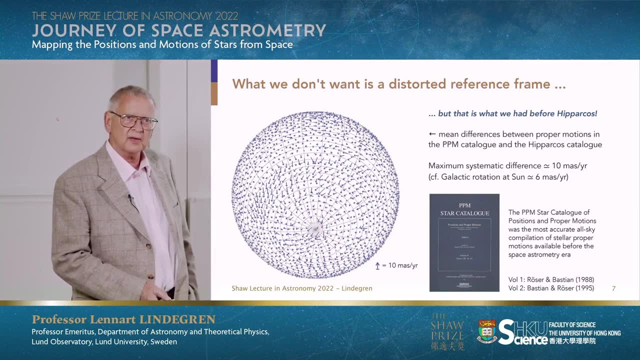 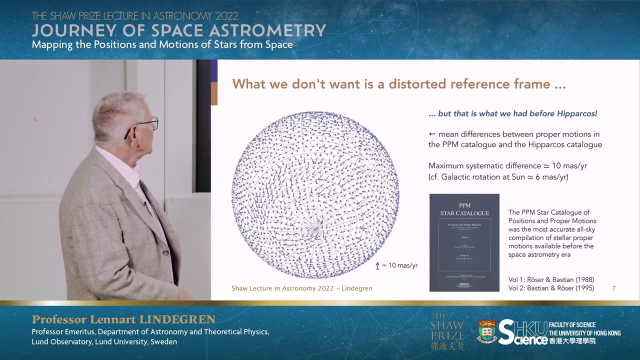 And it's clear that if we have this kind of systematic errors in our proper motions, we would not be able to see the much more subtle patterns corresponding to the Haller streams or the precessing warp I talked about before. So with these kind of errors, 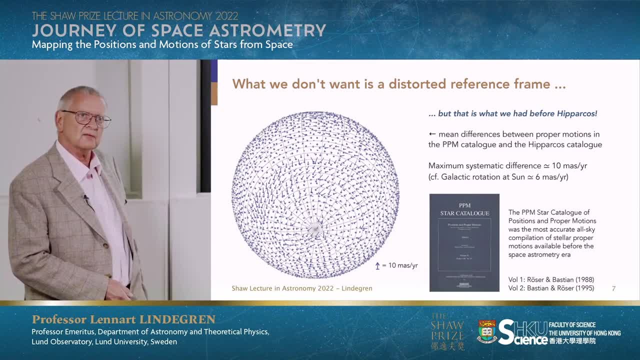 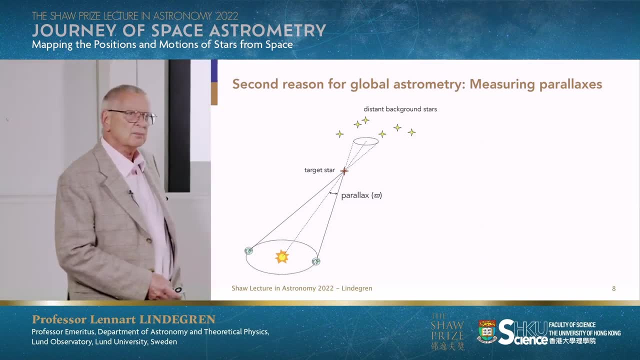 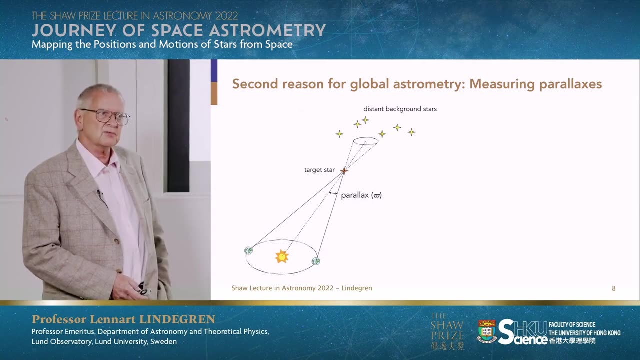 systematic errors in the proper motions, we could not do that kind of science. The other reason why we need global astrometry is in order to measure parallaxes. This could come as a surprise to you, perhaps, since it is well known that. 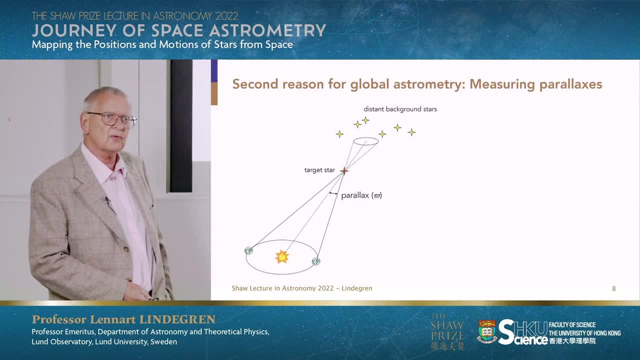 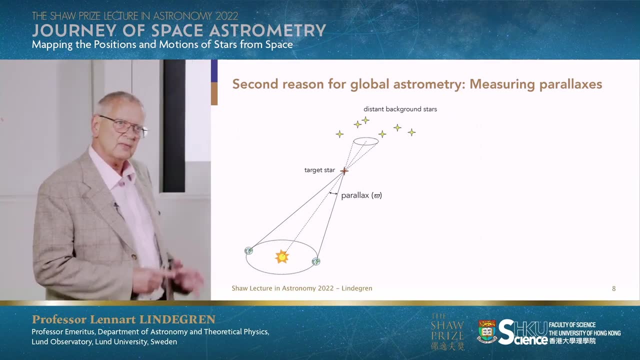 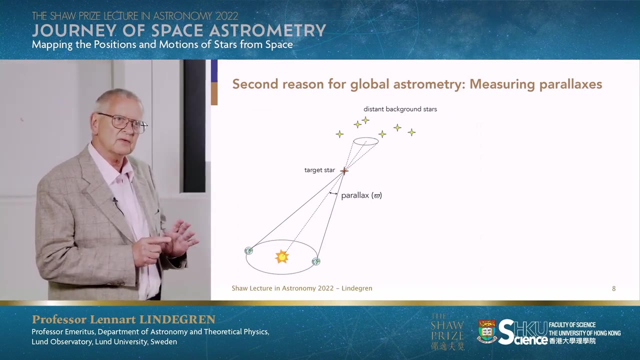 we have been able to measure parallaxes from the ground for almost 200 years with quite a lot of success, But these parallaxes were always measured within the field of view of a big telescope, which means that we only measured angles between stars that were. 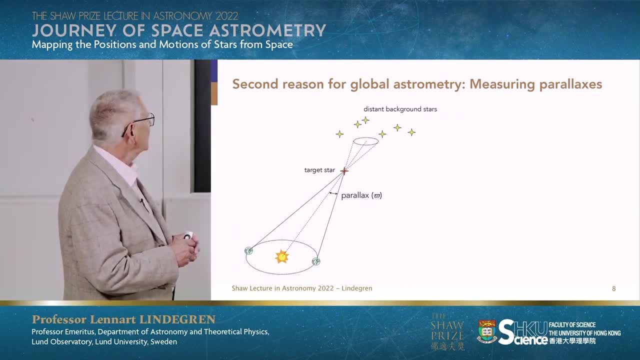 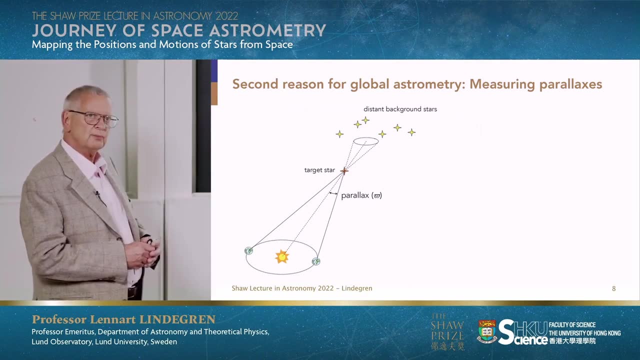 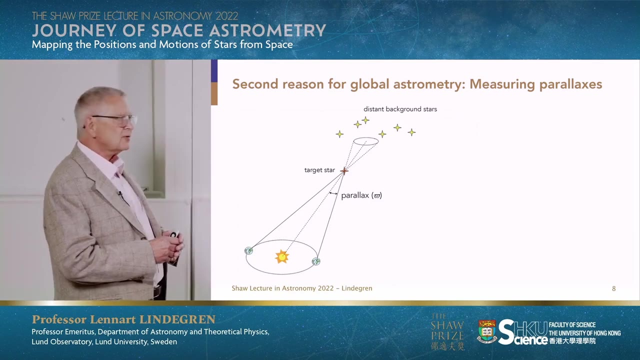 very close to each other. on the sky, Parallax is usually described by means of a diagram like that to the left. So as the Earth moves around the Sun over the year, a nearby star, the target star imaged here, appears to move in a small ellipse. 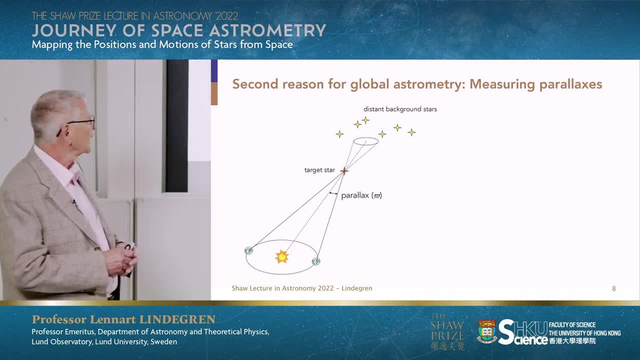 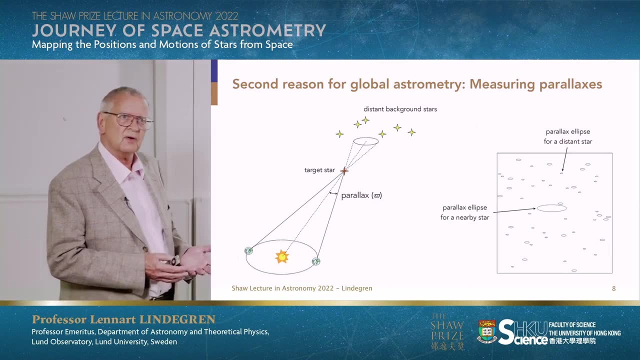 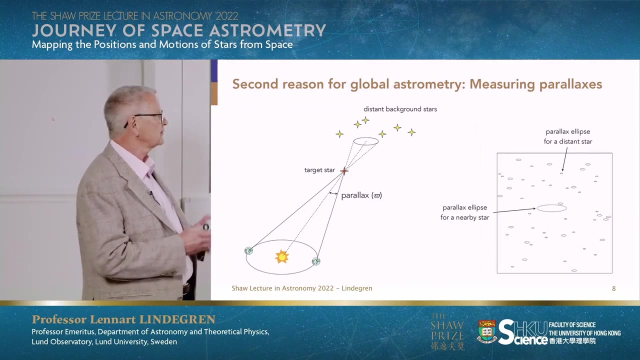 compared to the background stars. This is the parallax ellipse. This parallax ellipse is actually the mirror image of the Earth's motion around the Sun as seen from the star, And the more distant the star is, the smaller this ellipse is. But even the background stars are not at infinite distance, which means that they too have a parallax. They also move in small ellipses, And when we do measurements in a small field, like we have to do from the ground, then we will not see the whole parallax. 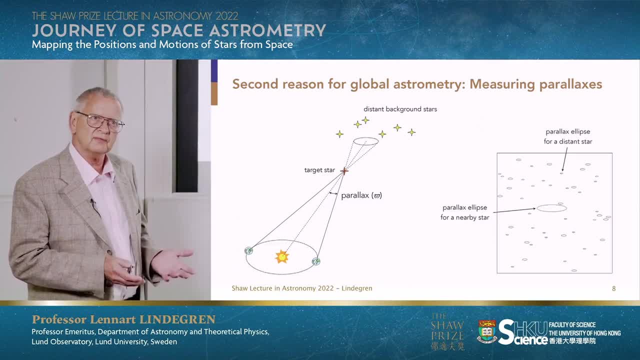 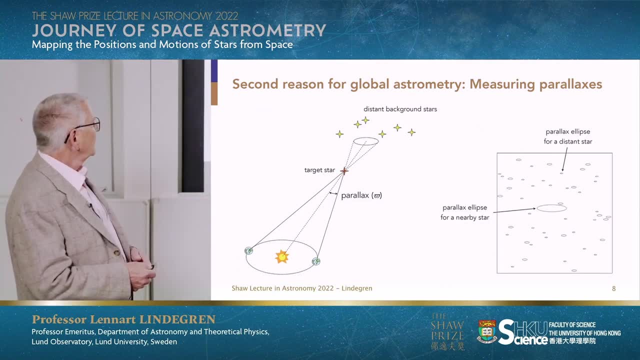 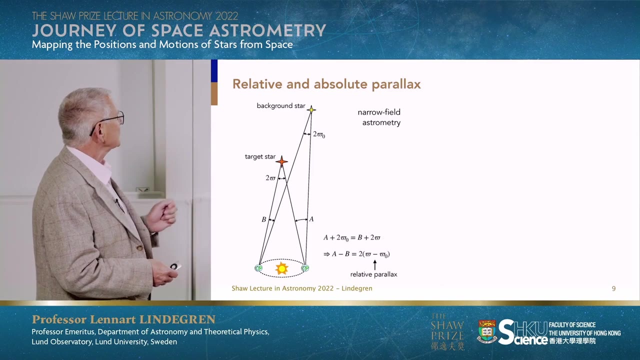 of this nearby target star, We will only see the difference in parallax between its parallax and the mean parallax of the background stars. This diagram illustrates the same thing in a slightly different way. We can see here that by measuring the angles A and B 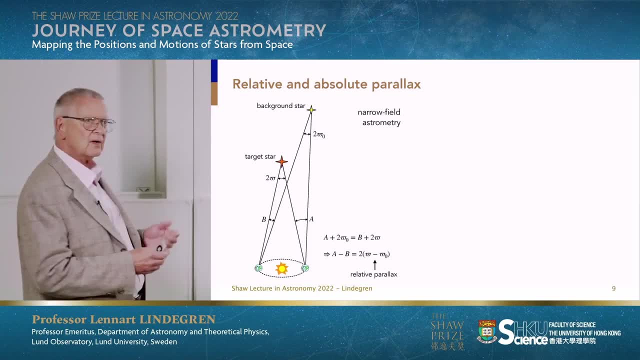 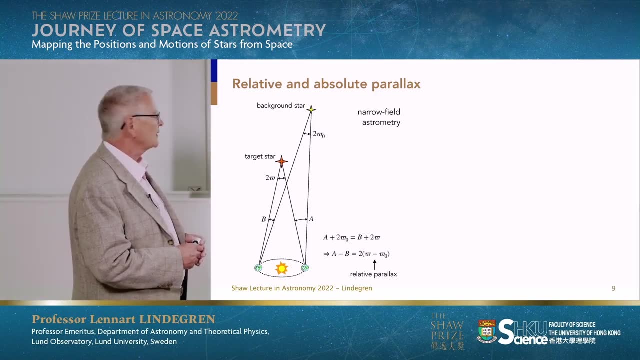 which are small angles on the sky between the target star and the background star. by taking the difference between these two angles, A minus B, what we get is twice the difference in parallax between the two stars, And that is what I call the relative parallax. 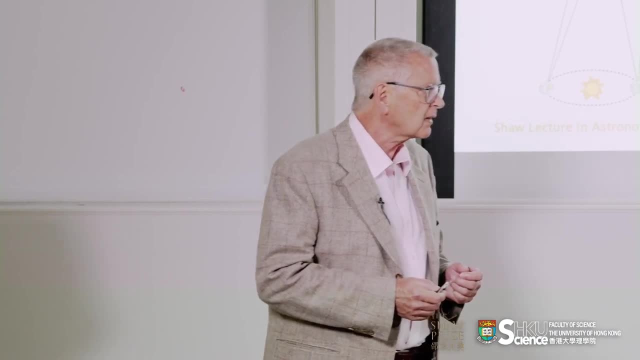 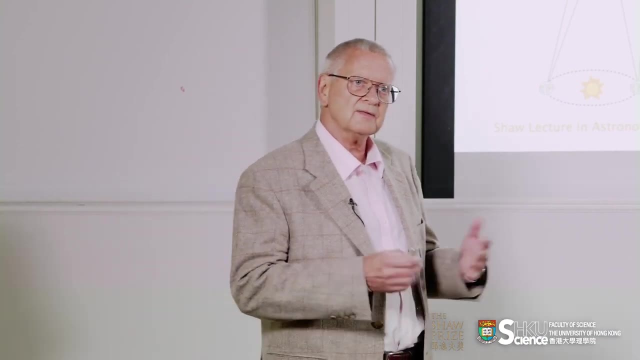 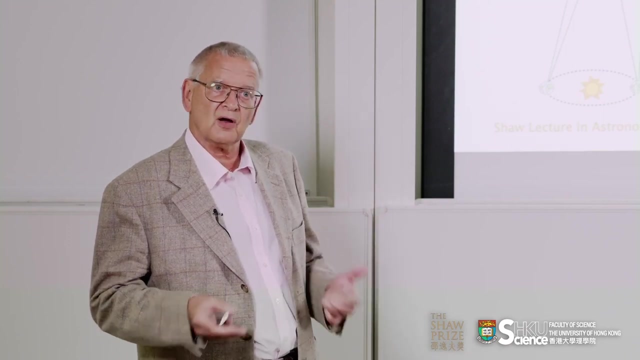 This is OK as long as we are only looking at some of the most nearby stars to our solar system, But if we want to map stellar distances throughout our galaxy, this method will not work anymore, simply because most of the stars are background stars. 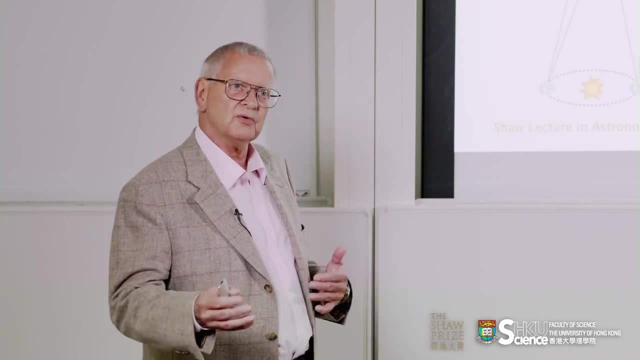 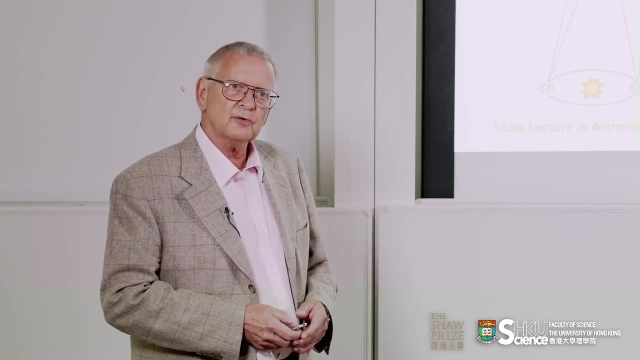 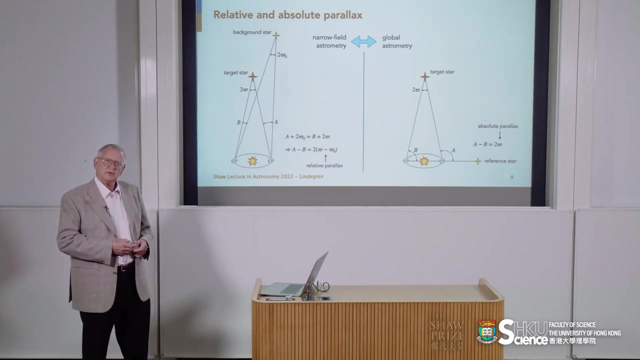 They are at such great distances that there are no more stars sufficiently further away that they can be used as a background. So the solution to this problem is, again, global astrometry. With global astrometry we can measure not only small angles on the sky. 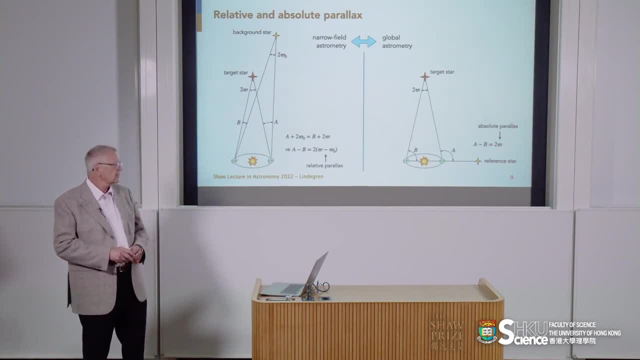 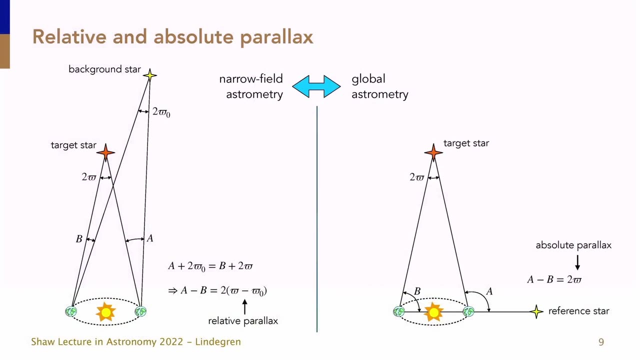 but also large angles of the order of 90 degrees. So suppose we measure the angle between the target star and the reference star about 90 degrees away from it, at two different times when the Earth is in opposite points in its orbit around the Sun. 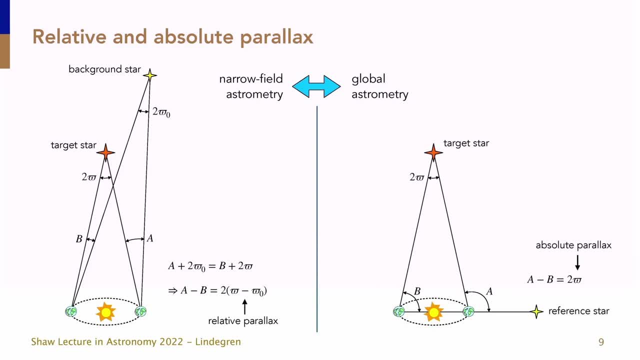 Then, by taking the difference between these two angles, we get twice the parallax of the target star, And this result is independent of the distance to the reference star. We can even have a reference star that is not at all in the background. 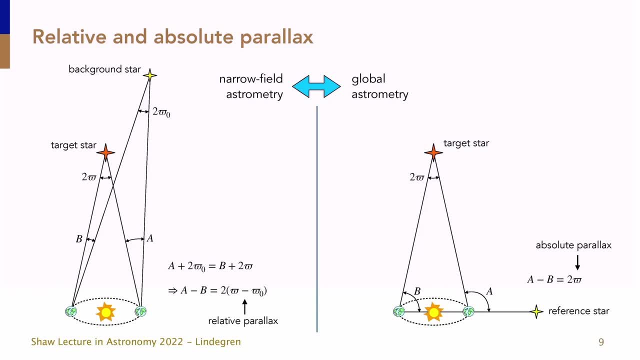 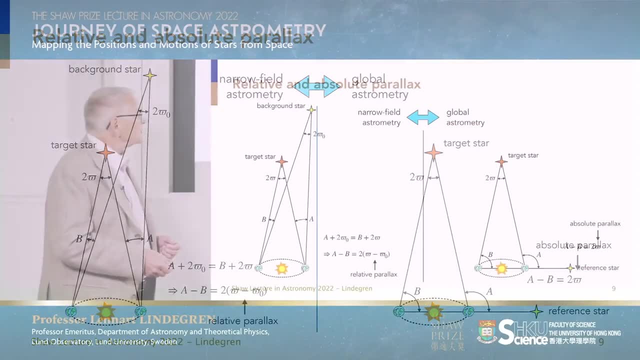 but even closer to us than the target star. In this way we get absolute parallaxes, But it requires to measure large angles of the order of 90 degrees. So now I have given you some good reasons why we need global astrometry. 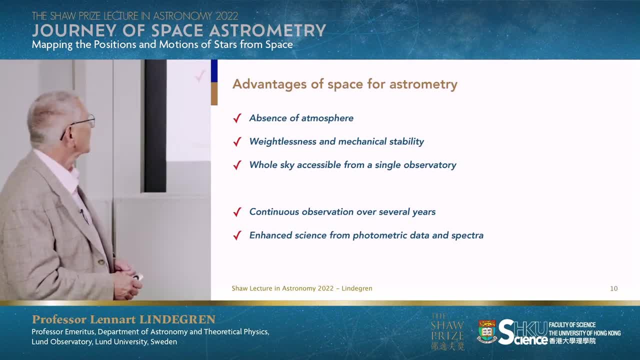 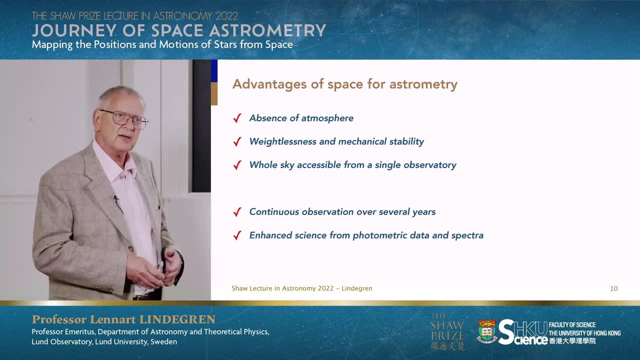 Now I have to tell you why we do it from space. Space offers some very important advantages for astrometry, and especially for global astrometry. First of all, we have the absence of atmosphere, which means that the images of stars are very sharp. 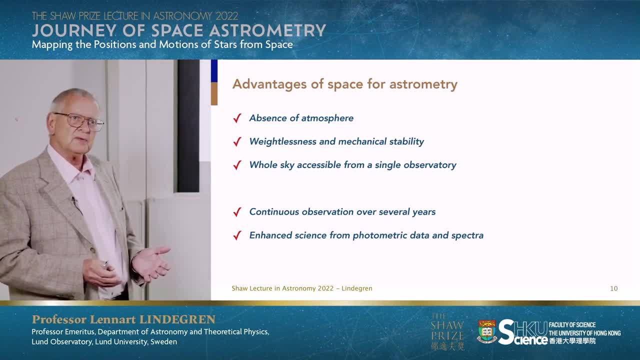 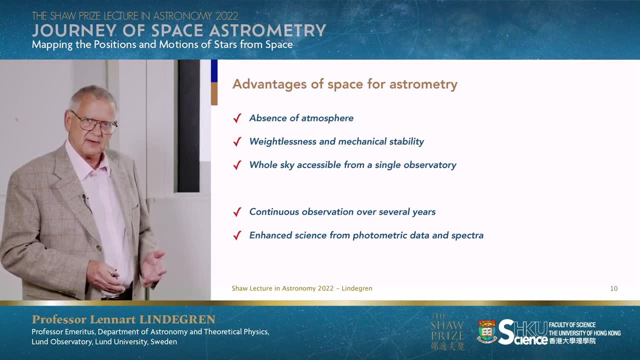 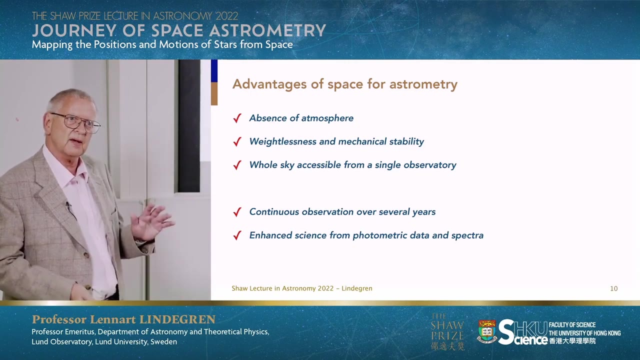 and stable, and we don't have a refraction in the atmosphere that changes their directions. We also have weightlessness, which means that we can turn the instrument in different directions without it being distorted by gravity, And we also have a stable thermal environment in space. 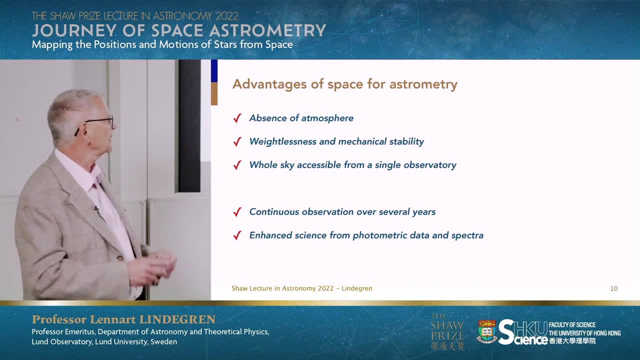 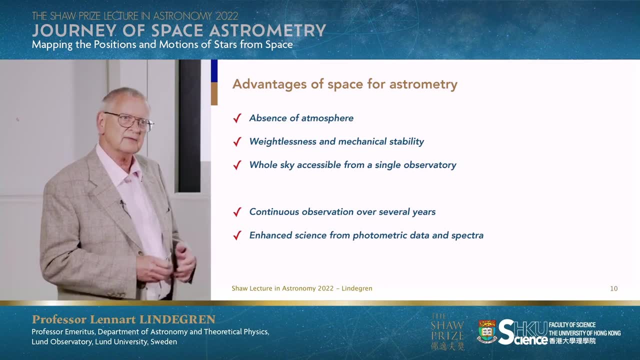 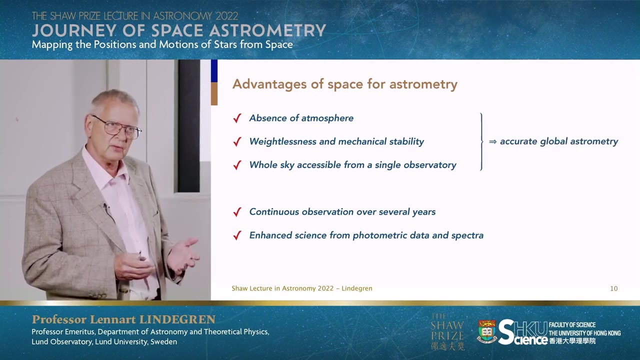 which means that we can also have mechanical stability in the instrument. And the final point, which is very important for global astrometry, is that we can access the whole sky from a single point, from a single instrument. These three points together means that we can do accurate. 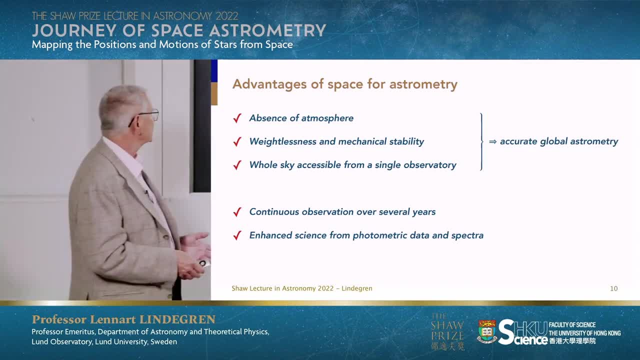 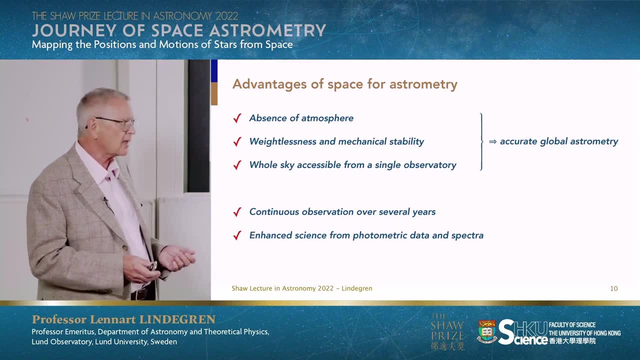 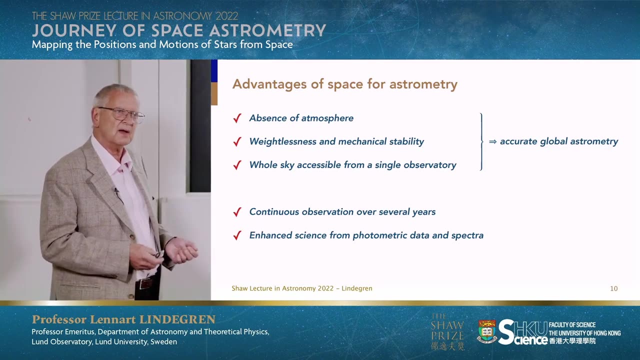 global astrometry from space. There are other advantages as well from observing from space, For example, that we can observe more or less continuously, 24 hours per day over several years, And we can also collect additional data like photometry and spectra. 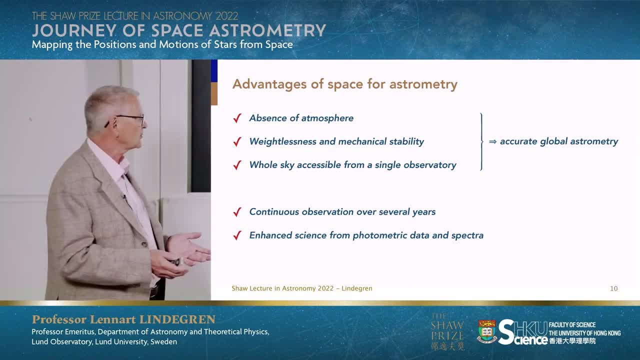 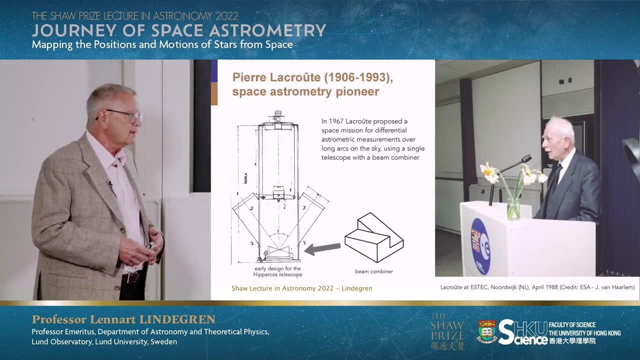 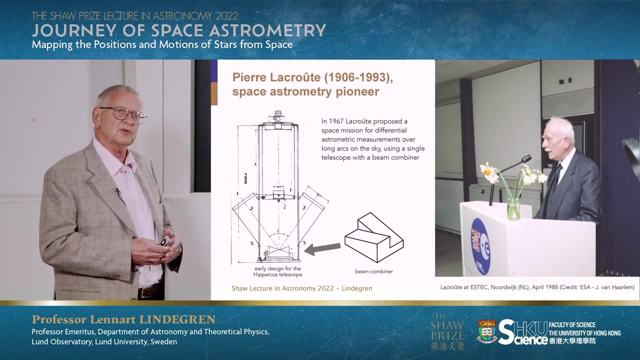 that are extremely useful for the astrophysics, and we get them almost for free. The idea to use space for astrometry was first put forward by the French astrometrist Pierre Lacoute In 1967. he proposed a space telescope. 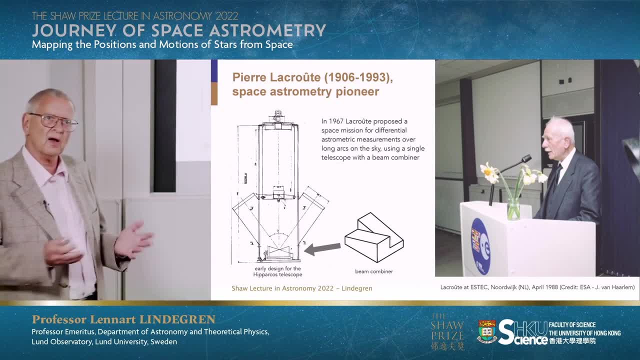 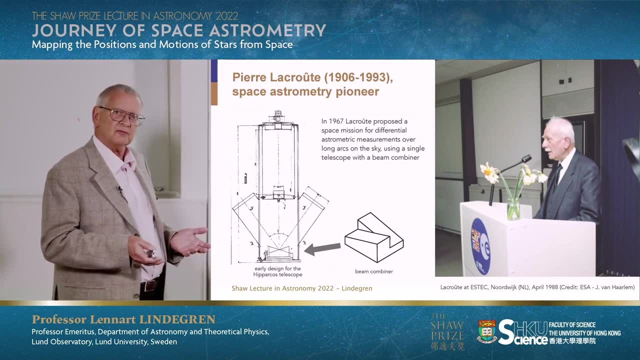 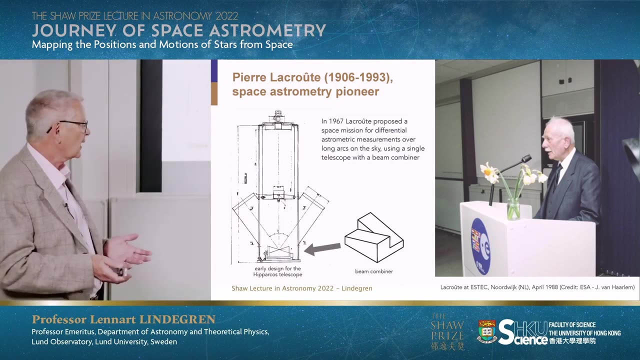 that was able to do differential measurements over long arcs on the sky using a single telescope and a beam combiner in front of it. This beam combiner makes it possible for the telescope to look simultaneously in two different directions, And that enables us to do 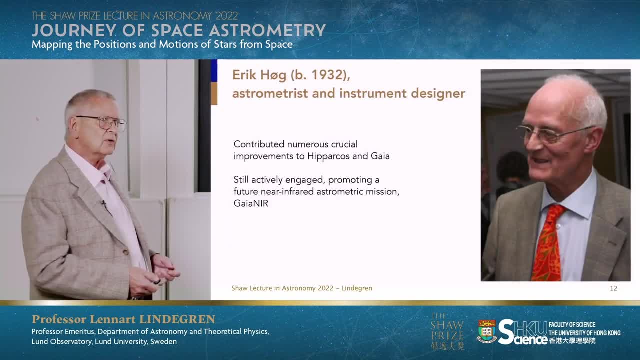 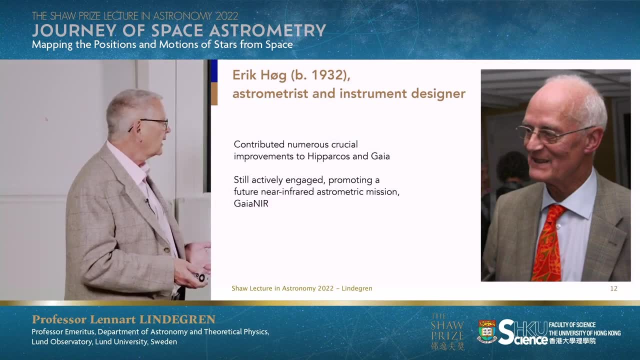 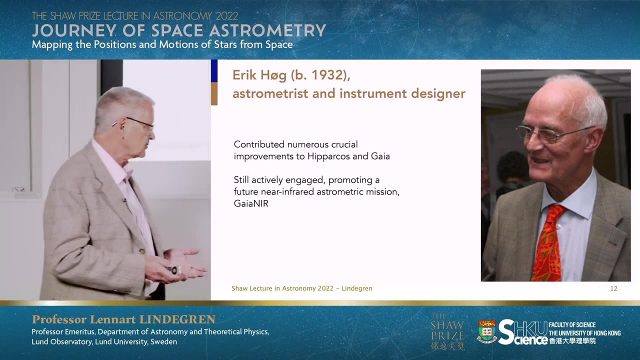 large angle measurements. It took more than 20 years for this idea to be realized, before Hipparchus was launched, And this development was the result of many people contributing to this mission. I will mention only one of them, the Danish astronomer Erik Hoeg. 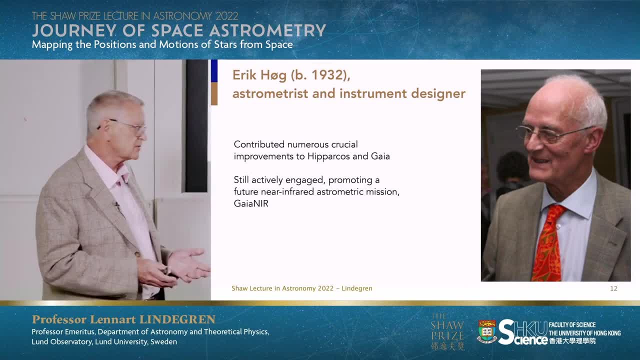 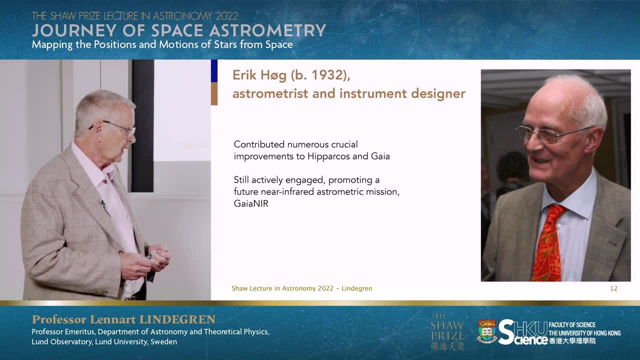 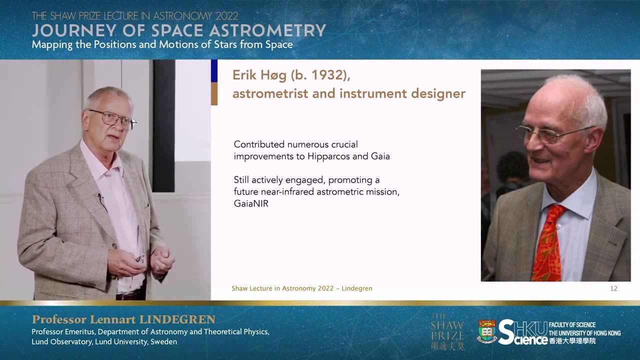 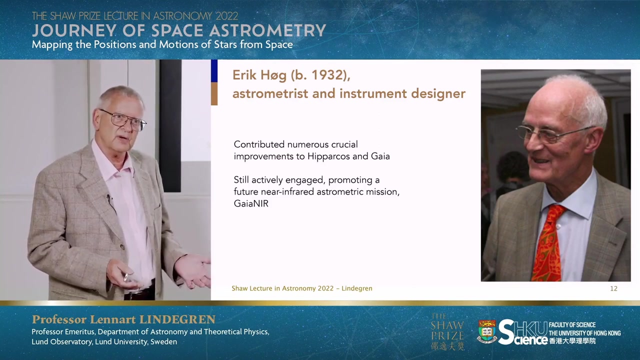 who contributed many crucial improvements to the original ideas, First to Hipparchus and then also to the Gaia project. It was the dedicated work over many years by people like Erik Hoeg that transformed Lacoute's vision into a real mission, or actually two missions. 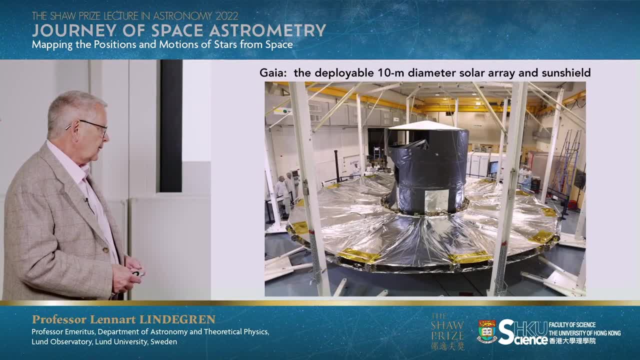 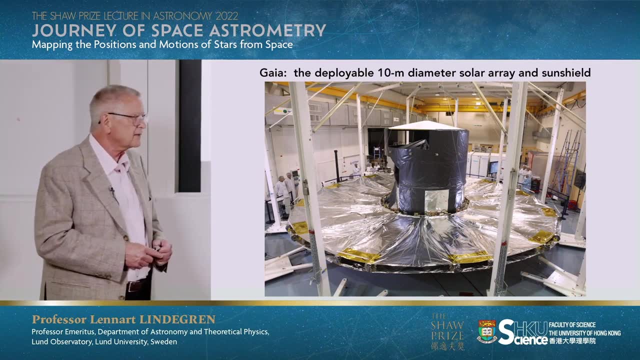 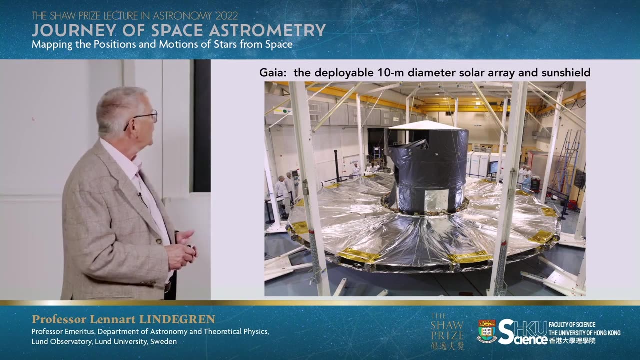 Hipparchus and Gaia. Now let's take a look how this actually works in Gaia. This picture shows the Gaia satellite shortly before launch, when the deployable sunshield was tested. Inside the central hut there is the instrument: the payload. 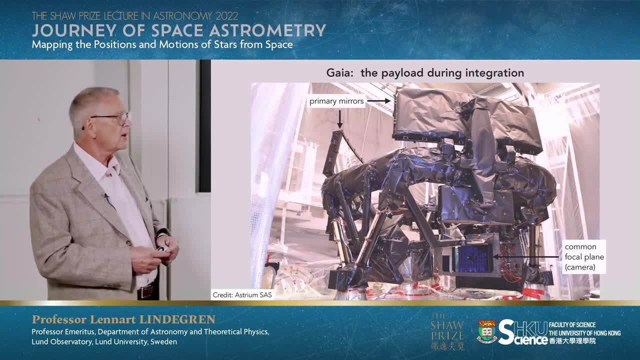 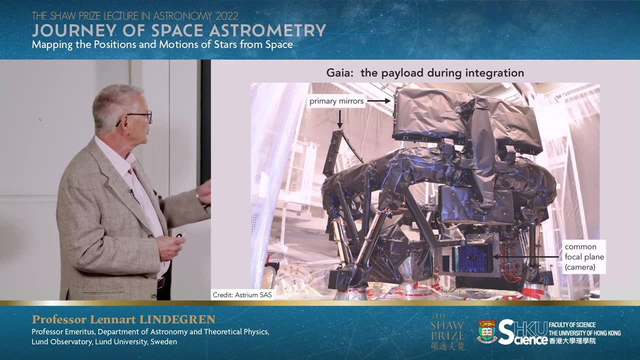 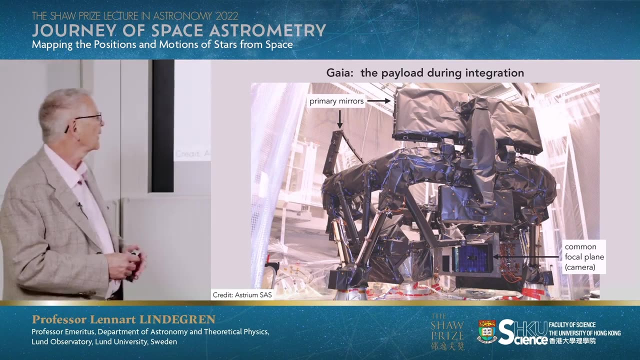 which is shown in this picture during integration. In the top part of the picture you see the two primary mirrors that look in two directions, And at the bottom right you see the focal plane for the two mirrors, or the camera, if you like. 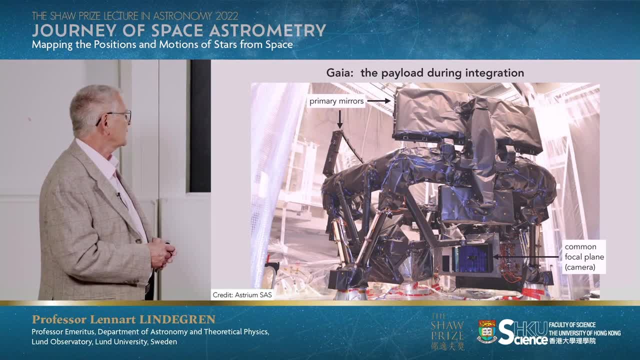 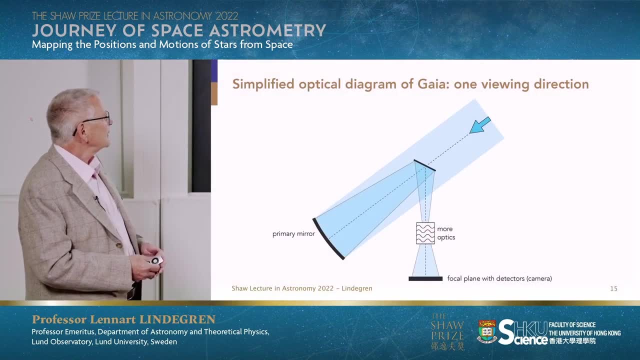 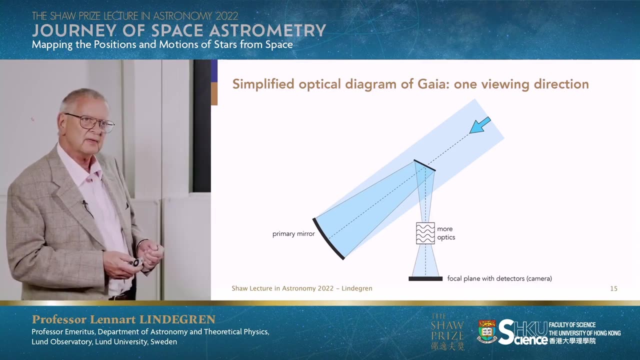 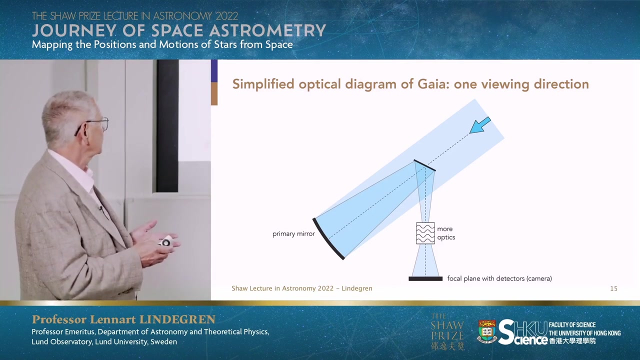 consisting of more than a hundred CCVs covering almost one square meter. This is how the telescope works. Light from one direction is collected by one of the primary mirrors and is then reflected by a flat mirror into some additional optics and onto the camera. Light from the other direction. 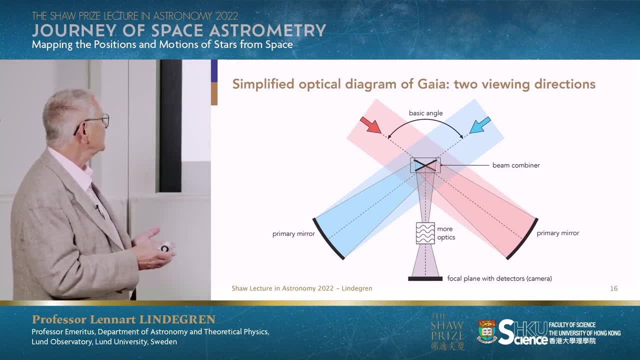 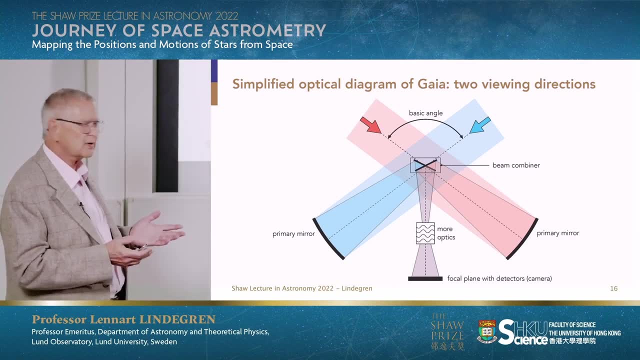 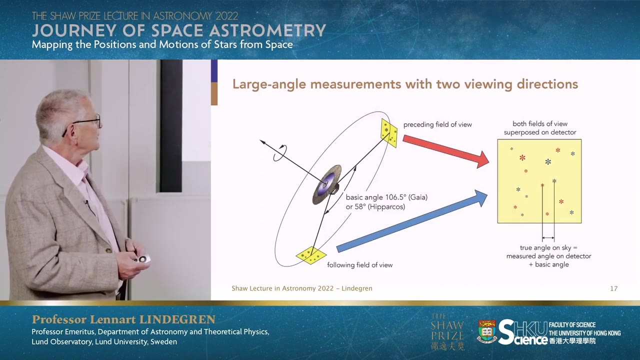 goes to the other primary mirror and is then reflected to the same focal plane, the same detectors. This means that the telescope can simultaneously look in two directions, separated by a large angle called the basic angle. The overall effect is that the satellite Gaia 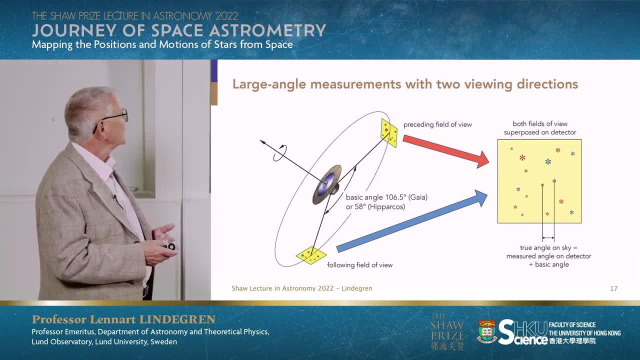 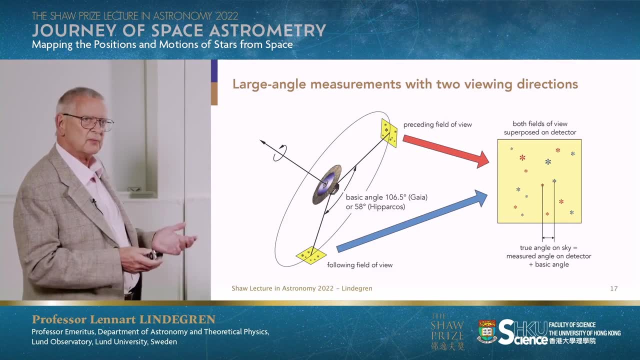 can look in two different directions on the sky at the same time, With some stars coming from the same field of view, here called the preceding field of view, and some stars from the other field, the following field of view, But they are all seen on the same detectors. 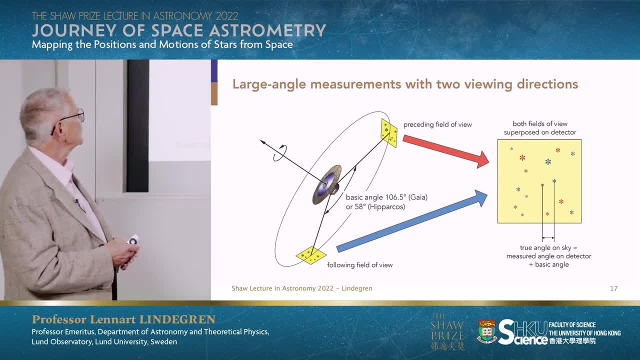 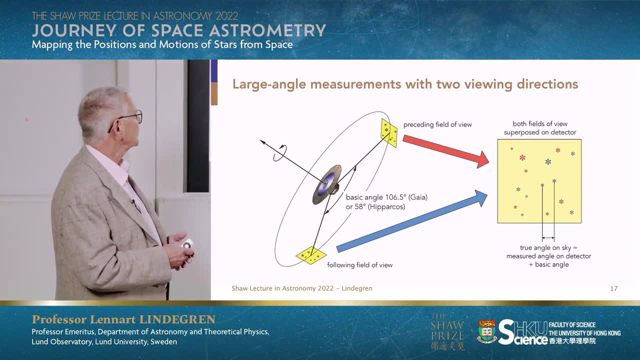 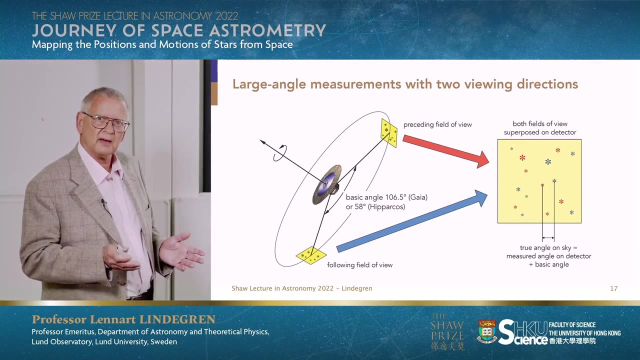 In the image to the right the stars coming from the preceding field of view are shown in red and in blue are shown the stars coming from the other field of view. On the detector you can measure the angle between these images, But to get the true angle on the sky 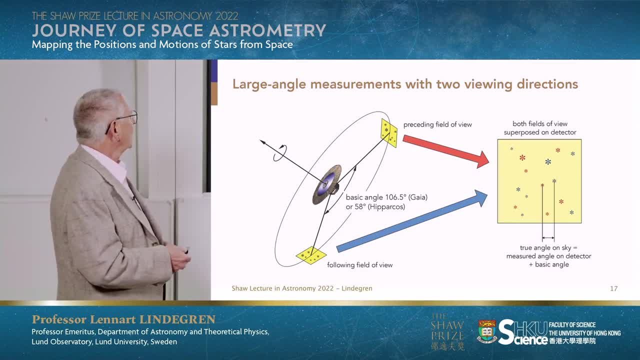 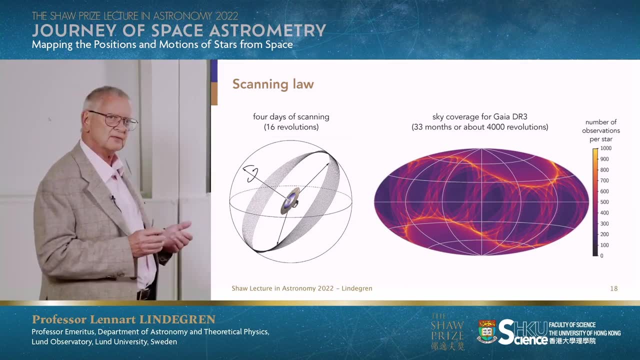 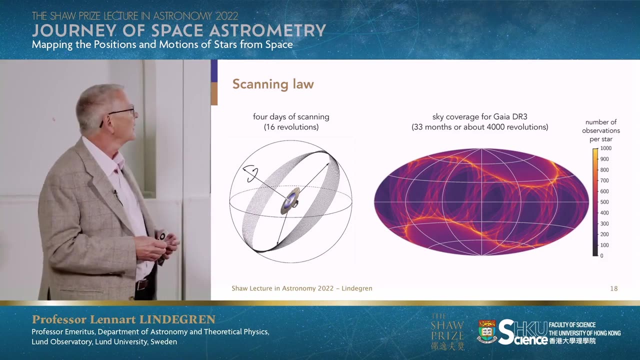 you have to add the basic angle. The satellite is slowly rotating around its axis, which means that the two fields of view sweep roughly along a great circle on the sky in six hours. But the rotation axis is not fixed in space but is slowly changing. 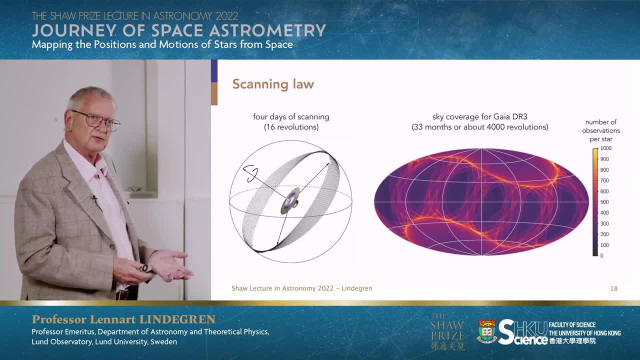 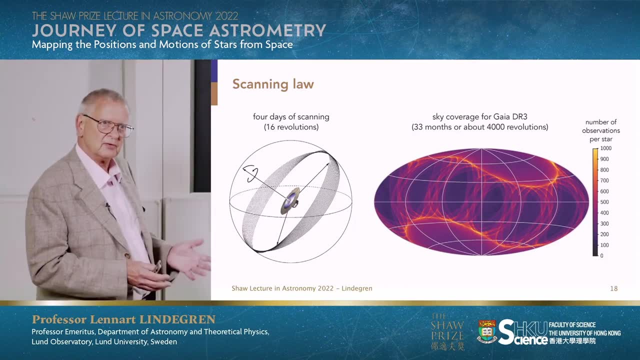 its direction, which means that a successively larger part of the sky is covered by the two fields of view, And after a few months you can see that the two fields of view have covered all the sky, And this is then repeated many times over the years. 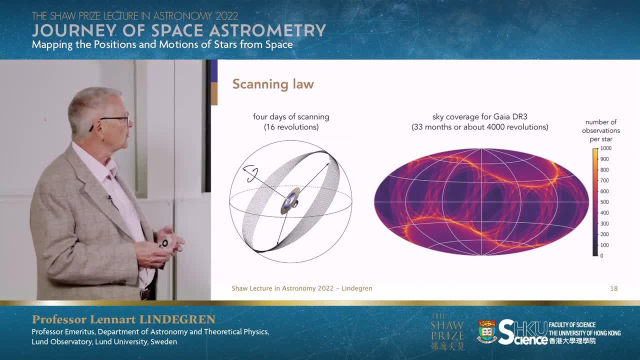 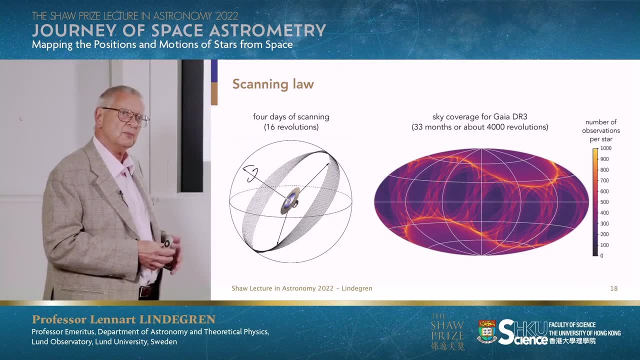 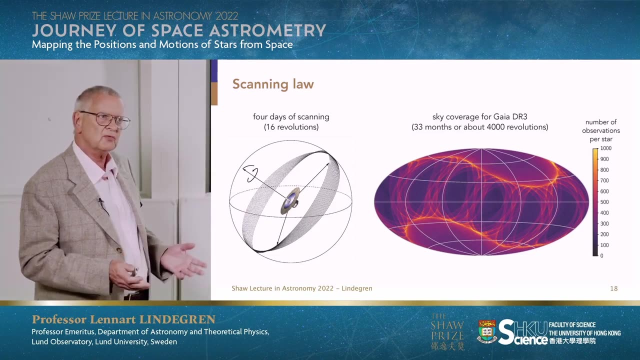 The diagram to the right shows the number of observations obtained at each point on the sky after nearly three years of observations, namely the observations that were used for the third release of Gaia data, Gaia DR3.. You can see that the number of 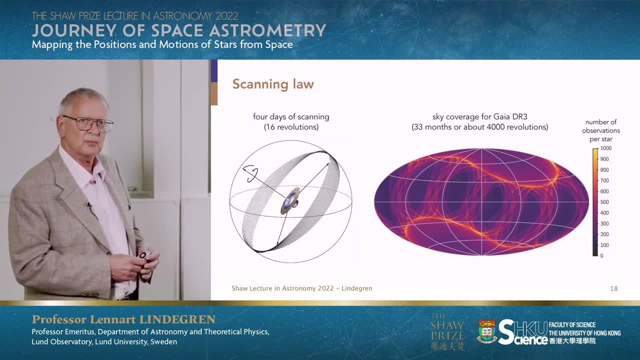 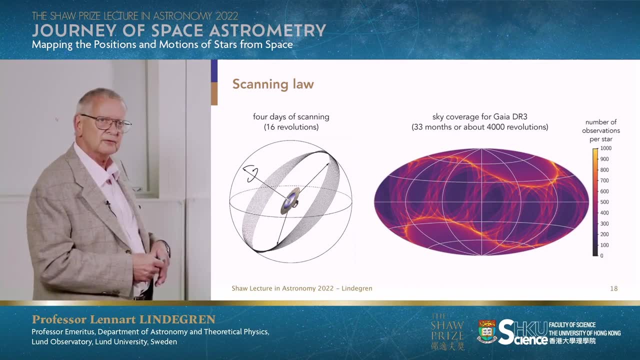 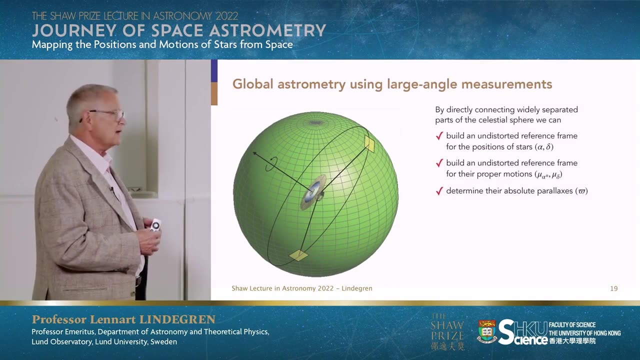 observations per point on the sky varies from a few hundred up to about a thousand. This is the so-called scanning law, for Gaia and Hipparchos used a very similar scanning law. Now I will try to explain how this makes it possible to do global. 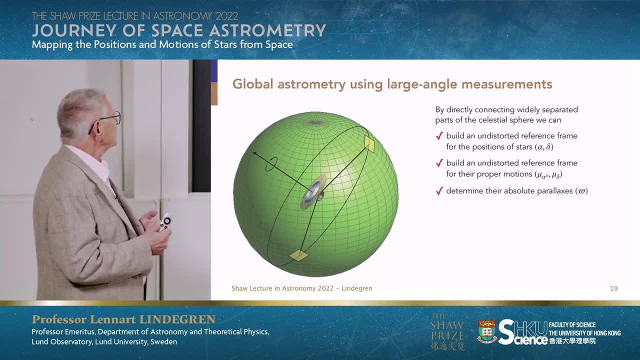 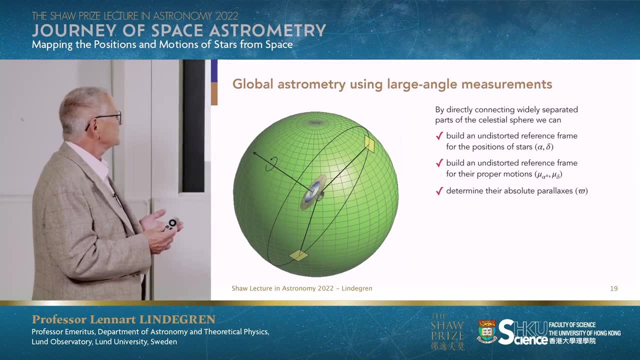 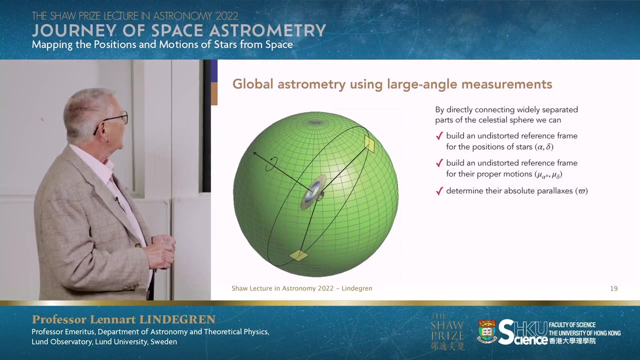 astrometry. The point is that we want to construct a celestial reference frame that is undistorted, as I mentioned before. If it is undistorted, there will be errors in the two fields of view that are not the same at all the time. 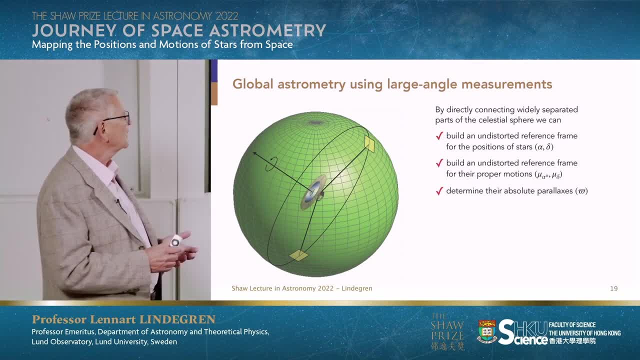 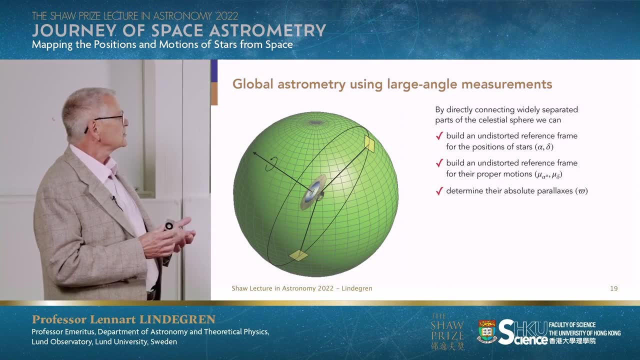 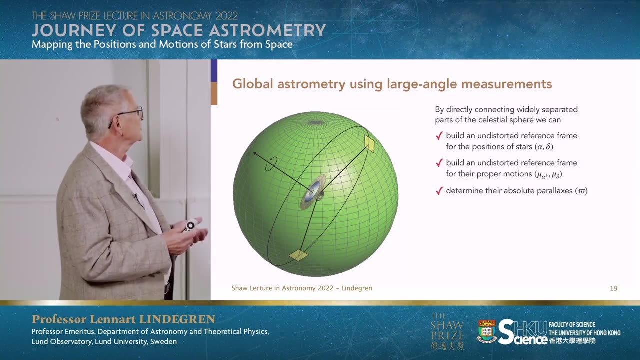 These differences can be measured by the satellite, and that makes it possible to construct an undistorted reference frame. We obtain this reference frame for the positions, but in a similar way also for the proper motions. we get an undistorted reference frame At the same time. 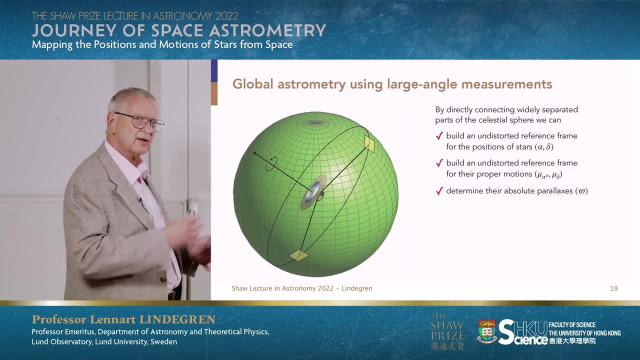 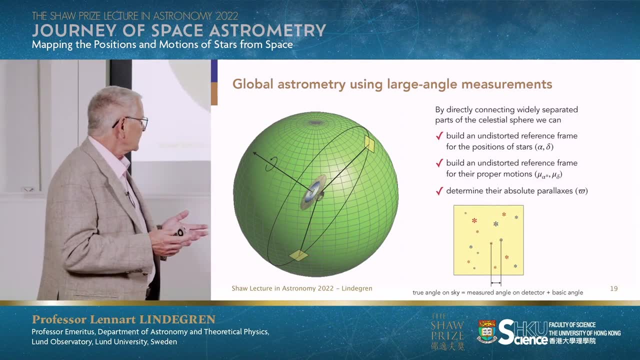 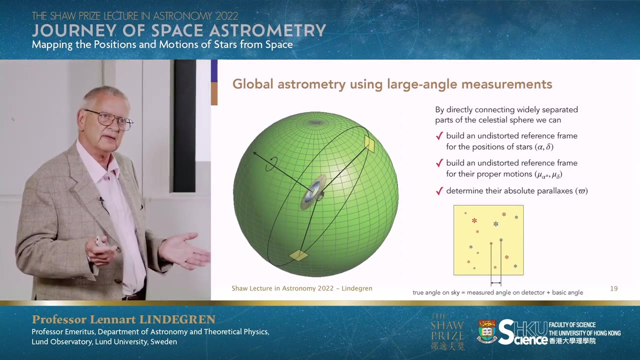 we can also determine the parallaxes using the large angles between the stars. But there is one problem, of course. As I said before, to get the true angle on the sky you have to take the angle that is measured on the detectors and add the basic angle. 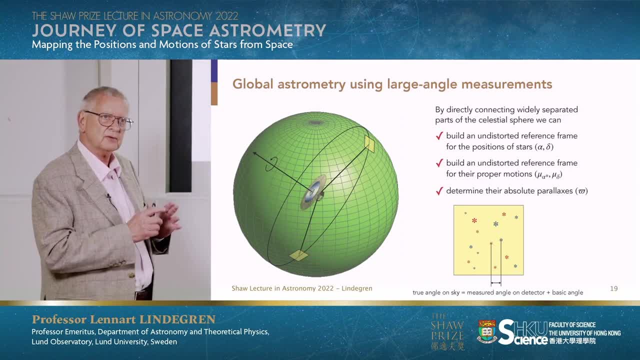 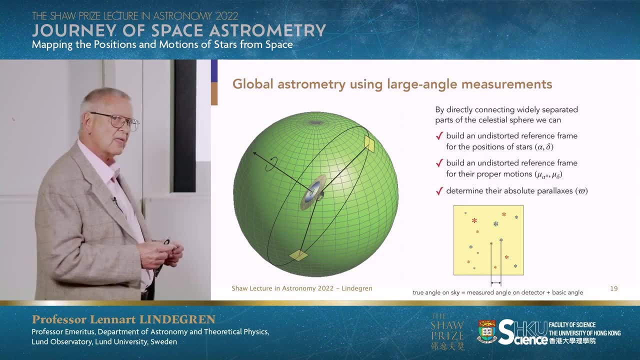 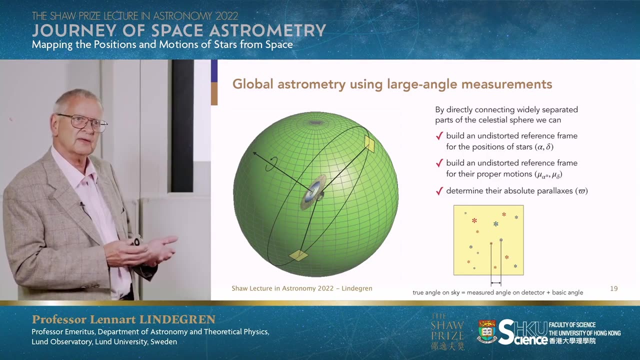 So how can we know the basic angle? We need to know it to the same precision that we aim for in the final astrometric data, that is, micro-arctosecond precision, And no device on board the satellite is able to measure this basic angle to that kind of. 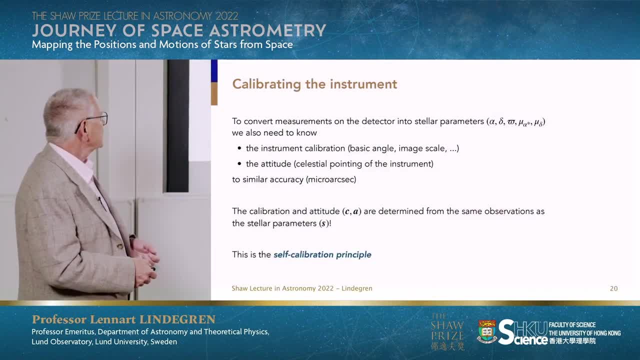 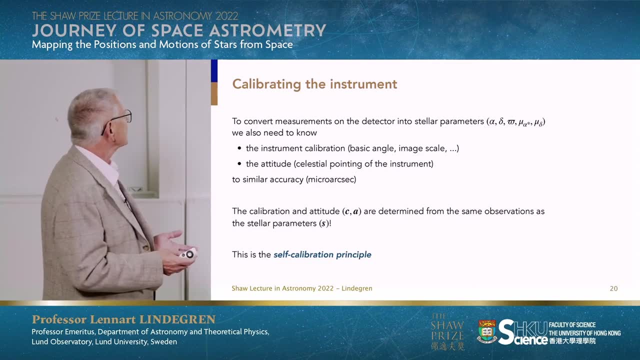 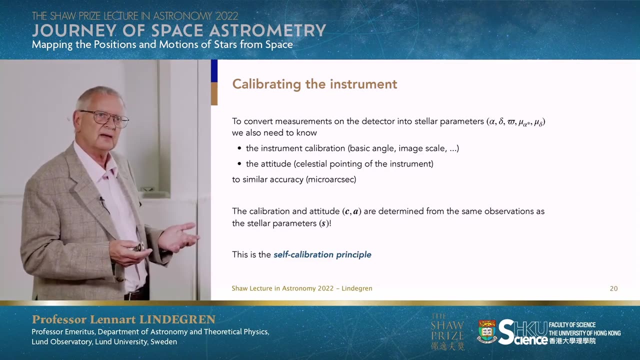 precision. So the answer to that is something called the self-calibration. We need to calibrate the instrument, like the basic angle, image scale and so on, but we also need to know exactly where it is pointing on the sky at each point in time. 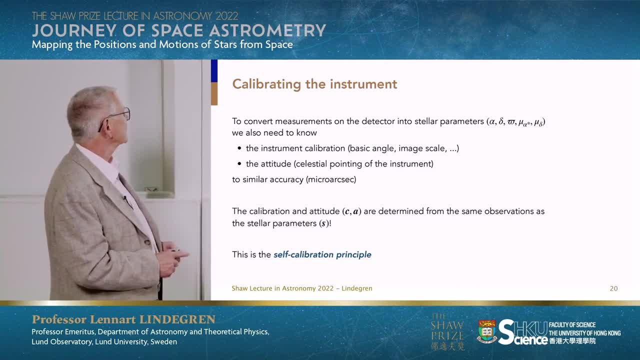 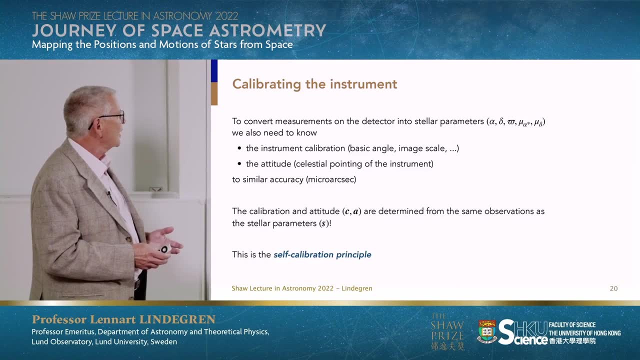 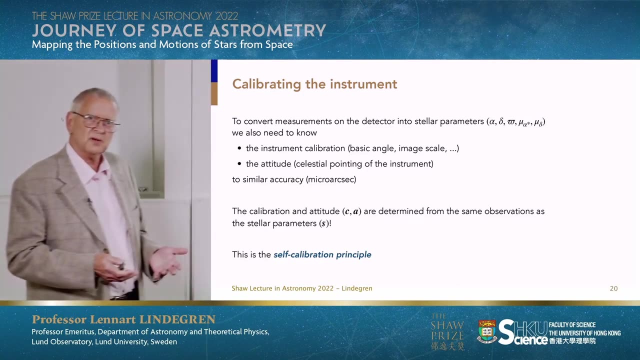 And all of this has to be done to similar accuracy, to micro-arctosecond accuracy. Self-calibration means that the calibration and attitude parameters are determined from the same observations as are collected to do the astrometry. We don't need any special device. 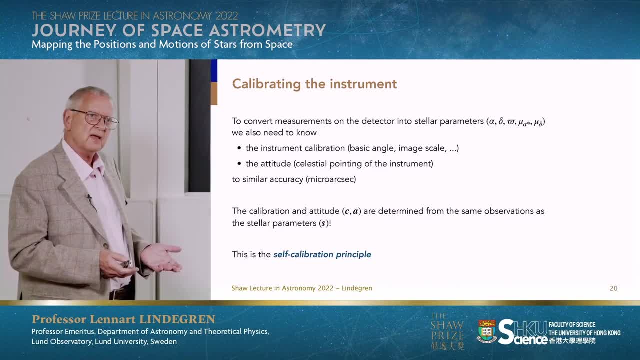 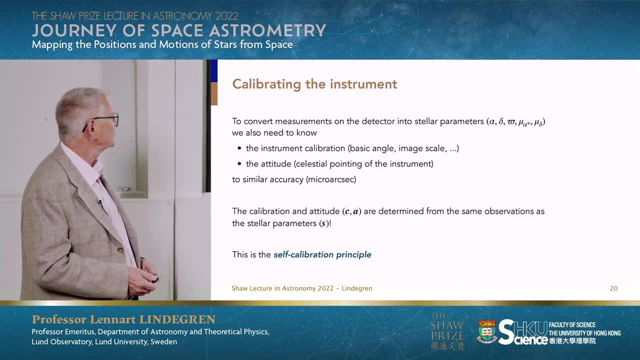 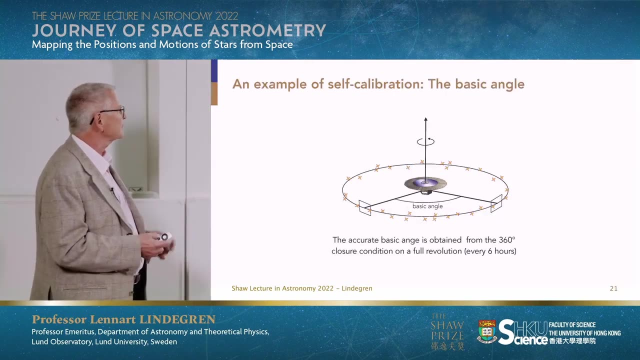 for the calibration or attitude determination, and we don't need any special observations for that. We use the same observations as are collected for the astrometry, So it is a self-calibrating instrument in that way. To illustrate how this works in practice, let me just 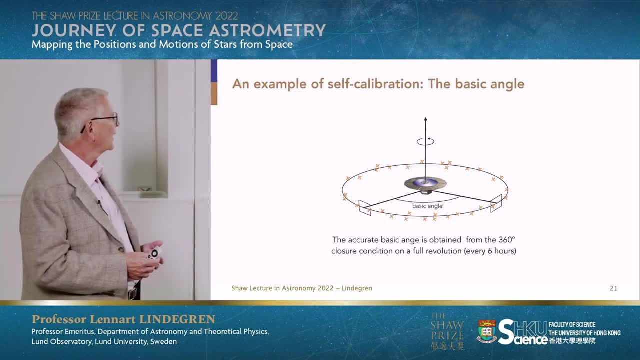 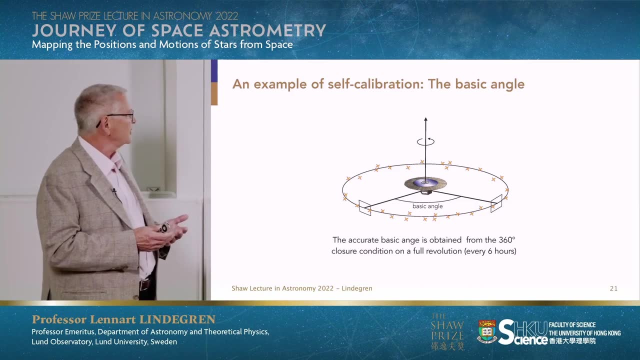 take the example of how the basic angle is determined. Assume that we know approximately what the basic angle is, We can use this value to compute the angles between pairs of stars in the two fields of view And as a satellite turns a full revolution in six. 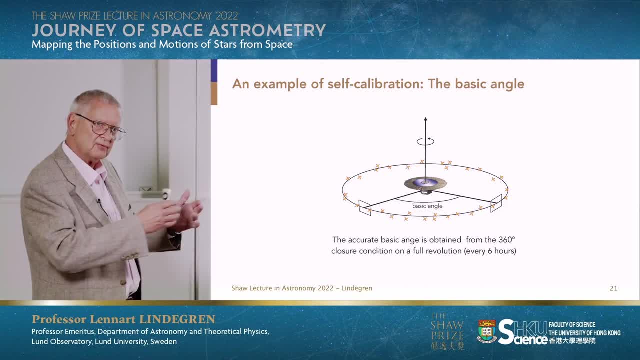 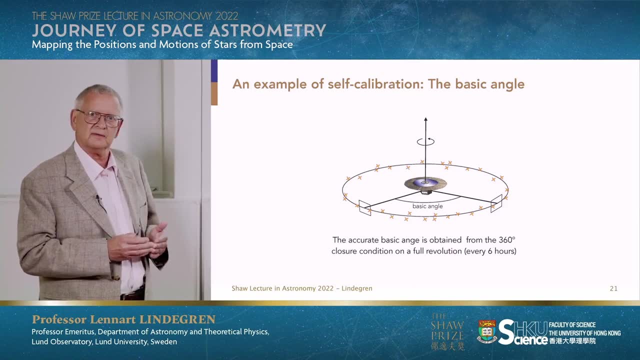 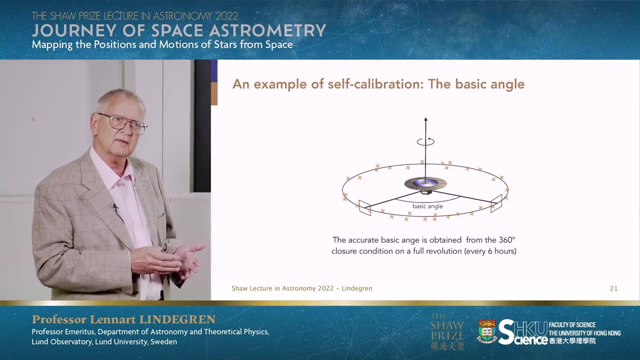 hours. we get angles between different pairs of stars And if we add up all these angles along the great circle they should add up to 360 degrees. But if we use the wrong value for the basic angle, they will not add up to 360 degrees. 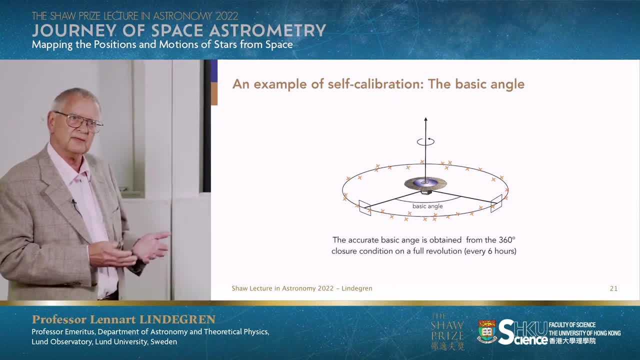 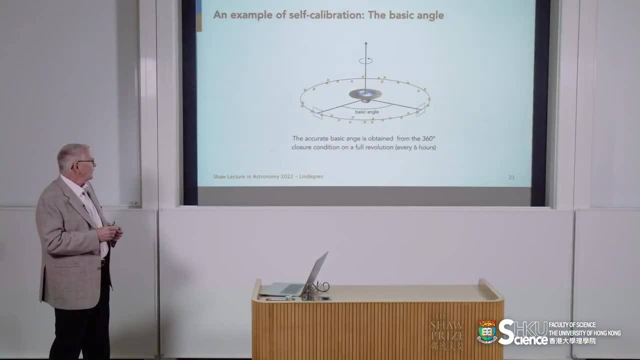 but to something different, And that allows us to compute what the basic angle actually was, And the result will be as accurate as the measurements are. So effectively we get the calibration of the basic angle every time the satellite completes a complete revolution over six hours. 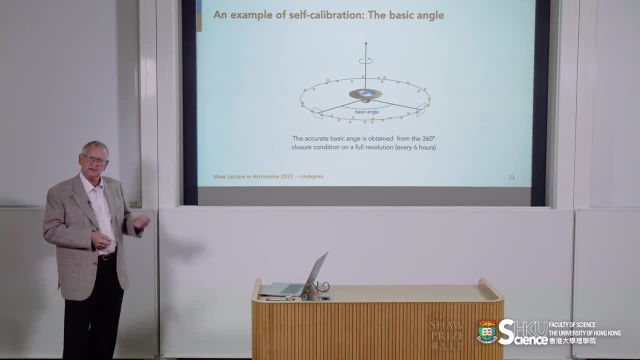 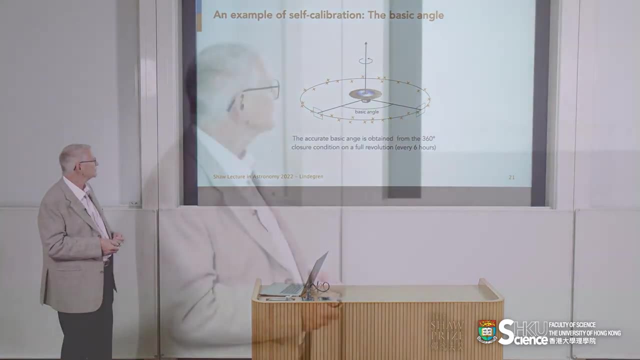 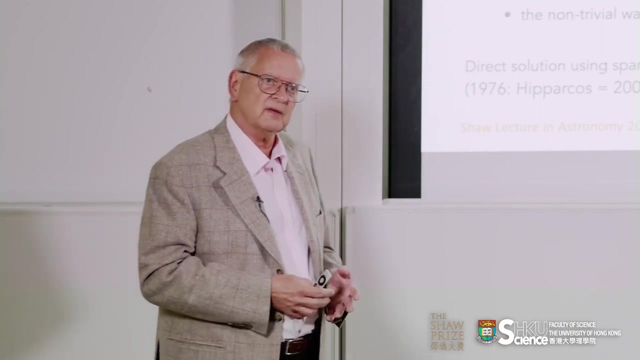 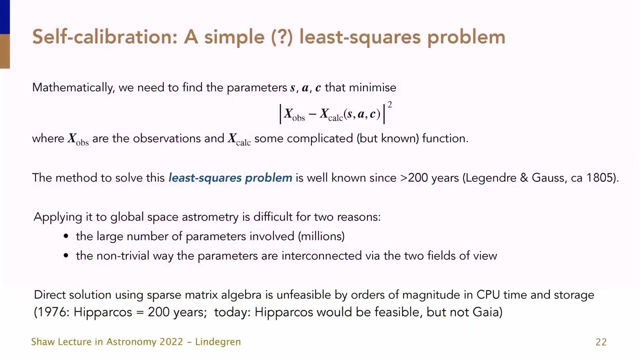 In a similar way, other parameters like the image scale and the attitude and so on are obtained from the observations, basically by the equivalent procedures. It is actually not difficult to formulate these self-calibrating principles in mathematical terms. The observations here denoted x obs. 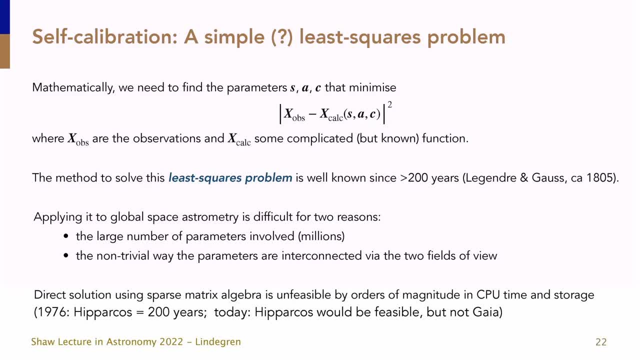 they can be described in terms of all these parameters, the stellar parameters as the attitude and the calibration parameters, by means of some complicated function: x, calc. It is complicated but known. What is not known is the values of the parameters s, a and c. 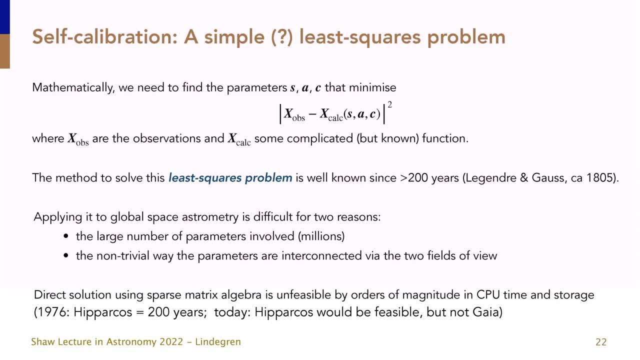 What we have to do is to adjust these parameters until we get the best agreement with the observations, as measured by the sum of the squares of the differences between the measured values on the detector and the calculated values, assuming that we have the different parameters. 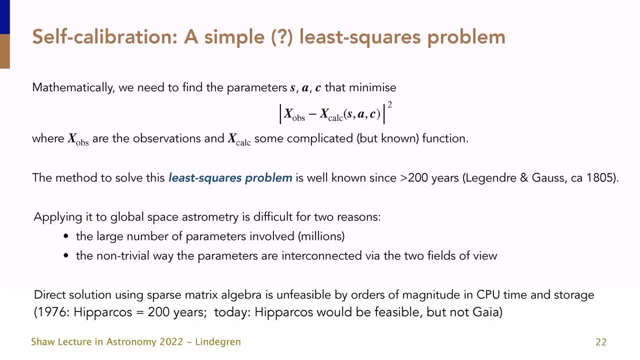 This is what we call a least squares problem, And the way to solve it has been known for more than 200 years. So in principle it is a simple problem, But in practice it is very difficult, for two reasons. One is that there is 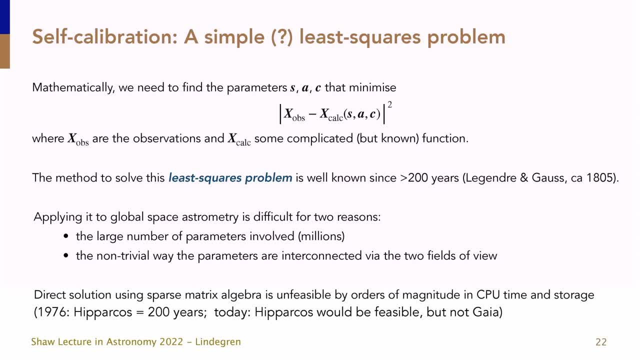 a very large number of parameters to solve, millions of them, hundreds of millions even. And the other is that these parameters are not. they are interconnected in a very complicated way thanks to the two fields of view, where the observations are mixed, and also the scanning law, which makes 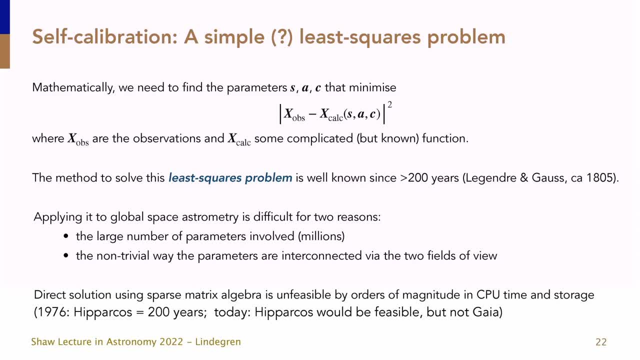 a complicated pattern on the sky, And this means that if we try to do a direct solution of this problem, using sparse matrix algebra, for example, it would require far too much computing time and computer memory to be solved, Even with the biggest computers available on earth today. 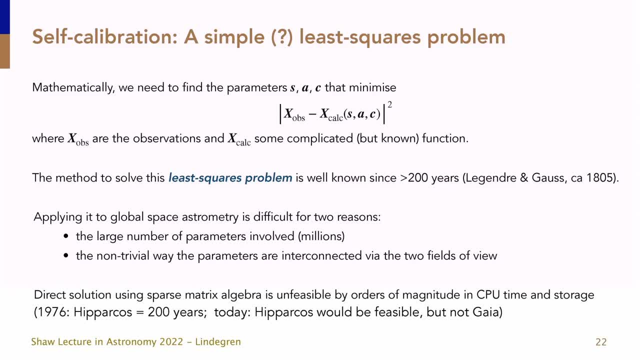 Already, in 1976, it was concluded that to solve these equations for Hipparchos would require 200 years on the most powerful computer available in those days. Today, this problem would probably be feasible for Gaia. Sorry, it would probably be feasible for Hipparchos, But 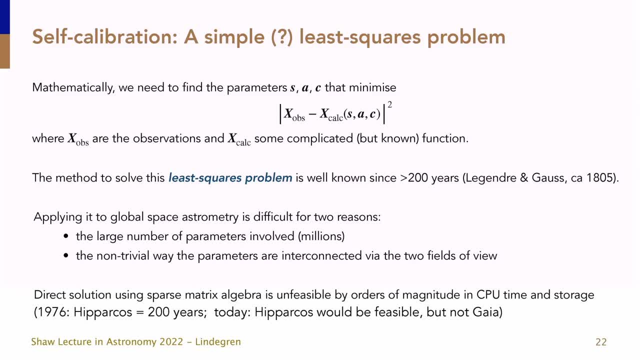 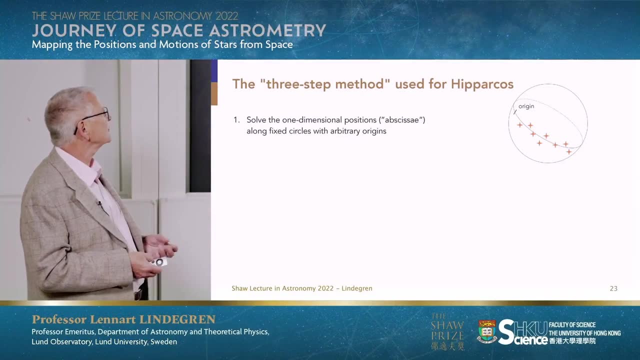 in Gaia. we have so many more observations and so many more unknowns that it is certainly not feasible to do a direct solution For Hipparchos. we came up with an approximate solution in the 1980s, and that is the so-called three-step method. 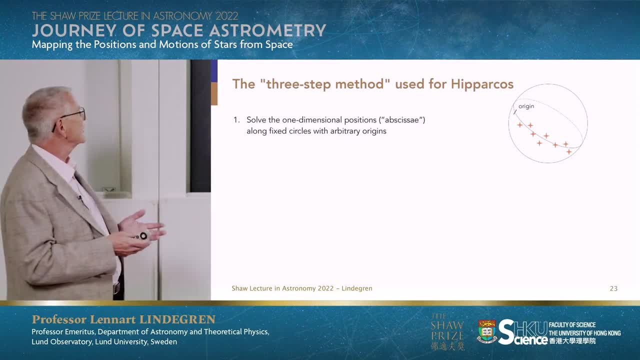 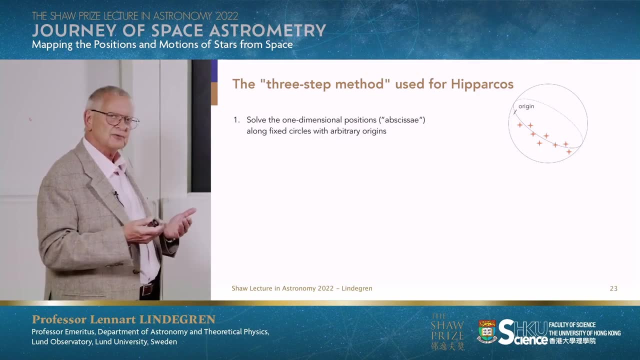 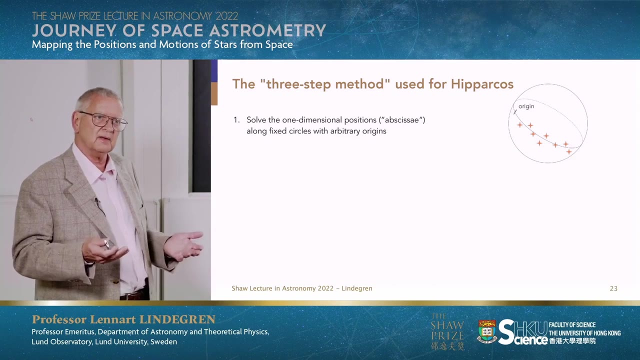 which I will briefly describe. So the first step is that we use one-dimensional measurements along a great circle on the sky, where we solve for the coordinates of stars along this great circle at the same time as we obtain the basic angle, image scale and so on. 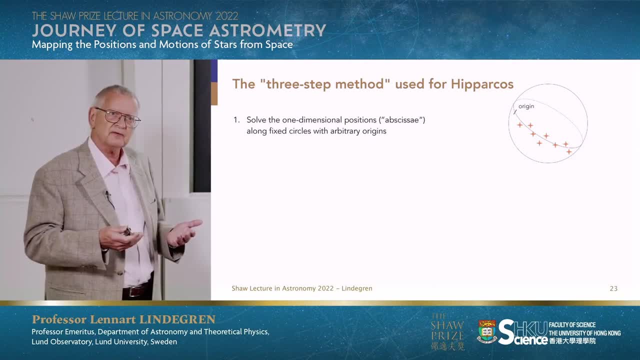 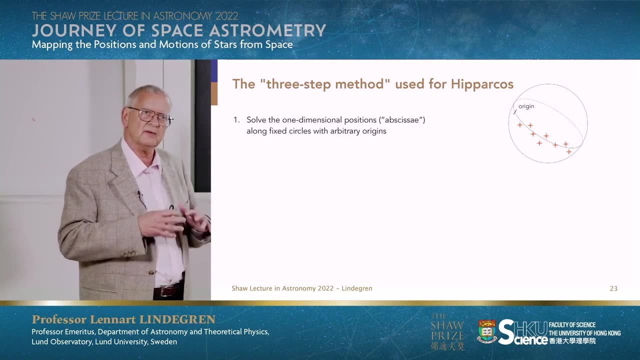 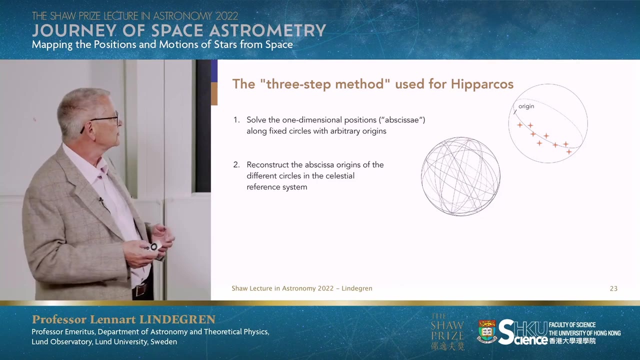 We can get these positions of the stars, but we don't know the origin, the zero point for these angles, because that is only defined when we have the celestial reference frame, which we don't know yet. In the second step we solve the origins of all the 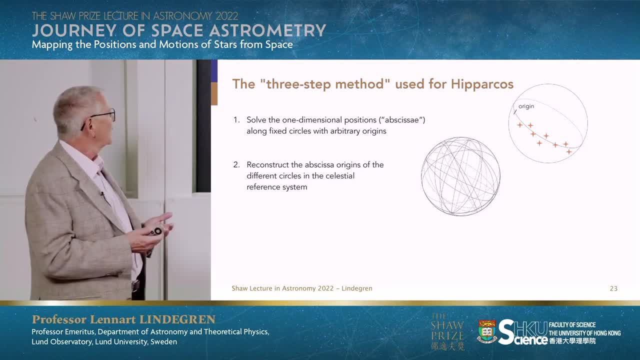 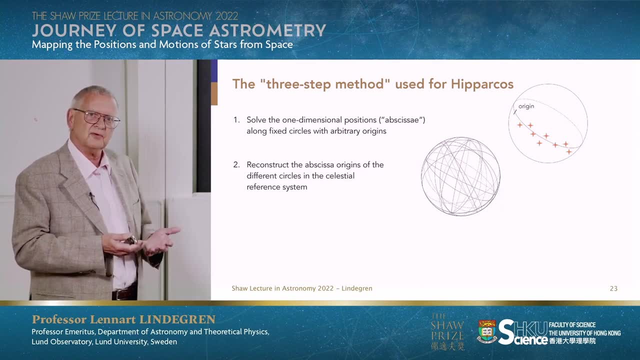 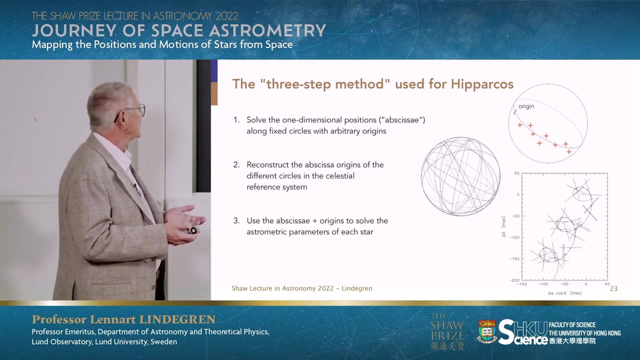 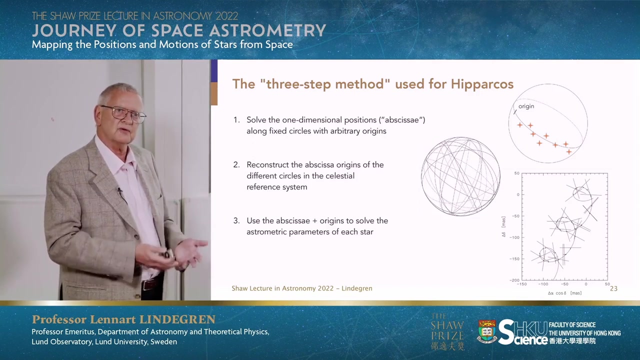 few thousand great circles in such a way that the coordinates form a consistent reference frame over the whole sky. And then the third step is simply to combine the abscissa and the origin for each individual star in such a way as to get its positions, propromotions and parallaxes. So this worked well for Hipparchos because in each step you don't need to solve very big systems of equations. so it was quite- I wouldn't say easy, but definitely possible to do in those days. It is, however, an approximate method and therefore suboptimal. 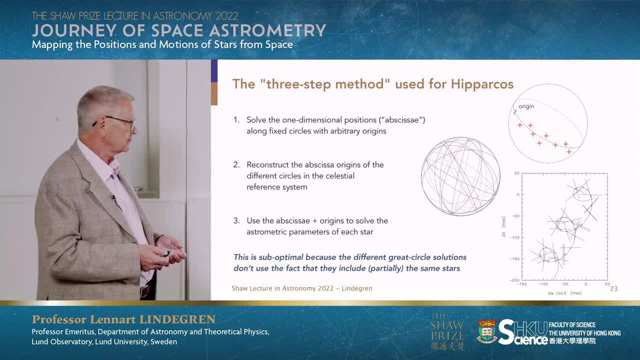 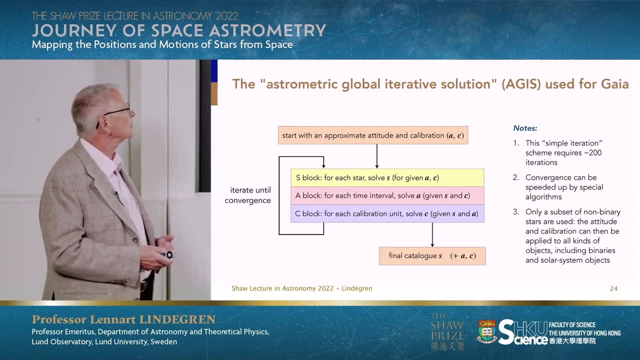 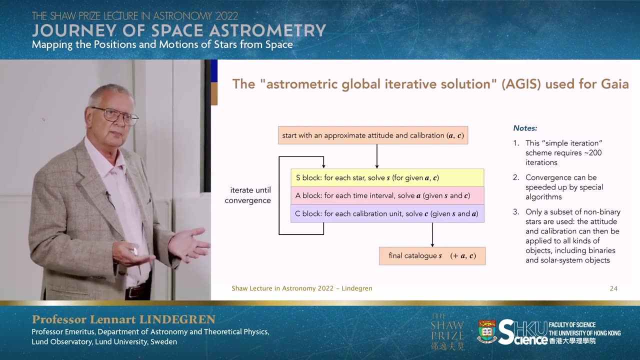 and for Gaia. we wanted to do something better, and what we came up with is what is called the astrometric global iterative solution, or AGES. The idea is actually very simple and was around already at the time of the Hipparchos, although it was not used at that time. 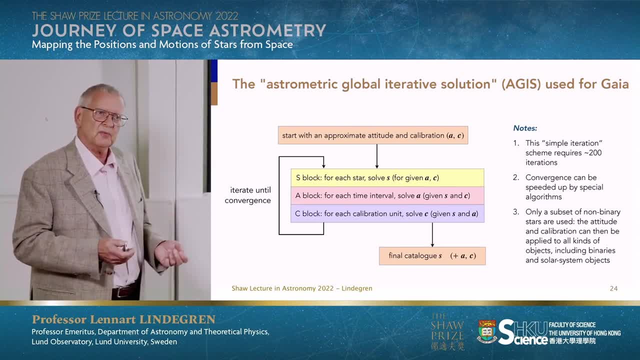 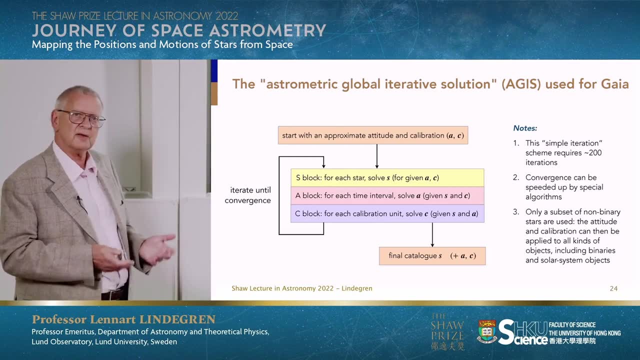 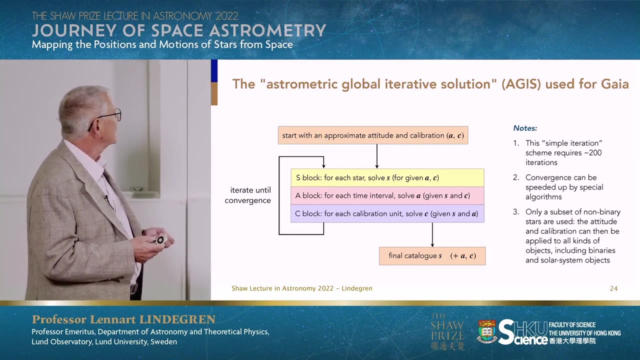 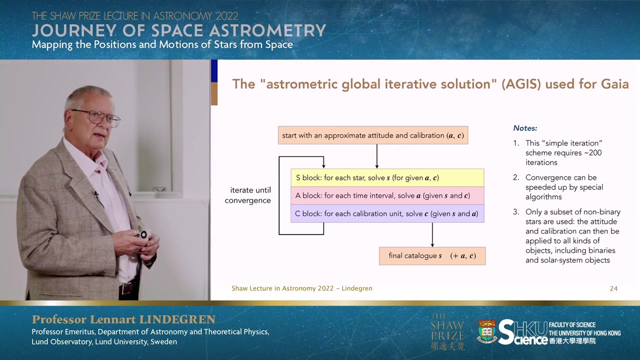 We already from the beginning have a good idea about what the attitude and the calibration parameters are, so we can use these initial estimates to compute the star parameters for all the stars observed, That is, the s block in the three middle block here in yellow. Once we have the star parameters, 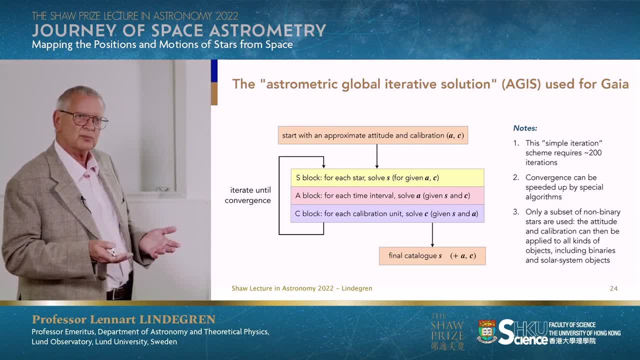 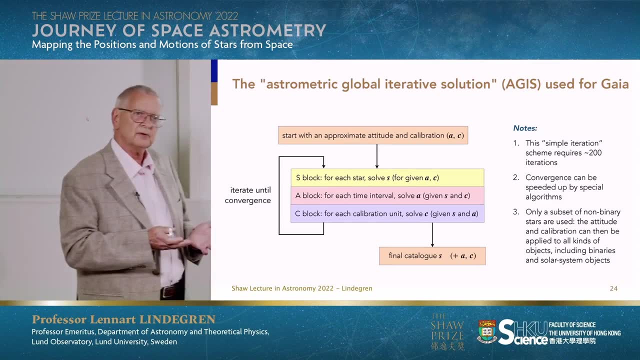 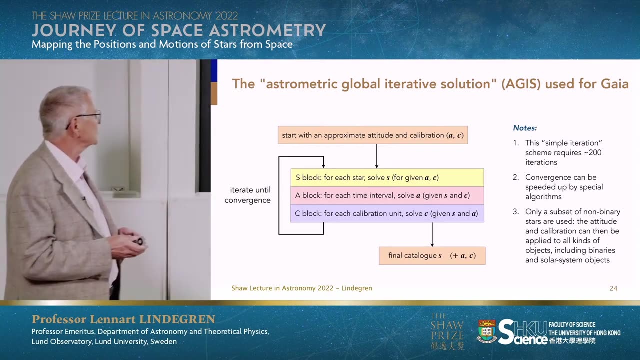 we can use them together with the initial calibration parameters to solve the attitude parameters, that is, the pointing of the satellite as a function of time. This will not be exact either, of course, because we have an approximate calibration and approximate stellar parameters, but it will be better than the 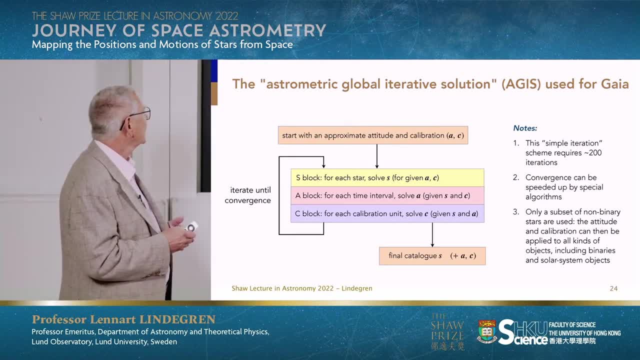 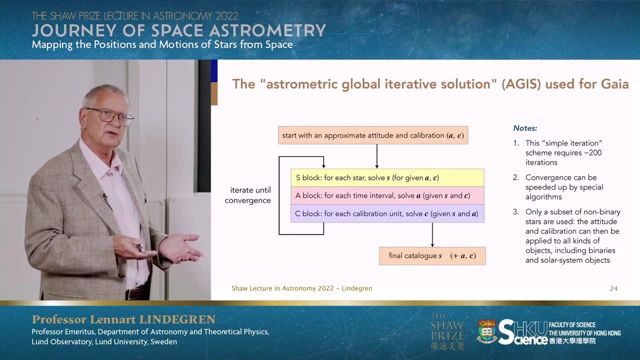 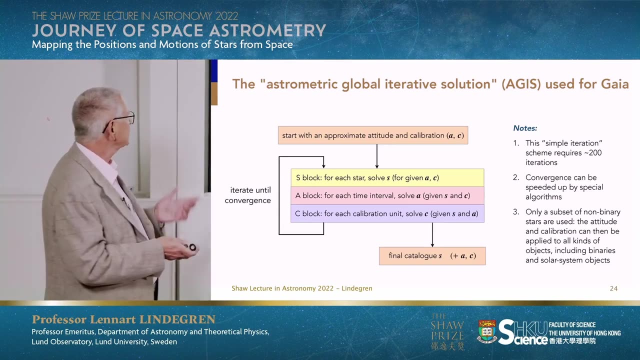 original attitude that we started with, And then in the s block we use the star parameters and this improved attitude to solve the calibration parameters. And at this point we have improved both the attitude and the calibration and we can start again by doing the same loop once more and 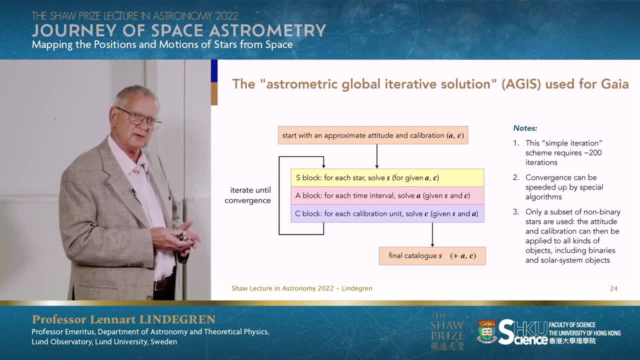 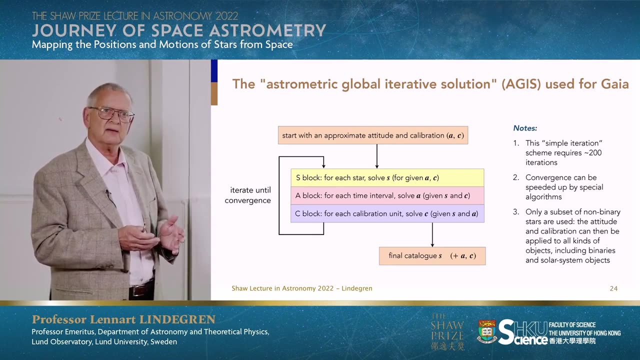 each time we do the loop, all the parameters get a little bit better. It turns out that you need to do some 200 loops like this, but in the end the parameters don't change anymore And it turns out that you actually have the same solution then as from a. 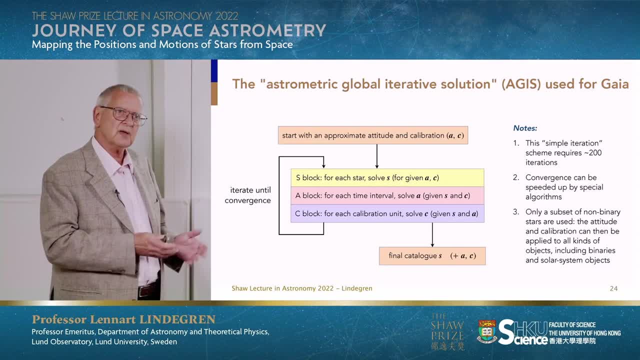 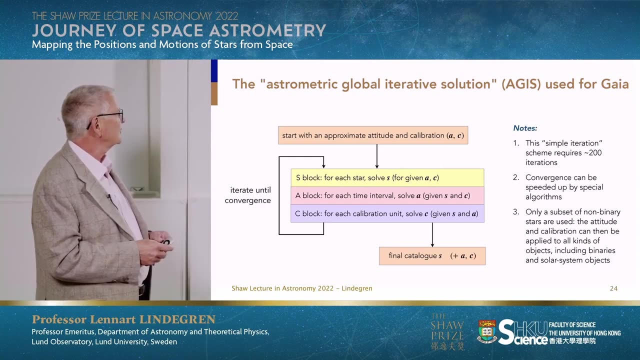 direct solution of all the equations, But you get it for only a small fraction of the CPU time and memory requirements that would be required for a direct solution. So this gives you, in the end, the final catalog And also, of course, the attitude and calibration parameters. 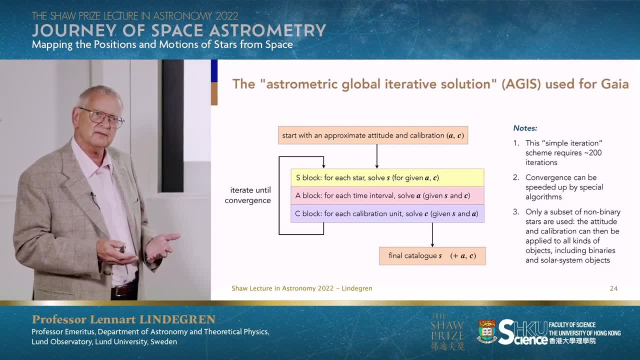 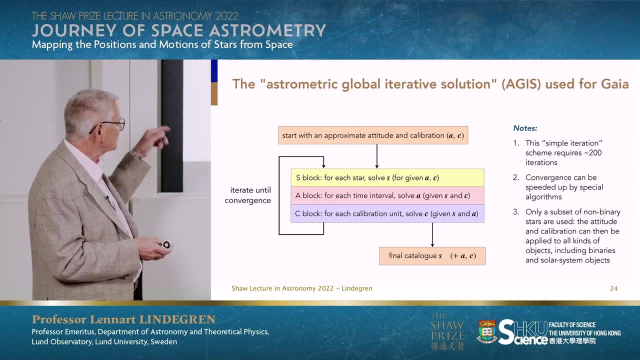 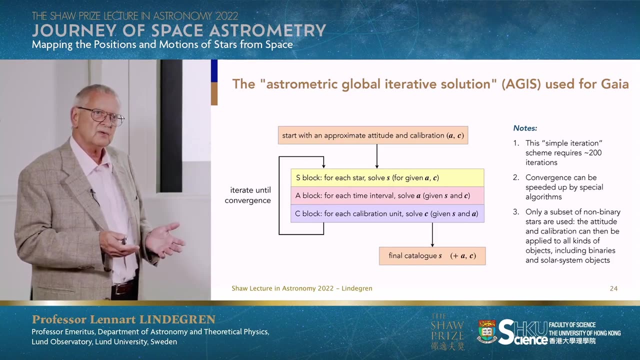 There are several ways to simplify these shortcuts. For example, there are ways to speed up the convergence of these iteration loops, And it is not necessary to do it for all the stars at once. You only need to do it for a subset of well observed and well behaved stars. 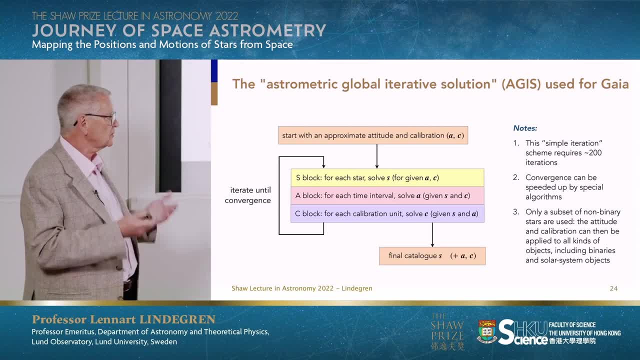 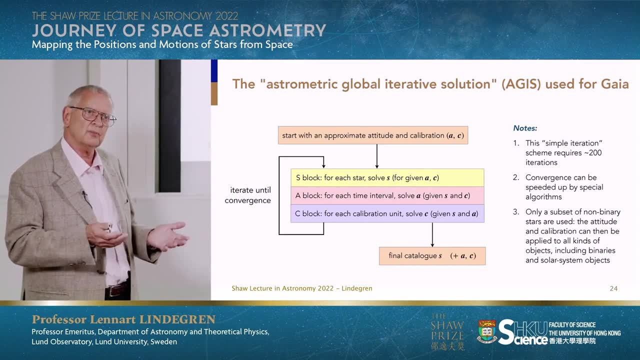 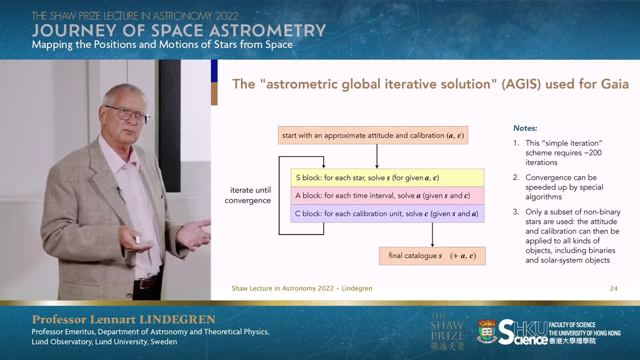 And, once you have done, got good estimates of the attitude and calibration using these stars. you can apply this attitude and calibration to all the observations and get stellar parameters for all the stars but also other kinds of data, For example the positions of solar system bodies and galaxies. 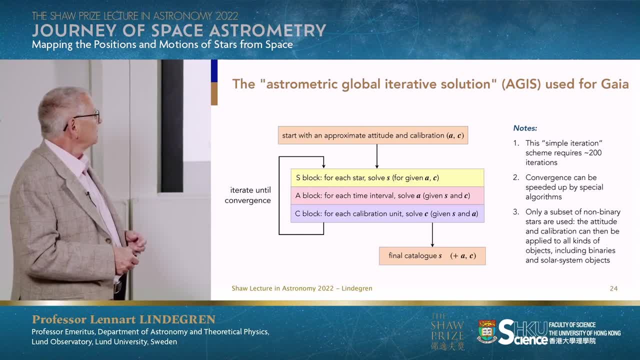 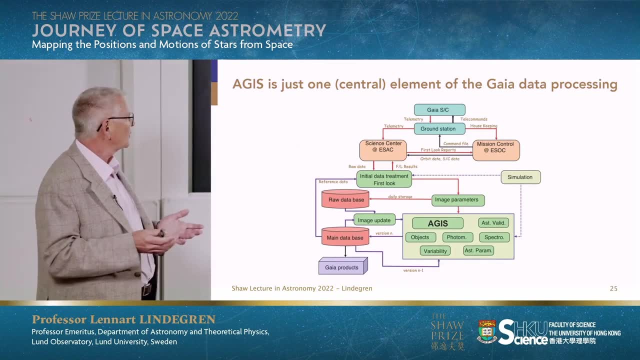 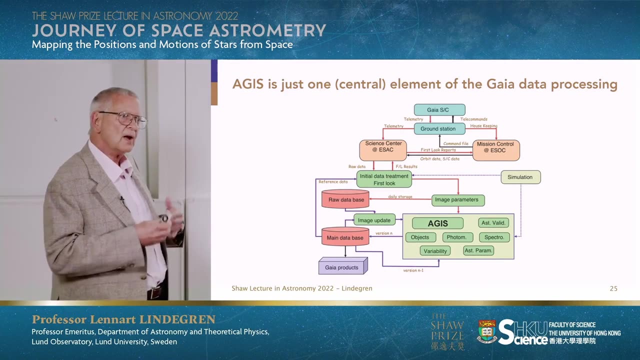 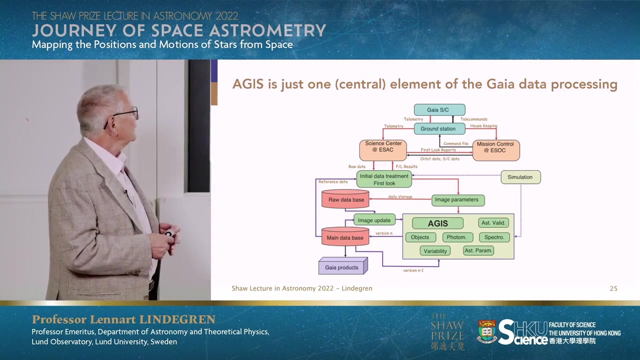 and so on. In this talk I have completely talked only about the astrometric data and the astrometric solutions, But we should realize that that is only one element in a very big and very complex data processing task for Gaia. There are 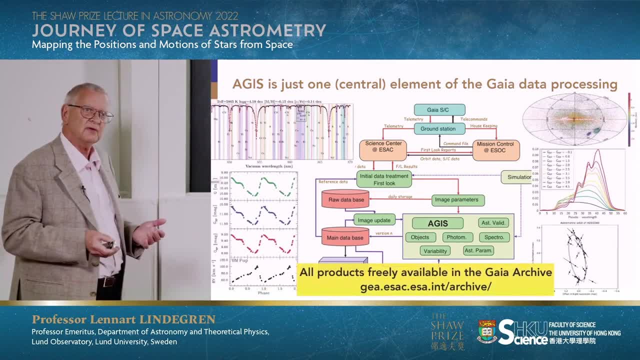 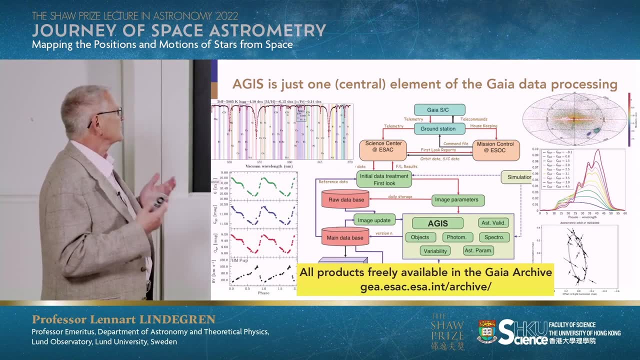 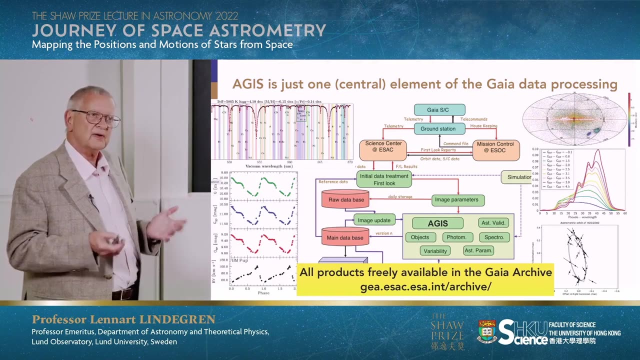 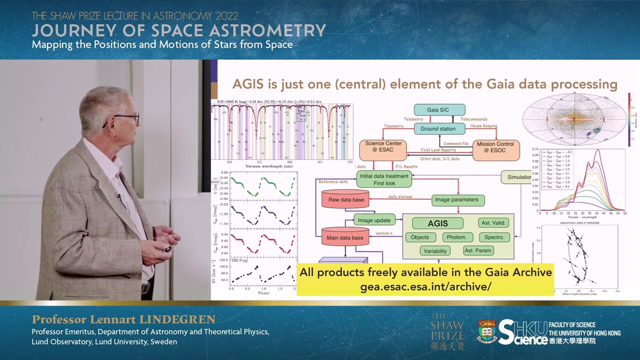 hundreds of scientists working on producing all other sorts of data- Photometric, spectrometric- for binary stars, galaxies, quasars and so on- And all of these products are freely available in the Gaia archive for everybody to use. I will end this talk. 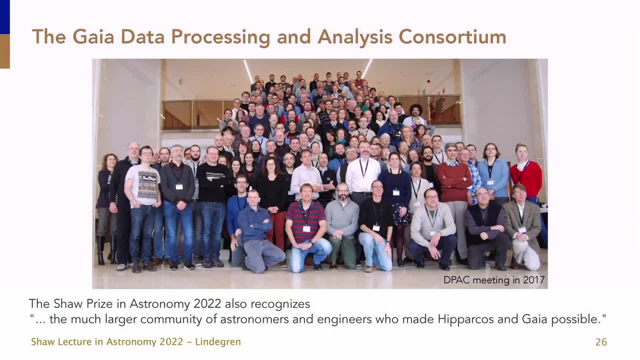 with this picture, this photograph of members of the Gaia Data Processing and Analysis Consortium. It is only a small fraction of all the people who have contributed to Gaia over the years, and many other people contributing to Hipparchos are not here in this consortium. 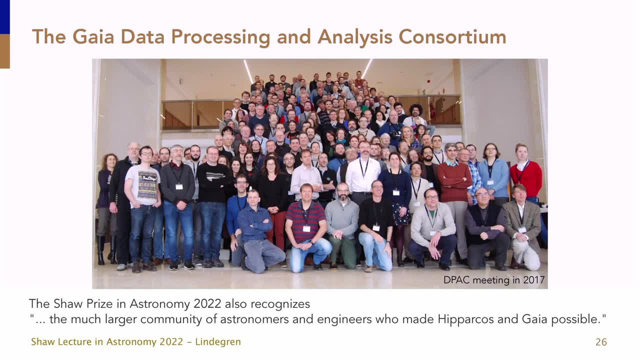 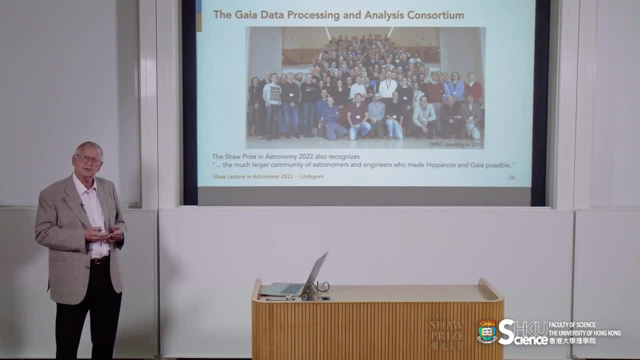 The Shaw Prize in Astronomy 2022 also recognizes the much larger community of astronomers and engineers who made Hipparchos and Gaia possible, And I will let this image represent all of them. To them, I say, and to the Shaw Prize Foundation I say, thank you. 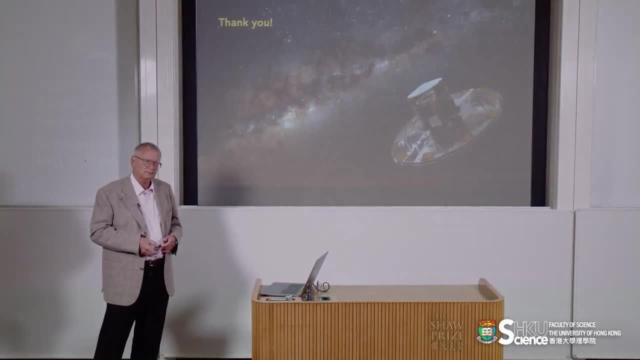 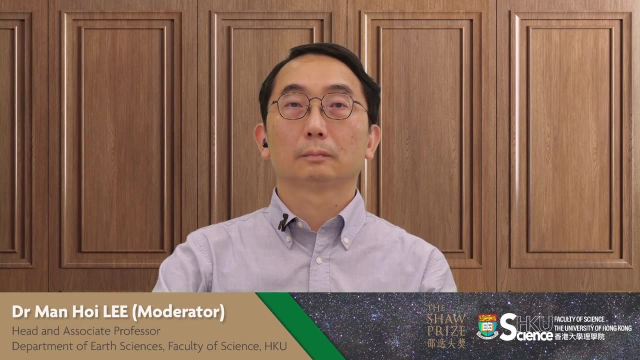 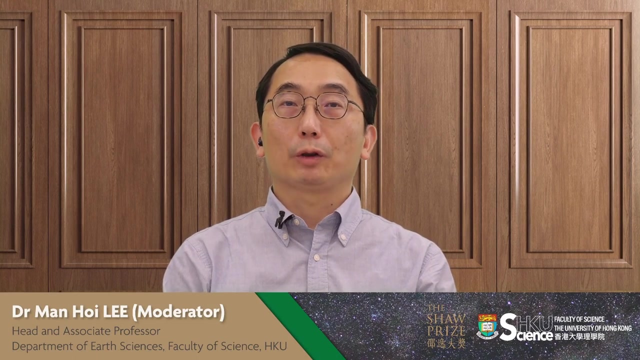 Thank you for your attention. Thank you for your attention. Thank you, Professor Lindgren, for the lecture. I am sure that all the audience benefited a lot from both lectures. For the audience: if you have any questions that you wish to ask our Shaw laureates, please take this. 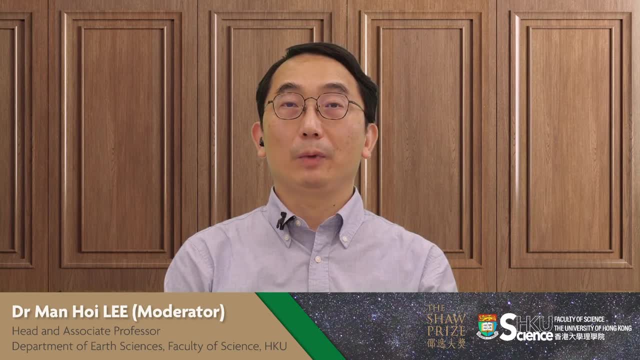 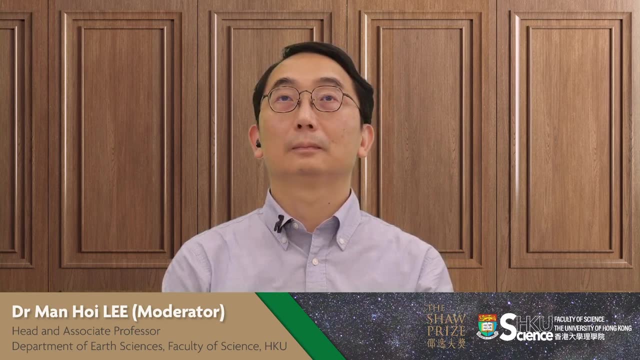 opportunity to ask them now. Just feel free to unmute yourself or type in your questions in the chat room here. So this is Mark Cropper. Can you hear me? Yes, we can. I wonder if Michael and Leonard can explain why. the basic 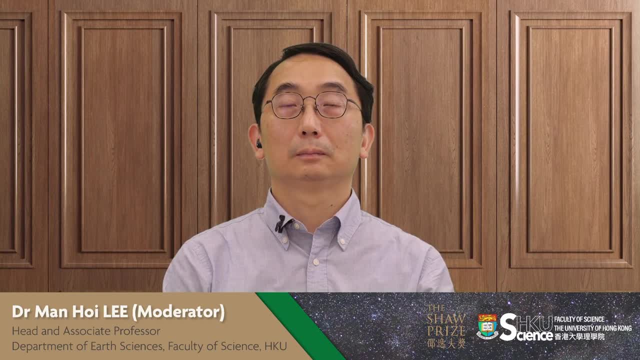 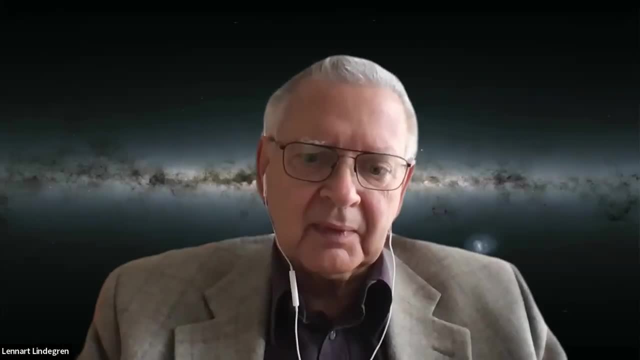 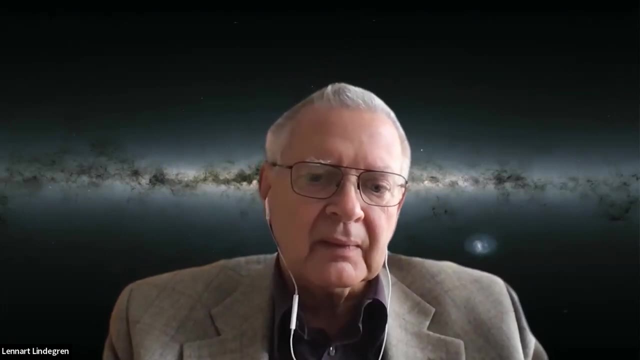 angle is not 90 degrees and why it was chosen to be the 106 degrees, 0.5 in Gaia. Yes, that's a good question. actually, It could have been quite a different angle, In fact almost any angle, from about 30 degrees to. 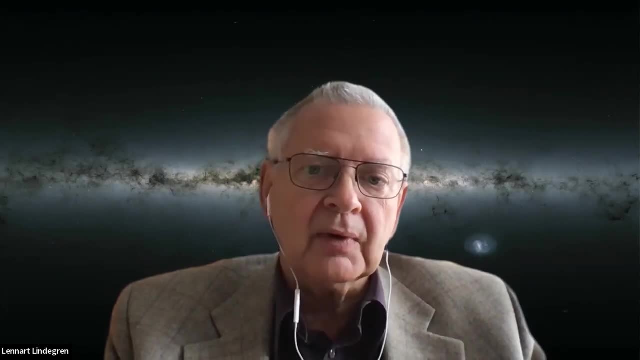 150 degrees would have worked equally well for solving the global astrometric problem. But when you do this solution on a great circle to calibrate the basic angle and scale, there are certain values that you should avoid and they are simple fractions of 360 degrees Like 90 degrees. 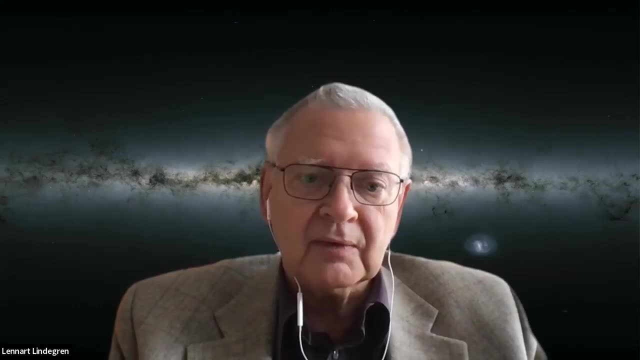 is not a good angle. 72 degrees, which is one fifth of a full circle, is not a good angle, and so on. And this value, 106.5, is one of the values that just avoids these simple fractions. There was a whole range of 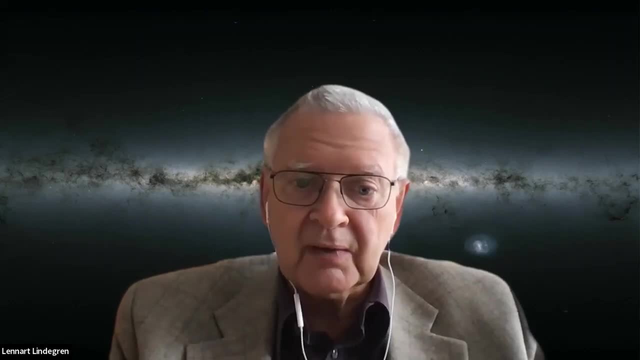 variable values, and the final choice, I believe, was up to the engineers that were going to design this instrument. They had to take into consideration that it could easily be accommodated, and and so on, So there were many constraints to be taken into account. 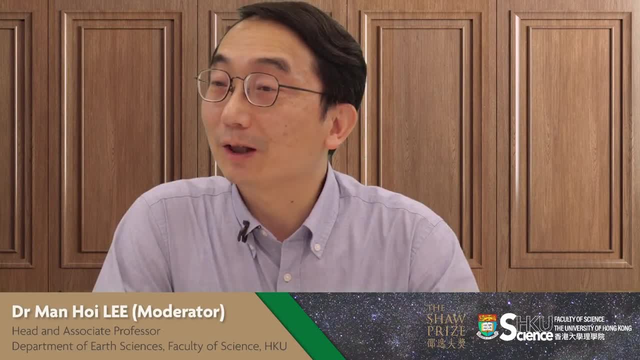 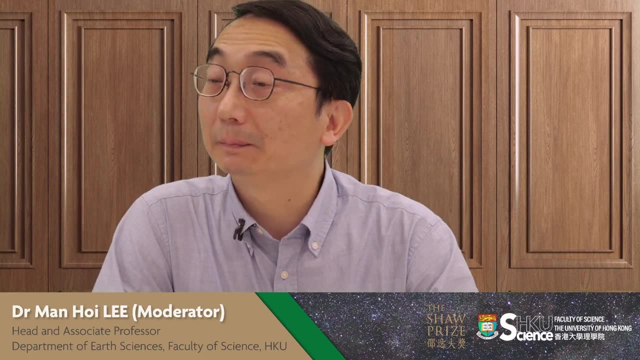 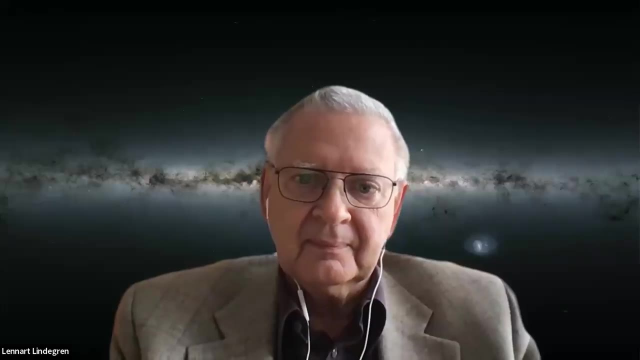 Thank you, Dennett. So someone asked: can you explain more about why we need to measure the star in two directions in the sky at the same time? Maybe shall I take that Go ahead Your question, Mr Fung. what we'd like to know is how. 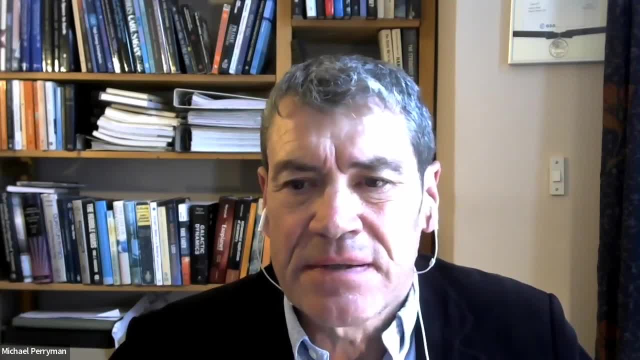 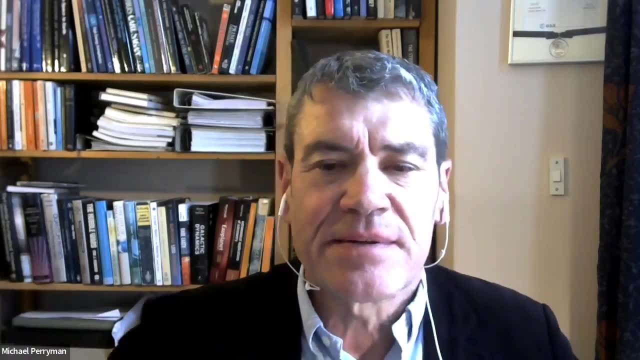 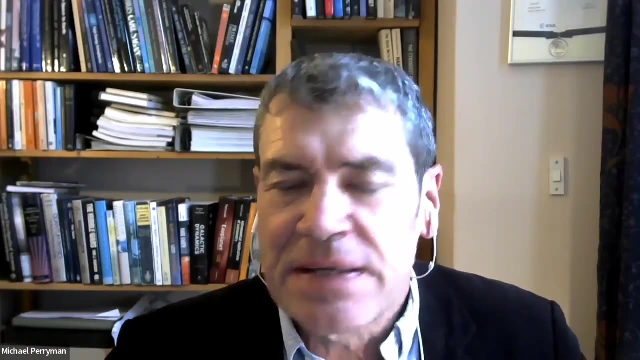 each star is moving through space. Forget any concept of coordinate directions. We'd like to know how the star is moving through space and any motion through space can be described by three quantities in Cartesian coordinates: x, y, z coordinates. You want the x, y and z values. 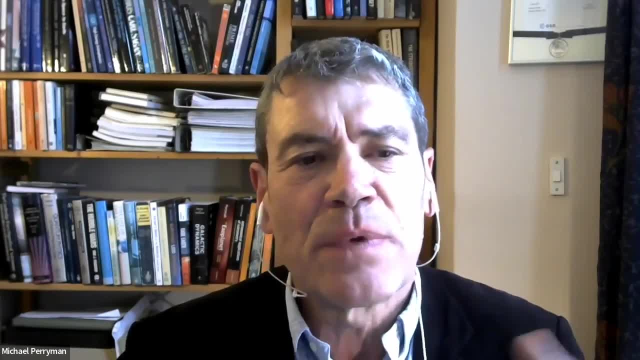 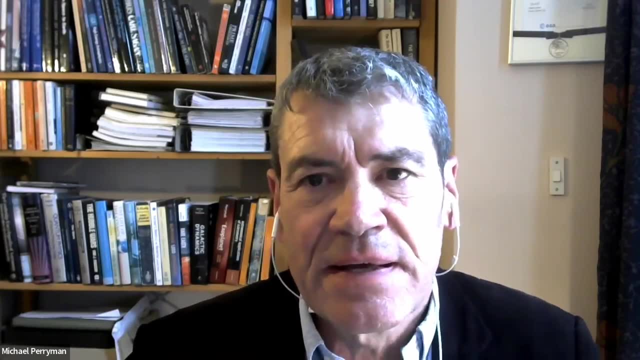 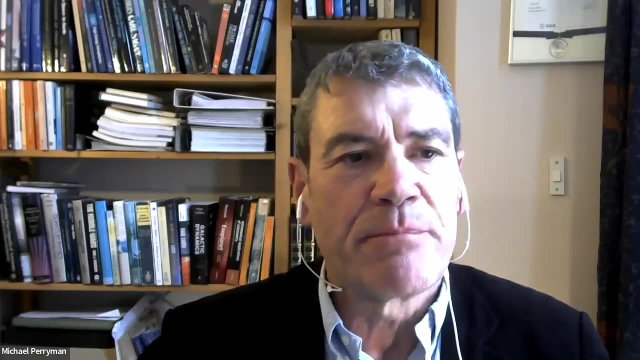 What we can only measure with a mission like Hipparcos and Gaia from the astrometry is how the stars move on the plane of the sky, projected on the plane of the sky. So we measure that using these astrometric measurements. 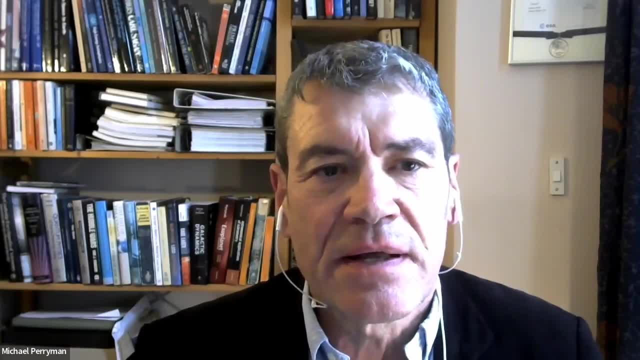 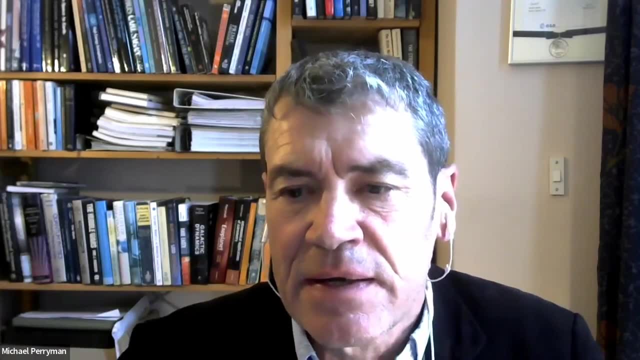 and you can think of that in two coordinates. I think it's simply stated like that. Ideally, we'd like to measure the radial motion of the star as well, and there is a separate instrument on board Gaia called the radial velocity spectrometer. 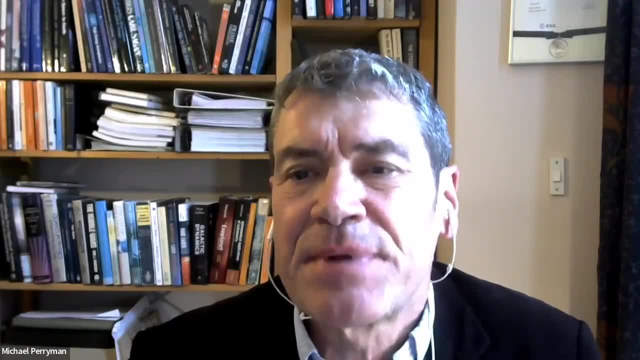 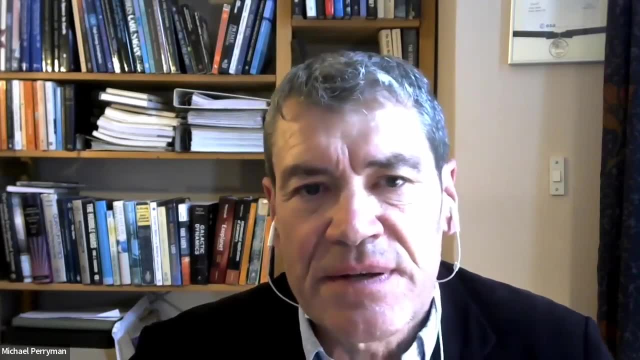 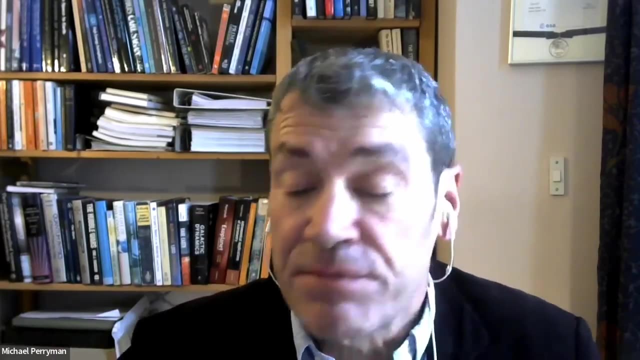 which measures the radial velocities of a subset of the stars, the brightest stars in the radial direction. So when you combine these astrometric measurements made in two directions, on the sky, with Gaia, with radial velocity, you get the full space motion. If you don't have 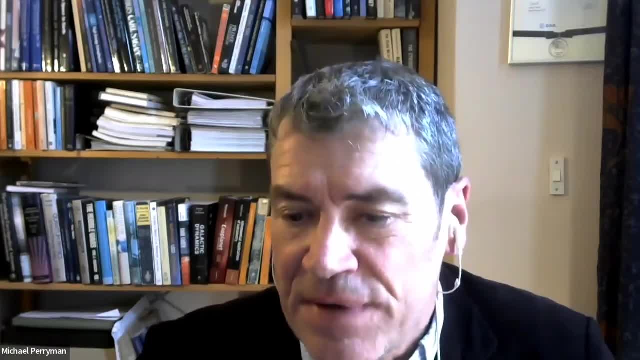 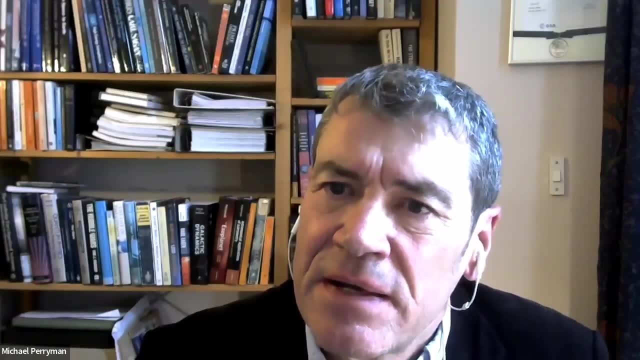 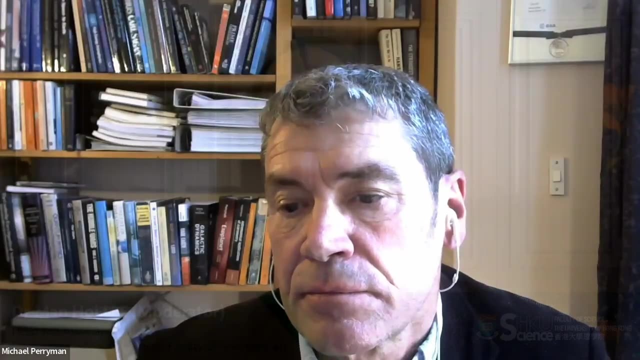 these radial velocities available, so we don't have those for the fainter stars. there's not enough photons, the stars are not bright enough to measure this. then you just have a projection of the stellar motion on the plane of the sky. Okay, thank you. 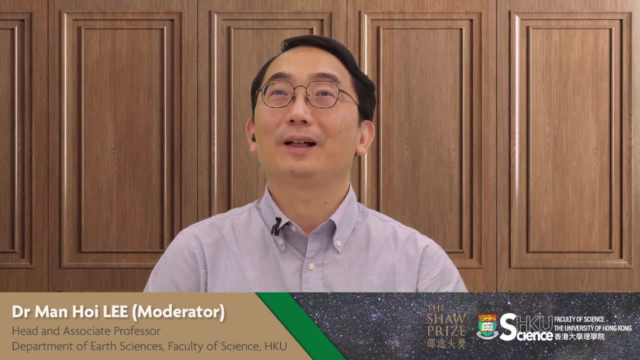 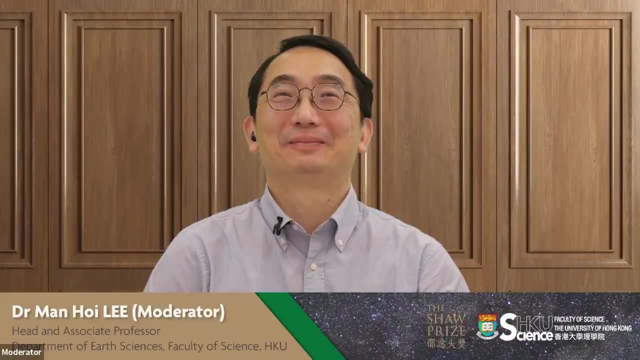 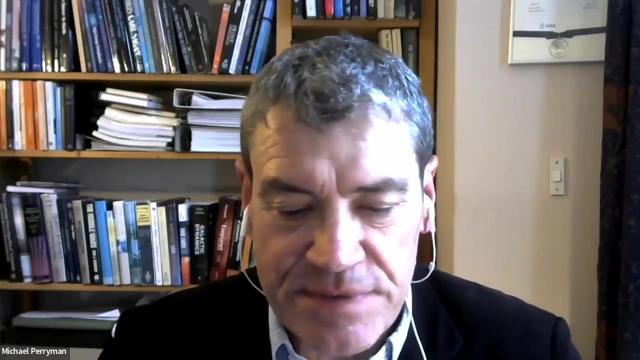 So we have another question. on the chat room, Someone's daughter was asking why it's called Gaia. Do you want to take that, Michael? Yes, when you come up with any experiment, you have to come up with a good name that will attract. 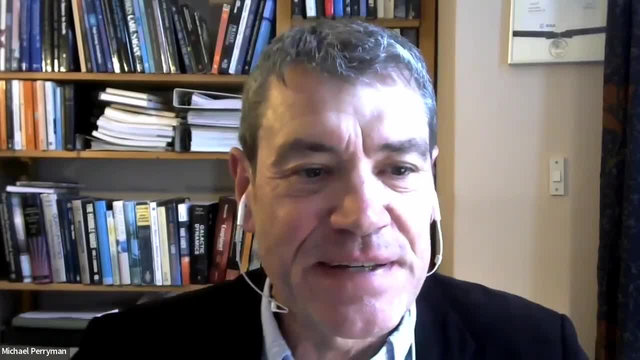 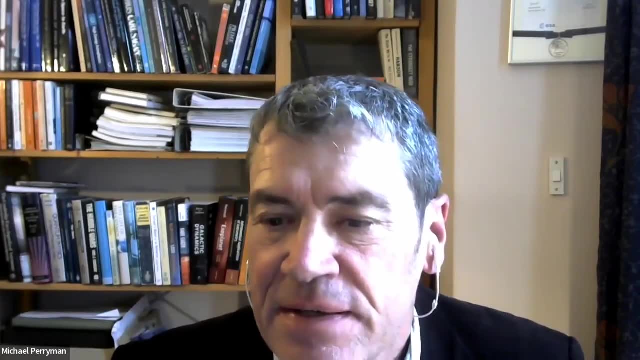 attention to the funding authorities. That's part of the answer. We liked the name, So you come up with a name and then you think about an acronym, And in the early days we thought that one of the early ideas was to make these measurements. 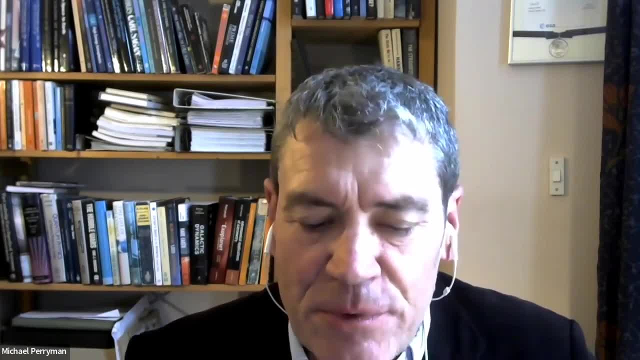 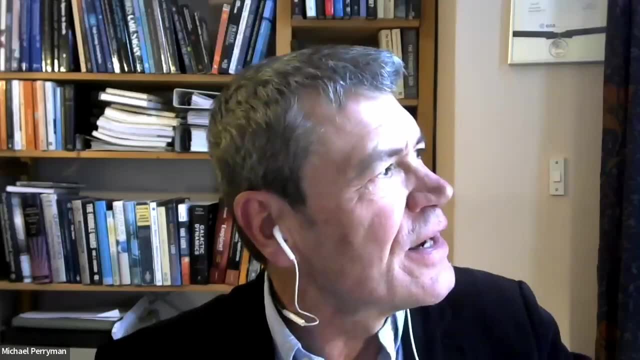 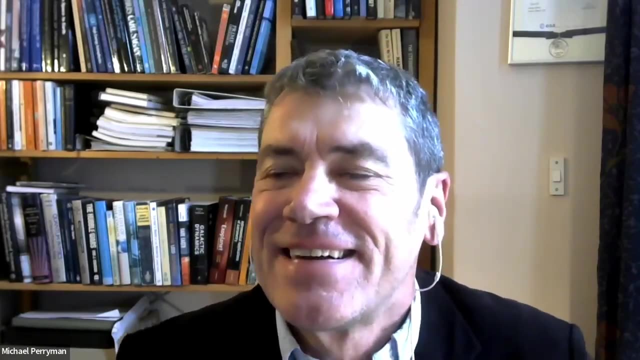 using a technique called interferometry And we dreamt up this name, this description, global astrometry, global astrometric interferometer for astronomy, global astrometric interferometer for astronomy, and abbreviated Gaia As the design of the satellite. 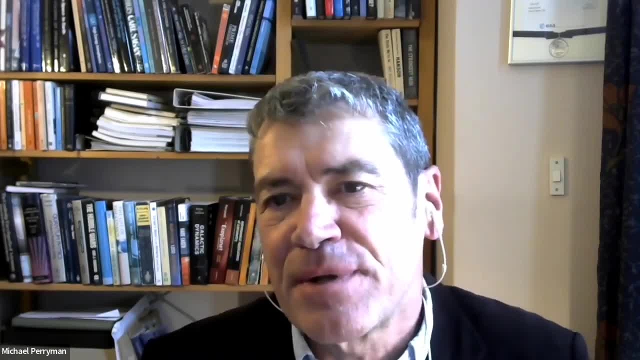 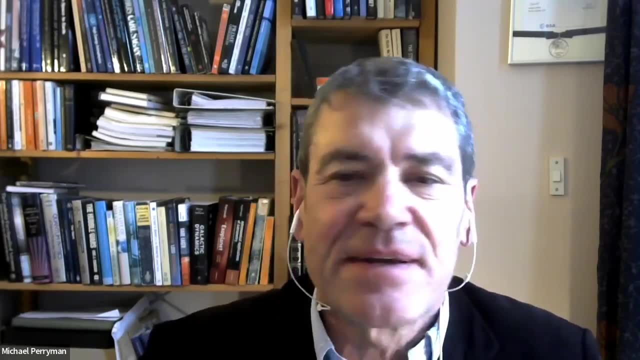 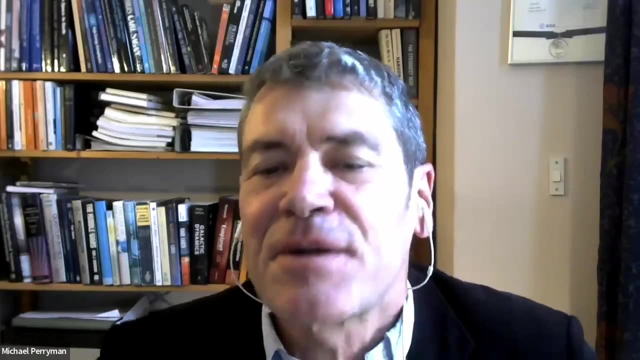 developed. the interface with the parametric principles was dropped, but we kept the name and we just called it Gaia. So it's a nice name. It's some kind of tenuous relationship to the goddess of the Earth. It's just a nice name. 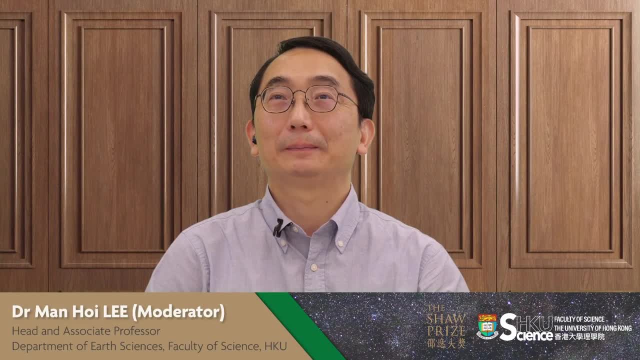 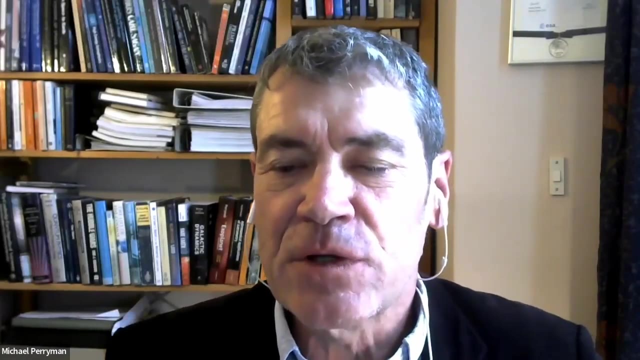 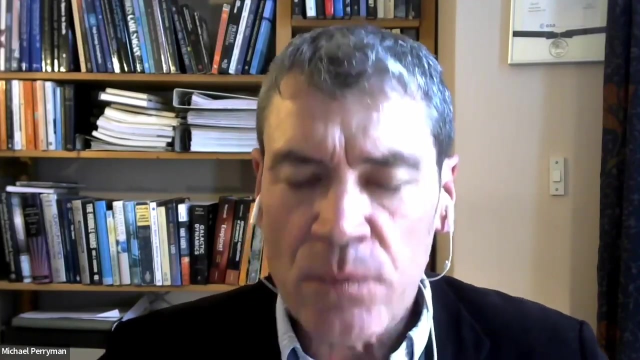 Okay, We can take more questions. What's next after Gaia? That's a problem for young people. The world is open to the new generation of astronomers to think of how to do it better, And what we know from our studies with Gaia is that you can make. 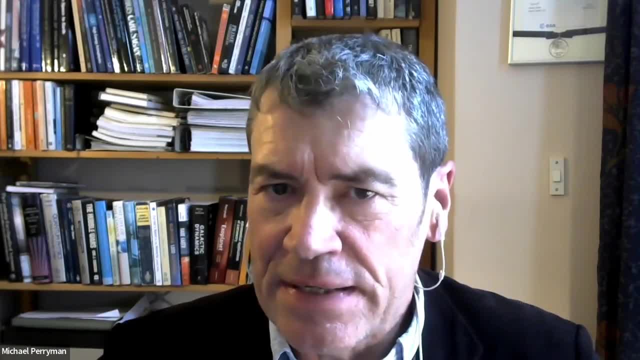 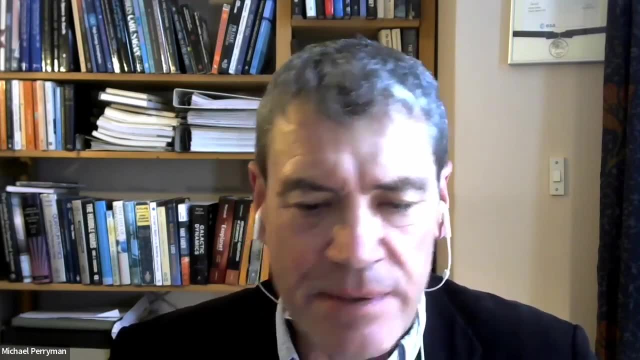 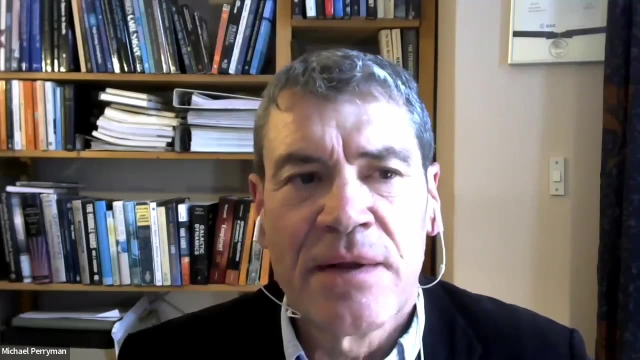 these measurements far more accurately than we could even with Gaia. In principle, one can go to much, much better accuracies. There are studies being carried out A little bit more on that. There are some ideas being pursued in Europe and elsewhere. 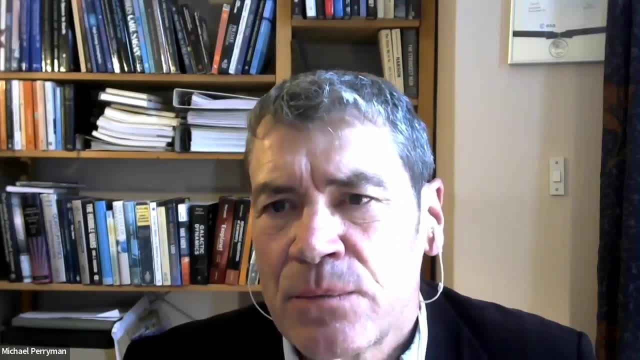 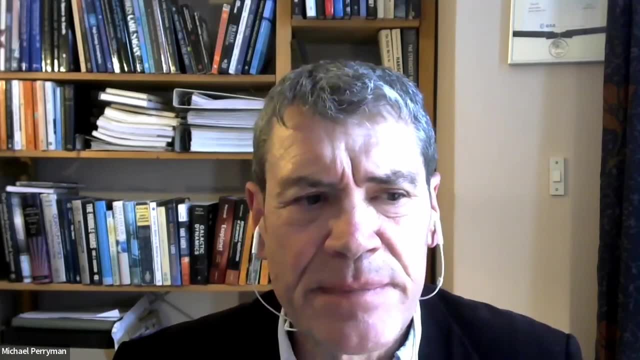 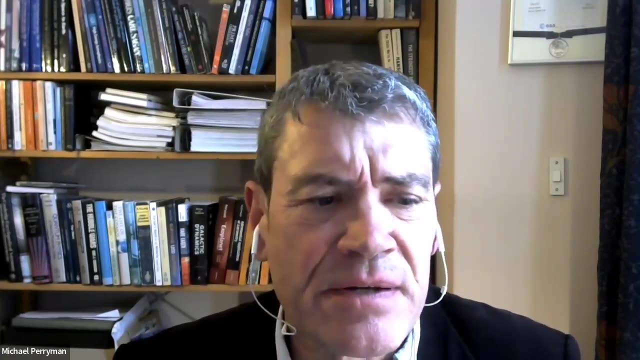 for the next generation. But I think what we, what has been demonstrated with Hipparchos and Gaia, is that this is a very, very clever, robust way of making these measurements: The scientific information available to us about the way our galaxy is formed and the way our universe is. 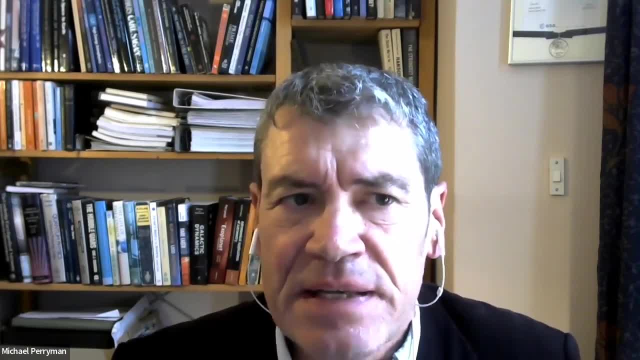 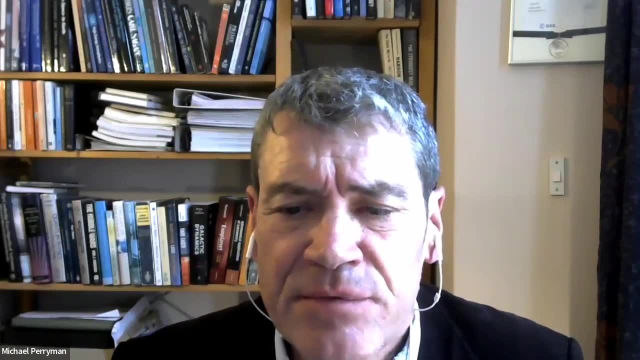 structured, would benefit from even more stars and even more accuracy. That's a possibility, and it's a challenge for the next generation to come up with the best way of doing that. Lennart, maybe you could add a few words about what's being done already. Yeah, it's not completely obvious how you should go forward here. There has been discussions about various directions. For example, you could go towards a pointed mission, that by being pointed, you can have much longer integration time on each object, which means that you can do it. 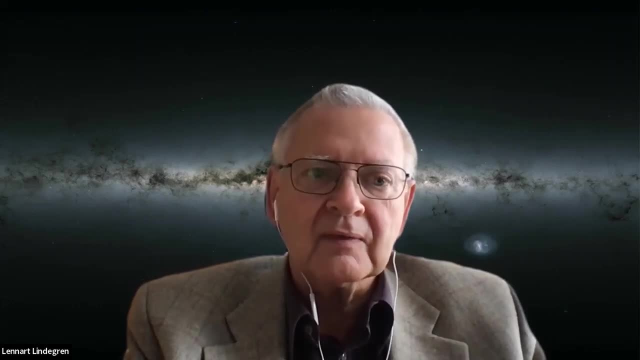 more accurately and also reach much fainter objects, And that would perhaps open the possibility to detect Earth-size planets around stars using astrometry. Another possibility is that you can extend the wavelength range. Gaia is essentially sensitive to visible light, but we know that. 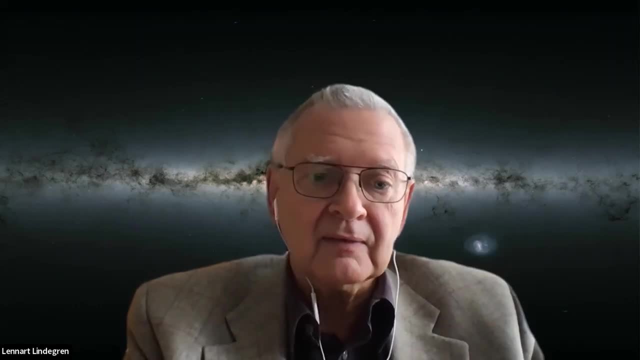 a large part of our galaxy is hidden behind dust clouds, and it would indeed be interesting to be able to penetrate these clouds a little bit better, which you can do if you go to slightly longer wavelengths into the near infrared, So that is also a possibility. 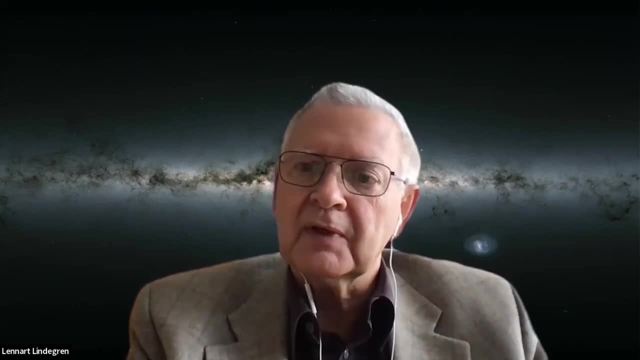 And there has been proposals for such missions, including the Japanese Jasmine mission and the European mission, which is currently called Gaia Near Infrared. As Michael said, we have to come up with a better name that captures the imagination of those who are going to give us. 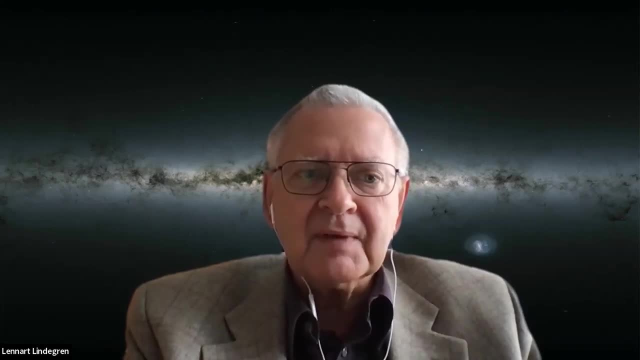 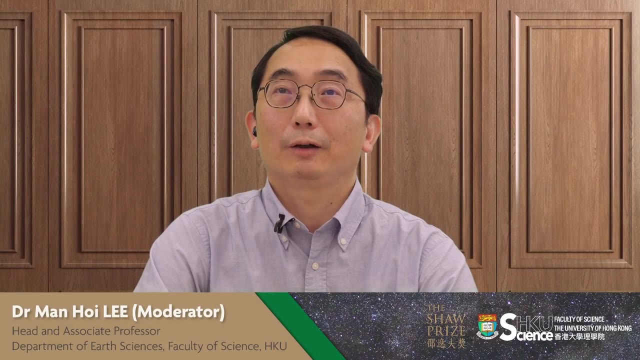 money for it, But these are some of the possible directions we could go with future missions. Okay, thank you. We also have a question on the chat room asking. it says that you both mentioned the measurements of very distant objects, including quasars. Can you explain the? 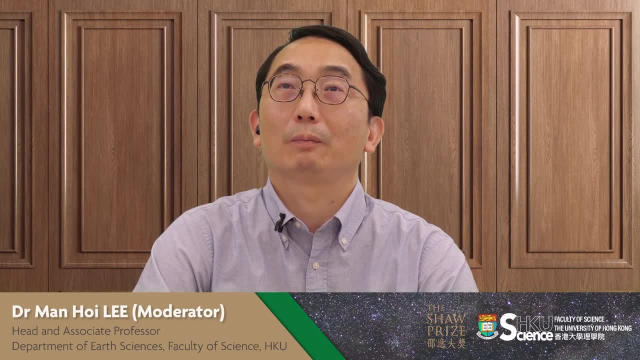 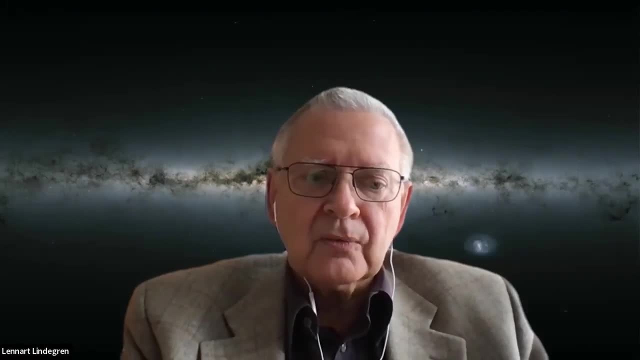 importance of using these measurements for the identification of the proper reference frame. Perhaps I can answer that also. Well, the concept of a reference frame is that you should define coordinate axes in space that are non-rotating, Because it is only in such non-rotating coordinate. systems that the laws of mechanics, like Newton's laws or Einstein's laws, apply. As soon as you have a rotating coordinate system, you get strange effects like centrifugal or Coriolis forces and so on. You don't want that, simply. You want a. 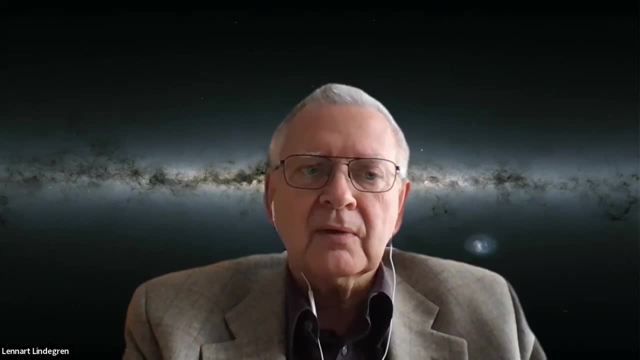 non-rotating system. And the simplest way to get a non-rotating system is to look for sources that are sufficiently far away that, even if they have large motions in space- thousands of kilometers per second- it really doesn't matter. They are so far away. 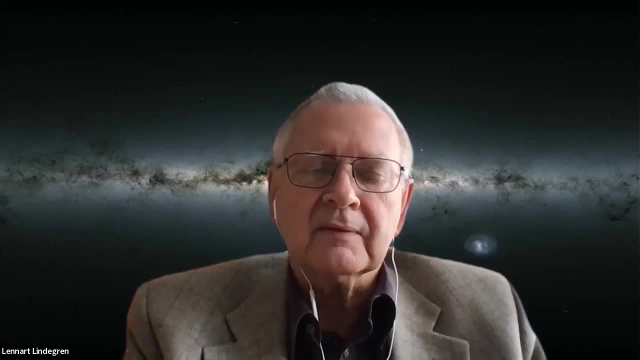 that they look to be stationary on the sky, And the quasars are the best objects we have for that, because they are very far away at cosmological distances and they are also more or less point-like like stars. So if you can observe stars to good. 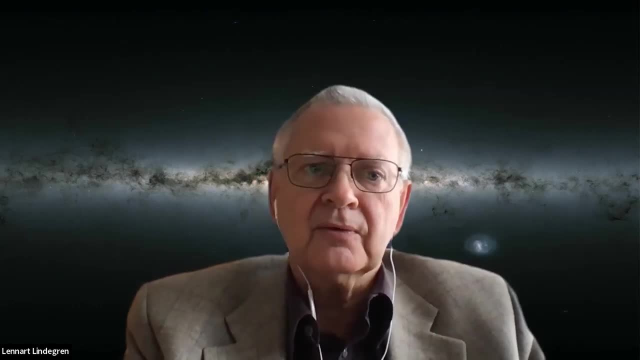 accuracy. you can also observe quasars to good accuracy. So, with Gaia, we observe a few million quasars, and they are used to define exactly this non-rotating reference system, And that is then very important when you want to study the motions. 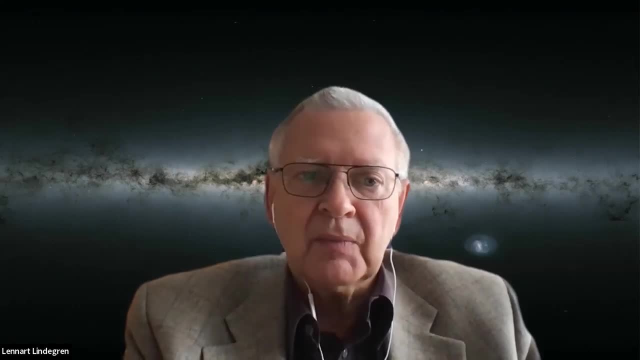 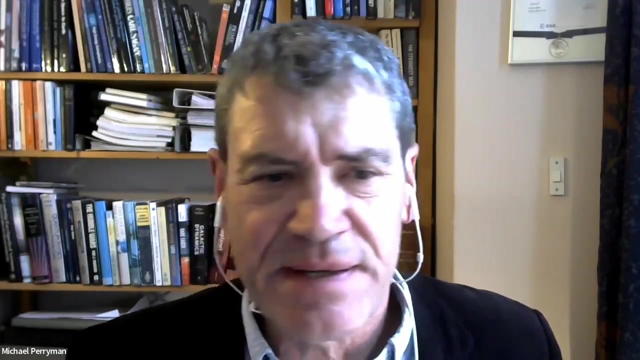 of stars in our galaxy, for example, or the motions in our solar system, asteroids and so on. For all of that you need a non-rotating coordinate system. May I take? there's several questions coming in and I must say how. 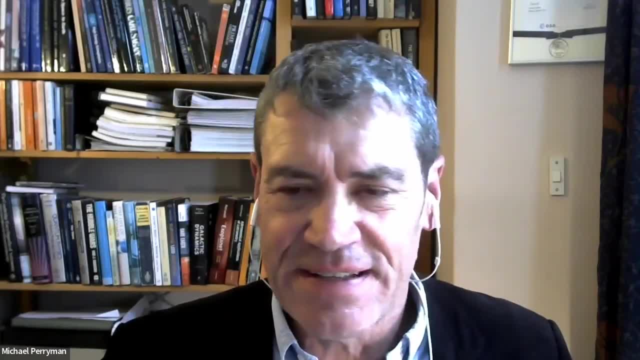 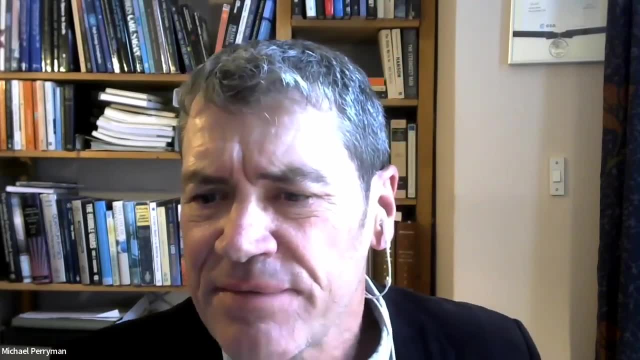 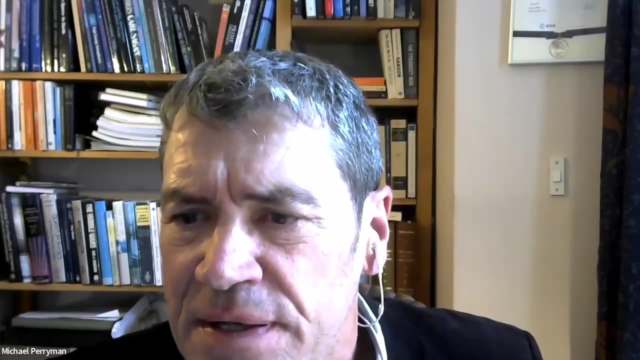 wonderful it is when you give a presentation to have interested questions which I think reveal the complexity of these missions. Can I see if I can take those three questions together fairly quickly? Sure, The first, Pearl Mong, has asked: is it correct to say that? 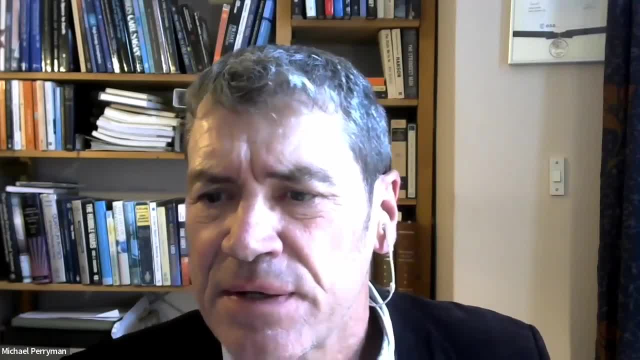 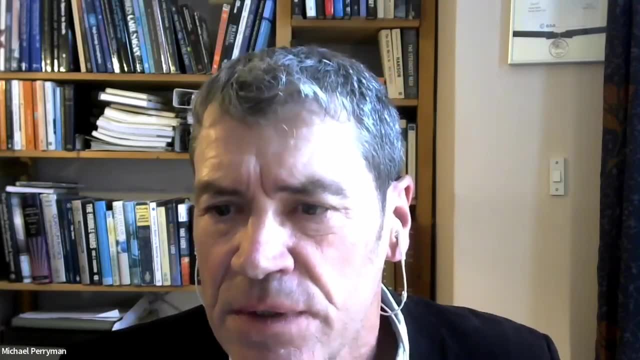 the definition of target stars, background stars and so on varies according to the location that Gaia is launched And, if so, how is the location picked? No Pearl, it's not correct to say that. The idea is: you can see, because the satellite is spinning. 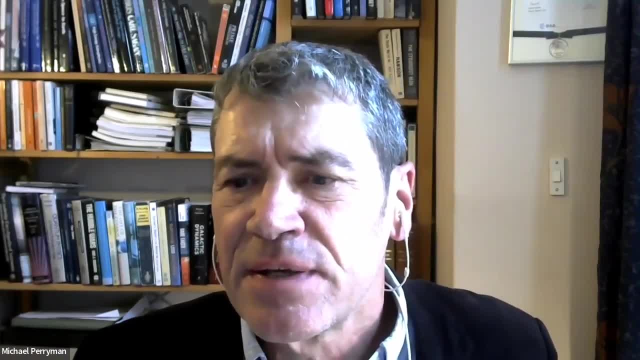 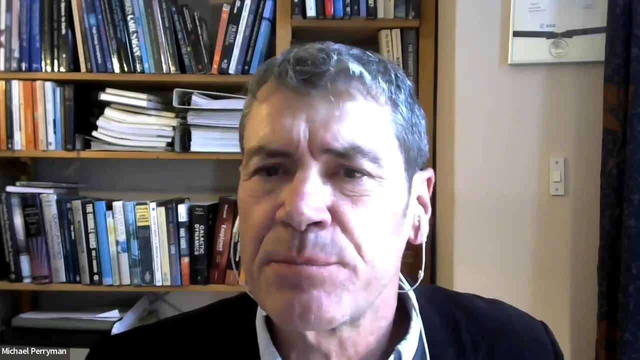 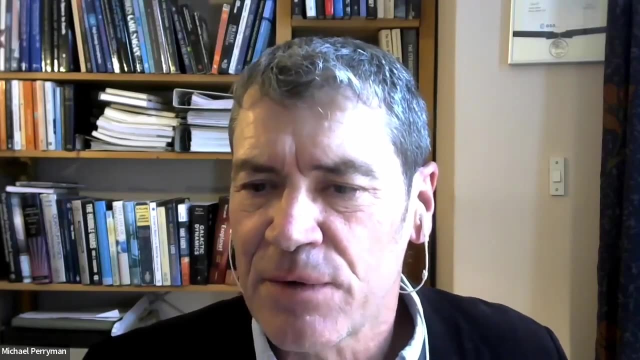 in the way that Professor Lindgren has described. you see the whole celestial sphere. you see all the stars and the question of which- where to launch Gaia and where to place Gaia- was just dictated by how the best possible physical location to place it, and we wanted to get away. 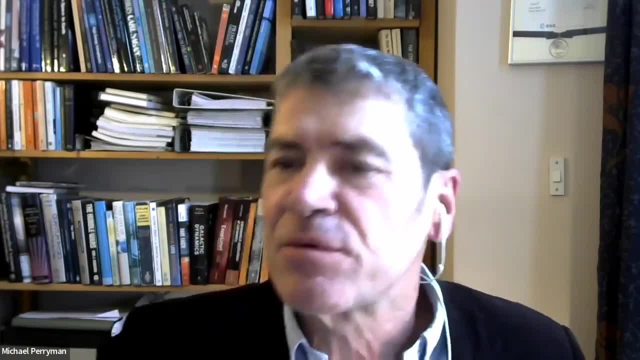 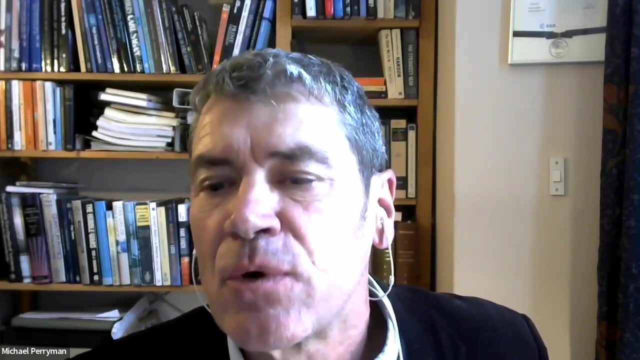 as far away from the Earth as possible to avoid several problems with radiation from the Earth and so on. and Gaia has been placed in something called the L2 Lagrange point orbit beyond the Moon, and we see the whole sky from there. so the 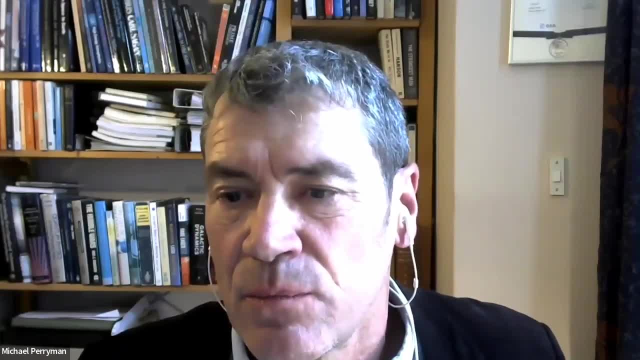 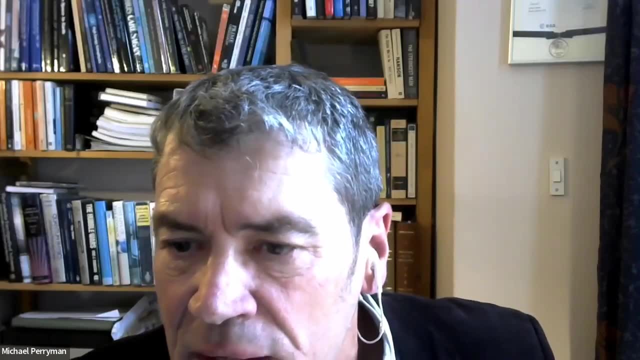 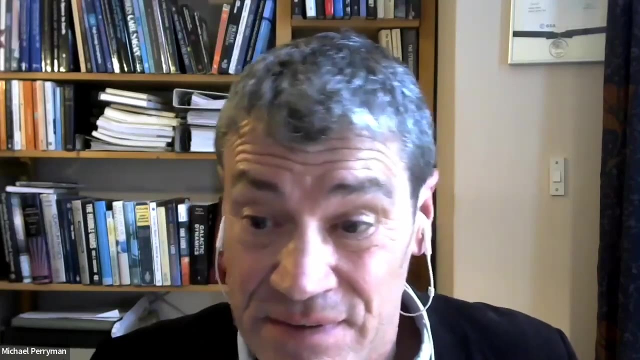 idea of target stars, background stars, doesn't depend on where we place the satellite. So Leung Chung has come, I think, a very important question that we didn't touch on at all, which is: what's the main difference between different data releases of the? 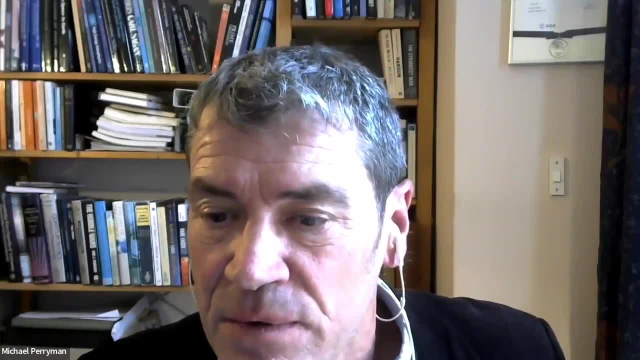 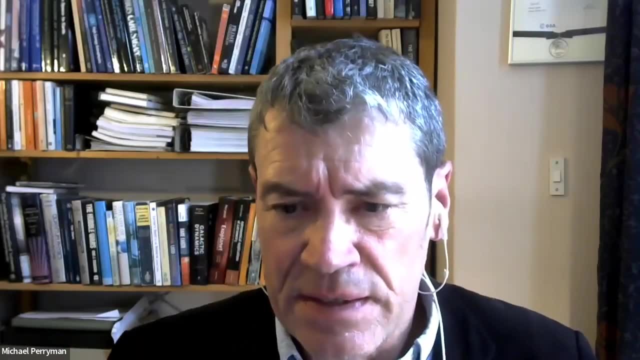 different catalogues? Are they mainly the time difference, or new data, analysis, or correcting mistakes? Well, it's a combination of all of those. in fact, The idea is that, as both of us have explained, Gaia will be operating for about 10 years. We didn't want to wait, and 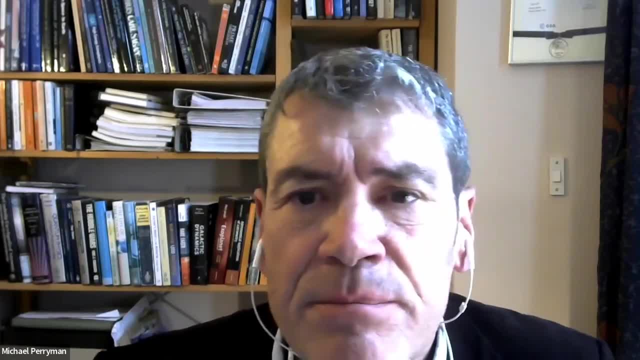 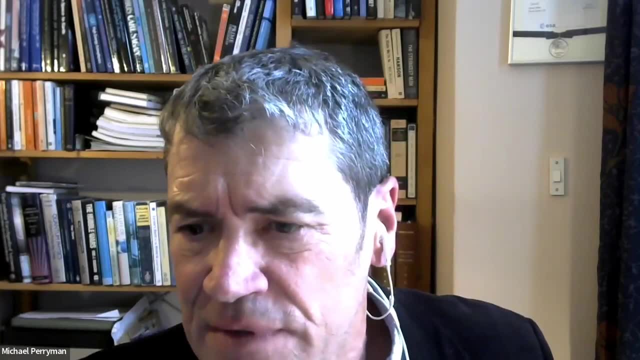 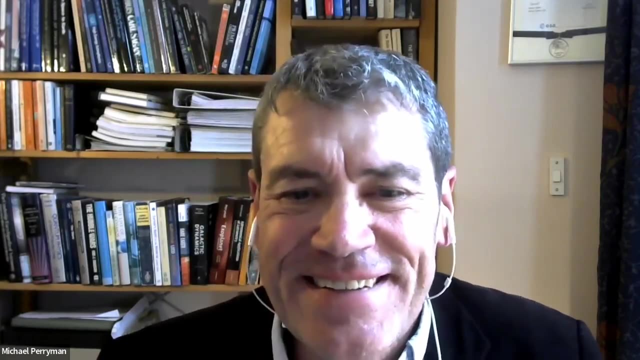 until the. in fact, I should point out, there's several people tuned in. Anthony Brown is listening into the Zoom meeting. He's actually chairing the entire data analysis consortium at this moment. The idea is not to wait for the full 10 years until 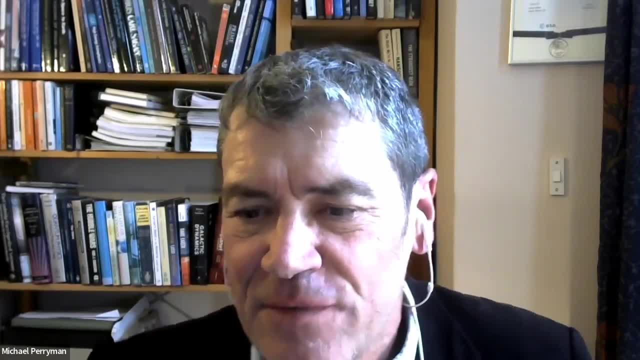 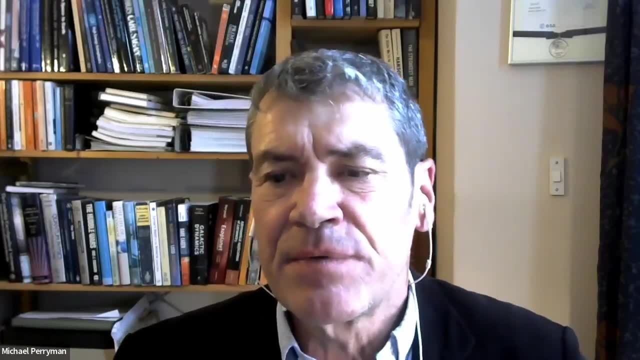 you have all the data and then give it out to the world's astronomers sometime in the 2030s. The idea was to take data in bunches, in packets, as it comes in, and the difference between the different data releases is just the addition of more. 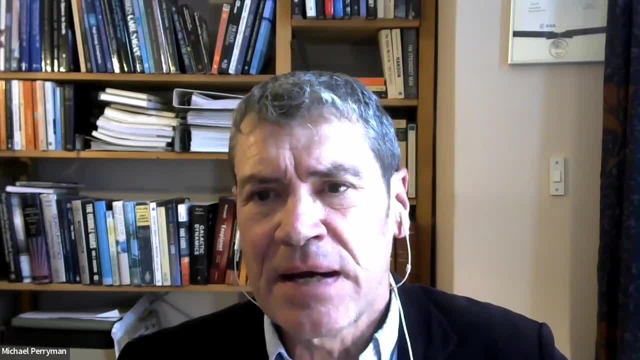 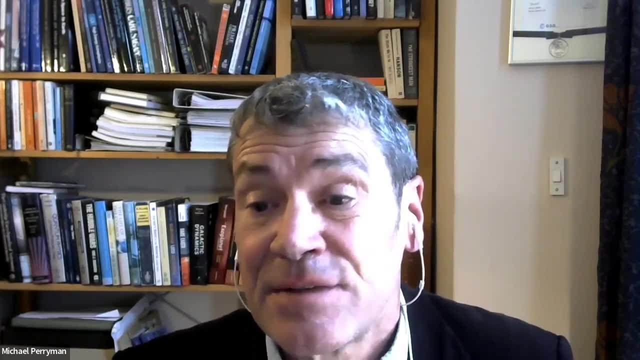 and more data with time. So the current latest data release, DR3, data release 3, is just based on the first 33 months of data. Data release 4 will be based on something like 60 months, 5 years of data And 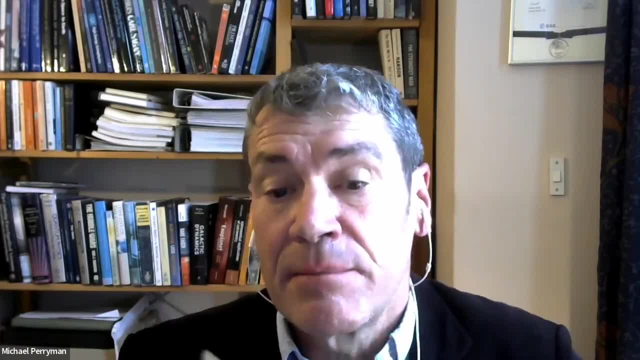 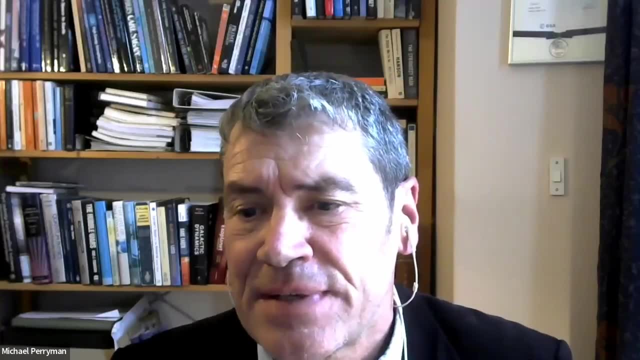 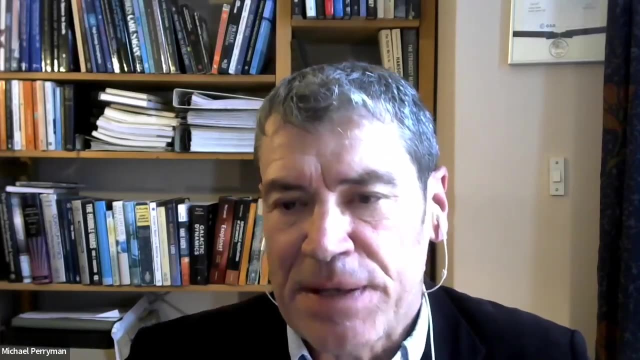 what happens is you're bringing in more data, completing more iterations and completing more interactions between, say, the photometric data and the astrometric data. So it's trying to come up with some compromise between the best possible catalogues that we have at this moment in time. 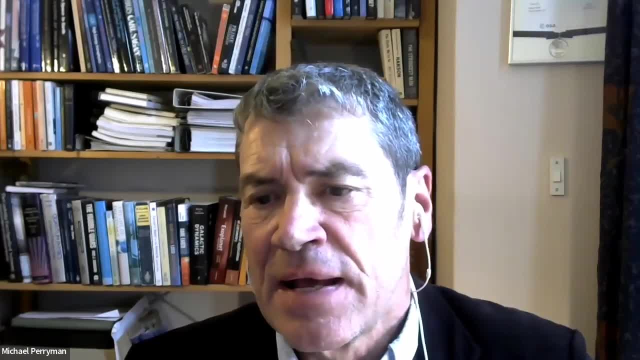 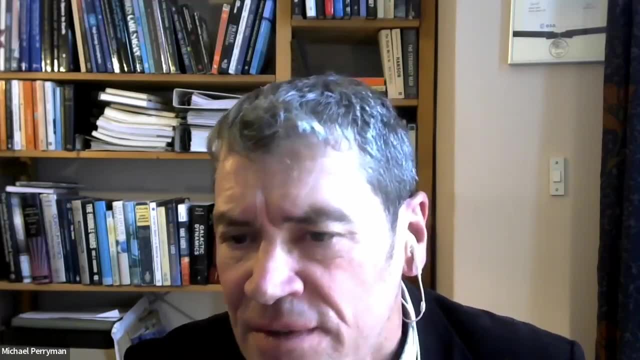 but not waiting too long for people to access it. So each data release supersedes completely the previous data releases, So you never need to go back to data release 2 or data release 1 or whatever. Data release 3 is everything and more. 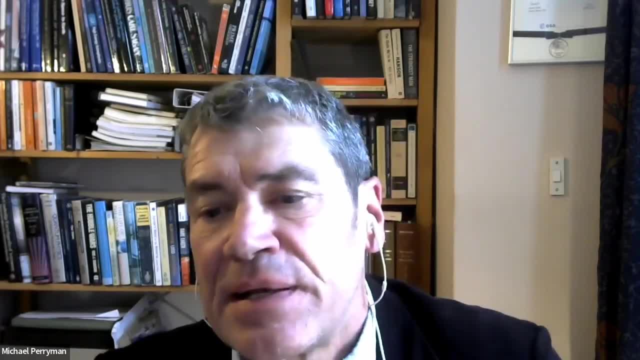 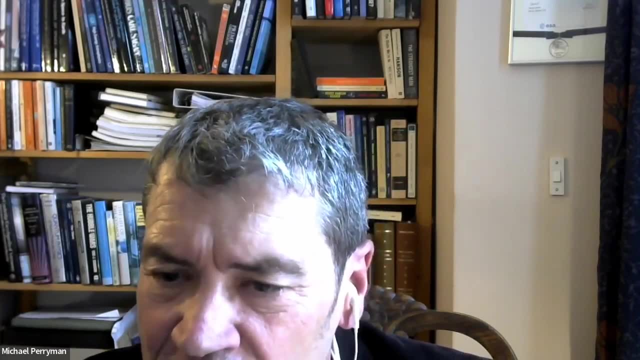 including the previous ones, And data release 4 will completely supersede data release 3.. And then, if I can take Michael Wong's question as well, You have two telescopes on Gaia. Will increasing the number of telescopes, if feasible, improve the?